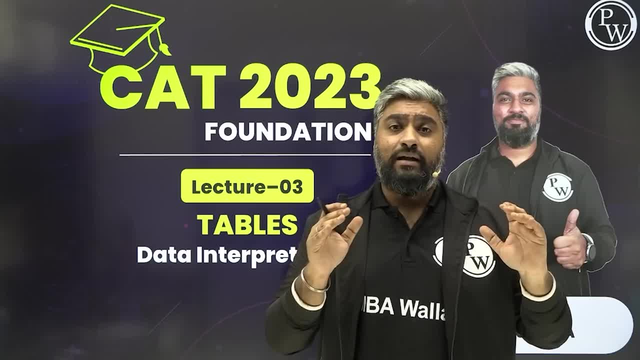 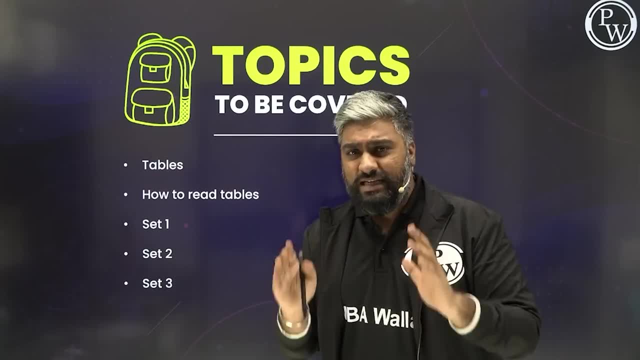 that get set. when it comes to you know DI specifically right And with tables, what are the things that you should keep in mind? So let's not waste any more time, Let's get started. Today's agenda is very simple. We're going to cover tables. 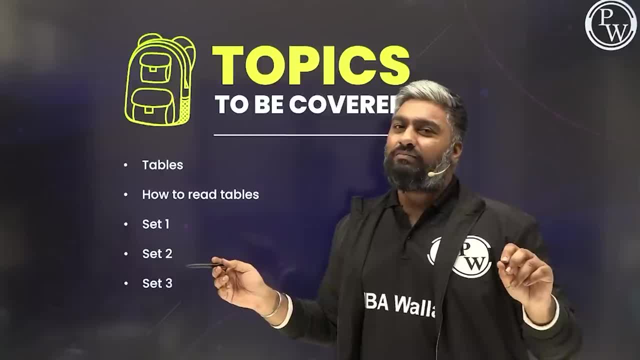 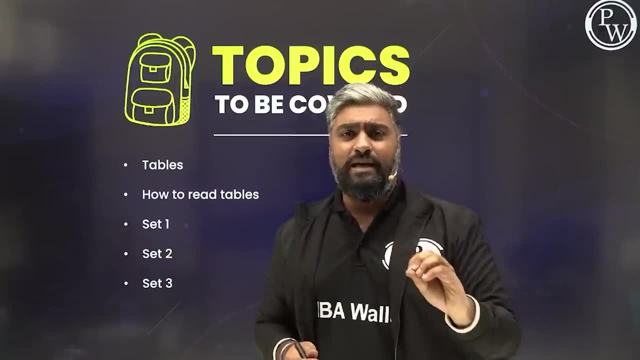 We'll quickly have a look at how to read tables. This is for people who've kind of forgotten, Yeah, or also for people who want to go through it once again. And we are going to do three sets today. Okay, three amazing sets, easy ones, yet effective ones. 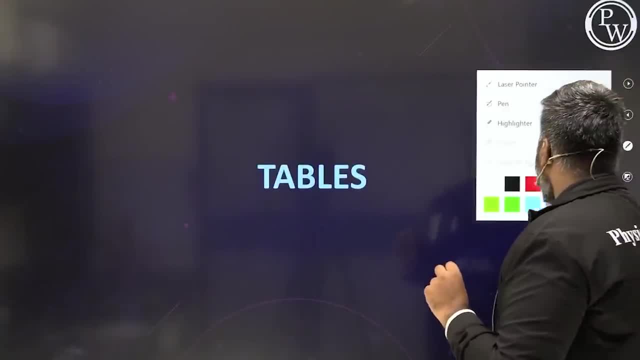 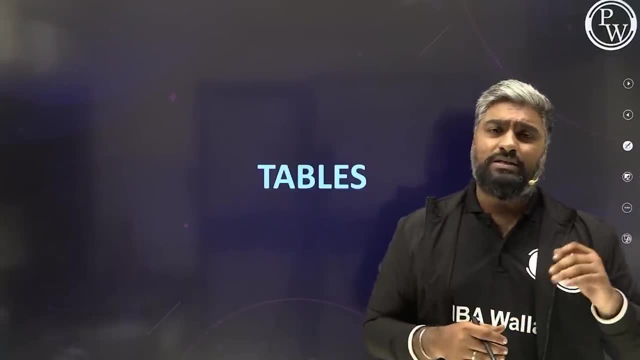 Okay, let's get started with tables. So we've seen over the years, tables gets that, the topic tables gets tested. you know, in your LRDI section quite frequently, right, You come across at least one set that has something to do with tables, if not directly. 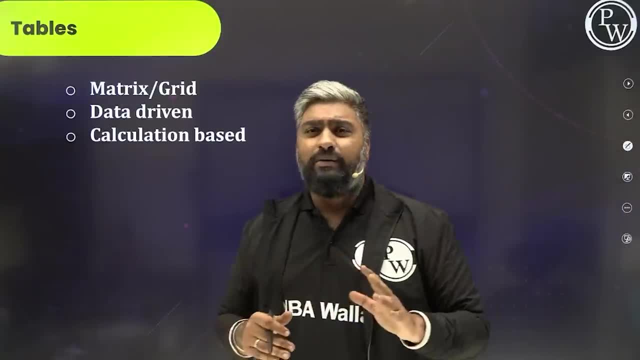 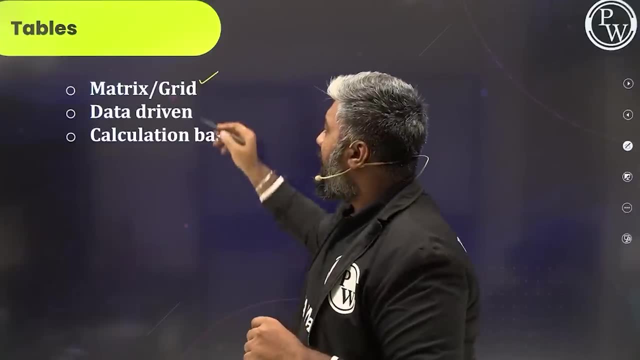 Yeah, let's get started. One you all know: a table is a way to represent data in a more organized manner. Yes, the data is given in the form of a matrix or a grid. Yeah, the entire question type is going to be data driven. 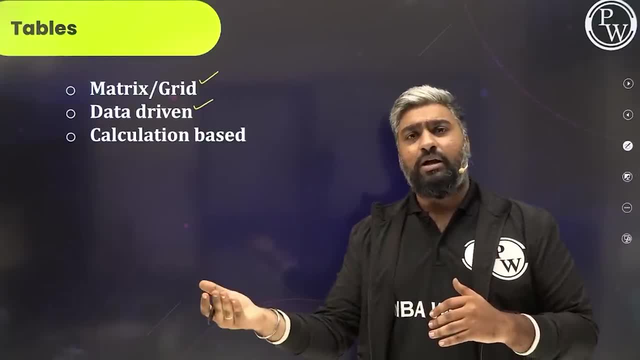 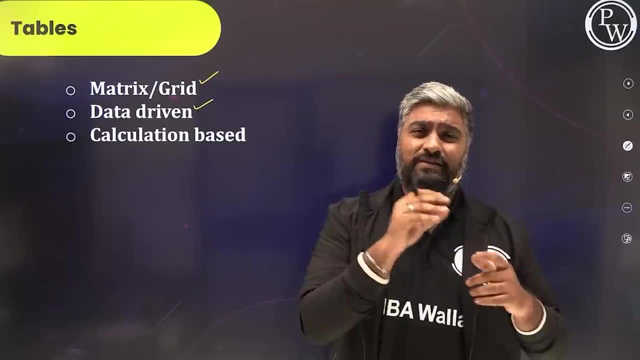 You'll have to read that data and figure out how to solve it right. Today We are going to do a simple tables right, Standard tables are going to do. we're not going to get into tables with missing data, tables that you know that are connected to some other charts. 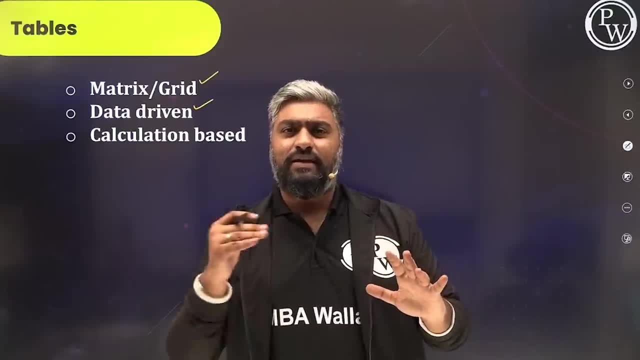 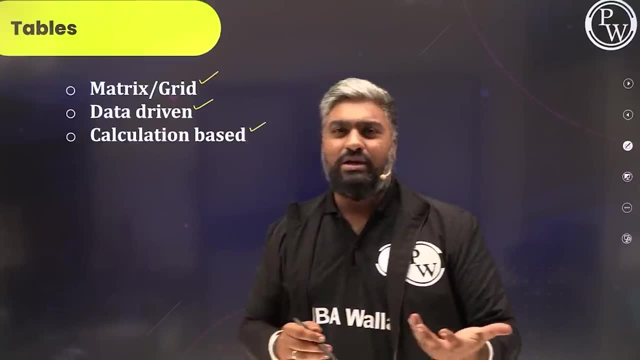 No simple ones, standard ones, because this is just our third lecture. We are planning on taking, you know, baby steps towards success in LR moving on, And we know that it's going to be calculation based. Of course. if there is data, then there will be calculation based on the data. 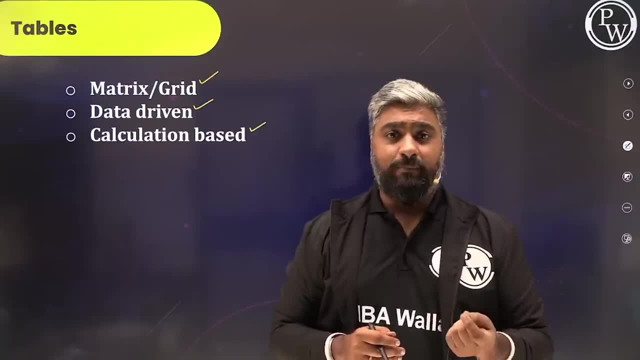 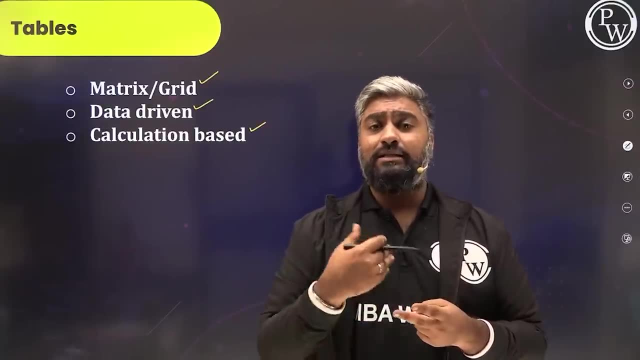 Yes, but then there are more than one types of questions that get asked in DI right. The two types of questions. One is obviously calculation driven right, Where you have to do the calculation. but the other kind of question has nothing to do with the set. 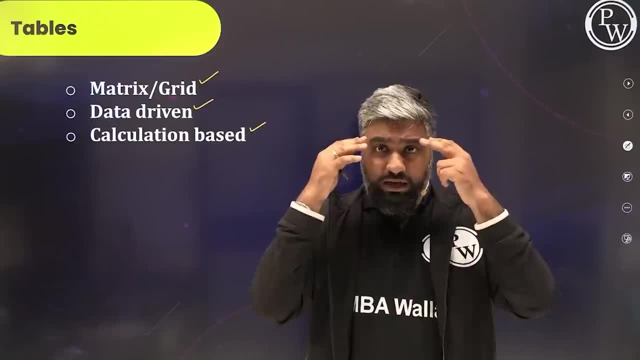 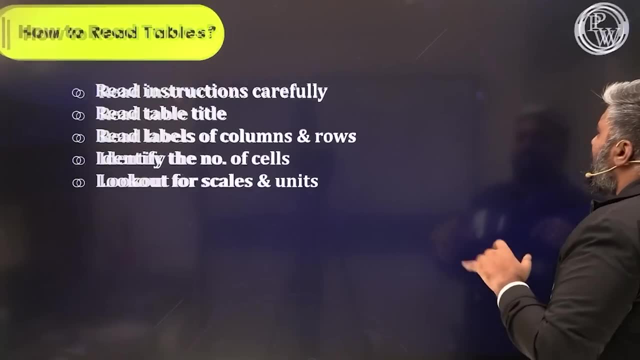 Uh, I mean the data. to be specific, no kind of calculation is done. you just have to analyze the table and answer it right. So analyze and answer. type and calculative type: two types of questions get asked in DI. We're going to see examples of both. 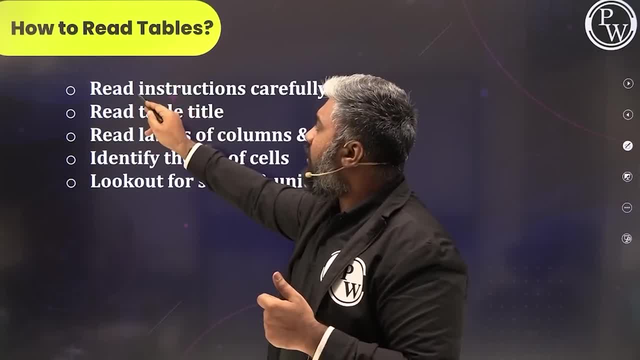 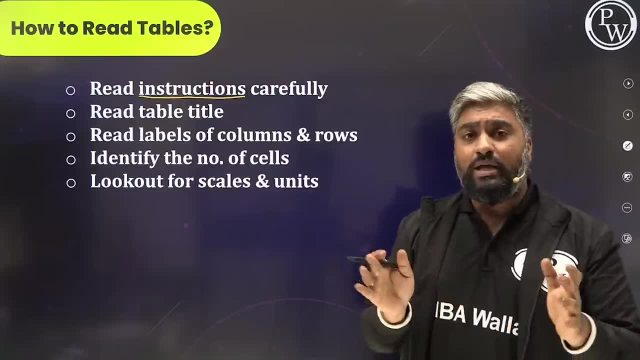 Okay, A few things to keep in mind. when you read tables Number one, do not forget to read this, often overlooked. Many people leave it think that, yes, they will see the table, they will understand how it is right. Don't do that. 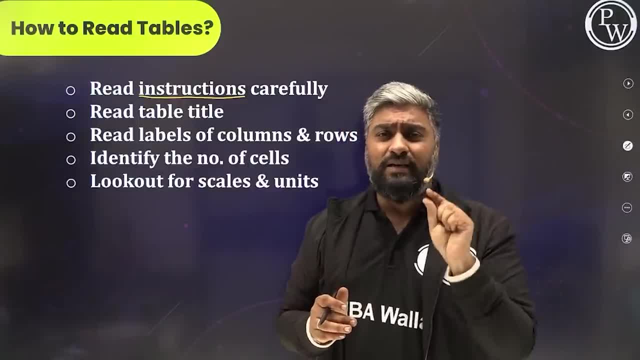 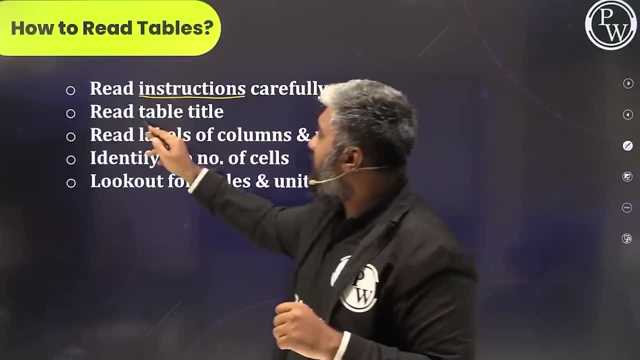 Spend time on the instructions. There could be key Pieces of information. Coffee Zara's already information. I put table key instructions where question statement may. hostess should do not miss out on reading that. Okay, And read the title of the table as well. 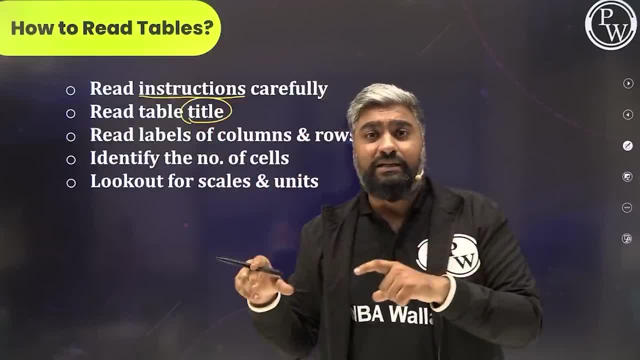 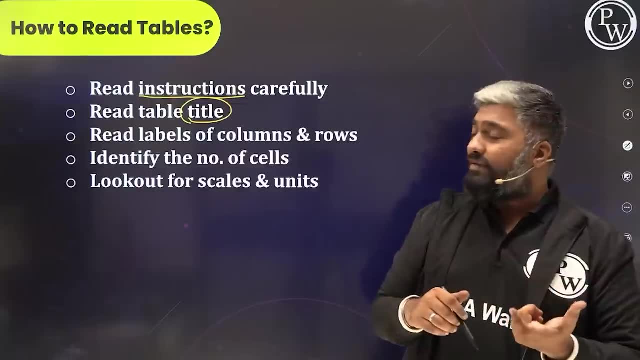 Yes, Table got your title. Have you said before that sometimes there could be multiple tables, so you need to know which one you're looking at. Sometimes there could be hidden information like scale, and the value could be given in terms of, say, uh, one, two, three, but 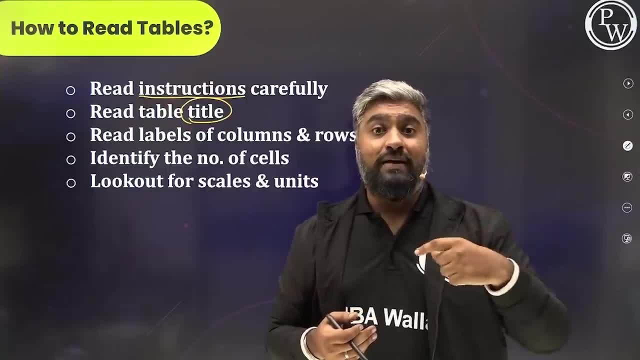 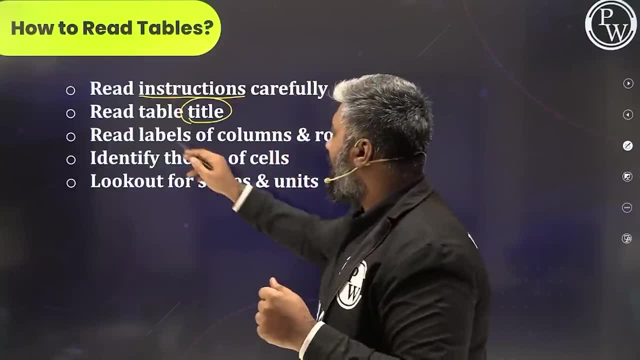 then scale media. these values are to be taken in thousands. Yeah, These values are percentage. right, We'll serve up for units scale. Yes, So Bob could be able to tighten the middle. That's what. do not forget to read that moving on. 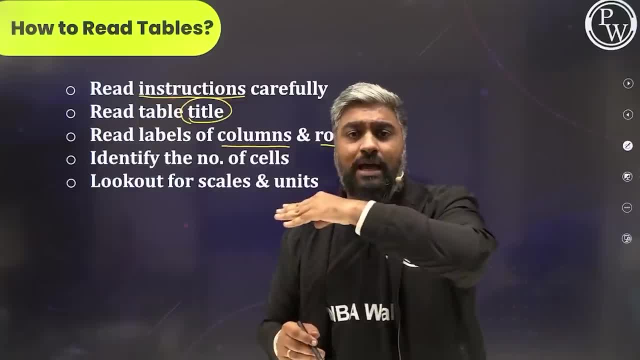 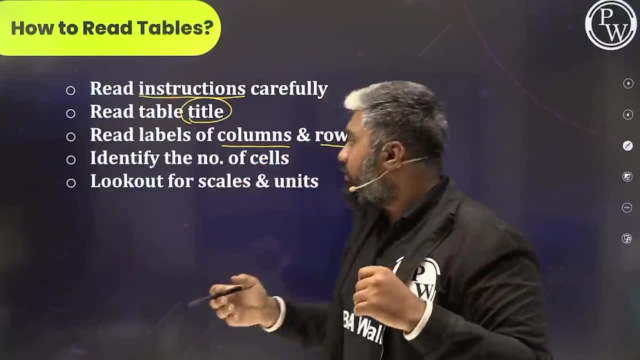 Do not forget to read the labels of the columns and the pros as well. Each column gas uh, uh, K, K, K K. type of data: Usman Hoga. each Roman case. type of data: Hoga. have a quick look at that while you're doing it. 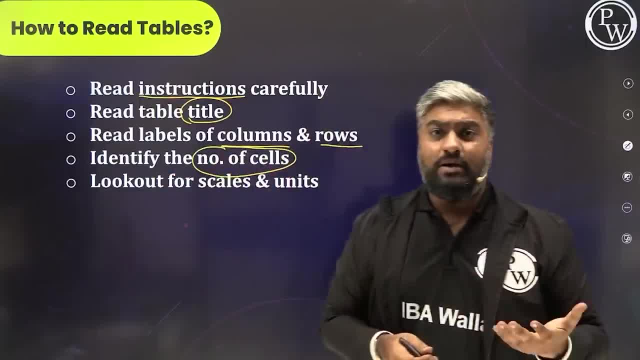 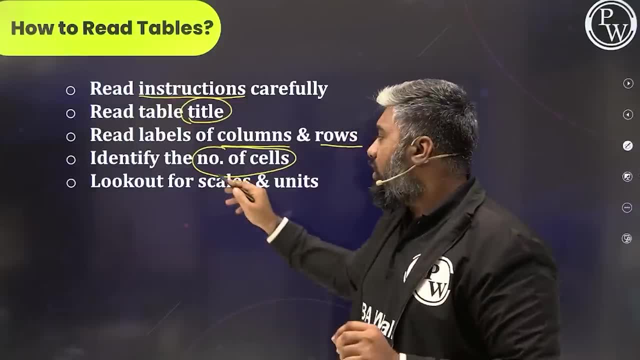 Also identify the number of cells. Yeah, That's a good answer. The Rooney identified corner, but then you will know the amount of data that you're looking at, right? I'll tell you how to do that as well, And always, always, be on a lookout for scales and units. 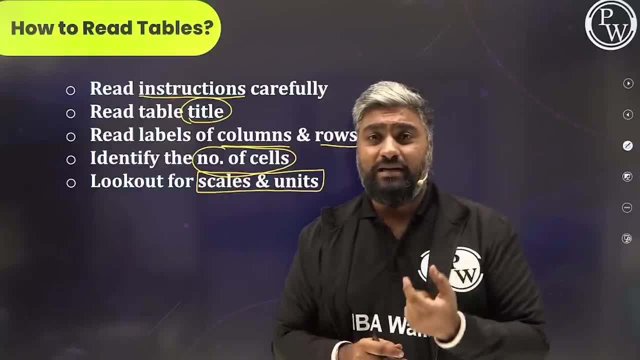 Yes, you do, Don't want to miss out on that. TK, Can you work out the data up for centimeter? My data but question may meet us My boots there right. So they mess. they mess with your mind by, you know, doing all these kinds of must carry. 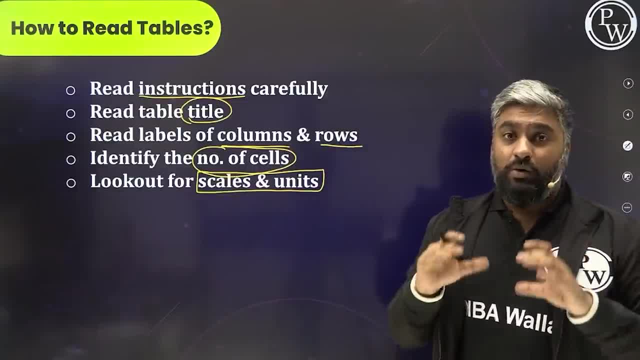 Okay, Yes, I'm musty Well as I got this, so you have to be super alert when you're looking at the chart for these things. Okay, Can you get it? Palace at KSAT right Enough, Yeah. 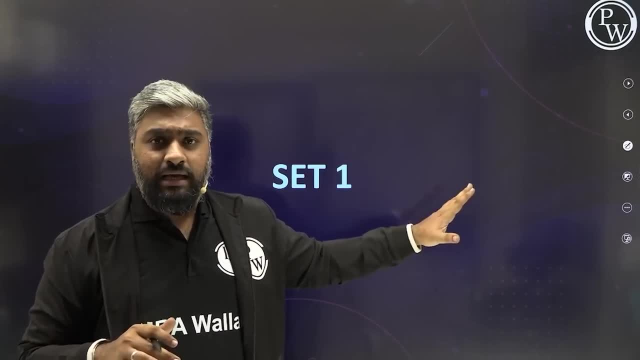 And Bazzi said that they sat myself. Yes, I'll first show you the set. I'll show you all the questions, Yes, And then we'll start. So maybe I'll go set, but I'm not questions, But I'm not there. 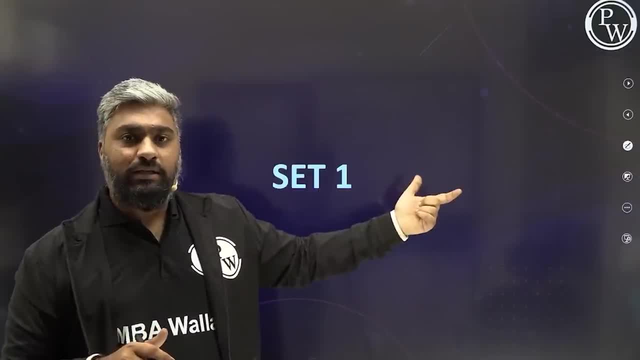 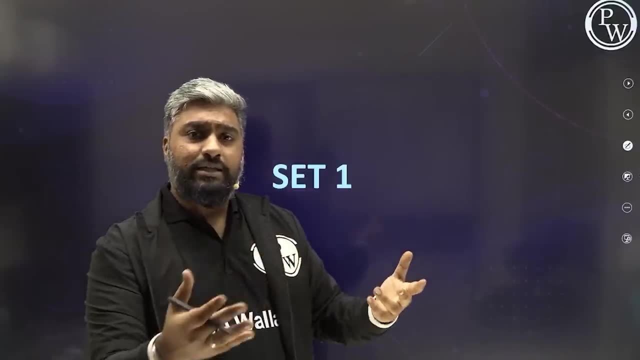 You can hit a pause, I'll solve And then continue with the- uh, the watching of the solution, right? Or if you think no, you want to try out one set with me and then the other two sets on your own. 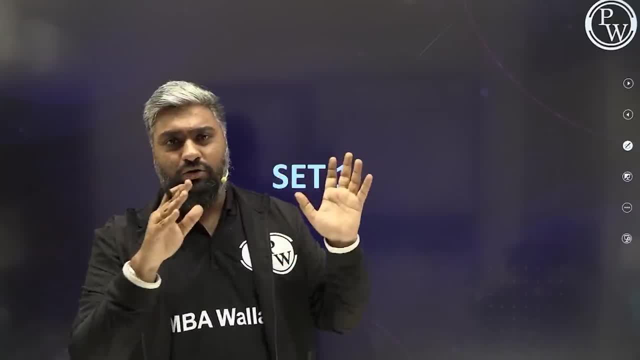 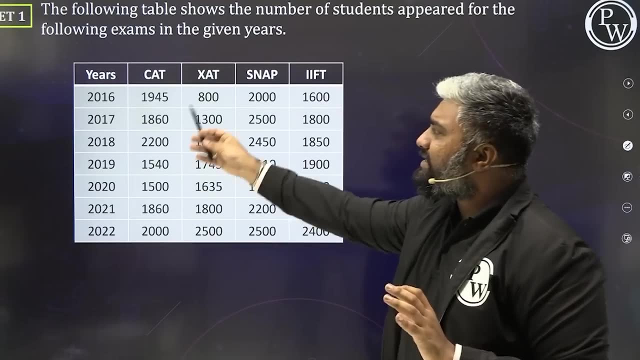 Jesse, be right up Molly case class. You want to pause, you want to solve and then you want to check out the solutions choices- Yours, Okay. So let's get started with the first set. This is set one. That's the simplest table. 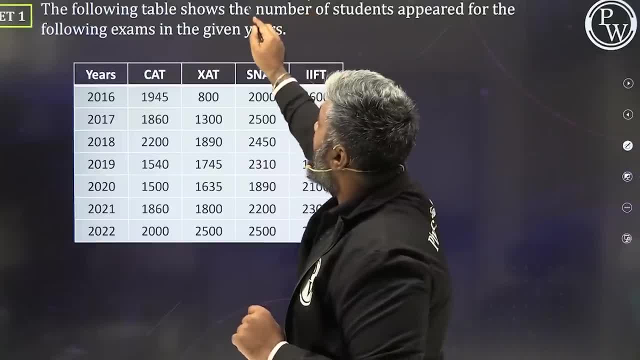 I am our repass right. They're saying: the following table shows the number of students. number of students, My unit Name, number of students Number is the count of this True Students, right? What's my point? 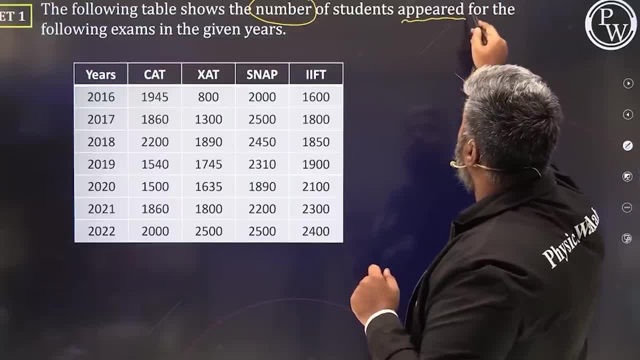 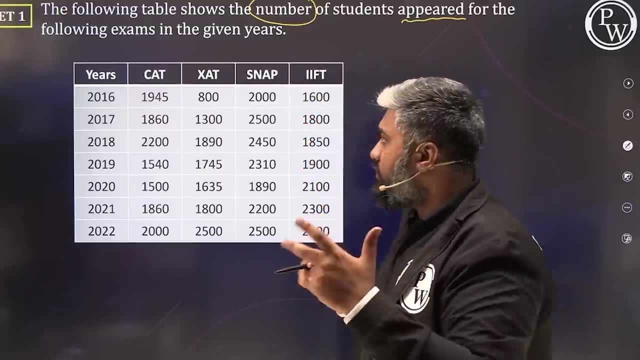 You need me. a very good number of students appeared, right, You're already up here for the following exams in the given years, So I might pass exams here and the number of students that have appeared for those tests. So you're like, Oh, for now, what do we see? 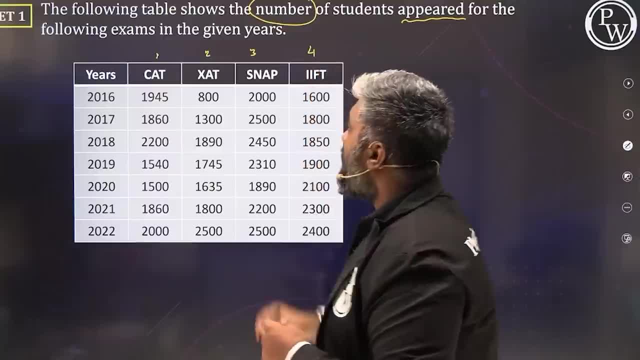 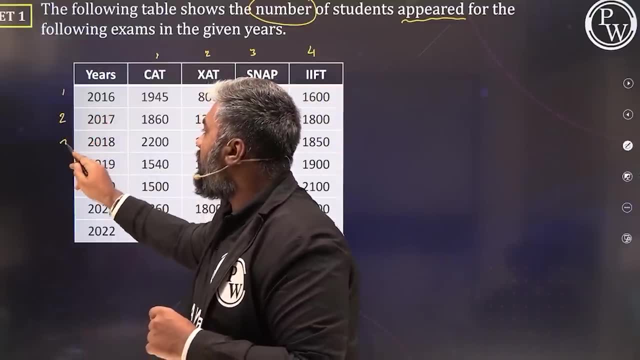 We see, first test the scat that snap, and IFT. So we have four columns, Yes, Four columns of data and yours The house, starting from 2016, all the way to 2022.. Yes, 16, select a 2022.. 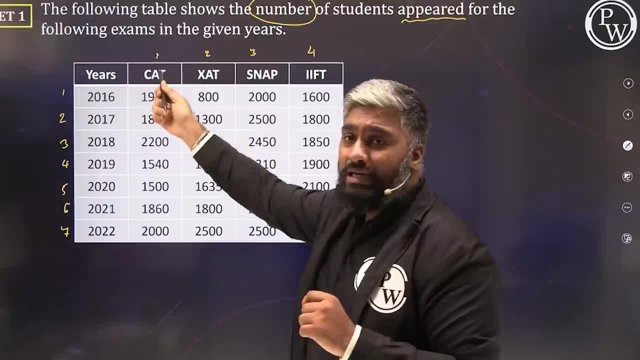 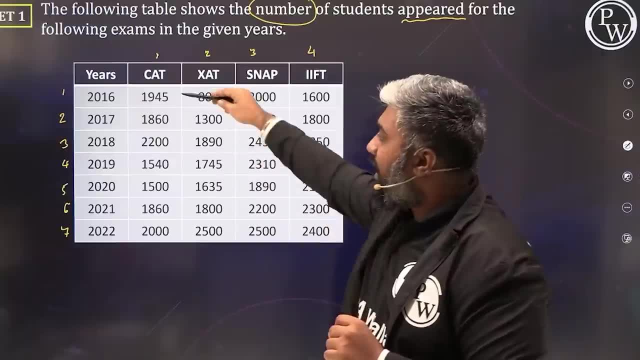 That is, seven years worth of data is given to us. Huh, But when they rose, they clearly columns. they clearly, yes. How to figure out the number of cells? Very simple: We have four rows, I'm sorry, We have four columns and we have seven rows of data. 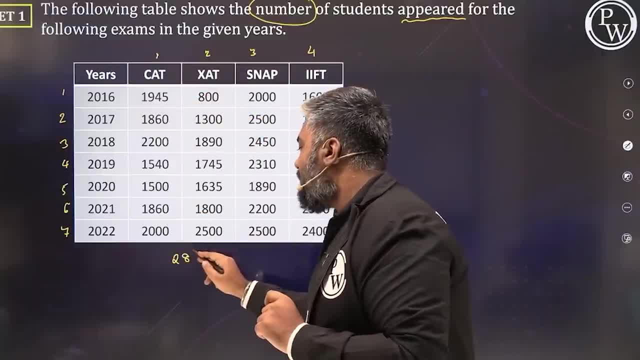 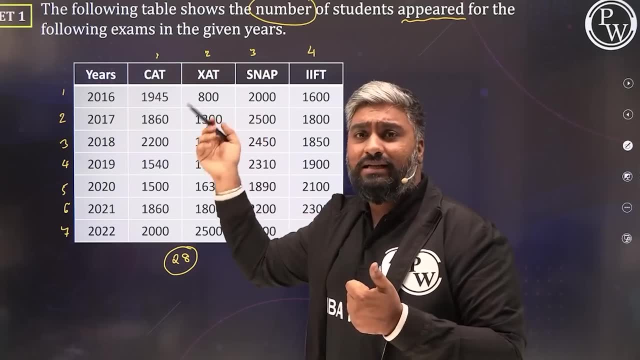 So four cross seven, 28 pieces of data. I have a market pass ticket: 28 cells at 28 pieces of data. Yes, Any uh scale given in hundreds and thousands in tense, which name data may put up? Cooper Nietzsche. 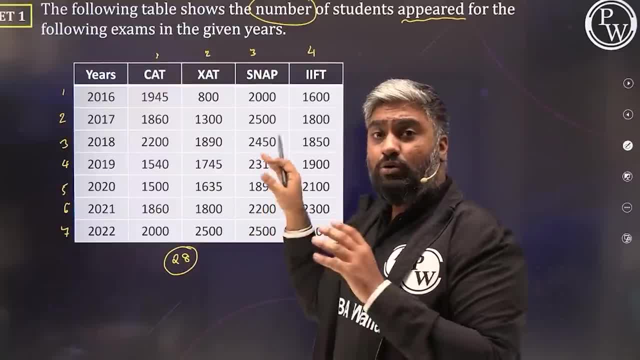 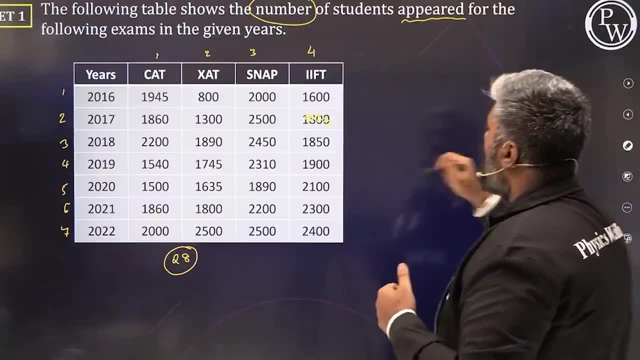 Dicker. No, we're going to quickly analyze. This is where the key other coach: you have a missing data, For example. if this piece of data is missing, then there could be questions arising from there, right? So we have to be on the lookout of that as well. 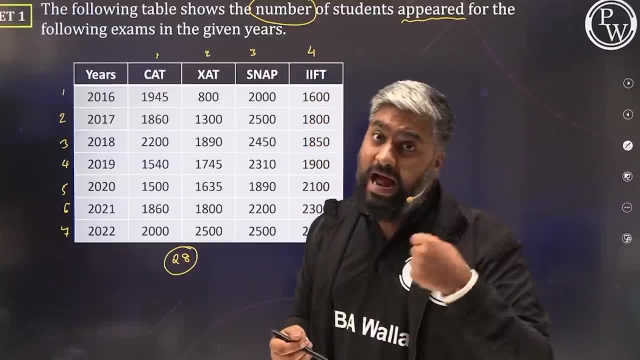 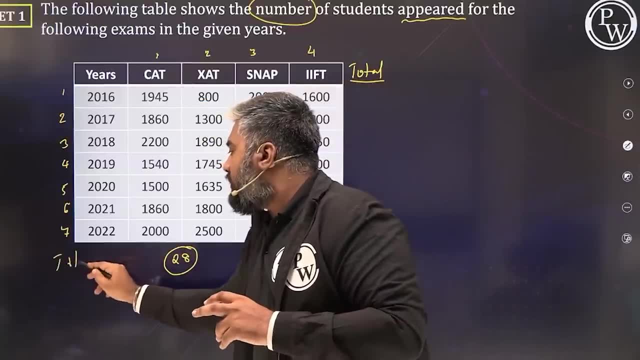 And you'll be there. Look, I hate pay. Sometimes what they do is they'll give you the total. Also, I had a good idea for the day: Another. another column could be total students in each year, right. Or another row could be total students, right. 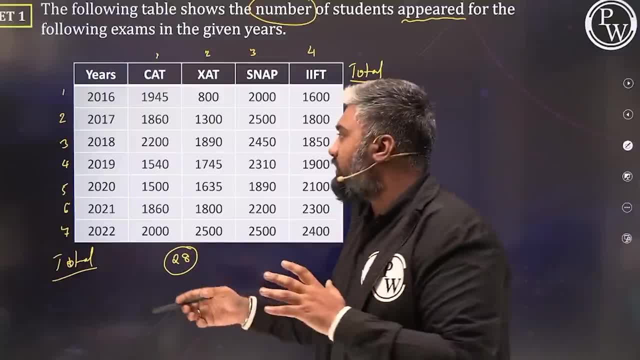 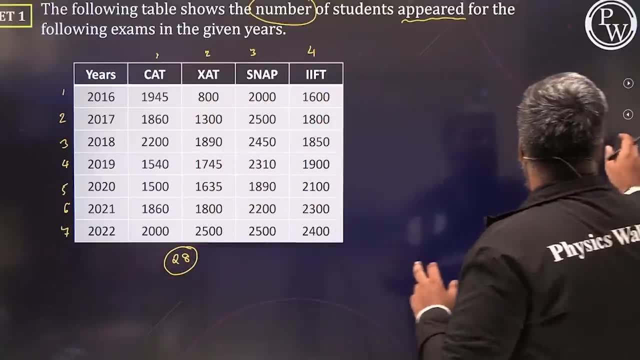 Total students for each test. So you have to be on the lookout for that. Also ticket. So as a coach we need. each piece of data is given in the form of the actual number, So it's not a scale, not a unit, not a table. no fun in the data. 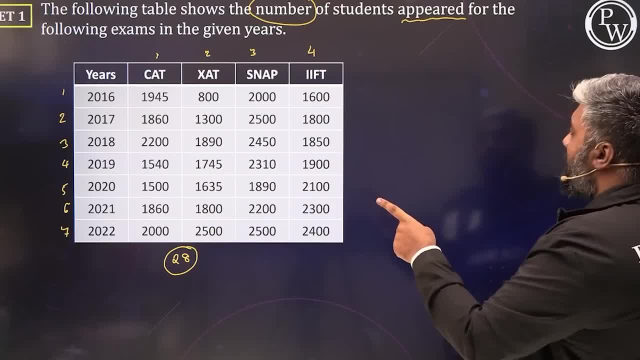 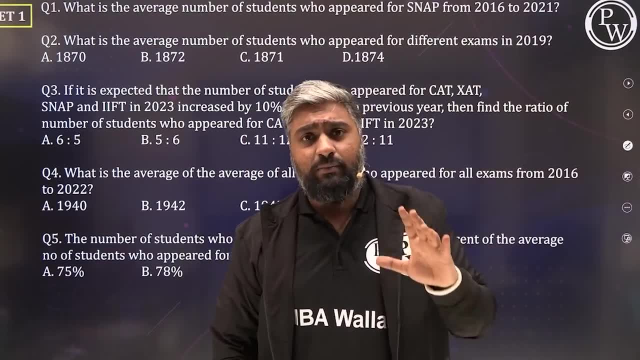 Everything is goody-goody. So here's the table and here's the question. Now you're going to get used to this whenever you look at a chart. specifically, if you're looking at a chart chart, immediately after reading it, have a look at all the questions, right? 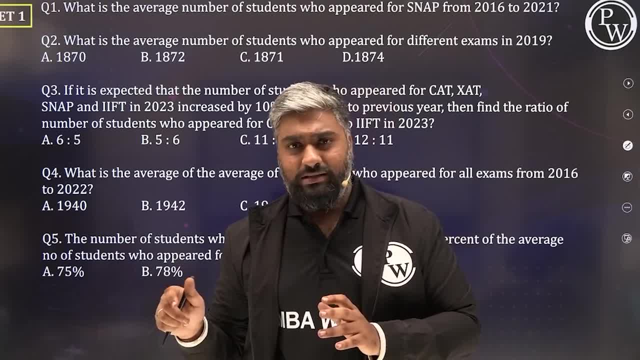 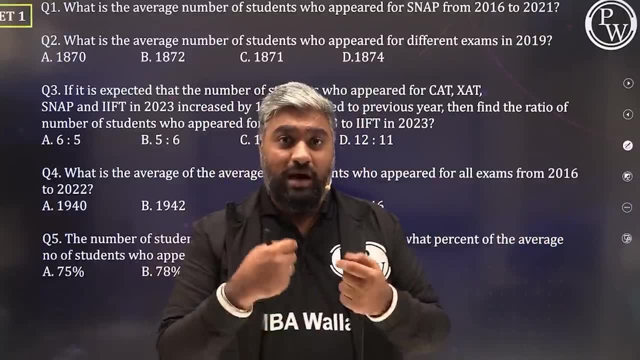 Whatever test will allow you to scroll through the questions, obviously, and not GMAT, secondary, right? That's something that we're not going to talk about. You keep going exams. You want that Well adaptive With them. you answer one question based on that. 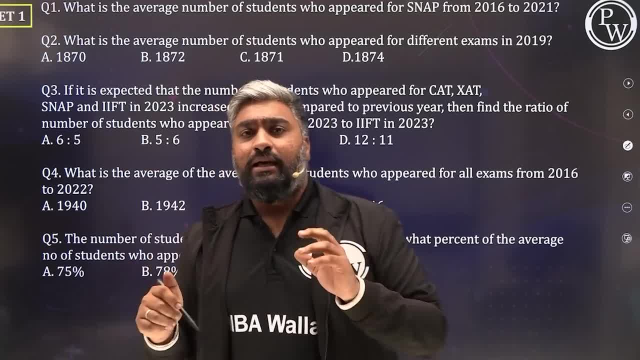 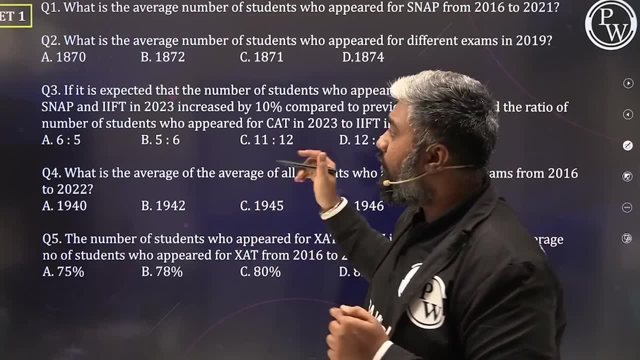 The next will appear to get that secondary, But for majority that is not adaptive to optimize questions. Then you have the liberty to scroll through it. right? It's called scroll through all the questions. Have a look out at the question, Okay. 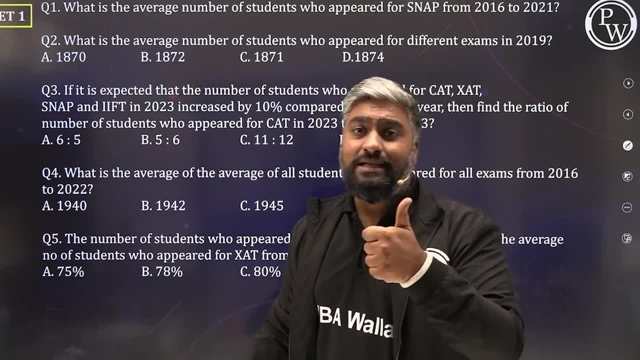 How am I going to approach Who got towards the chart? These questions will decide questions They go, answer choices They go and also figure out if there are any questions that are Tita. Yes, Tita, I'm going to miss it. 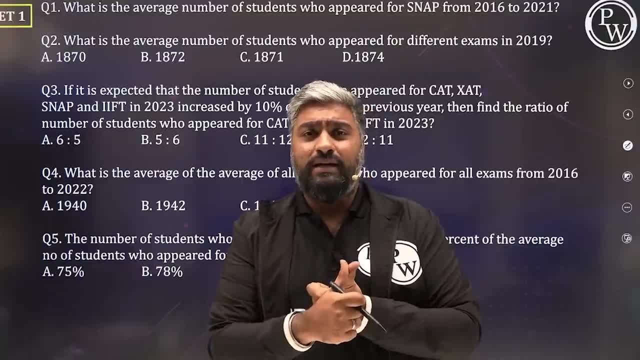 Not specifically. We're looking at my table. They can't. let's have a chart. They can't put so much money out Up. next question: They can put someone in there. but I'm going to put that together: Get Tita. 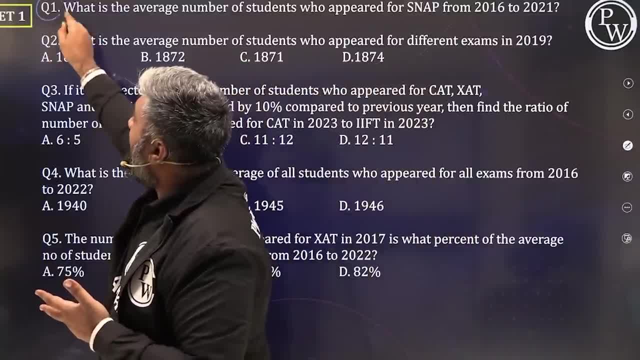 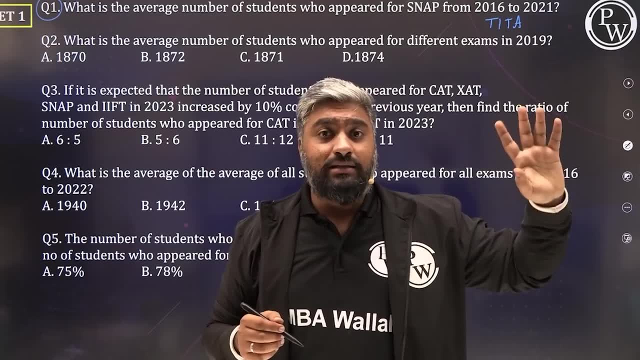 Right. For example, here in this question we have first question to be Tita Fella question. So I know, even if I don't understand the chart, I can still go ahead and answer the Tita question randomly. Q, key number one: no negative marks. 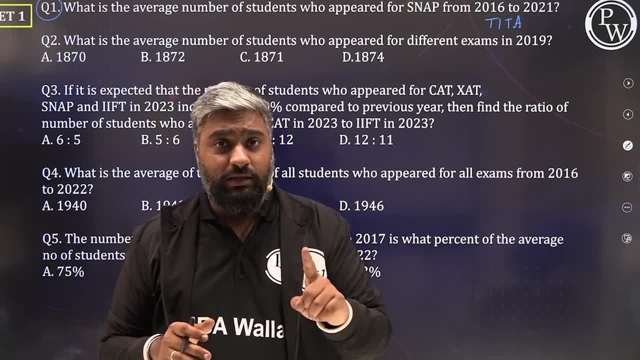 Yes, Tita me, Agar apka answer galat ho gaya, toh koi negative mark Nei hai. That's a very good thing. Number two: it's go answer Tana pe aapke number of attempts pe asar nahi padega. number of attempts change. 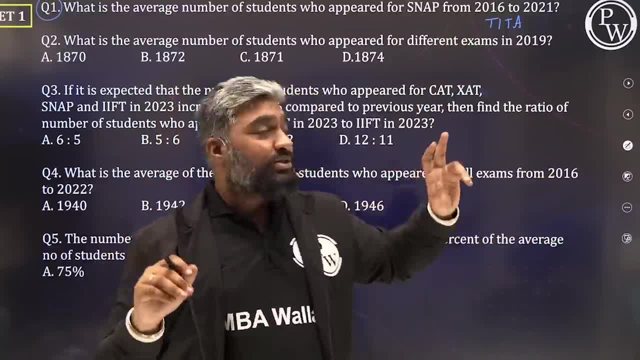 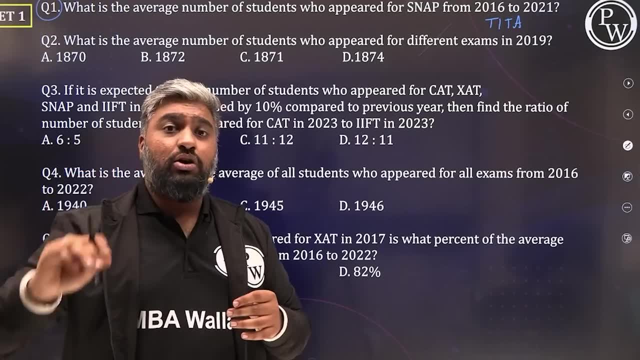 hongi: yes, but Q key negative marks nahi hai, So you can rest assured. So these are those, you know win-win kind of a Question type of Tita question. Do not leave them unattended. Tita question. make sure you attend them under any cost, whether or not, whether 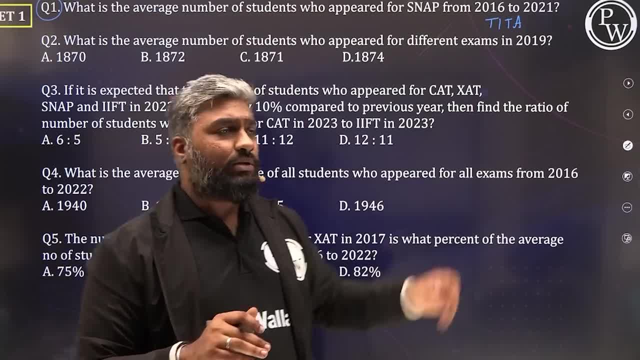 you're planning on leaving the entire set chalega koi rikkat nahi hai, but Tita question ko nahi chhodna hai. Okay, So let's have a quick look at the questions. also, What is the average number of students who appeared for snap from given years? 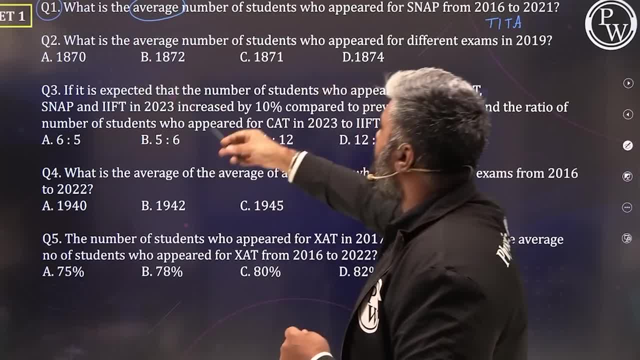 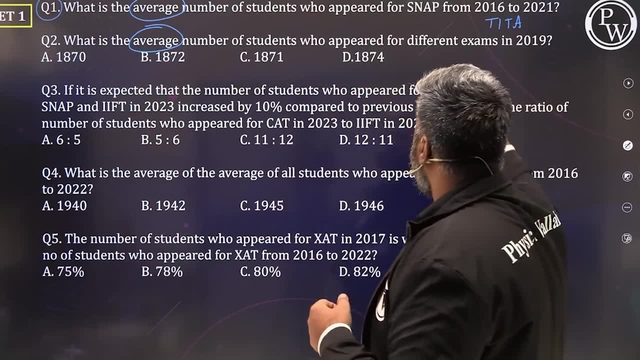 Average dhundna hai. Okay, For that data ki zarath padegi. What is the average number of students who appeared for different exams in 19? Average, again, calculative hai data ki zarath. What if it is expected that the number of students blah, blah, blah increase hua hai? 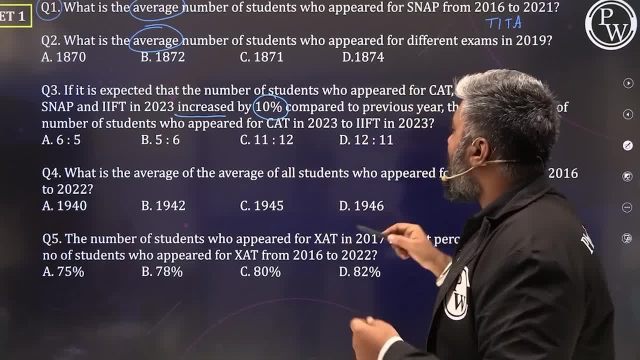 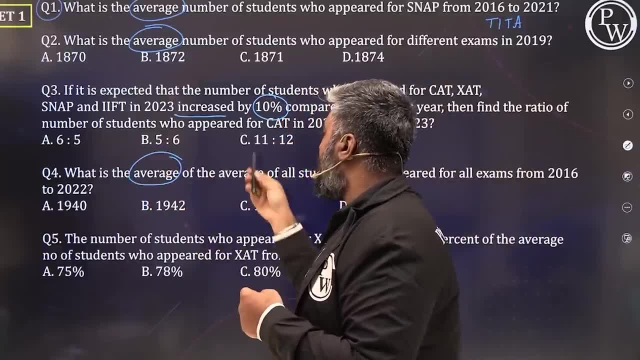 10 percentage. So percentage values increased and they're asking for the ratio. Okay, Very good question, for what is the average of the average? average to dhundna hi hai, but uska bhi average dhundna hai of all students who appeared for the exams from 16 to 22.. 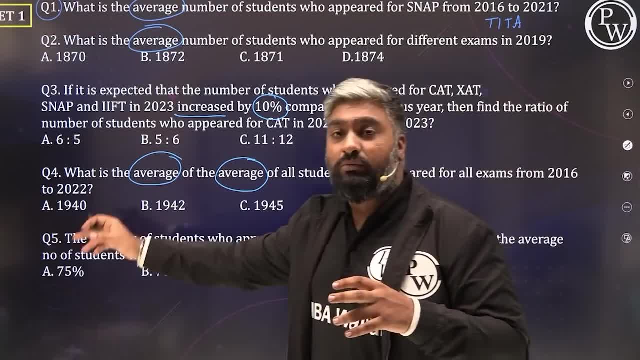 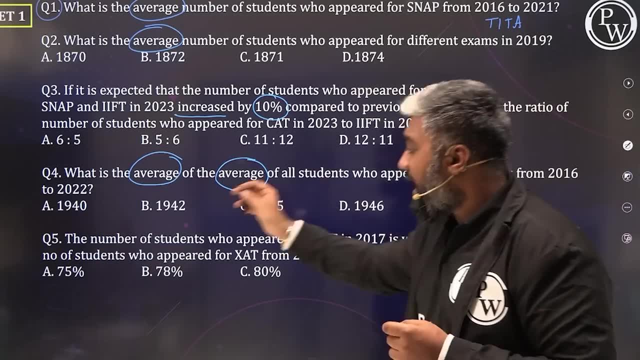 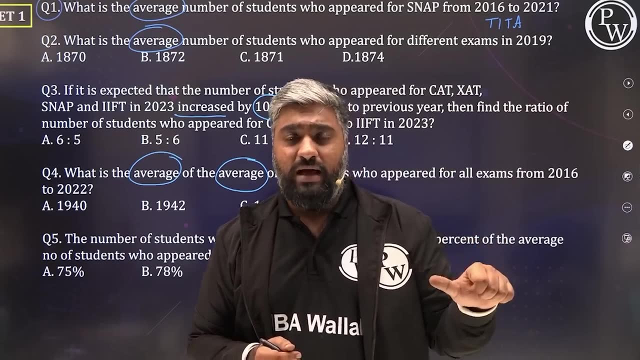 Mallab, kya aisa? koi bhi piece of data nahi hai jo miss out ka sakte, especially for the fourth one, right Kaafi heavy hai right in the set. We have a lot of questions from average, So let's keep that in mind. 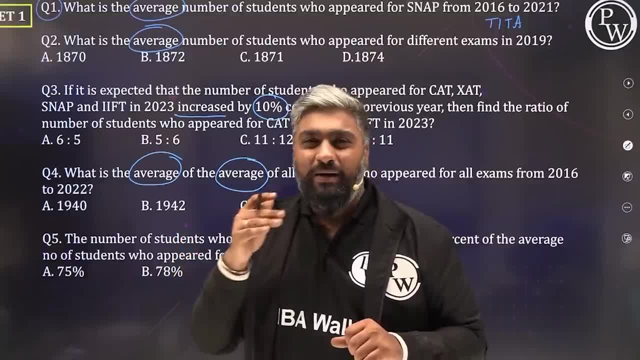 Okay, Another disclaimer. ye question aapke DPP mein hai, So I'm kind of helping, kind of cheating on you know, helping you how to solve that particular question from your DPP. Yes, I've taken only one question from your DPP. 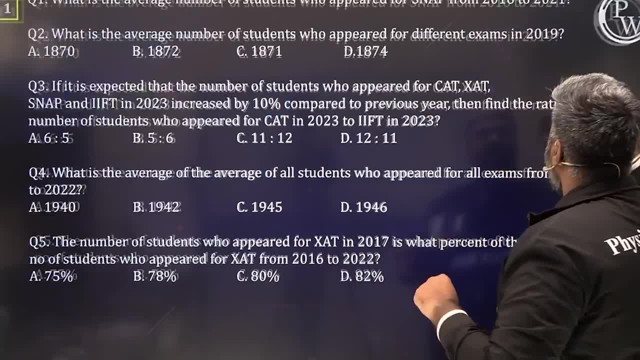 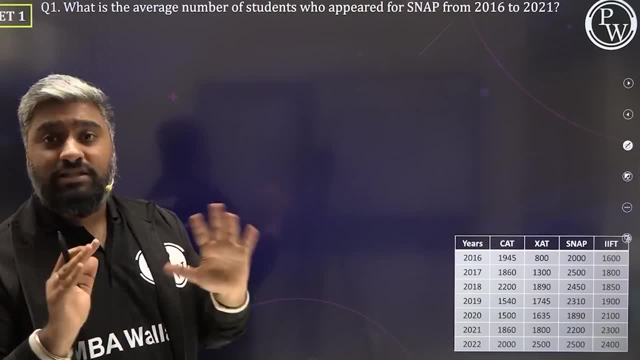 Two other questions are fresh ones. The other set jo hai wo fresh hai Chalo, let's get started. Let's have a look at the first question Table. maine yaha pe rag diya Aapka your exam, your test interface. 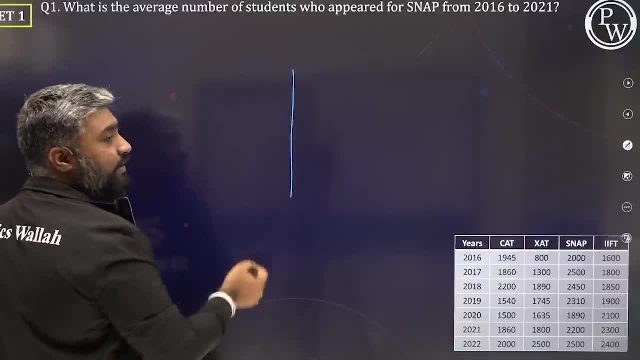 Aapka jo test interface ho ga. O bhi aisa hi ho ga. Your screen will be divided into half. On one side you will have your chart and your question and all that Chart, question, wo sab rahega. 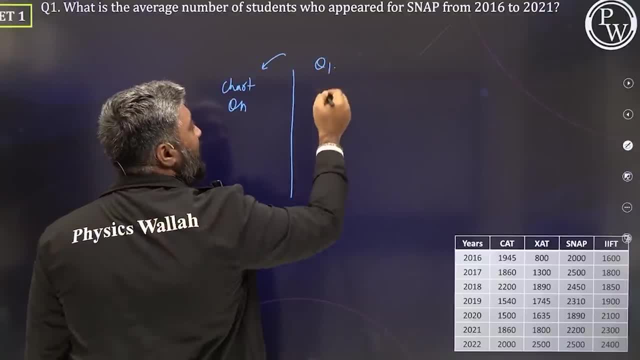 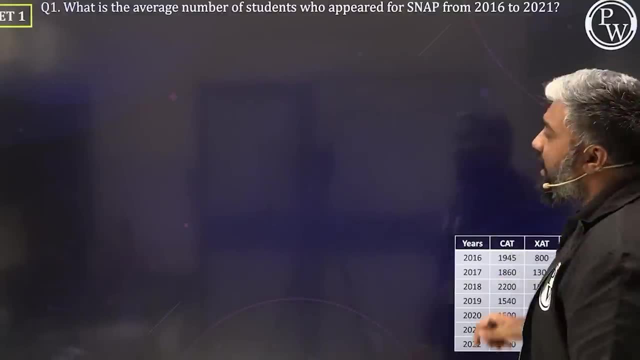 Question statement: jo instructions wo sab. On the other hand, you will have question one and blah blah blah, the question answer choices, if there are any. Theek hai to aisa rahega aapka interface, which means you'll be able to see the chart. 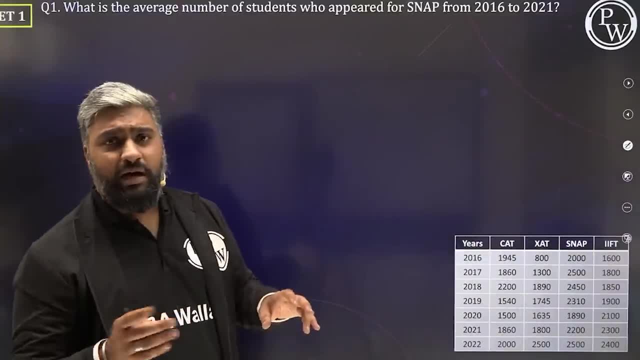 the questions, the information. at all times Theek hai to aapko scroll karne ki baar baar idhar udhar panne ghuvaane ki zaurat nahi hai. Panne ka to scene hi nahi hai. everything is computer based. test na right. 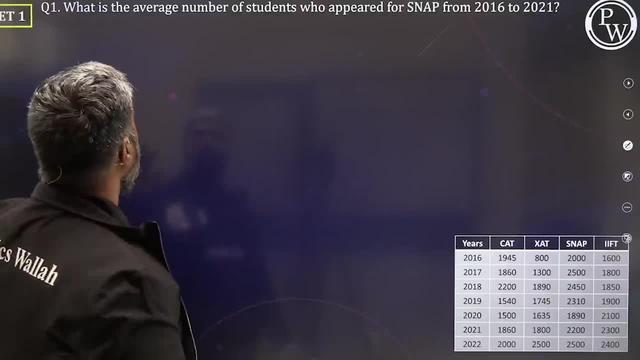 But still you don't have to be on the lookout. Theek hai scroll baar baar karne ki zaurat nahi hai. So what is the average number of students who appeared for SNAP? from 16 to 22?. 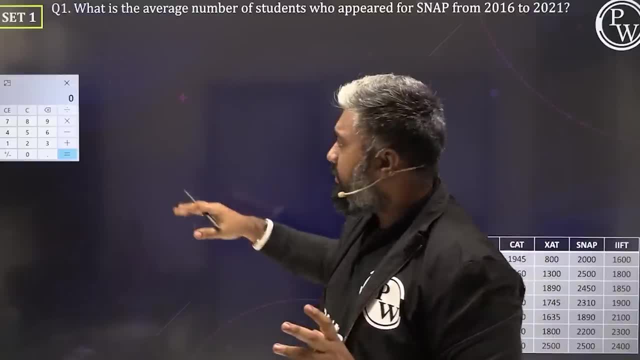 To chalo. let's have a look at the first question. Hume pata hai yeh poora set calculation based hai to hume calculator. laga diya right. You will also have access to the calculator, especially for CAT. 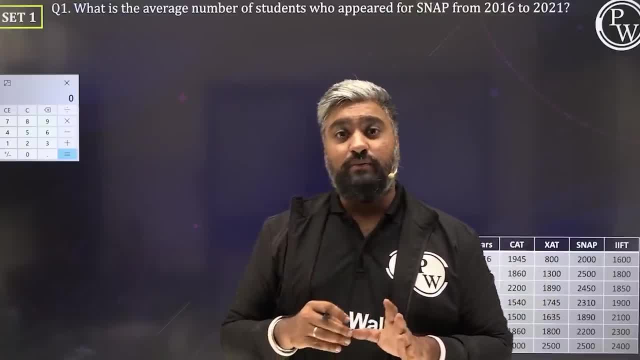 Other tests, like ZAT, SNAP. they won't give you an onscreen calculator, so you will have to make do without them. Theek hai, So let's quickly get on with this. Our first question is asking for the average number of students. 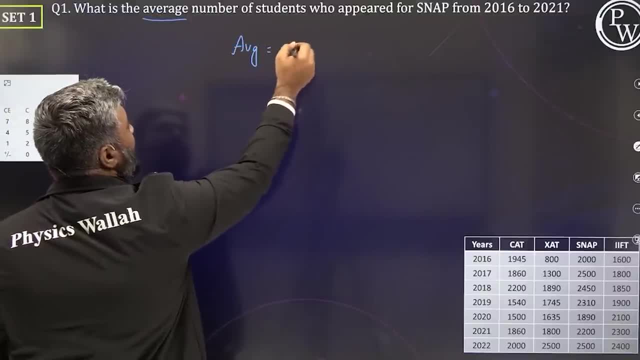 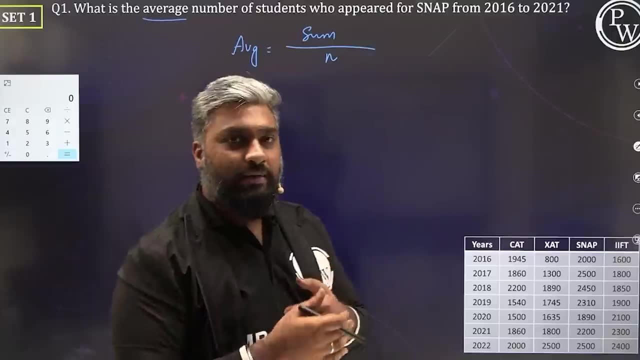 To average bola hai. we know average of anything is going to be what? Some of the number of terms, Some of all the terms, Appointments On the number of terms hai na. So hume sum dhundna hai phir usse divide karna by the number of terms. 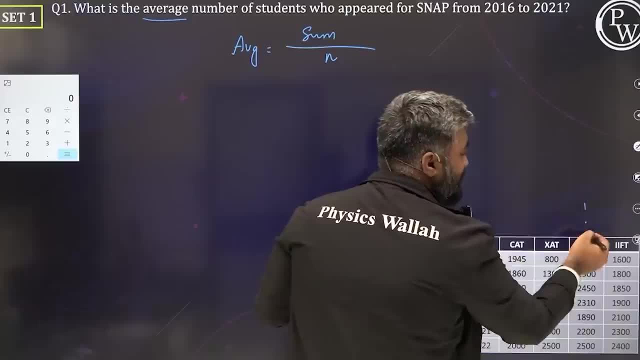 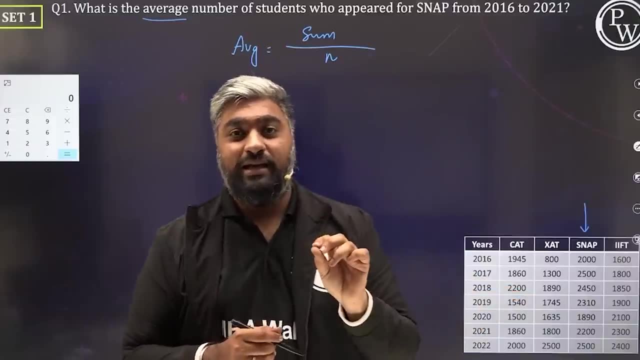 So average number of students who appeared for SNAP. SNAP ka pucha hai matlab sirf, iss column pe hume dhyan dena hai, not any other column. from 2016 to 2021.. Ab yaha pe aapko bohot carefully, yeh cheez dekhni hogi ke table mein from 2016 to 2022. 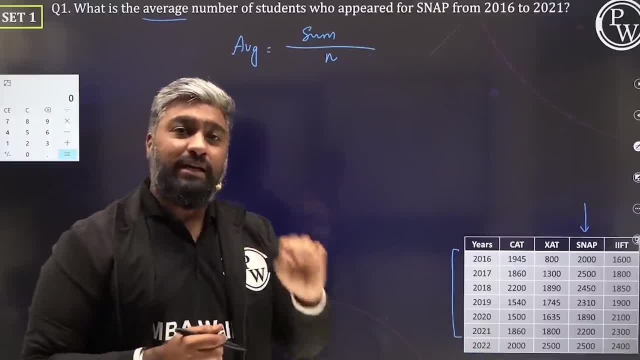 diya hai, but question mein sirf 21 takka pucha hai. A lot of people in a rush. they quickly run through all of it right. fata-fata, poora, sab kuch add kar denge, divide kar denge. phir hume pata chalega ke galti kariye. 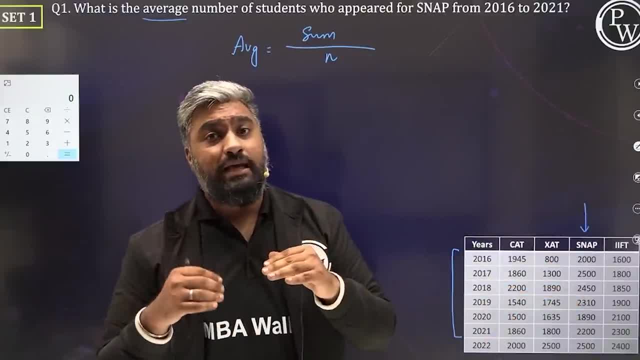 So teta questions Hai. you have to be very careful kyunki aapke paas answer choices nahi hongi to confirm Number two. agar answer choices hai bhi to, they will intentionally put a trap like this. 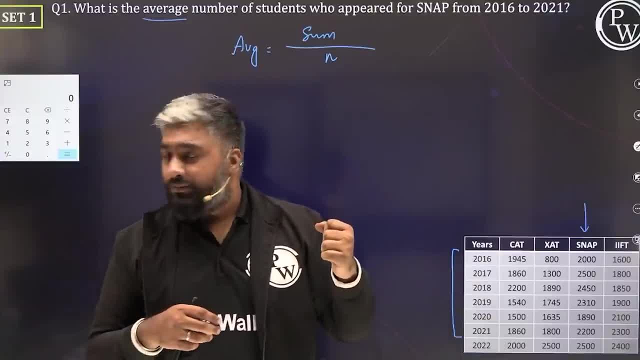 Yes, so you have to be super careful not to lose out on easy marks like this: tige Chalo, let's get started So sum dhundna hai and then divide from for SNAP from 2016 till 21 alone. 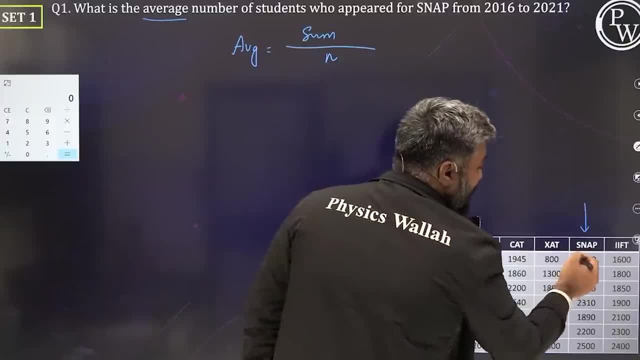 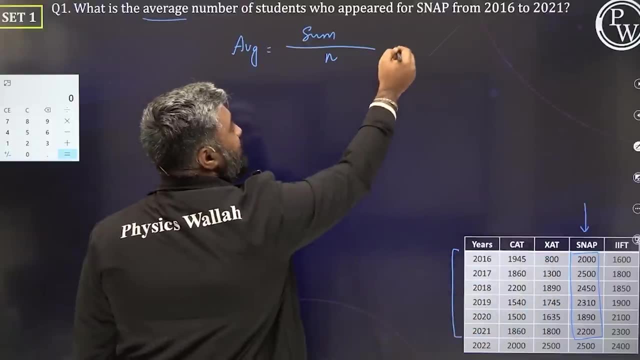 To yeh 2500 ko exclude karna hai. Yes, all. what do we have to do? Basically have to add up all of these values till here and divide by what? How many terms. 16 to 21 is 6 terms. 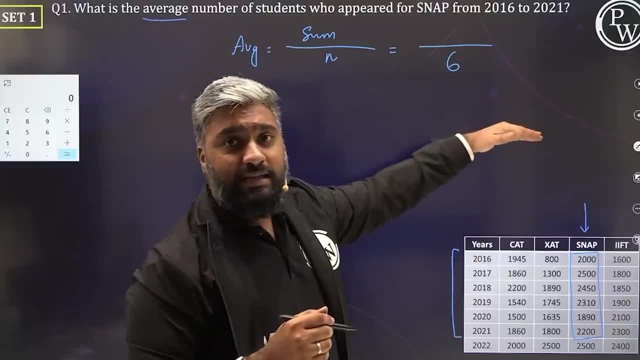 Everything Divided by 6, karna hai. Yes, denominator kaafi dhyan se dekhiye ga, guys, do not miss out on that. tige Calculator ka use karenge, let's not. you know, do a lot of mental calculation and all here. 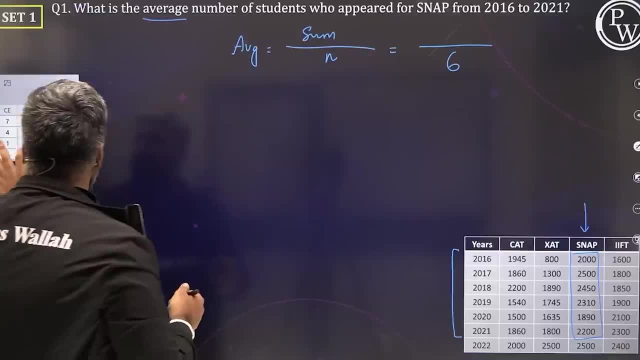 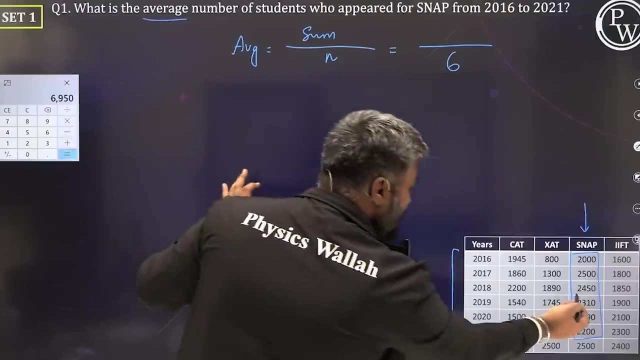 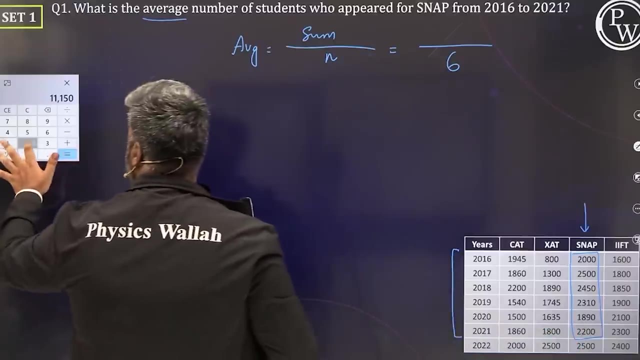 Yes, fata-fata calculator hai. let's get this over with Yes. so what do we have? We have 2000,. so I've added 2000 plus 2500 plus 2450 plus 2310 plus 1890 plus 2200.. 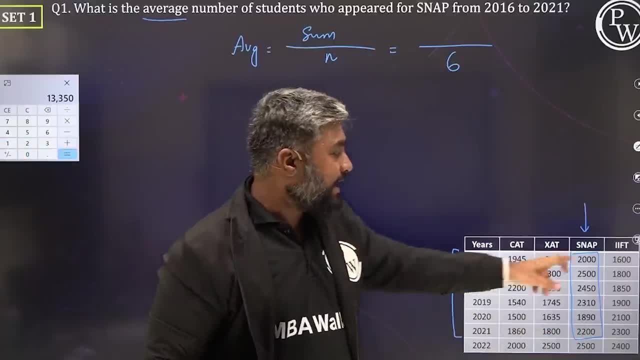 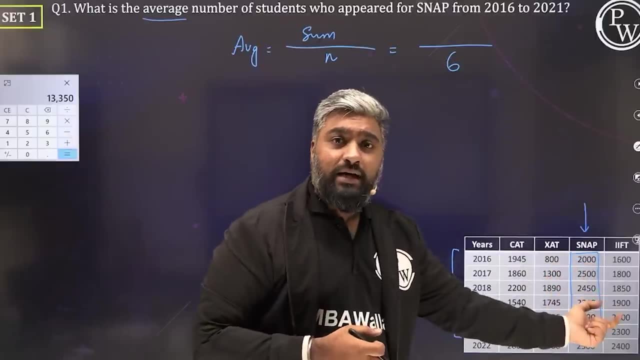 Yes, yaha pe agar aap chaho. If you want, You can also kind of get rid of the last zeros. Yes, ek zero aapne count type karenge Then. but don't forget when you do that, when you make, make the data into scales right. 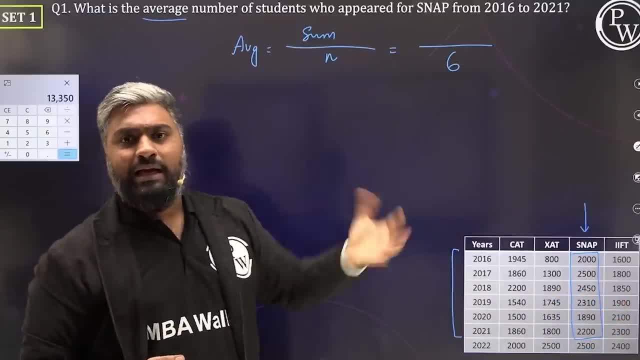 Scale me. agar aap convert kar raha, toh do not forget to include that in the calculation right. Isliye, maine toh risky nahi liya, ek ek zero hi lagana laga diya tige. 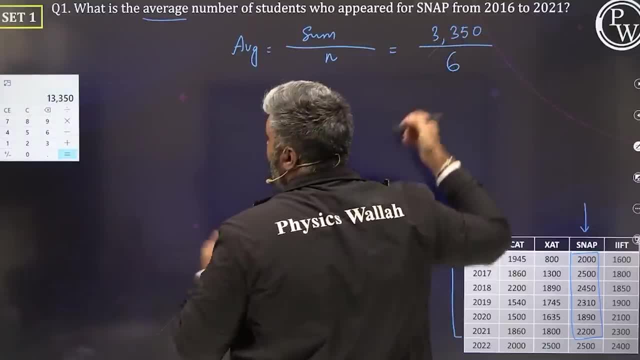 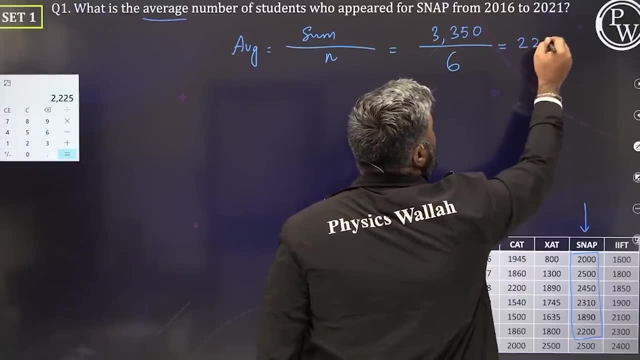 So the sum is 13,350.. I need to divide this by 6.. Again, division vaise toh merko aa jaata. but I'm not going to do all of that. kyunki calculator hai open hai. Let's use it and get rid of it. tige. 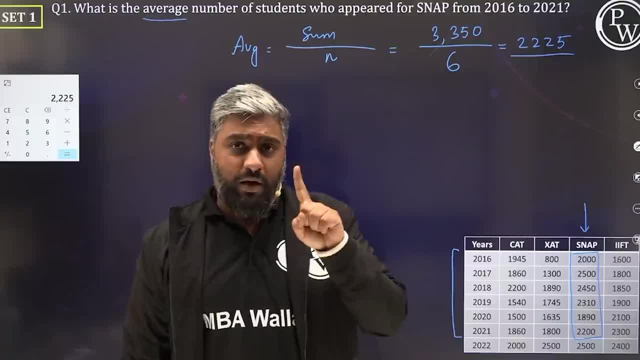 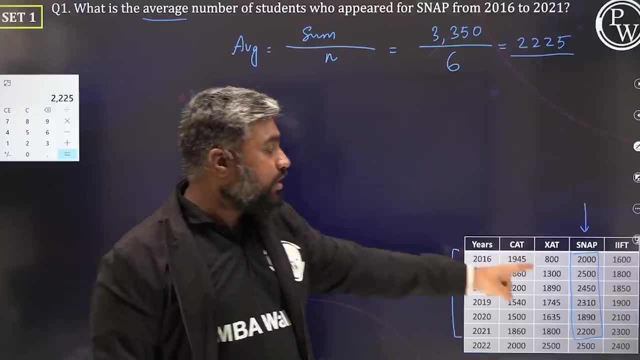 Simple ja question: The average nikalna hai kaafi galtiya hone ki chances hai. Number one: the biggest mistake you can do is with the denominator. Instead of considering seven years, you have to consider six years. Okay, Number two, also with the sum 2500, jo aakhri ka data hai. usse aapko skip karna. 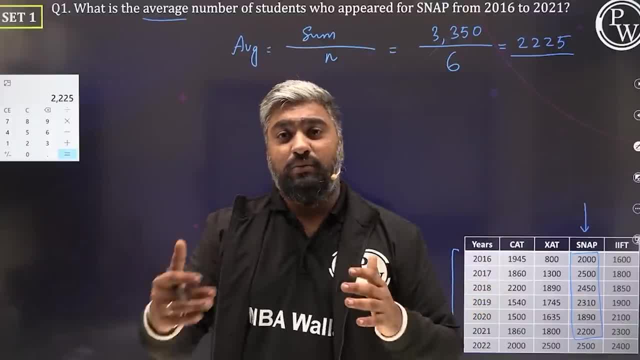 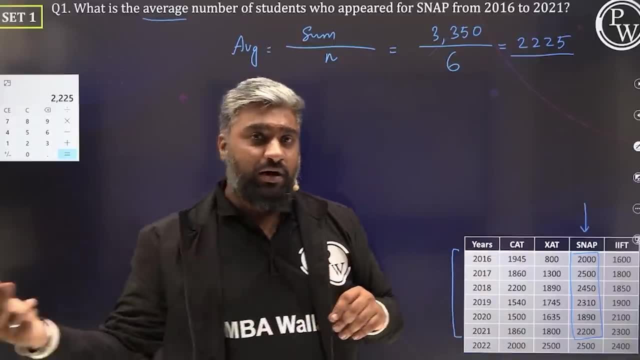 Yes, Number two, the amount of time that you spend on doing the calculation should be reduced as much as you can. Even if you are saving up seconds, aap seconds bhi agar bacha rahe hai, toh vo aap kahin aur invest karke uss question ko aap solve kar sakte. 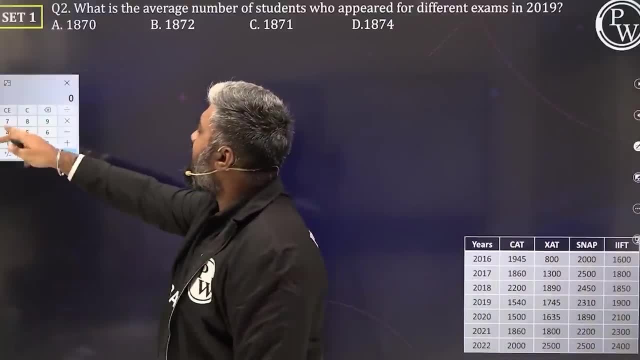 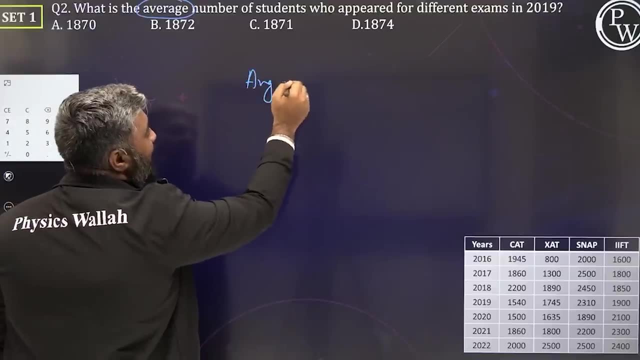 The first question very easy. Let's get on with the second one. Here's our second question: What is the average? Again, this question is dealing with average. Toh, average mein hume kya karna hai? I have to add everything up and divide by the number of terms, right? 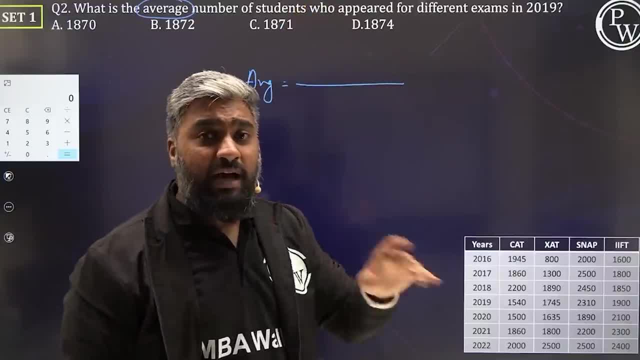 What is the average number of students who appeared for different exams in 2019?? So apki baar hume column nahi dekhna, hume row dekhna hai, Kaunsa row dekhna hai 2019.. 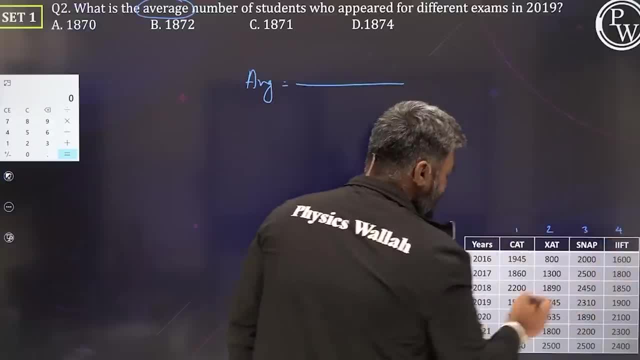 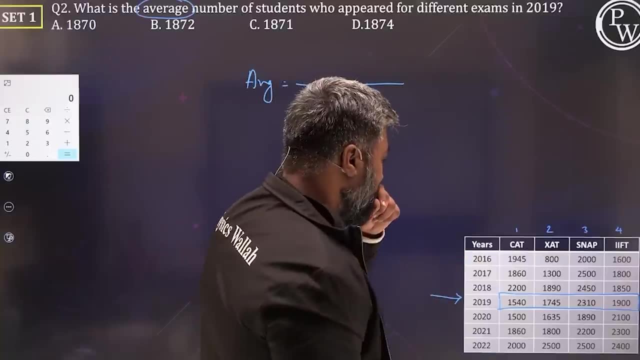 Different exams. that means all the four: One, two, three, four. That means our four cells that we should have a look out for should be these four: Hai na Yeh chaar cells ko hum dekhenge. We'll have a look at these four cells. 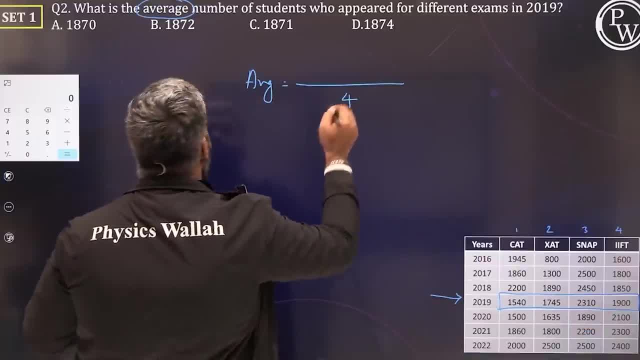 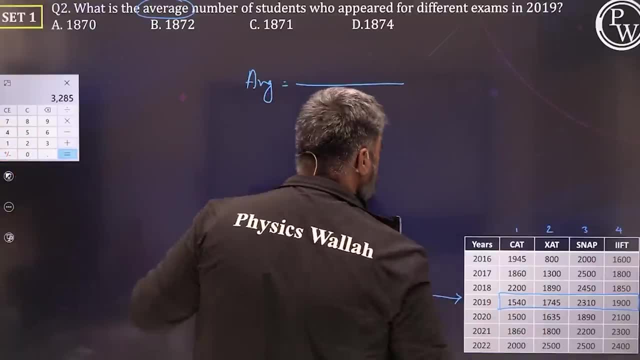 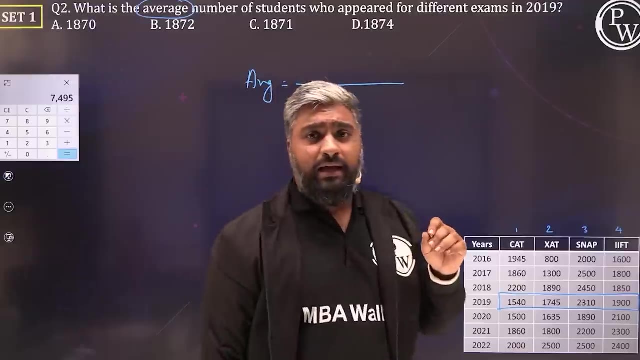 Add them up. divide, Divide by what One, two, three, four terms hai, So four. Let's quickly get started with this: 1540 plus 1745 plus 2310 plus 1900.. Now, guys, one thing you have to be careful about: ki aapke CAT mein jo calculator hoga. 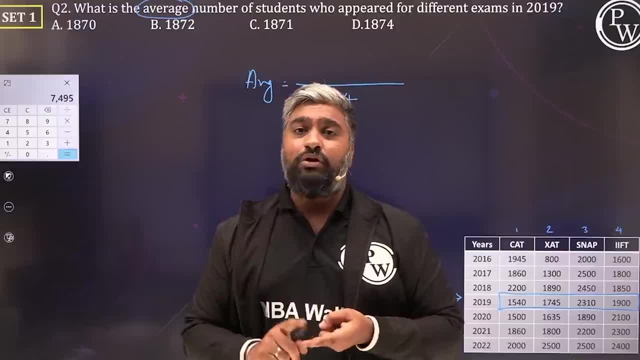 you cannot obviously meri tohra touch karke, toh nahi kar sakte. Number two: aap keyboard bhi nahi use kar sakte. You will have to use the mouse for everything. Navigate karne ke liye, answer, type karne ke liye. type karne ke liye. type karne ke liye. 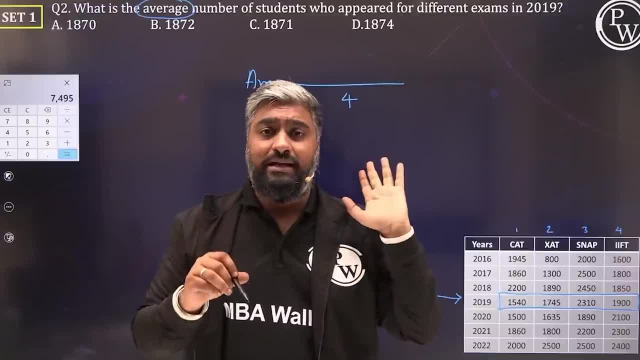 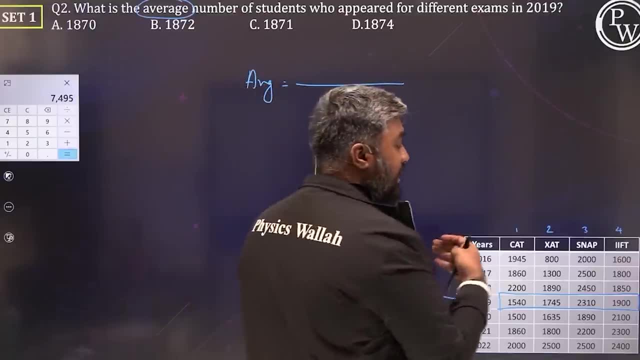 write in the answer. mein aapko jo answer type karna hota hai, Uske liye bhi aapko number pad on screen number pad hoga, Mouse ko rakke aapko click karna hai. So you have to be very careful when you look, jab aap dekh rahe hai, between when you're. 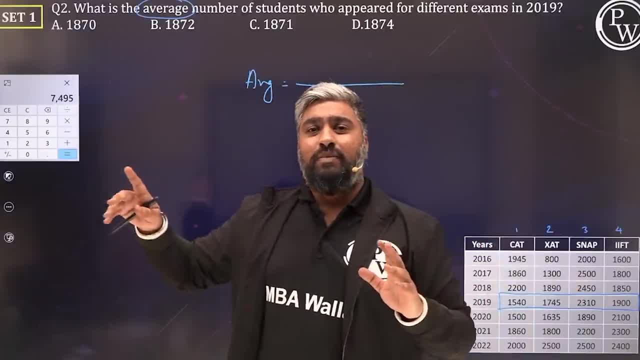 juggling between the table and the calculator. Dhyahan se karna. Do not make mistakes with this. Theek hai bahut silly mistakes hai. Abhi se chalu kar. do Get used to using a mouse instead of a keyboard for calculation. 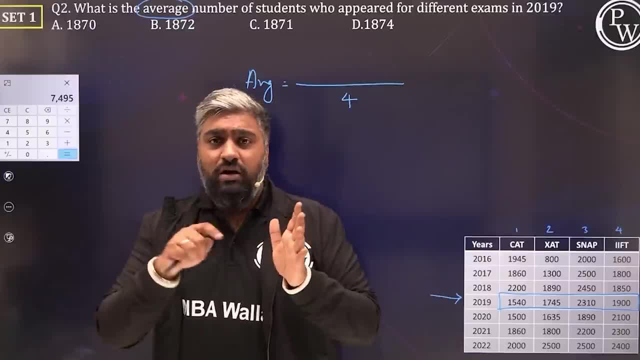 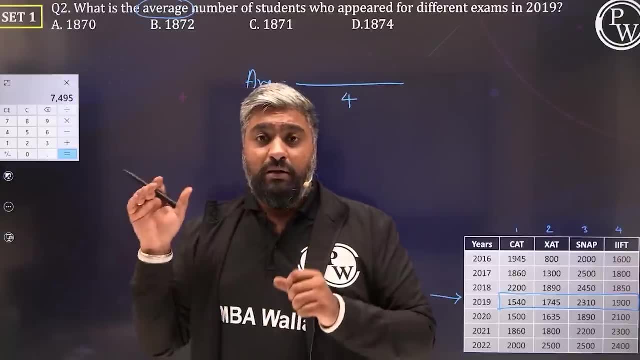 Apne phone pe calculation karna. band kar do. Stop using your physical calculator. also, Casio bagaera ka scientific calculator. Stop using it. Use your computer, laptop hai, PCA, Desktop hai, jo bhi hai, But mouse connect karo aur do everything with the help of the mouse. 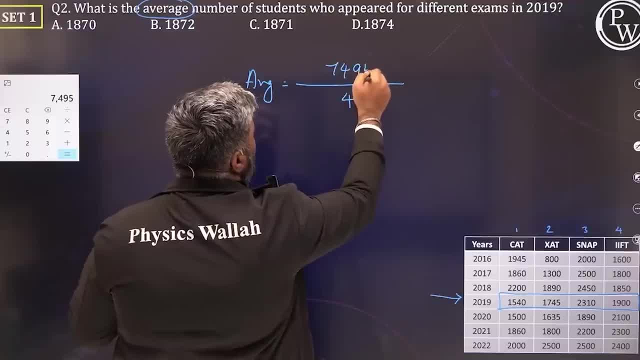 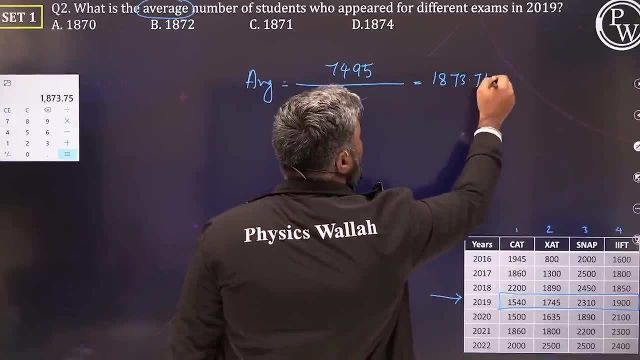 Chalo, So 7495.. We have the sum. Divide this by 4.. We have 1873.75.. Acha, Another thing that you should notice Ki mai kya kar raha ho Sum karne ke baad. I'm writing that data down. 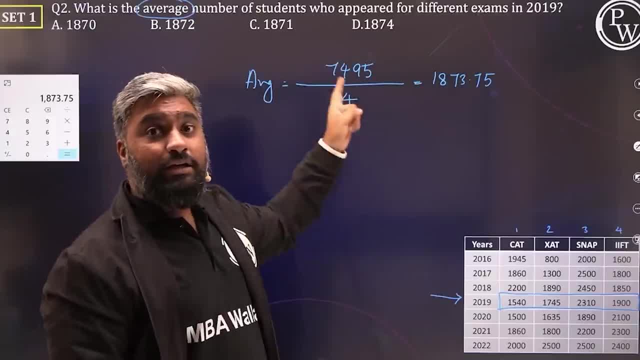 Add karne ke baad jo sum aaya, mai yo likh raha hoon. Why? Because I might use this elsewhere. Ye jo data apne likha la, ye kahin aur use kar sakte hai, number 1.. 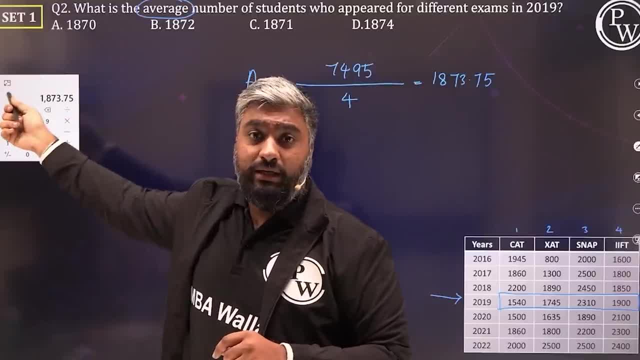 Number 2.. Agar, for example, This is the pending calculation that you have on the calculator. You don't want to mess that with Right Iske saath, wo mix hoke phir kuch alagi answer aega. 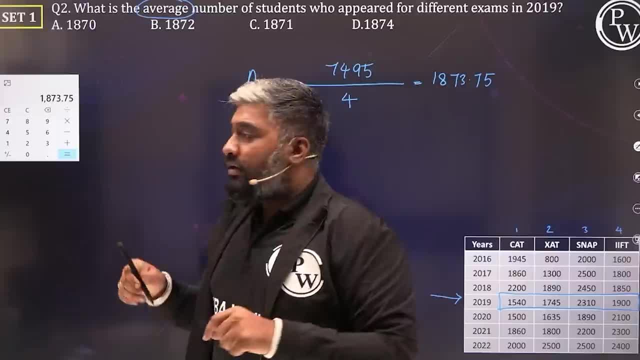 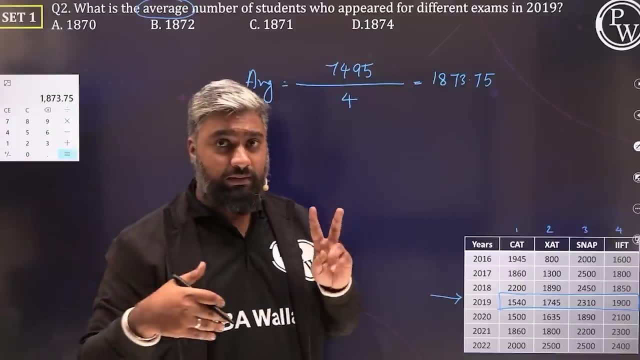 Yeah, So you have to be careful on 2 things: Number 1. Write down any vital piece of information that you get from the calculator. Kyuki calculator, mein history option nahi hai, Toh aap jaake nahi de sakte ke aapne kya calculation ke. 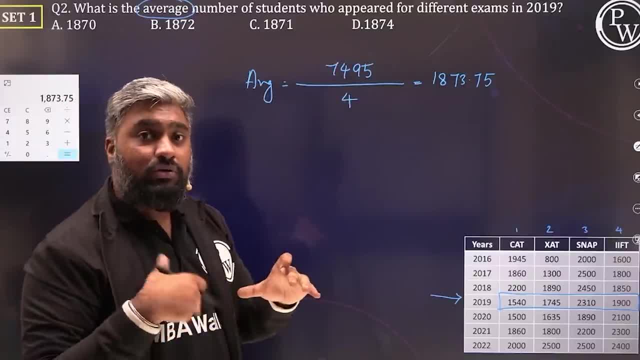 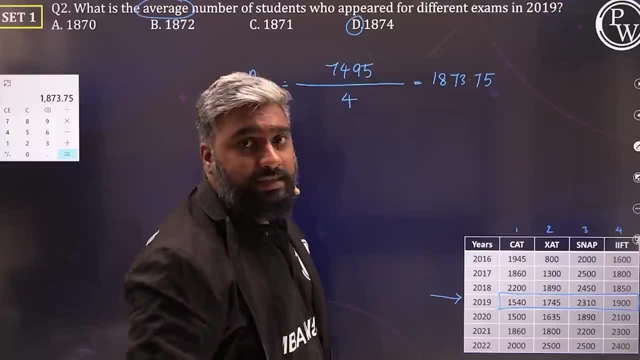 Number 2.. Whatever you are writing is going to be on the paper. for you to revisit The 1873.75,. the closest answer that we have is 1874.. Yes, And that should be our answer. Aapke paas koi aur answer choice hai. 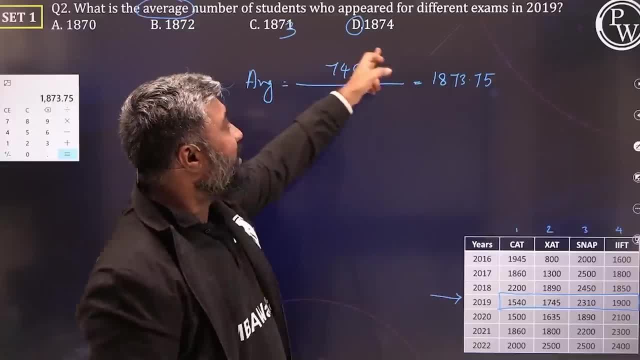 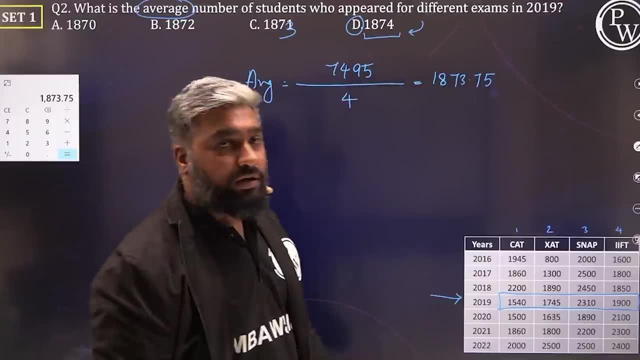 Let's say 1873. hai, That will not be Between 1873 and 1874, 1873.75 is closest to what 1874. Okay, So you have to be super careful about approximation also. Easy question tha. 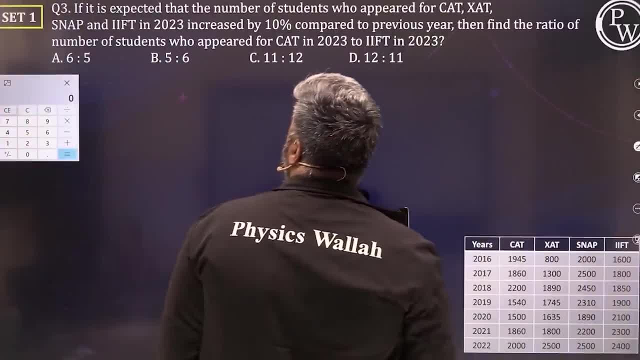 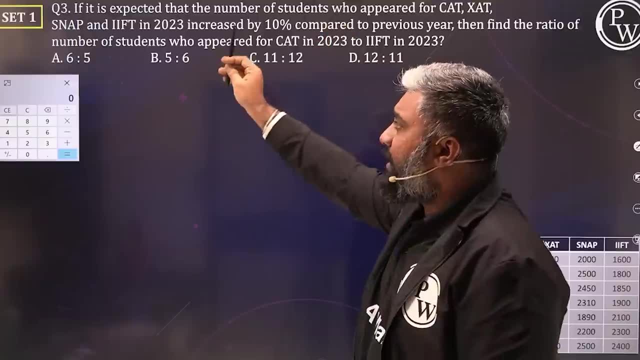 Very good. Moving on to the third question, Calculator ko refresh kar loo. Now this question has some data statement. Thik hai Dhiyaan se parta hai. If it is expected that the number of students who appeared for CAD, ZAD, SNAP and IFT 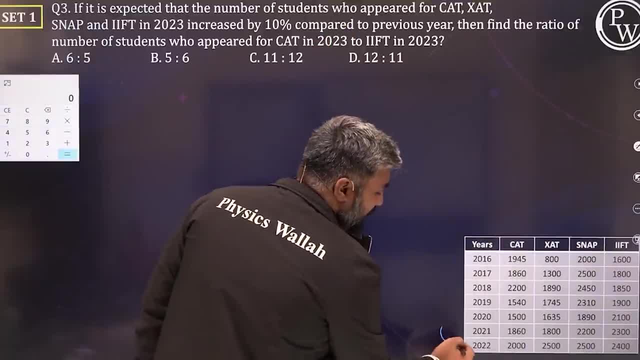 which is all the 4 tests in 2023.. 22 tak ka data hamare paas hai, 22 tak ka data hamare paas hai. 2023 ka bola hai. Kya bol raha hai? That it has increased by 10% compared to the previous year. 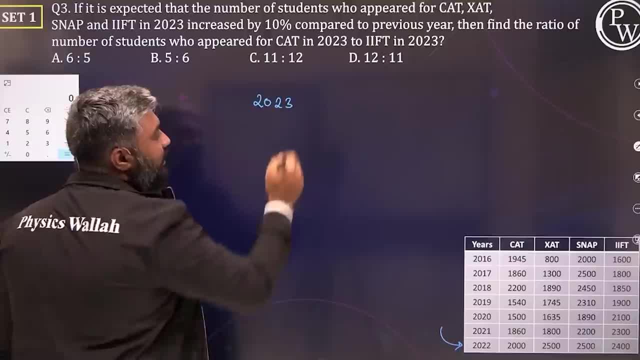 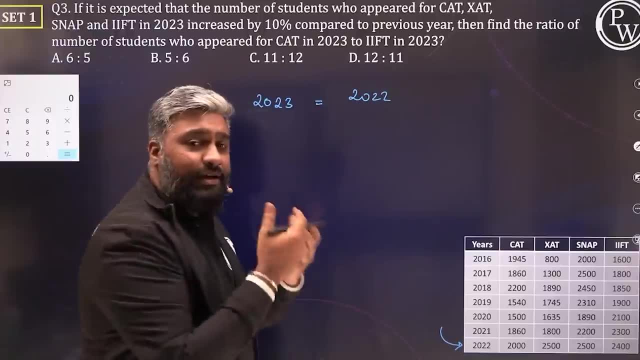 To 2023 ka jo bhi data hoga. Yes, That's going to be what 2022 ke data pe: 10% extra 10% increase means what 100% hai, Uspe 10% aur. 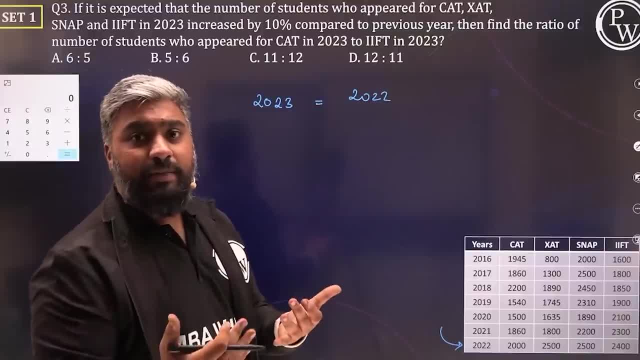 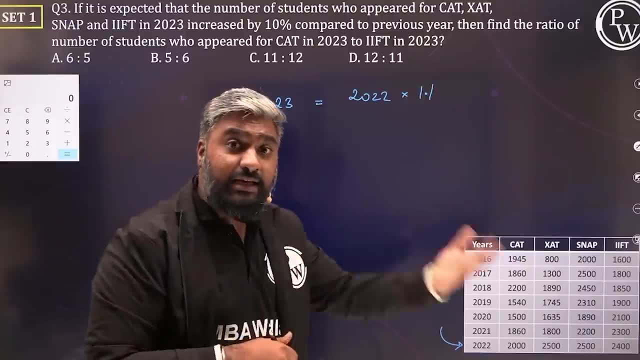 Which is 110% Percentage. wala ke Divide by 100 hai na To 110. divided by 100 is how much 1.1.. So multiplying it with 1.1 will automatically give us the increased value on 10%. 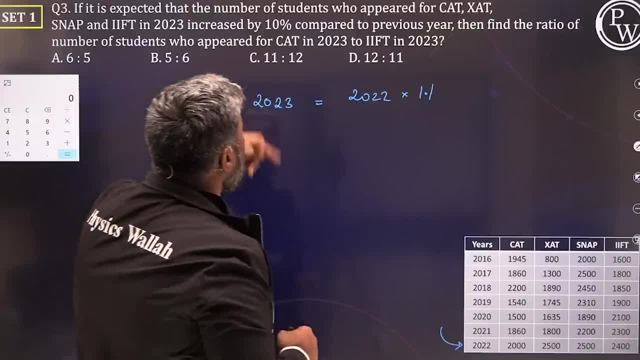 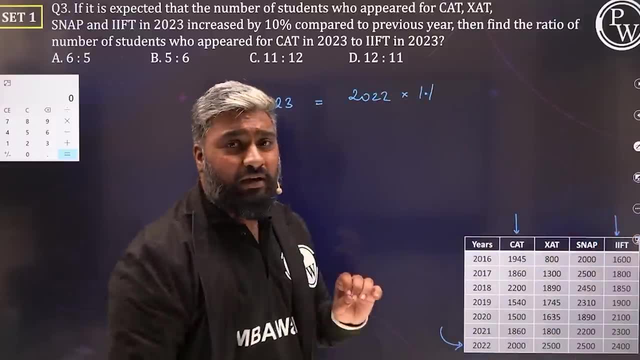 Okay, So this is the data Question. kya hai Find the ratio of the number of students who appeared for CAD in 2023 to IFT in 2023.. Again, be super careful, Do no 2023 ka hi poochaa hai. 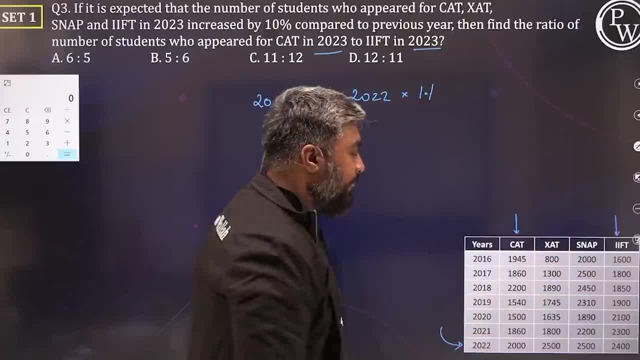 So that's good, And for CAD and IFT only. So ZAD and SNAP pe dekhna nahi hai, Kya karna hai For CAD and for IFT. So iska ratio humein nikalna hai, CAD ka kya hai. 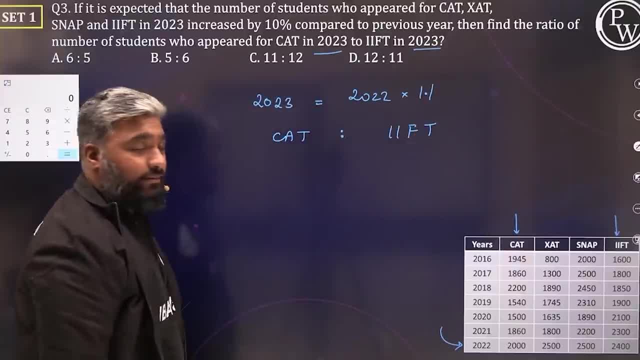 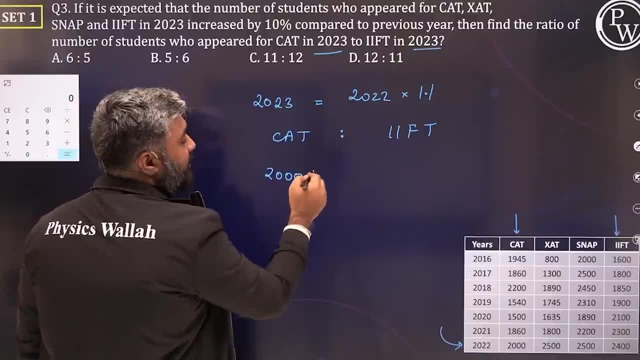 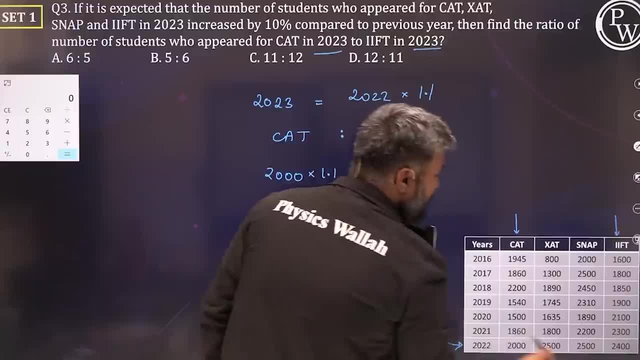 Yes, To what value? IFT is 2400.. Again, 22 ka value hai, 23 ka, kya ho jata hai Into 1.1.. Yes, Ab aapko ratio calculation karna hai. You don't have to find the value 2200, 2640.. 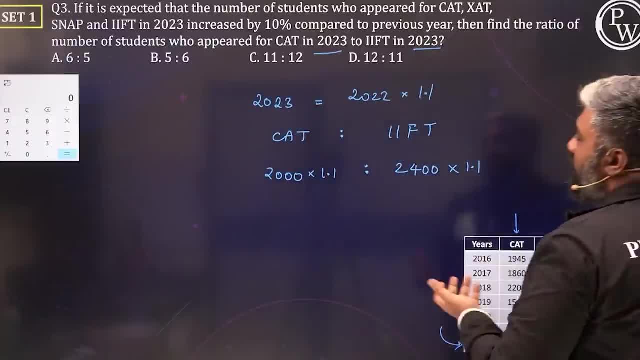 Fir jaa ke aap usse ratio nahi Ratio hai. Start dividing this. Ye dono cancel ho gaye. Two zeros goes off as well, Right, This is 4, 6 times. This is 4, 5 times. 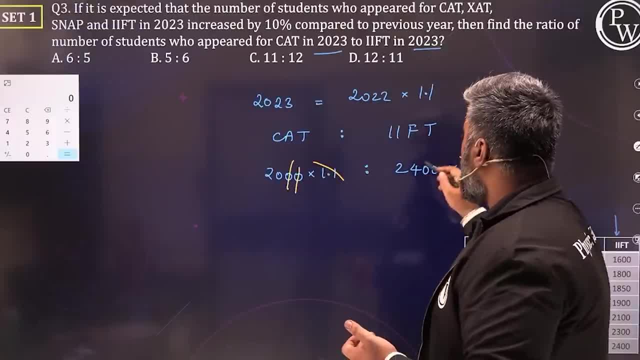 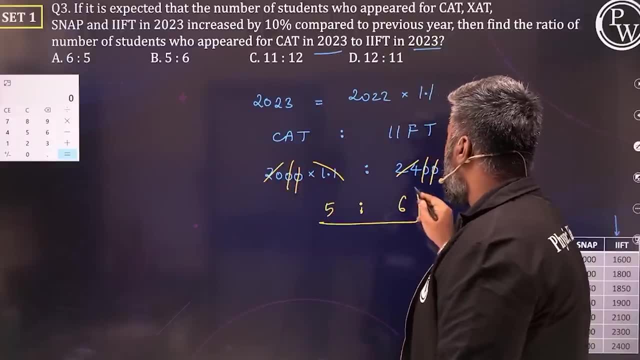 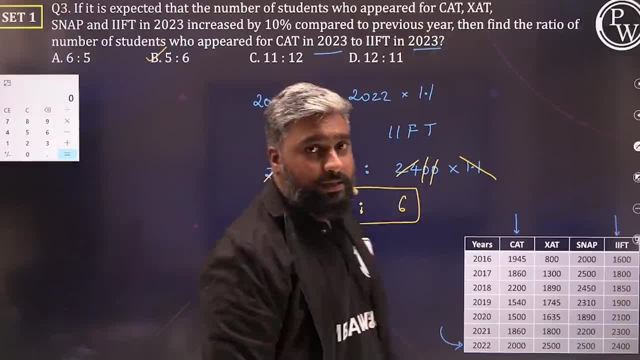 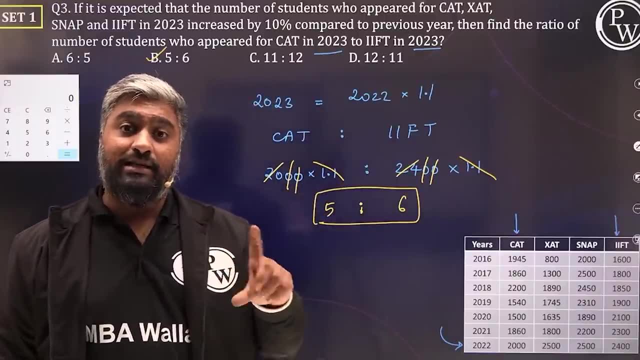 Yes, 5 is to 6 hai answer choice mein. Yes, it is, That's our answer. Again, one thing that you should notice: ke jab bhi ratio based question hota hai, you will always come across one answer choice, jo correct answerka ulta hota. 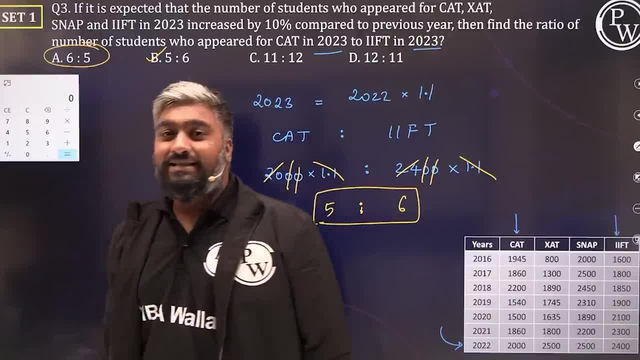 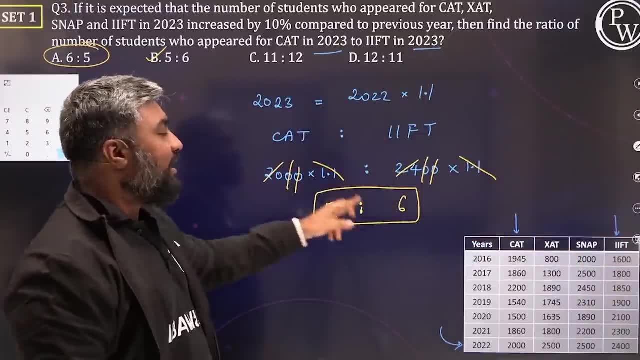 Right Trap set karne ke liye, Like this: 6 is to 5.. Ye galti kab hogi Jab hum, instead of taking cat is to IFT, we take IFT is to cat, IFT is to cat ka ratio ka ho jata 6 is to 5.. 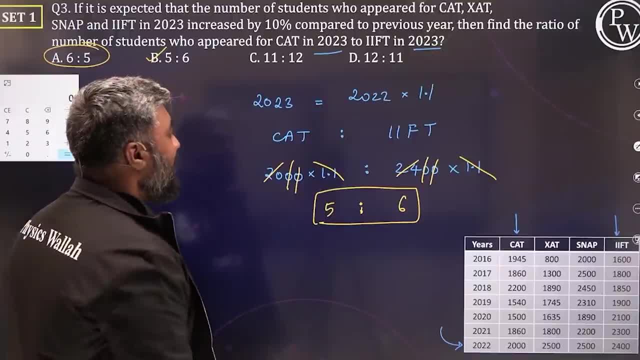 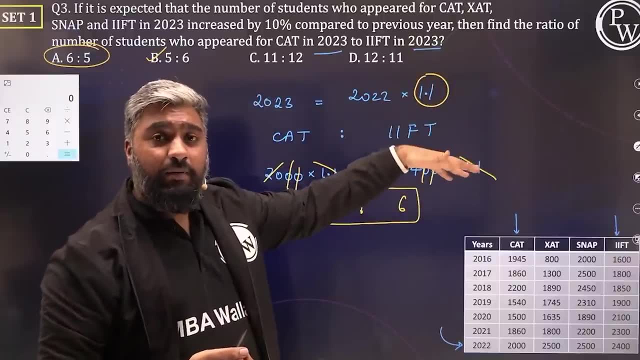 Yes. So you have to be supercareful about that Tink hai. So in this decrease, you understood why we multiplied it with 1.1, it is called multiplicative factor. You will read in detail in percentages, but I will tell you from top to bottom. 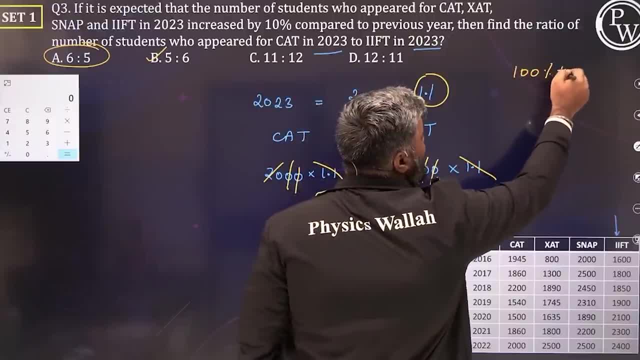 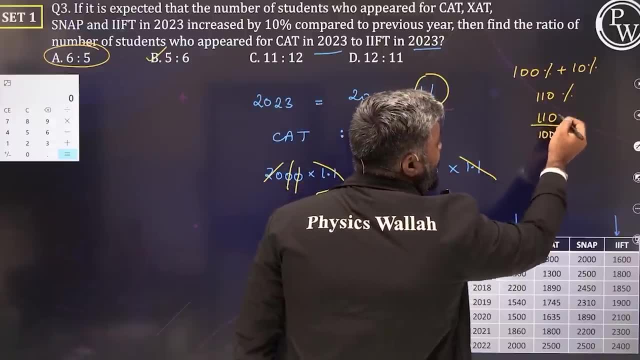 On 10% increase means 100% was earlier. if 10% increase on this, then how much is it? 110%, Yes, what does percentage mean By 100.. So 110 by 100 is what? 11 by 10,, which is 1.1.. 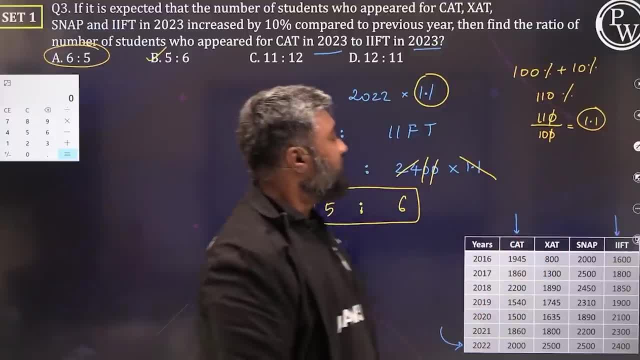 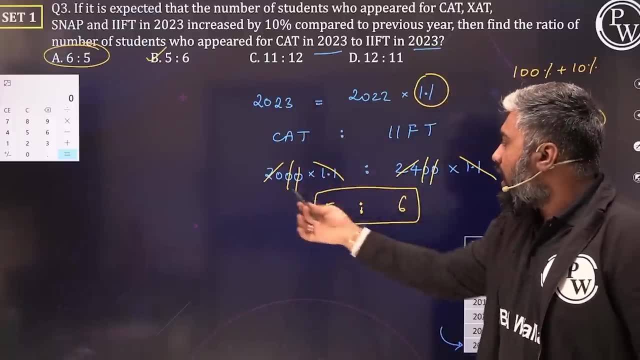 That's why we multiply it with 1.1.. Got it Beautiful. This is a very interesting question, very good question. So, whenever you come to the ratio right, instead of doing intrinsic small calculations, keep it out front. something or the other will be cancelled and you will get the final answer. 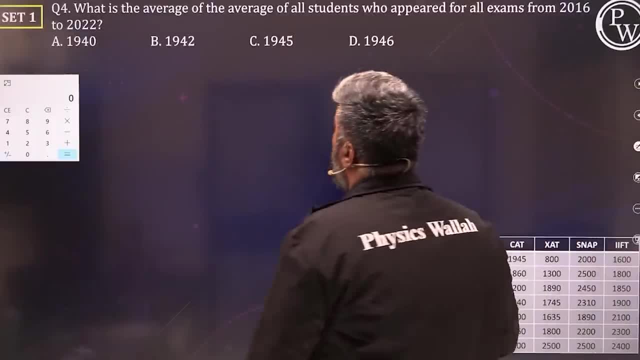 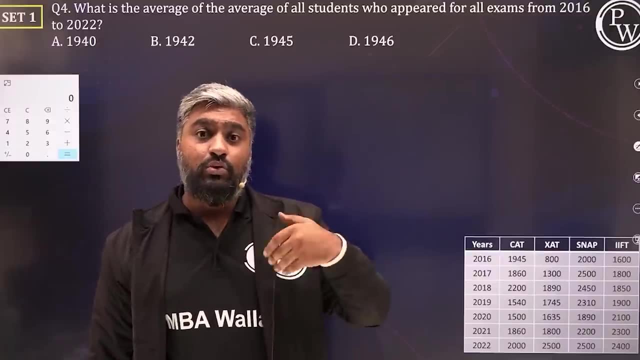 Okay, let's move on. Question number 4.. What is the average? Now look carefully at the question here. Sometimes what happens is, whenever we see repetitive words, our brain tells us to omit that. If 2-3 things are repetitive, then our brain tells us to leave it because there is repetition. 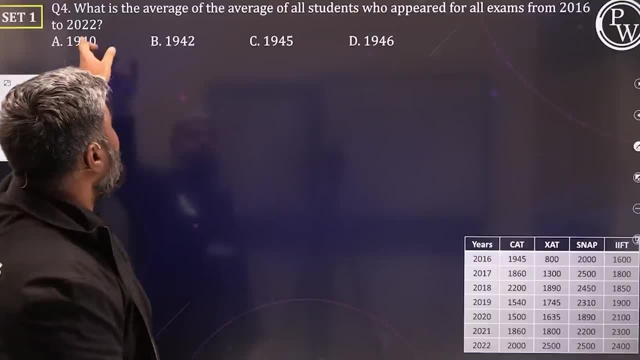 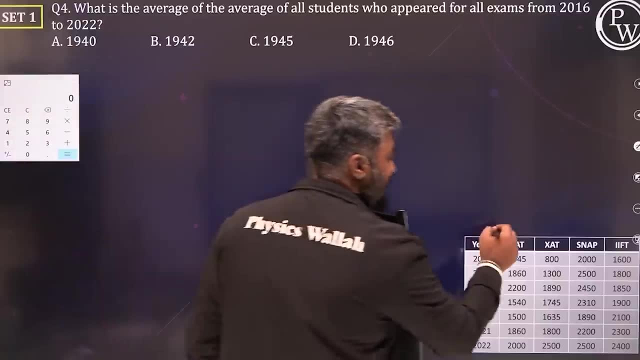 less efficient way of reading. right, but you have to be very careful here. What is the average? What is the average of the average of all students who appeared for all exams from 2016 to 22?? You want to see all the exams? Yes, 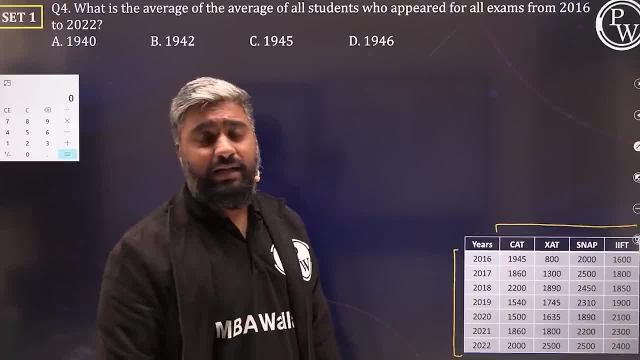 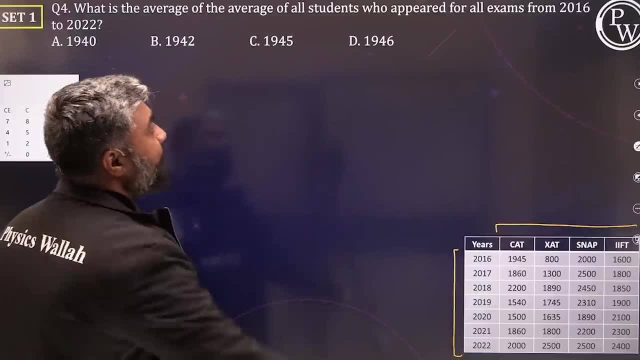 16 to 22,. full table. you want to see full 28 pieces of data? Yes, But what to do? Add everything and divide by 28.. Average of the average, right? So what are you to do? All exams? So first of all, let's look at CAT. okay? 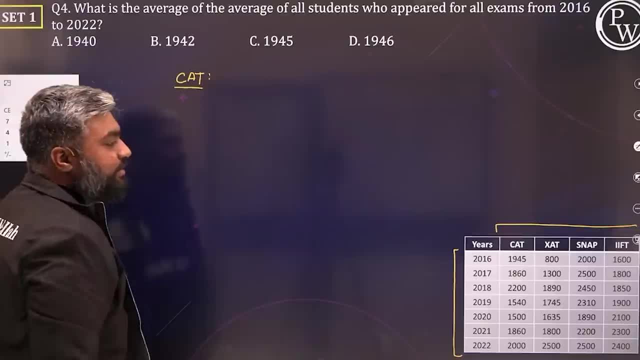 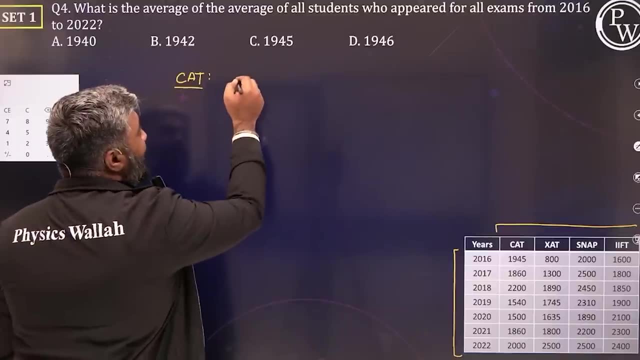 I'll give you. let's solve this. If we solve this, you will understand the question too. So what do we need for CAT? We need the average of the number of students who have appeared, from 16 to 22.. So what will be the average of CAT? 16 to 22 is 7 years. 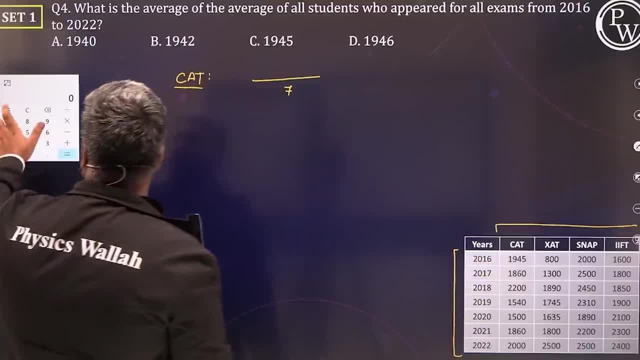 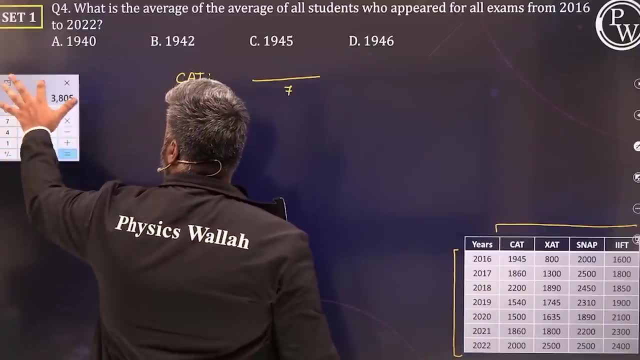 So 7 in the denominator, What will be the sum of all these in the numerator? Yes, So let's quickly do that. We have 1945 plus 1860.. Let's bring the calculator a little closer, It will be easy, Okay. 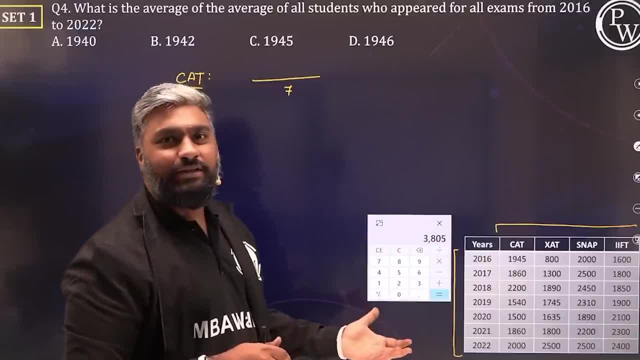 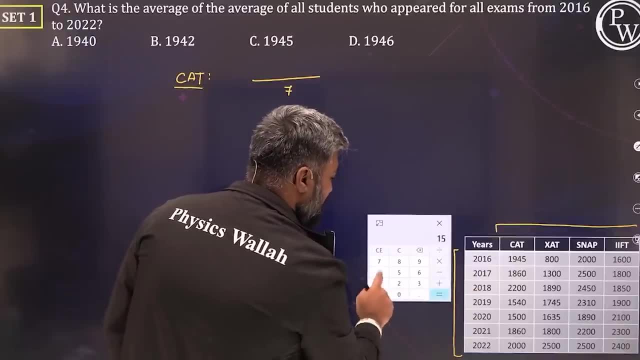 I'm doing this for you. You do this in the test. Actually, you can move around your calculator also. That's good. So 1945, 1860 plus 2200.. Plus 1540 plus 1500, plus 1860 plus 2000.. 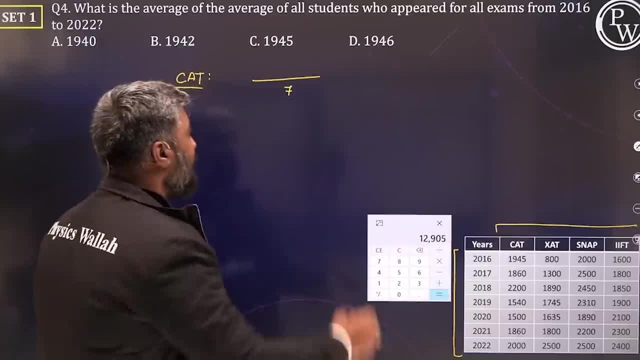 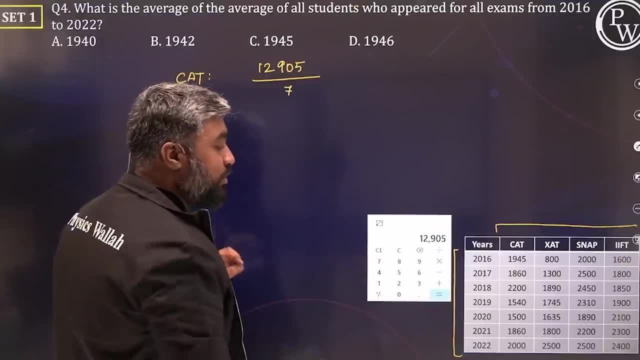 Yes, Here is our total: 12905.. 12905.. Now, one thing you have to keep in mind: You have done the sum right. Please don't make this habit that the moment you add 2000.. What do we do in the calculator? We do 2000.. 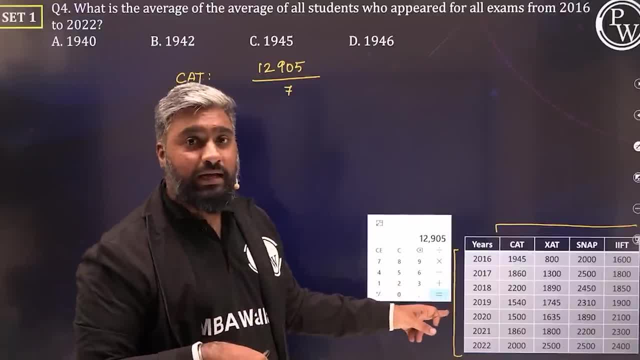 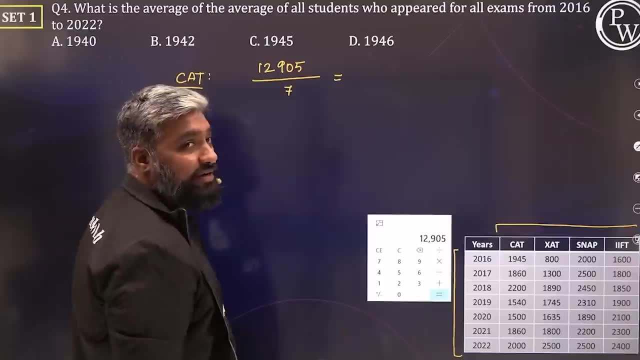 Immediately. you don't have to divide by 7.. You have to hit on the equal to sign Because you don't have to do 2000 by 7.. You have to do 12905 by 7.. According to the board mass if you directly divide by 7,. 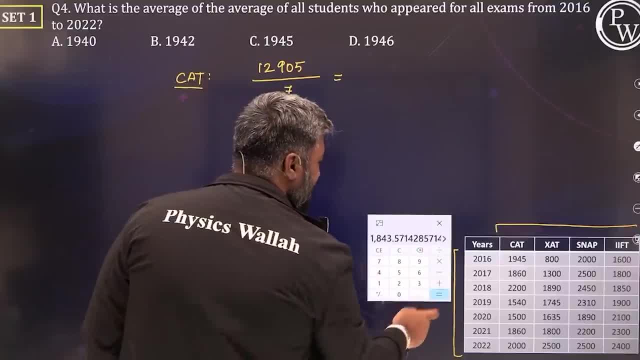 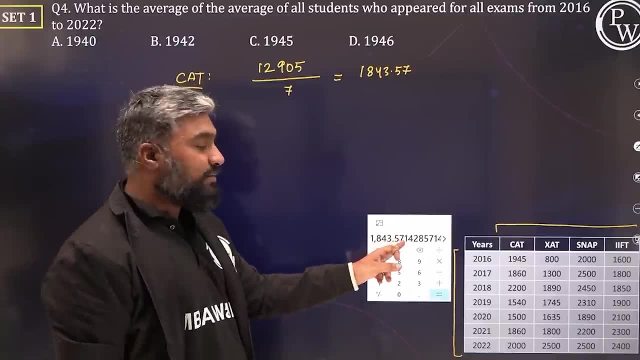 then it will be 2000 by 7.. Please be careful about that. Divided by 7, we get 1843.57.. 1843.57. Did you understand? 1843.57 is what Is the average of all cat takers from 16 to 22.. 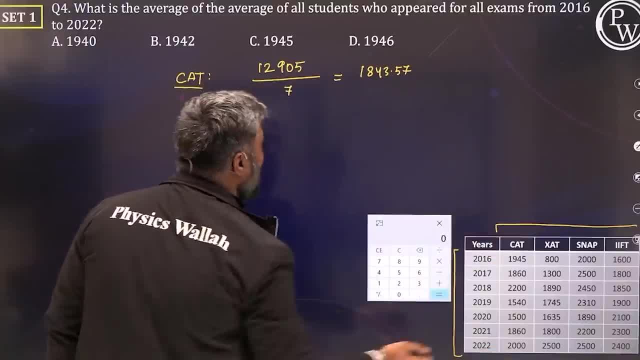 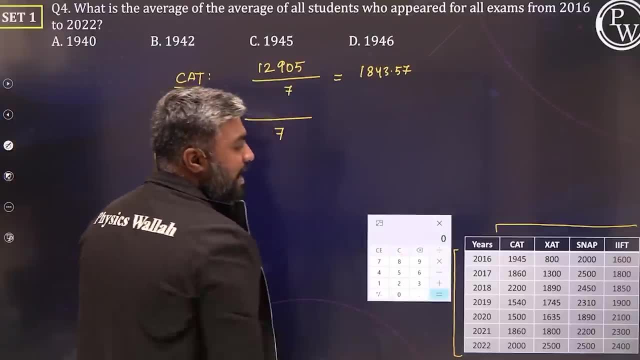 Okay, The same thing you have to do. You have to do the same thing for ZAD, snap and IFT as well. I will do it with you. You guys also take command, Start adding up the values. Right, You can do it manually. 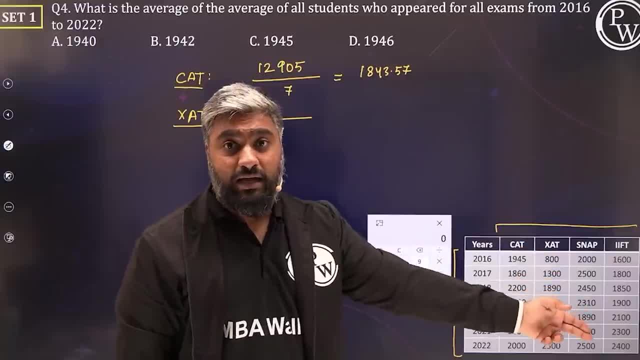 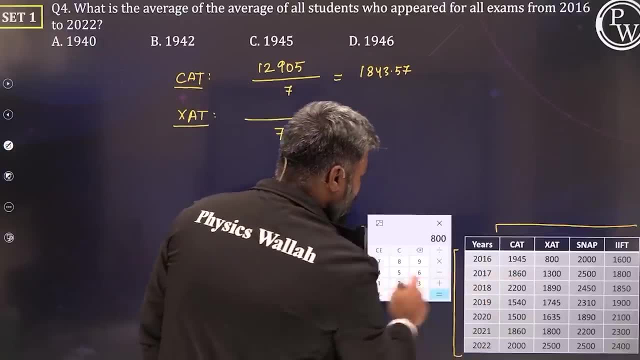 No harm there, But because there are 28 pieces of data, Right, It could be one small mistake and it could blow up, Right? So please be super careful. What is next? Let's do ZAD 800.. Plus 1300. 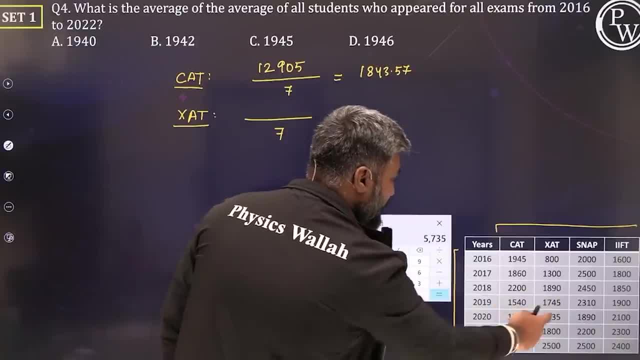 Plus 1890.. 1745.. 1635.. 1800. Plus 2500.. Which is 11670.. 11670.. Now you have two choices. One, You have to divide by 7, by 7.. 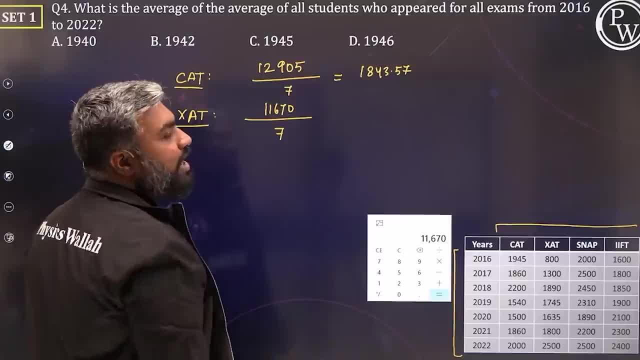 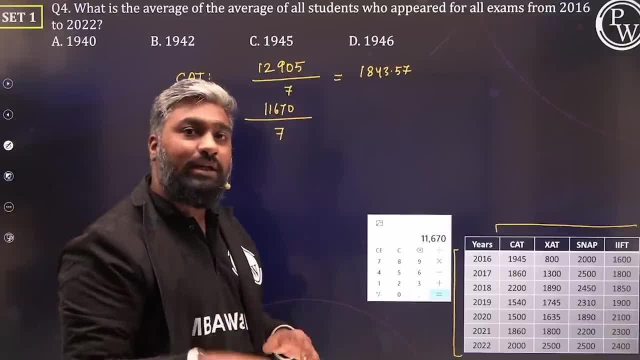 Or you can add the total And then divide the whole thing by 7 at once. Either way the sum will remain the same, But anyway We are doing it individually, So let's go with that flow Divided by 7.. 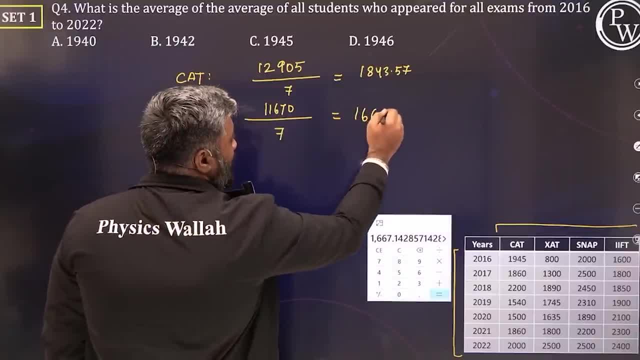 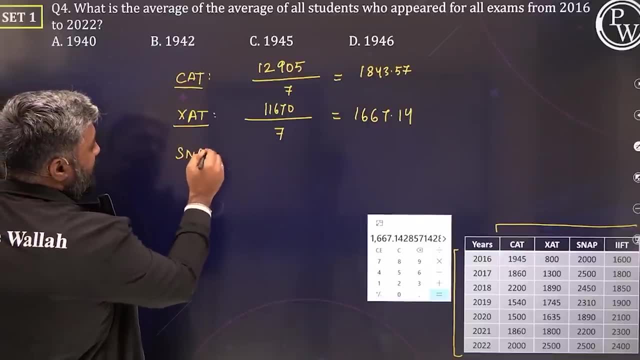 We get 1667.. Point 1428.. So I will take as 14.. Right, That is done. Next, Moving on to snap, Let's do the same thing, Whatever we get divided by 7.. Let's add this up for snap. 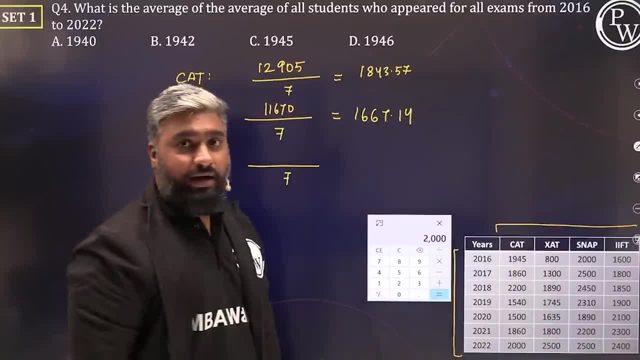 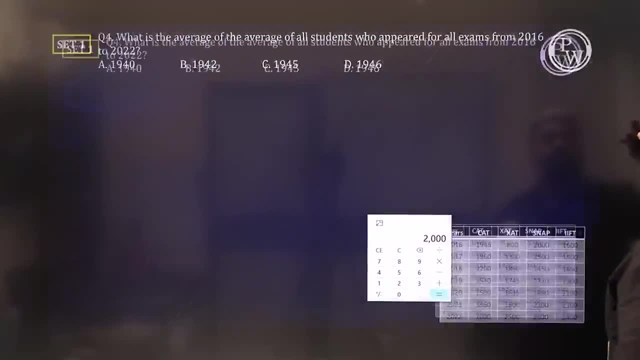 2000.. You must remember. So we did snap already, Right, So here you can save some time Because you have already done snap. Do you remember Till 2200.. Where did we do it In the first question? 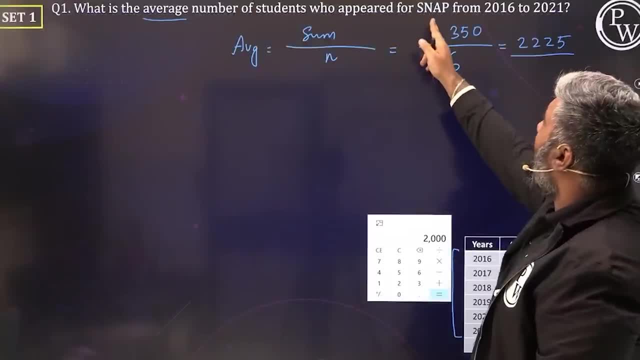 See this In the first question. we have already done snap, But only till 2021.. What did we get? the sum as 3350.. Are you getting this guys One second A break? It was on 12 minutes. 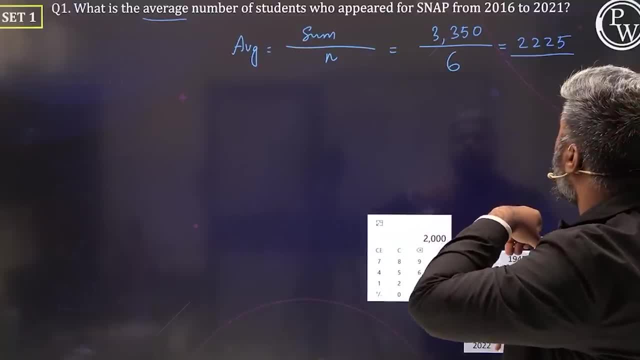 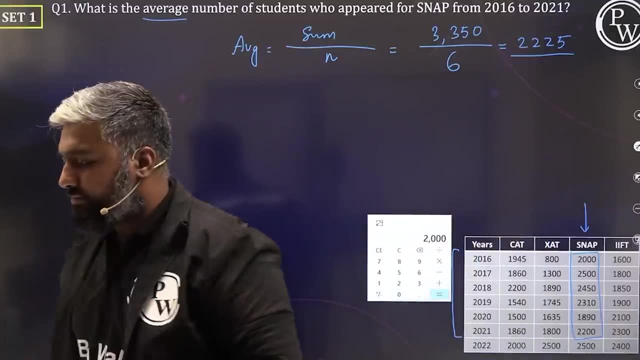 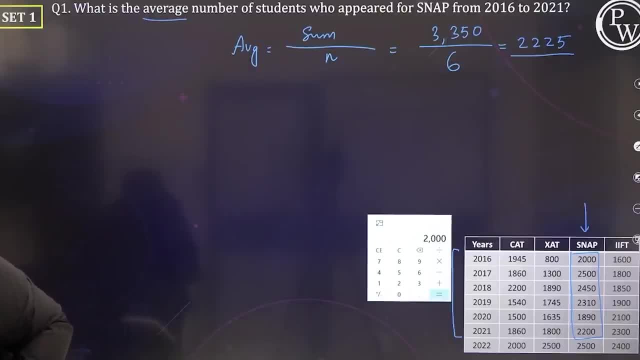 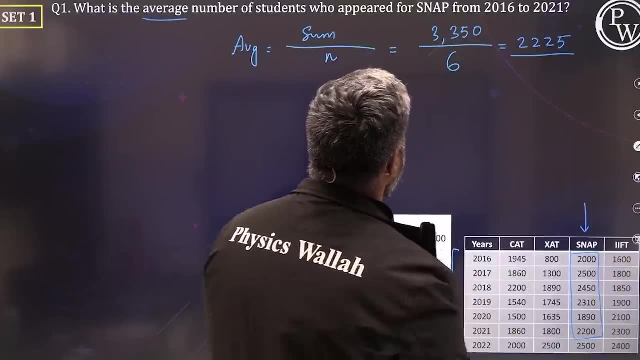 So we did snap. So we did snap, So we did snap: 0. 0.. 0. 0. 0.. What is it? Sum of 3350.. Wasn't it 1?? Okay, A little bit. 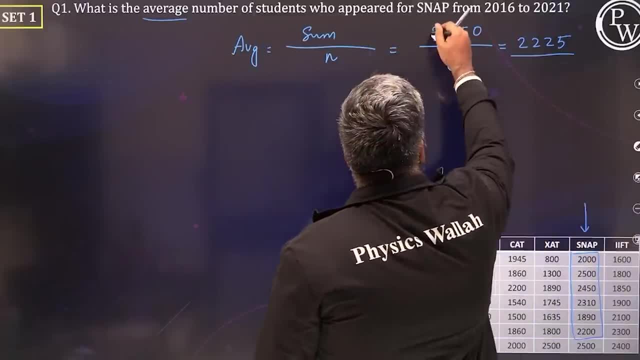 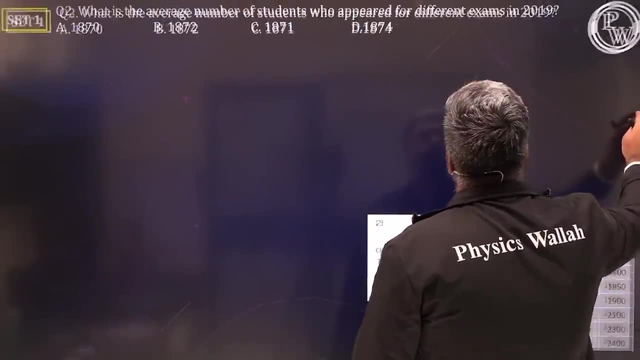 I will write it: 1. 1., 10 minutes Or something. Let's see: 1. 1., 2., 1., 2., 1., 1., 2., 1. 2.. 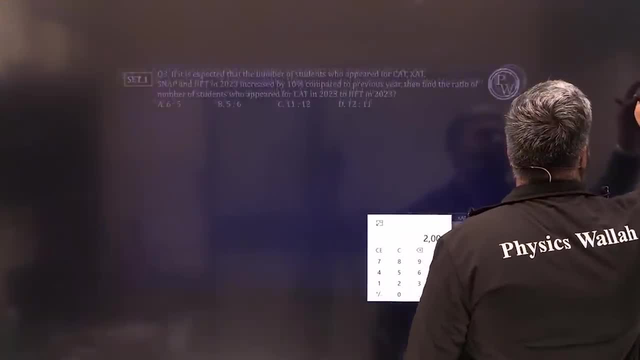 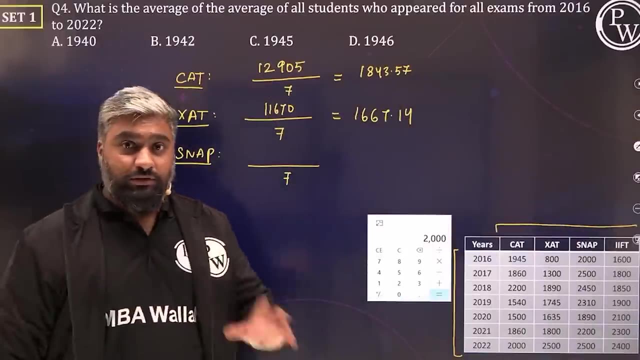 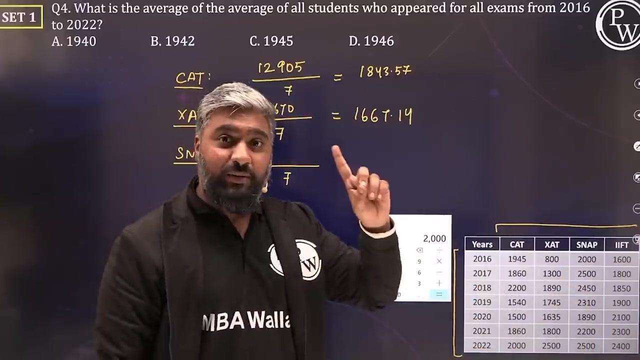 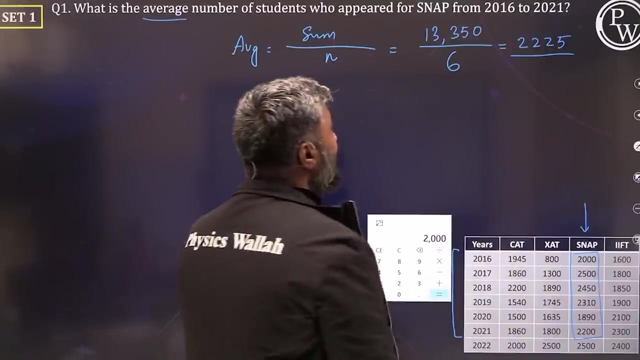 1. now snap. you must have seen that we have already done from 2000 to 2016 to 21, right? do you remember in the first question? now here we can save some time on the addition part if you could quickly scroll back and see what was the sum that you used for snap from 16. 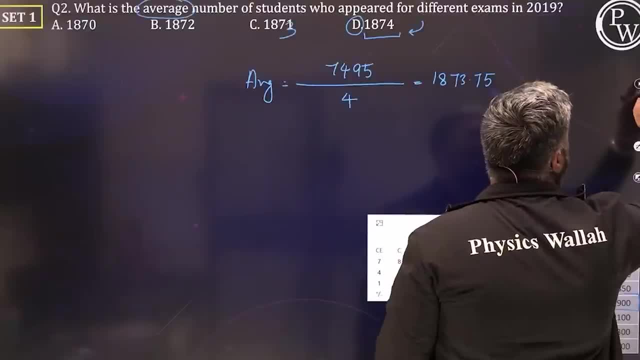 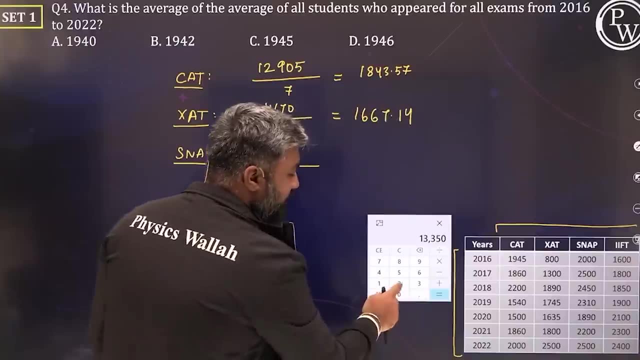 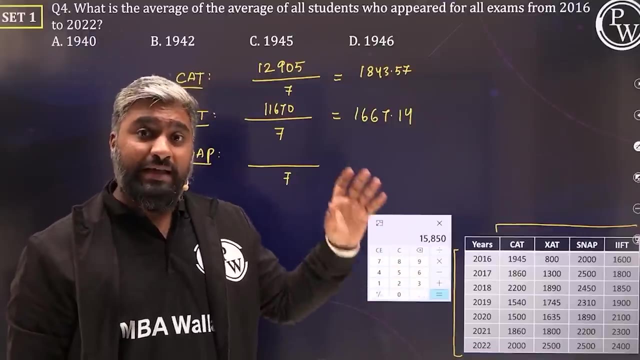 to 21, which is 13 350. right, this is already 13 350. yes, 13 350 is already there. till 2021. you have to add 22, which is 2500. what has happened with this? you have saved maybe just 10-15 seconds. that is okay. this 10-15 seconds for 2-3 questions together will end up being: 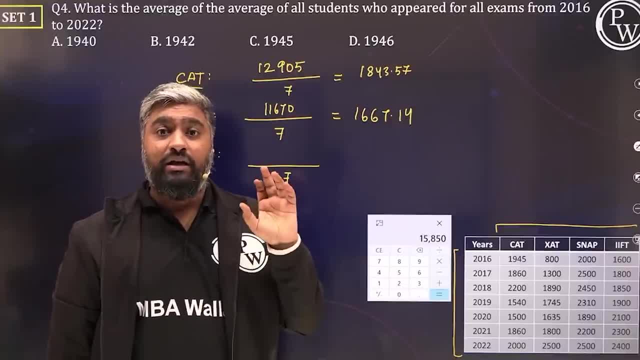 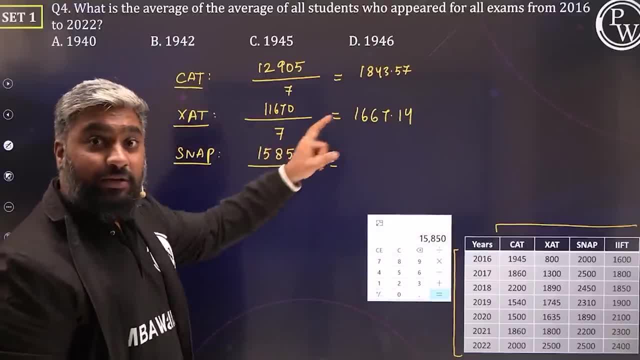 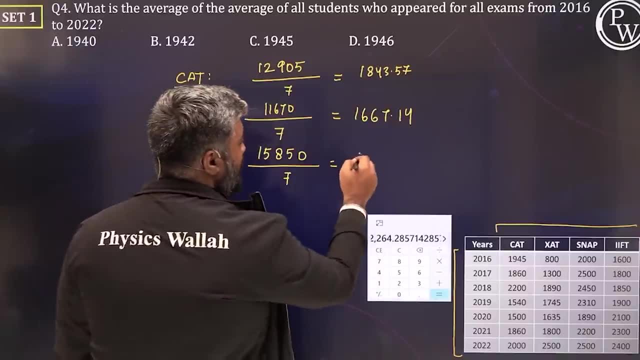 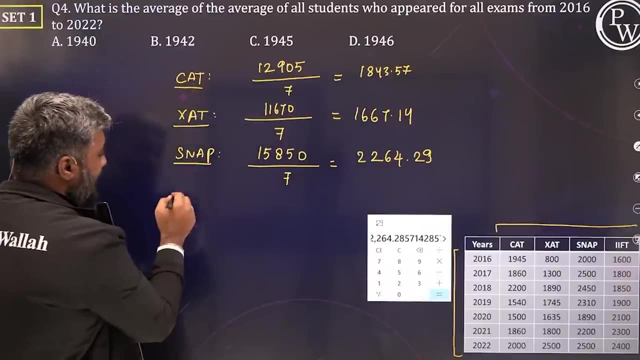 why I am writing down these values, the reason why I'm writing down these values, ke baad mein jaake kaam aayenge, jaise yahaan pe kaam aaya hai na. let's divide this with 7, we have double 2, 6, 4, point 2, 8, 5 hai toh main point 2, 9 likh raha hu for the approximation and towards the end, IIFT baj gaya. 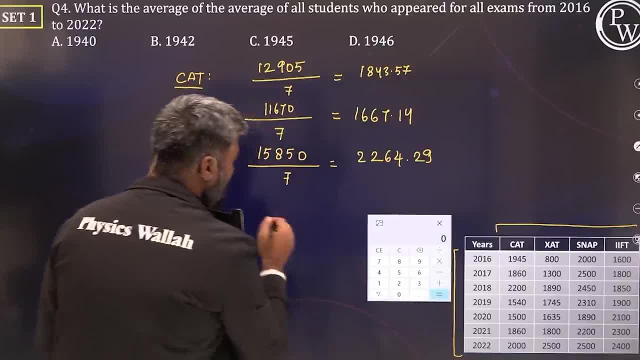 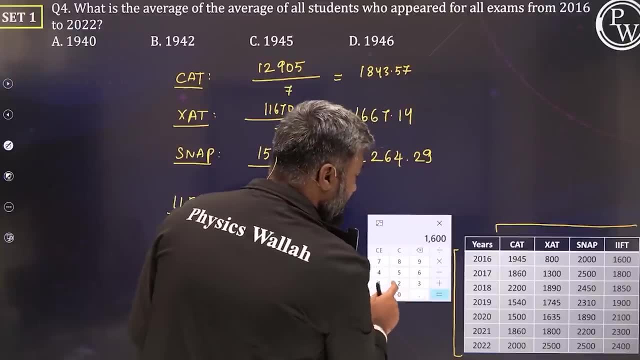 let's get IFT also over with same thing karna hai, add karna hai by 7. let's go for IFT 1600 plus 1800 plus 1850 plus 1900 plus 2100 plus 2300 plus 2400. so yahaan pe bhi hum, by scaling down these. 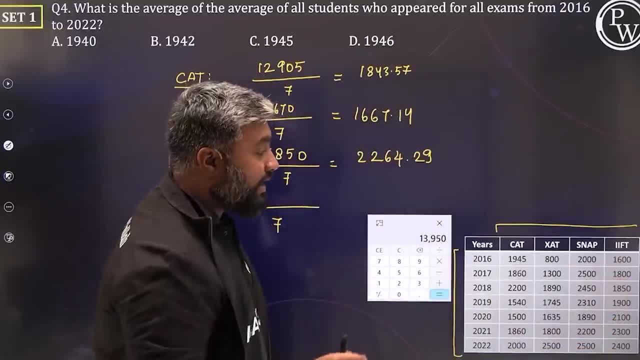 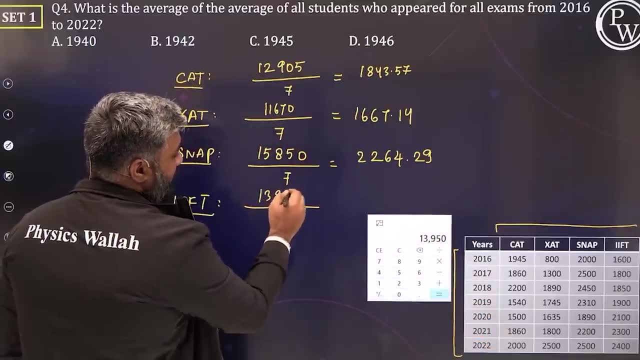 two zeros. we could have saved some time, right. but phir dhyan mein aapko yeh rakhna hai ke if you are scaling them down, you have to use them later. theek hai wo bhulna mat anyway: 13 950 hai 13 950 divided. 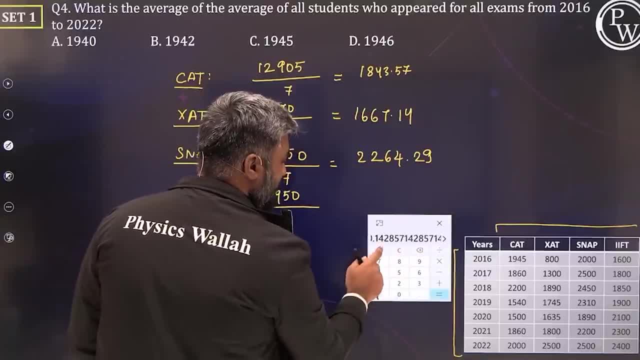 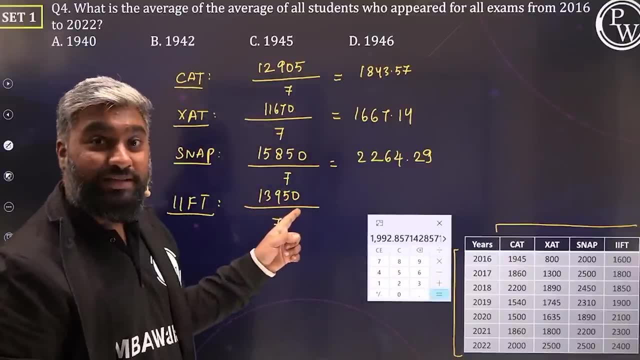 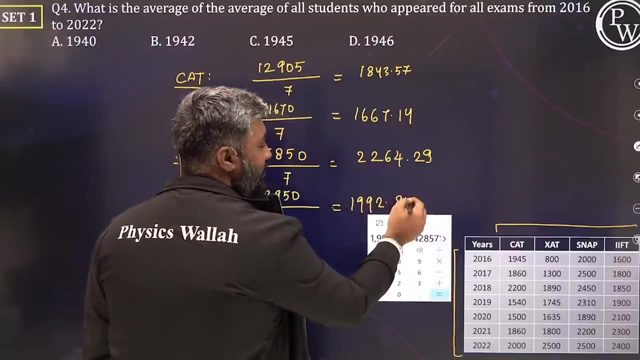 13 950 divided by 7. see 13 950 divided by 7. that's why I write down these values, so that we don't miss them out. yes, which is 1992, 1992, point 8, 5. yes, yeh 8, 6, karlo kyunki, 8 by 7 hai toh 8, 6, 2, 2 decimal toh theek hai, yeh bhi. 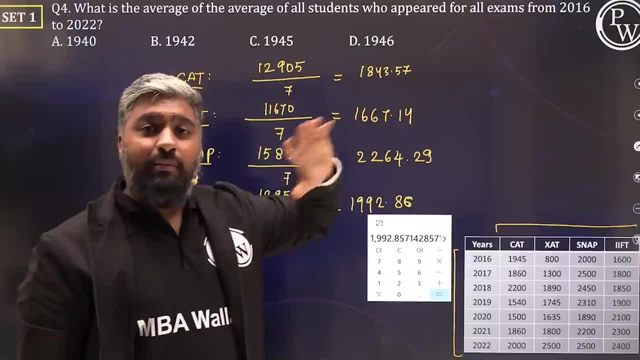 zaruri nahi hai vyaise, kyunki answer choices hume diye hua hai in integer values. but one thing you have to be careful: ke values kaafi close hai, 1945, 1946 kaafi close hai. isliye maine 2, 2 decimal liye. agar yeh dur hota hai, let's say, this was 1930. 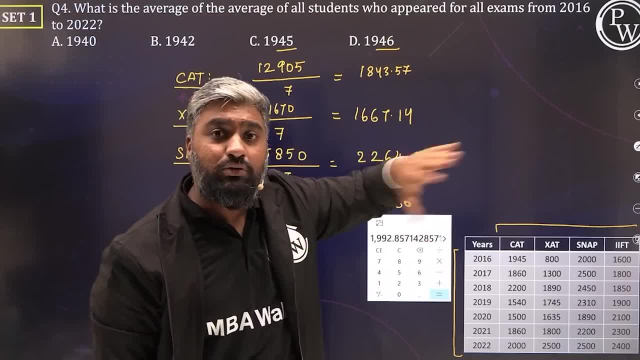 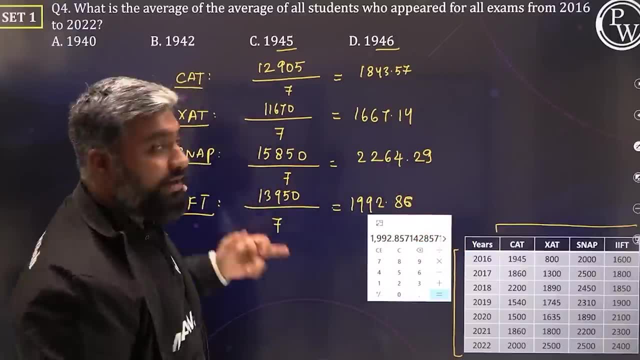 agar yeh dur hota hai- let's say, this was 1930, this is 1946- itne dur dur hota hai, toh theek hai. then you know, these smaller values won't badger us, irritate us so much, but agar values close enough hai, so you have to be super careful. 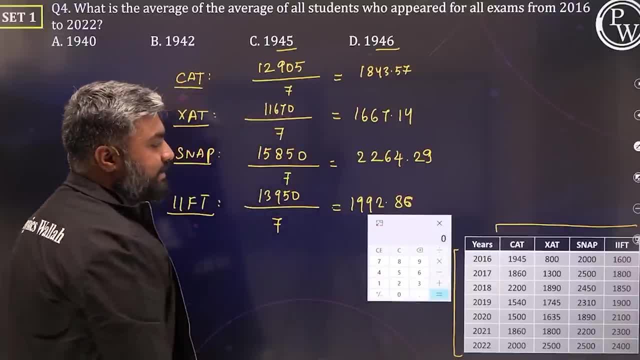 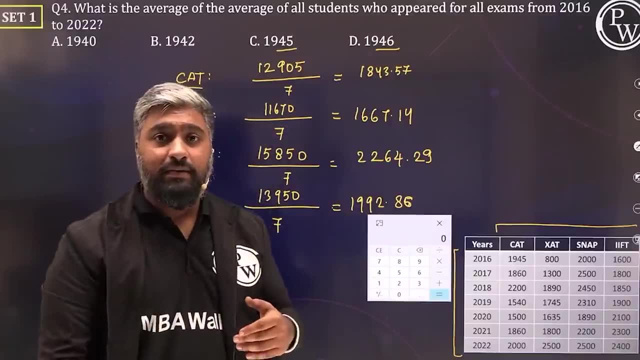 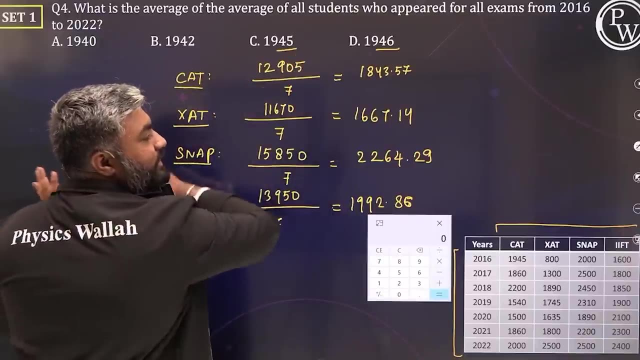 there. okay, so we have all the averages now. yes, ab humare paas saare averages hai ab kya karna. what's the next step? we have the averages. we need to find the average of the average. yes, so for average of the average, hum kya karenge. now, forget about all of this. yeh sab jo apne ab tak kiya hai na. 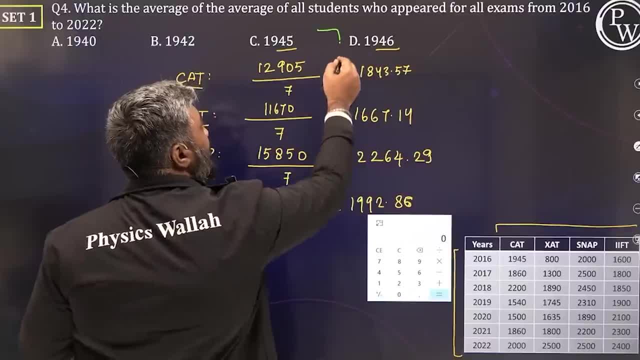 yeh sab ko aap abhi hold me rak denge you'll. you'll kind of forget about all of this. yeh ab hume matter nahi karta hai. we only care about these four values. right, toh aapke paas 4 term hai, unka. 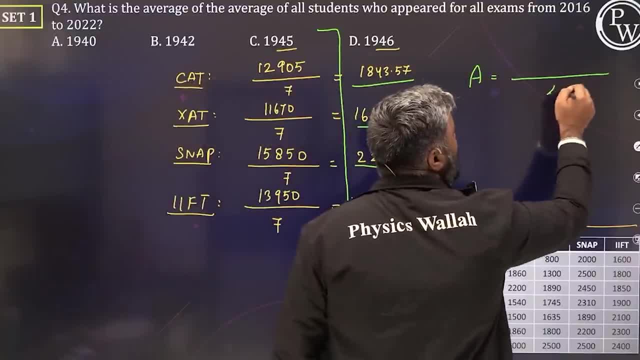 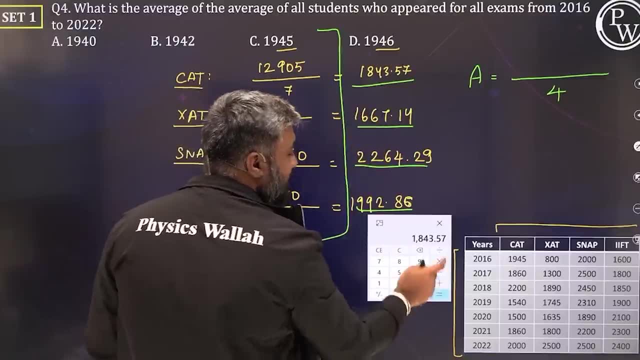 average nikalna tab. kaise karoge what will be the average 4 terms. so you have to add them up and divide by 4, simple right. so we take the calculator again. 1843.57. please mind the decimals. kyunki answer choice: kaafi paas, paas, maine hai, let's not take the risk, okay. 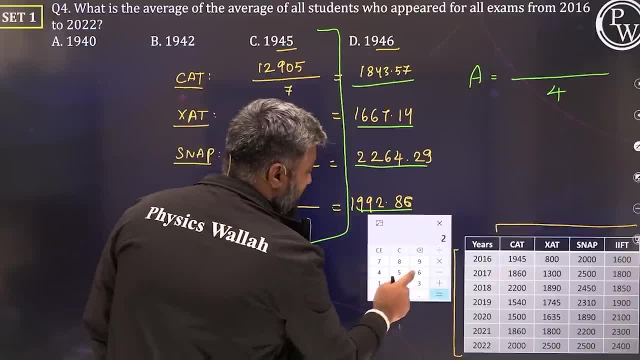 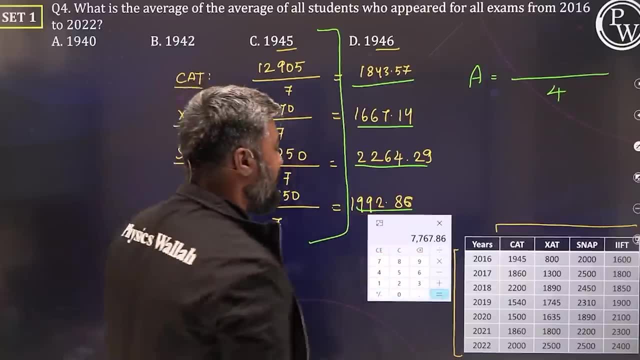 1843.57, 1667.14, W264.29 plus 94.9. so this is the average of the four terms. so you have to divide it by 14, 16.9 plus 1992.86. yeh agya amaar, total sum here: double, 7.67, double. 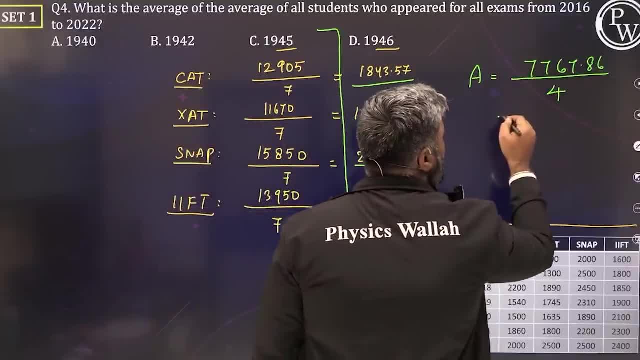 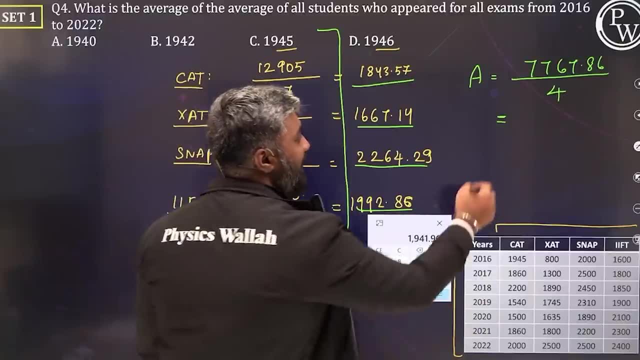 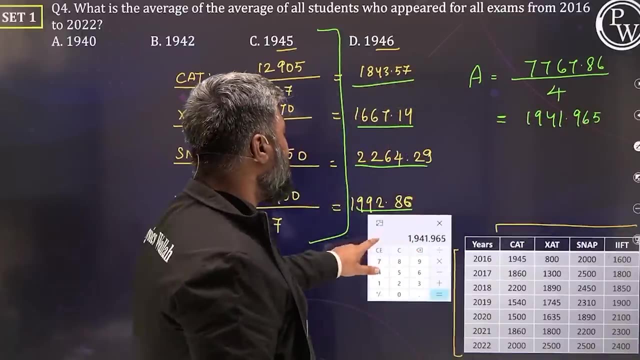 7.67.86. this needs to be divided by 4 to get the overall average, sorry, which comes up to 1941.9. 1941.965. yes, what do we understand from this is: se fab me, kya baata chal trak in 1941.965. 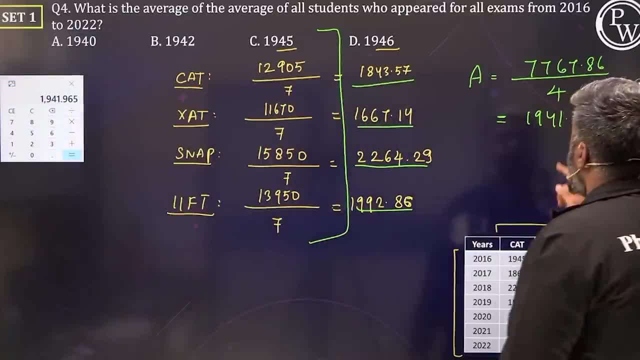 that means the third term in current time is nekta six nine. that means total point is one point nine hundred and one half nine hundred and one half four Century. so now that's three. closest that this could get to is what? 1942, approximately 1942. this will be our 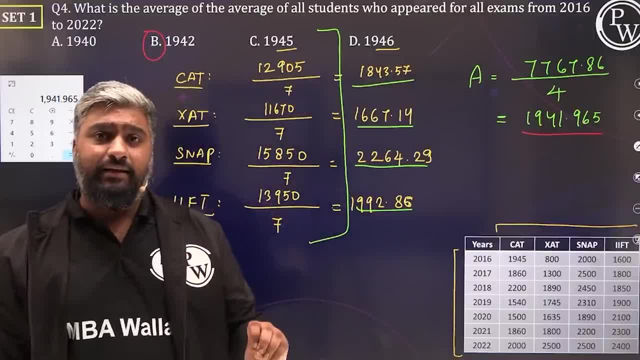 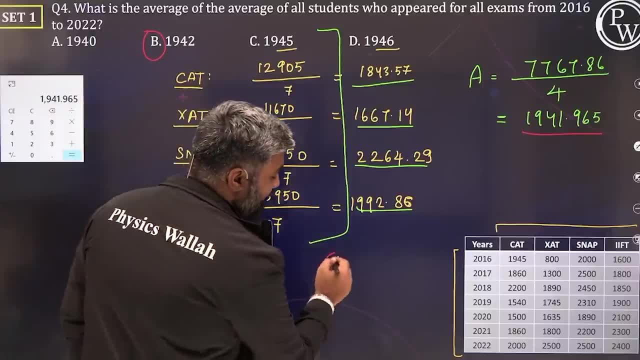 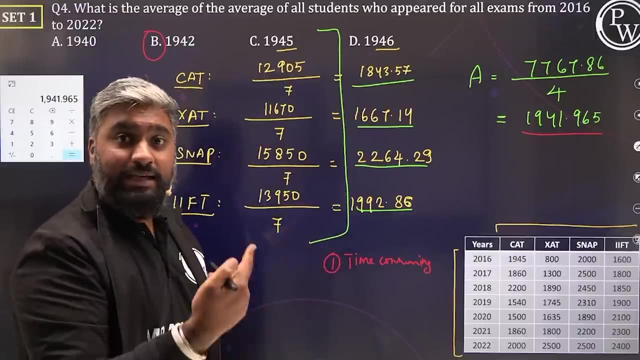 answer. I hope this is clear. process told us a lengthy head. yes, so if you were to, if you were planning on skipping a question, this could be one of those. why? because one time-consuming here- okay, so cookie time-consuming here. you might as well spend this time in some other set some other questions. you have a easily. 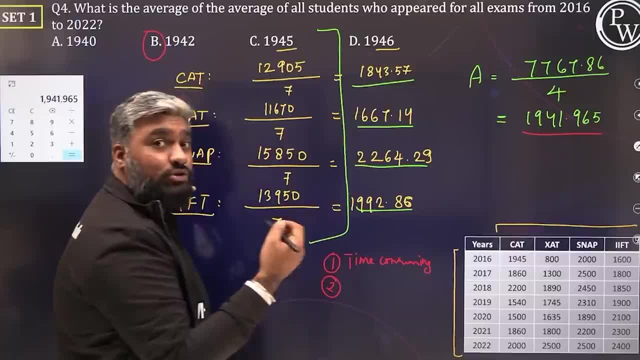 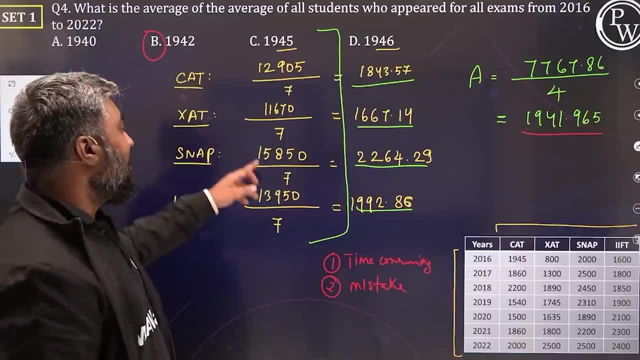 answer that. number two, because there's so much data, right. so much data, higher chances of making a mistake. yes, I got up to me, but we got the same equal value for me. check on, though, right, instead of 150, 850, you end up writing 185, 50. 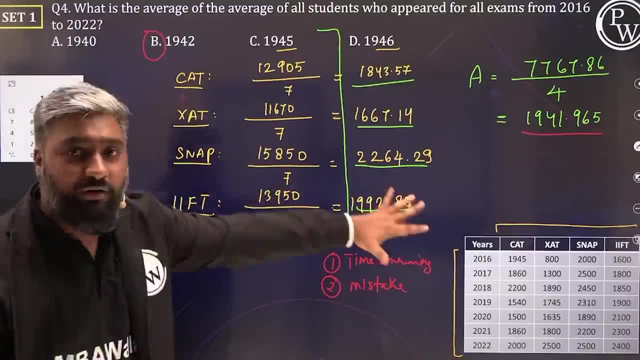 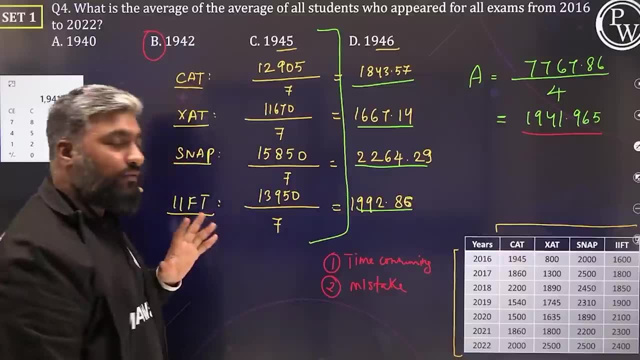 Canada a digit swap? oh yeah, by mistake, because you were dealing with so many of them who are cut up right, your entire answer will flip out. they have to be very, very careful not to make that mistake. yes, so other, if you were planning on skipping a question, this would be one of those. why, okay, coffee? 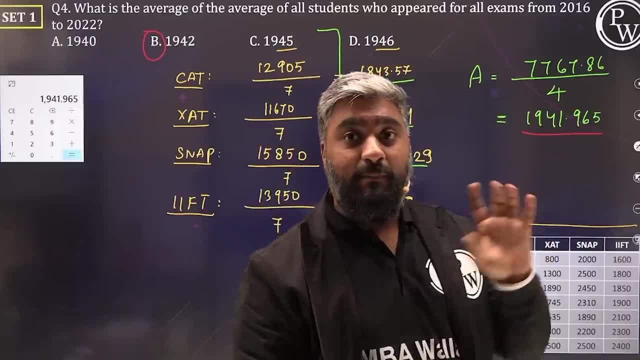 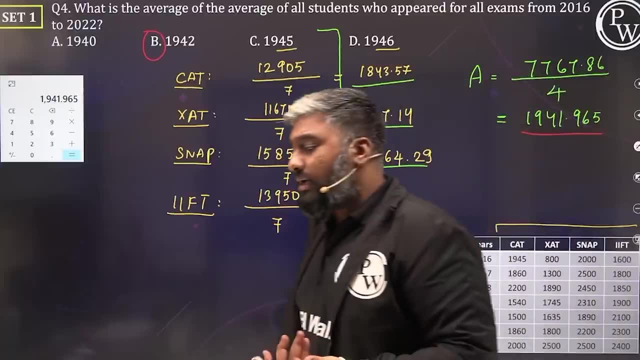 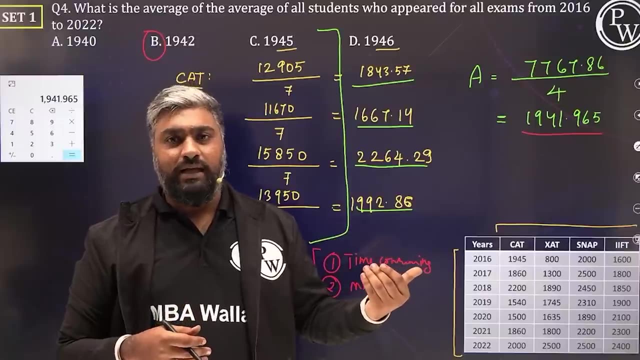 time-consuming here or mistakes. Carnegie coffee soda chances. but on the concept part, coffee, see concepts here, both he's other, easier to you. I had a very good divide turn. I could tie it name in a toast man, right, if you like to simply just add and divide. how much time do you think this is going to be? yeah, time later, yes, but 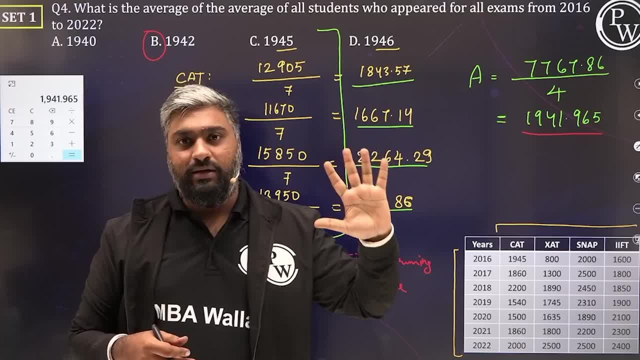 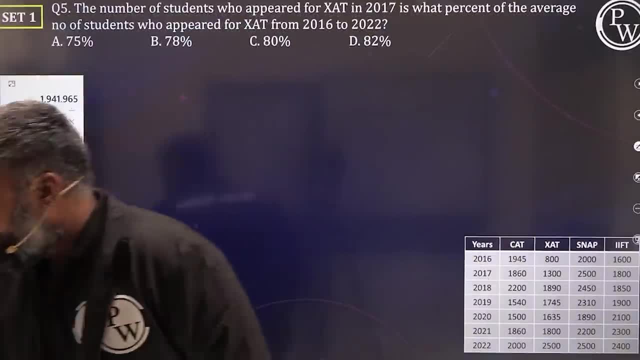 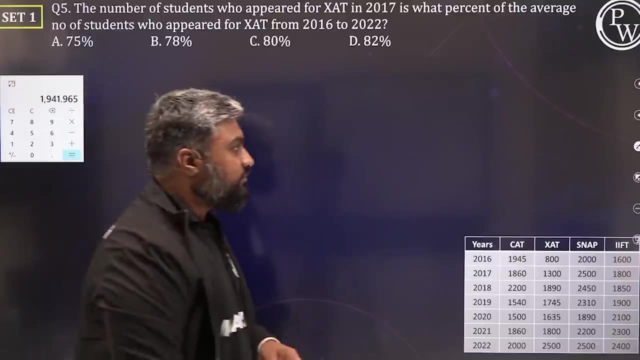 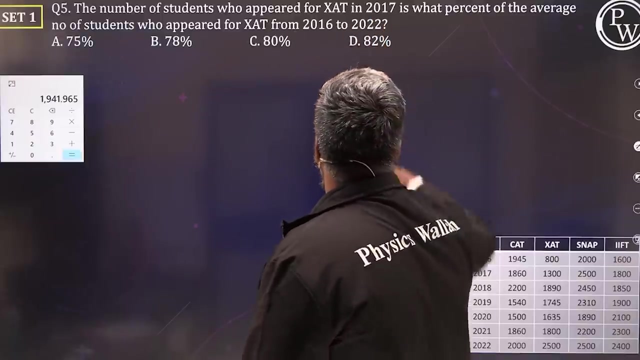 get not the mark giant elsewhere. in terms of concept, yes, I think that calculation you can do here. okay, let's go you. now. let's have a look at this question. the college in the last one from the set the number of students who appeared for sat in 2017. that is here. 2017 is yours when we're talking about this data. 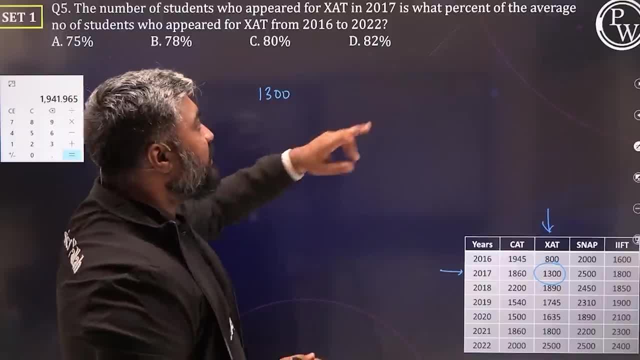 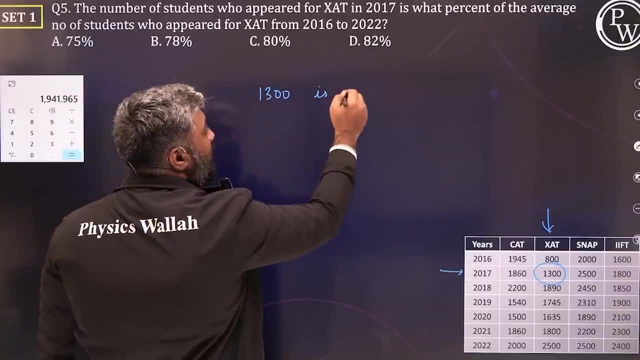 1300. is what percentage of the average number of students who appeared for Zach from 2016 to 2022- the year I knew Jo ahead- is what percentage of average of number of students who appeared for Zach? that average he poor average. you told him that the average number of students from 2017's. 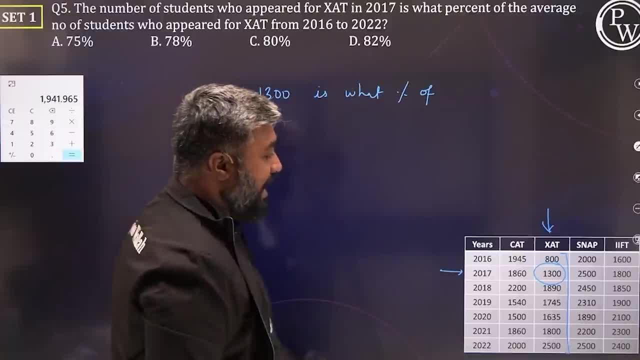 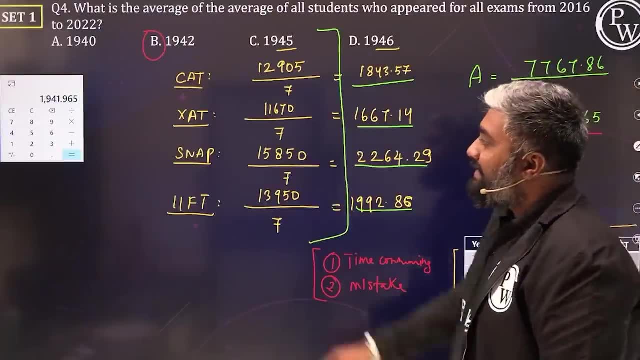 from 16 to 22,. correct, From 16 to 22 average. Now will you sit down again and add and divide for the average? No right. How will we save time here By looking at the previous one, Zat's average. we have already. 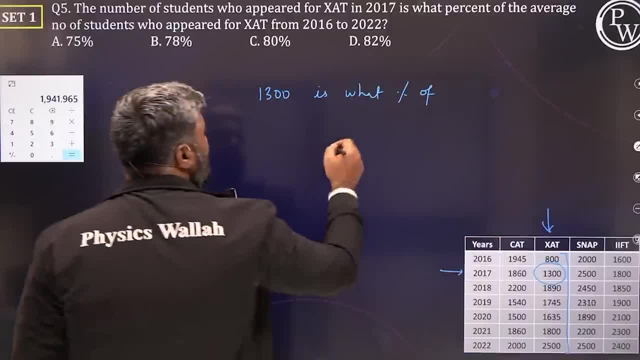 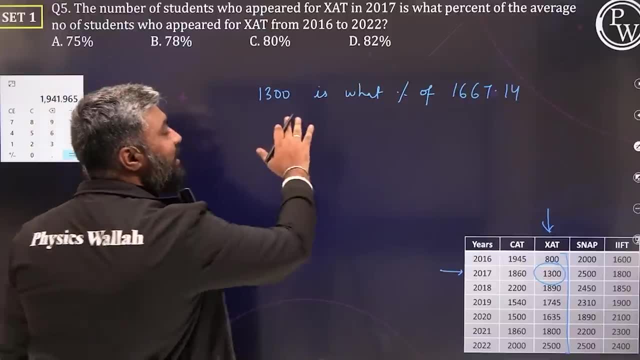 found, which is what: 1667.14.. Finished 1667.14.. We just have to find this. Finished Right. Simple division. question 1300 is: what percentage of? What percentage means what fraction of Right? 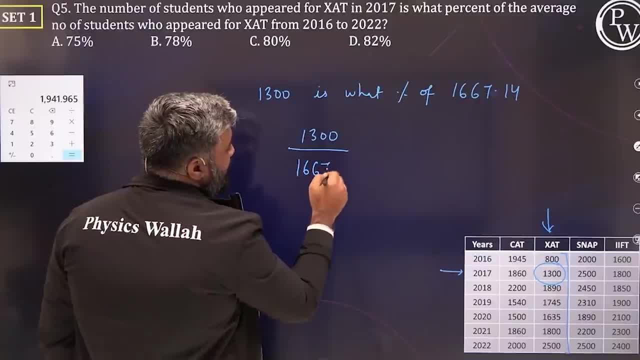 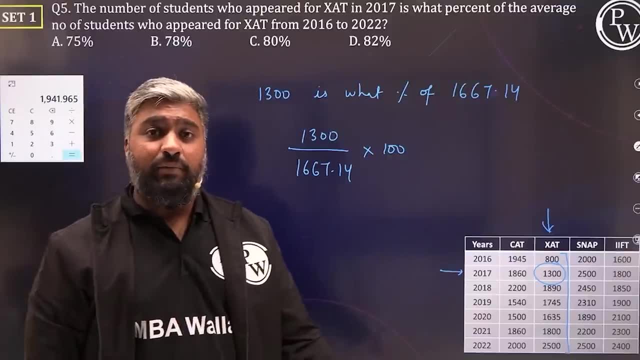 So 1300 needs to be compared to 1667.14 because it is asked in percentage, So into 100.. Yes, Normally the test which doesn't have calculator. I will suggest that you approximate it Right. Look at the answer choices and make a guess. 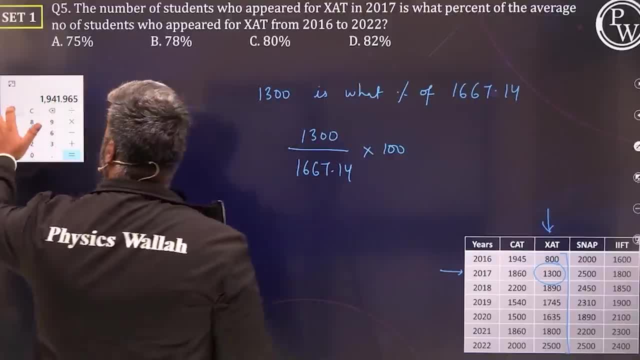 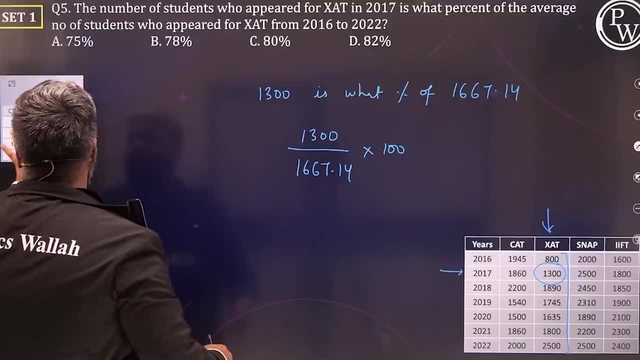 But because there is calculator here, let's not do all that extra fancy stuff, Let's keep it basic. Okay, So we have to do what? 1300 divided by 1667.14? What do we have to do with this? Into 100.. 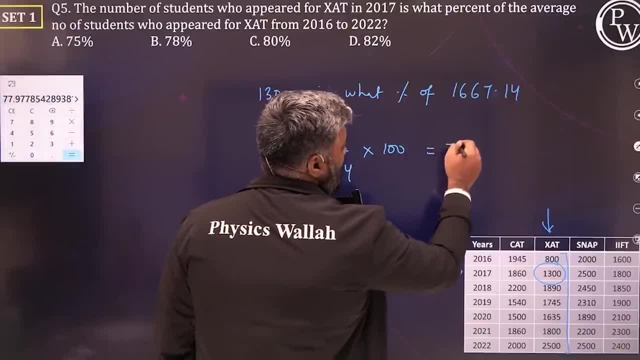 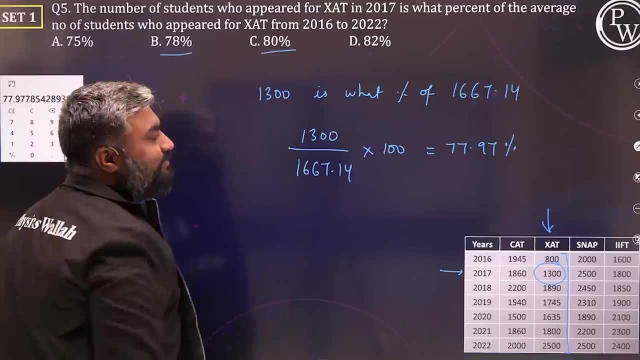 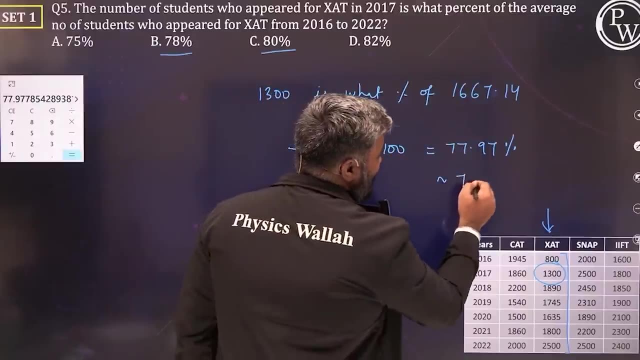 So we end up getting what? 77.97.. 77.97 percentage, which is very close to which value. 78 or 80? 79.97. Please be careful. 77.97, which is approximately 78 percentage. Yes. 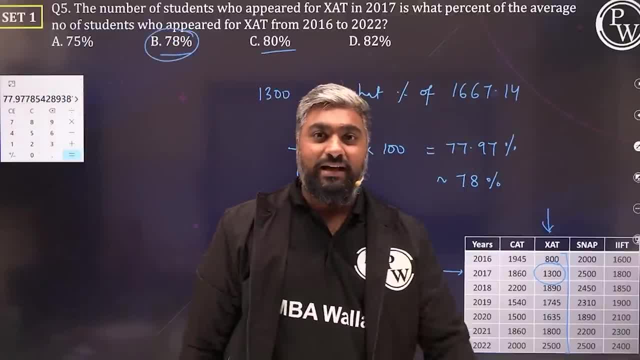 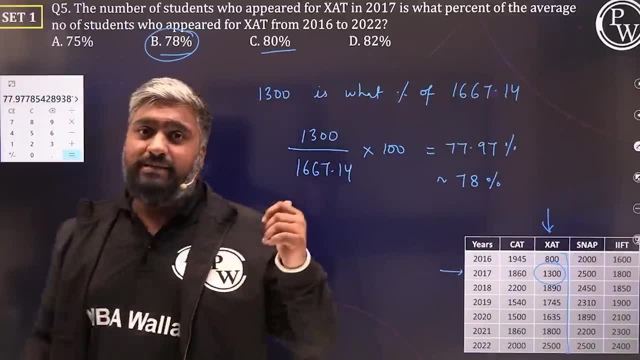 We end up making this mistake: 77.9.. The next value is 78.. Okay, Done. So first set is done. I hope you guys understood this. Then you can use the same thing. Right, But don't forget to subscribe to our channel. 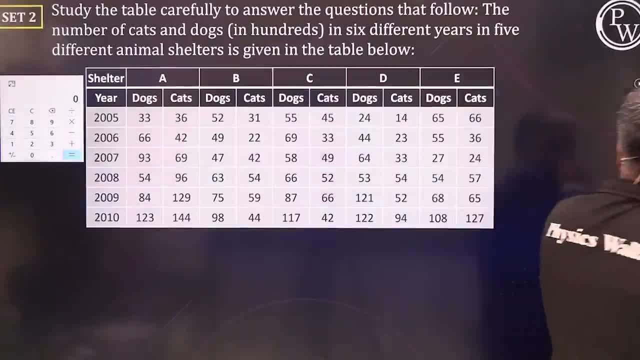 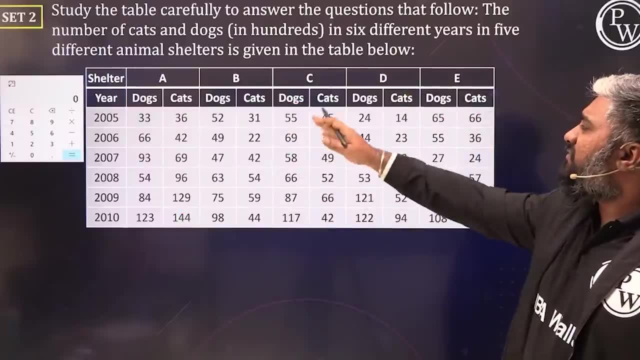 Don't copy, Don't set. So let's get started. Here is the set. Look at the table. There is a lot of data, So much data, So many different values. Right, I can see 1,, 2,, 3,, 4, 5. 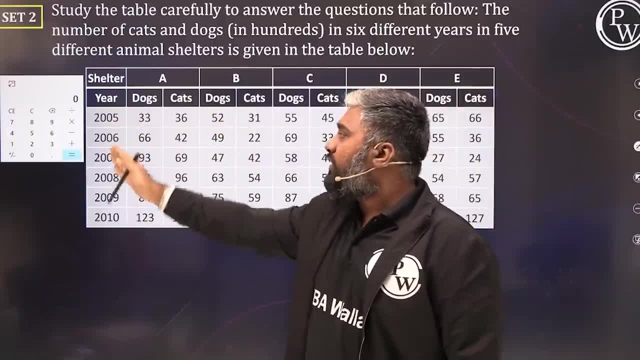 columns. There are 2 sub-columns Right And years go from 5 to 10, which is 6 years. Common mistake is from 2005 to 2010. we will say 5 years, but no, it's 6 years Right. 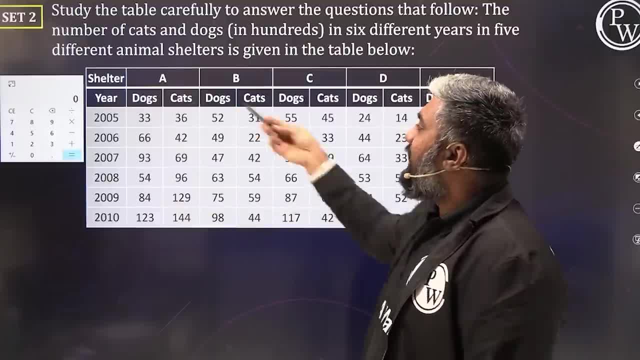 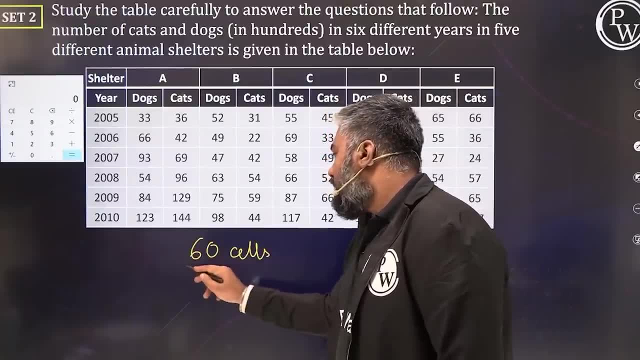 Because we have to count 5 too. So 5 to 10 is 6 years. 6 into these 10 columns, that's 60 pieces of data. There are 60 cells, Okay, So don't get overwhelmed. 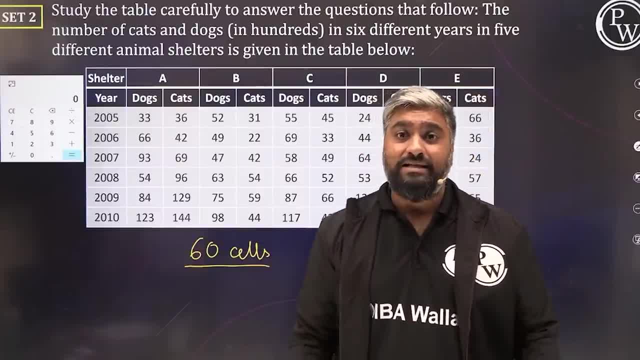 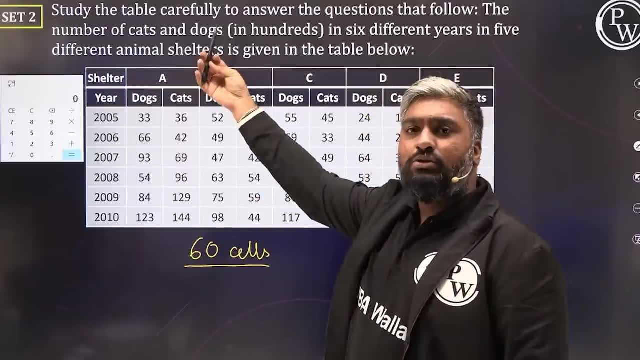 If you ever see a big table, a big chart, don't get scared. Size has nothing to do with complexity. Sometimes big sets become easy. Smaller sets become very complex. Right, Let's do the usual: Read the question statement, Study the table carefully to answer. 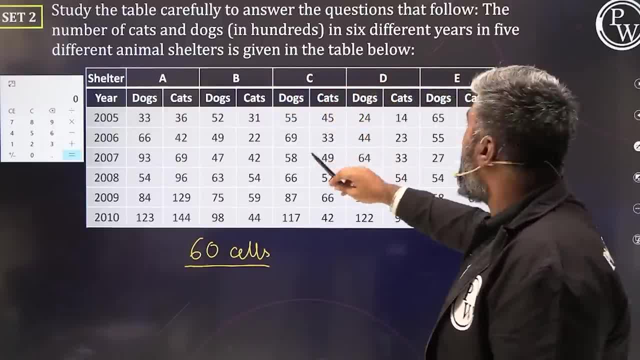 the questions that follow. That's the question statement. We also have information on the table. What did you say? The number of cats and dogs, Dogs, Cats- I have given In hundreds. So what is this, guys? What is this? 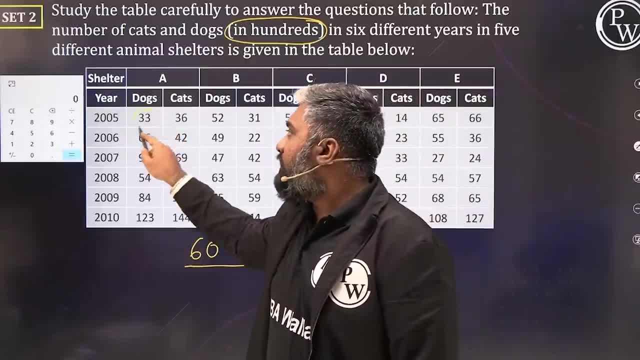 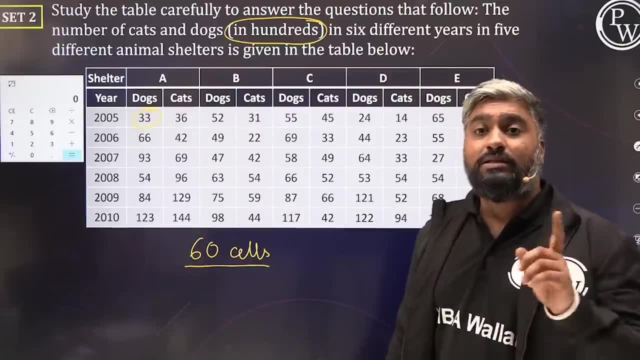 This is your scale. What does it mean? Yeah, In 2005, the number of dogs was not 33.. It was 33 times 100, which is 3300.. 36 into 100.. 3600.. So we have to put 2 zeros. 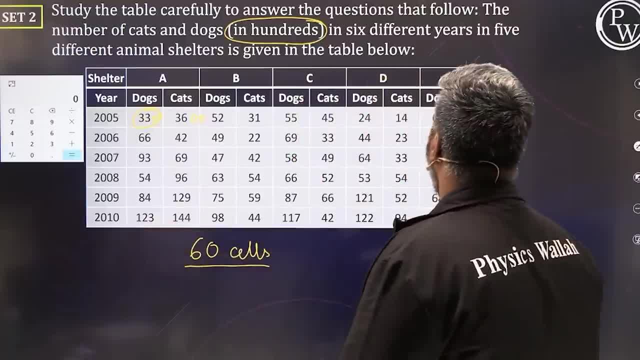 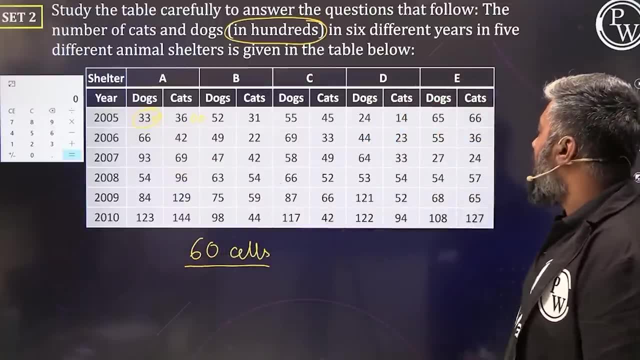 Yes, this is the scale. You have to be very careful about this. Okay, Moving on, In 6 different years in 5 different animal shelters. 5 shelters are A to E. 6 years are given. Very good, All data. 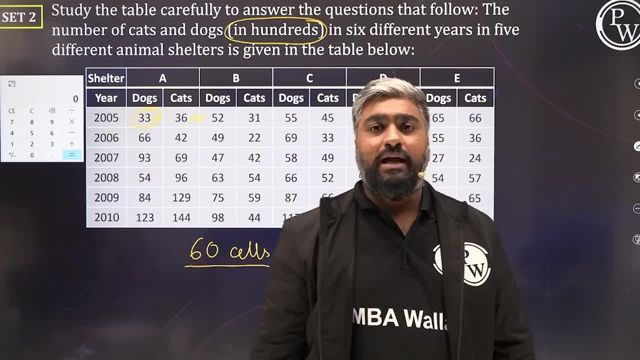 everything is there. We have given all the information Right. Once we are done looking at the set, the next thing we are going to do is what? Have a look at all the questions. So in this set there are 5 questions Right, We are going. 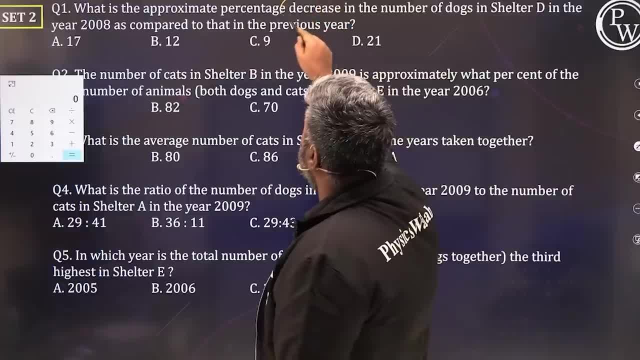 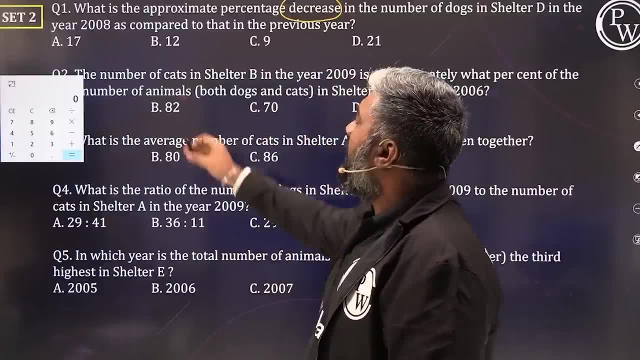 to quickly have a look at this. What is the approximate percentage decrease in the number of dogs in shelter D for 2 different years? Percentage decrease: We can do it Easy. question: Number of cats in shelter B in the year 2009 is approximately what. 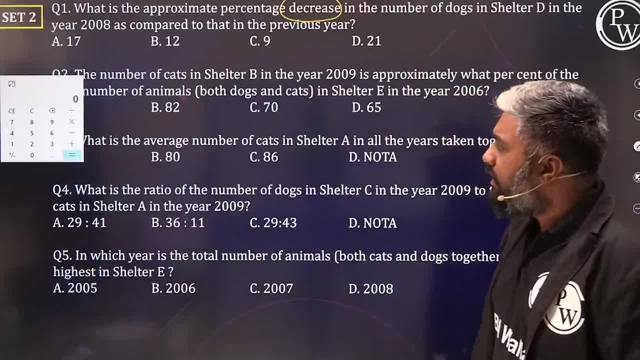 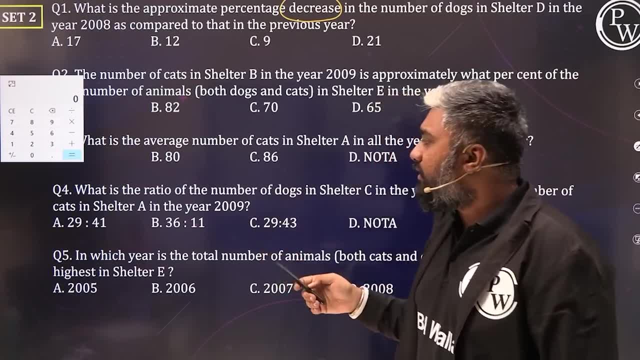 percentage of the number of animals. This will also be done. Simple calculation: What is the average number of cats in shelter A in all the years taken together? We have to get the average. We have done a lot of average questions. Very good Ratio is asked. 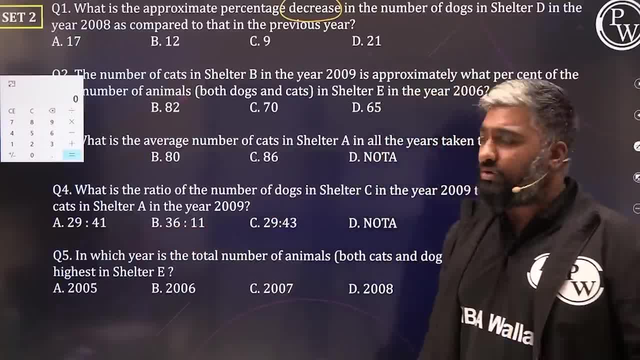 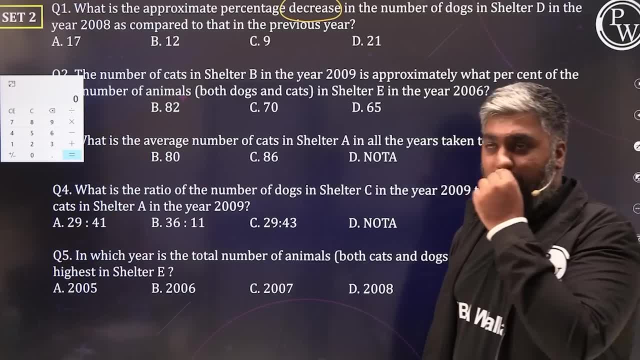 Dogs in shelter C to the number of cats in A, Ratio will be taken. Which year is the total number of animals, The third highest Right? So what to do? To find total animals, to find the third highest. Okay, So of the 5, 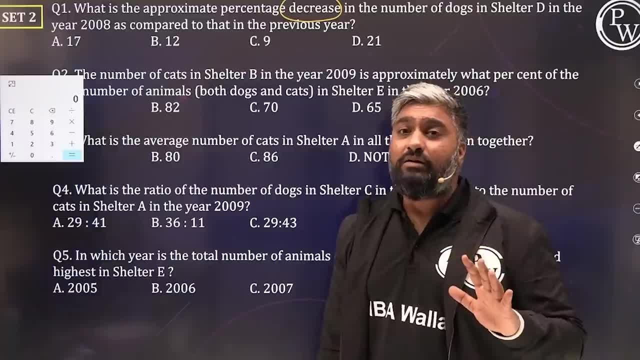 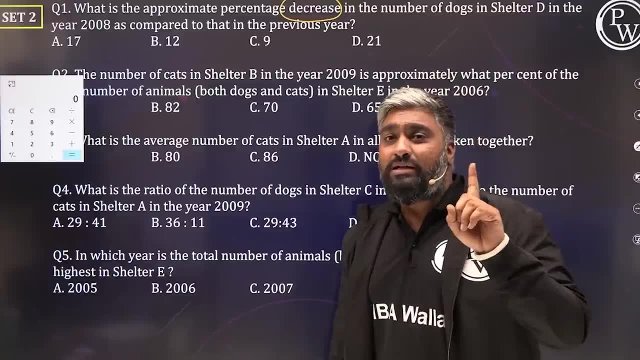 questions. of the 5 questions, is there any theta? No, There is no theta question, Meaning you have no easy questions which even if you don't solve answer then there is nothing like that, But there is one question that you can. 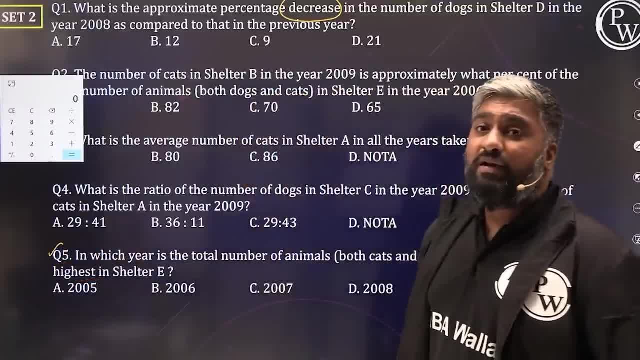 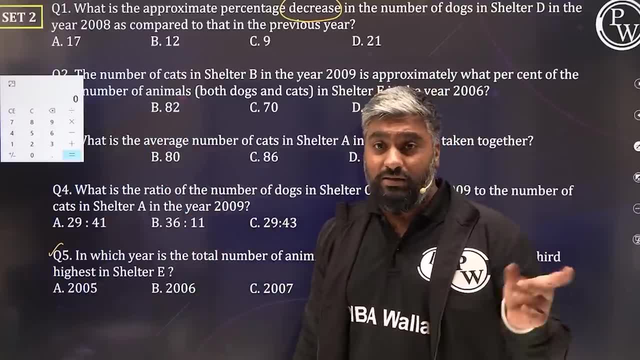 analyze and answer, which is this Fifth one, Right? So if I were you this question, if it comes in any test, then I would start with fifth, Because the one is easy. I can easily answer this. Just add and compare, Right. 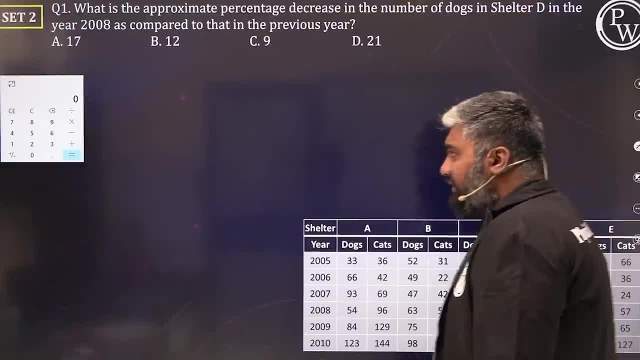 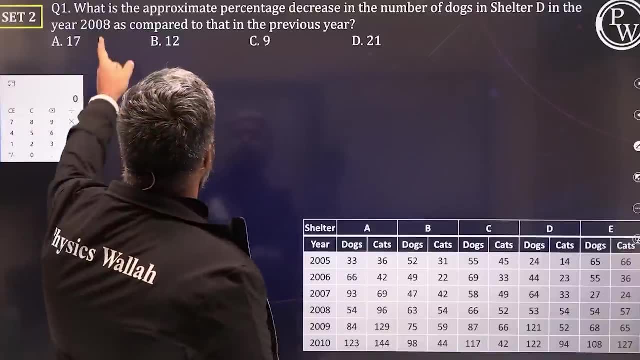 But now let's go to the flow. Let's start with the first question. I have put the table here. I have taken out the calculator. Why? Because I know that this is going to be a calculative question. Okay, So let's get started. What is the approximate percentage? 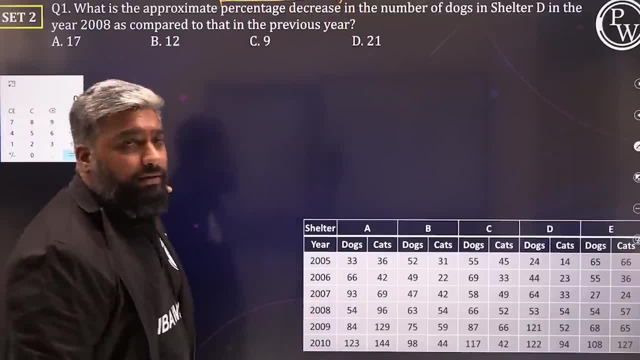 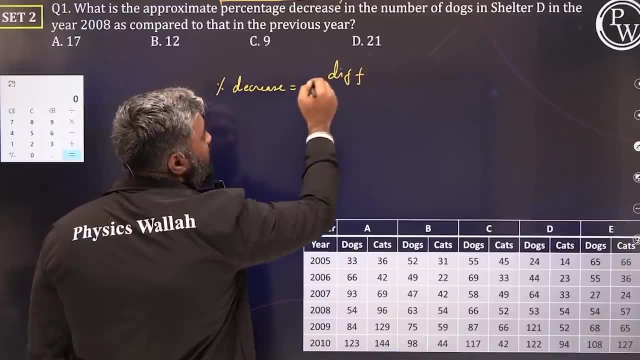 decrease. So to decrease the percentage, what will you have to do To find out percentage decrease? yes, you will need. what One? you will need the difference of the two values. You will have to divide it by the base value. Yes, we have already. 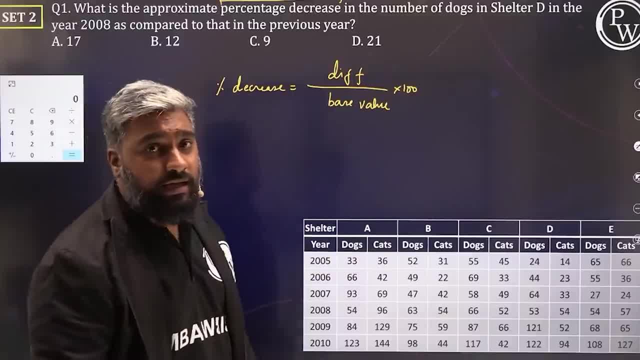 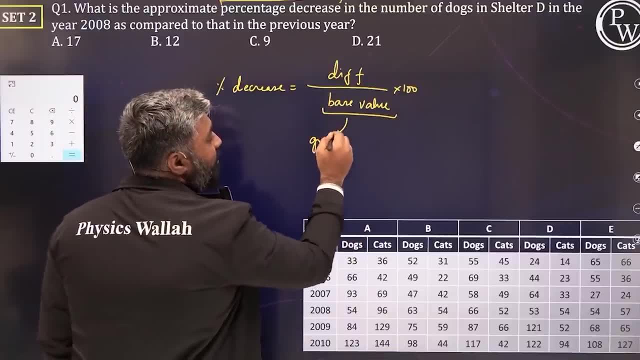 discussed in the first lecture, in lecture one, in introduction, and essentials that whenever we talk about decrease, whenever we talk of the decrease, then the base value is going to be what. Whichever is the greater of the two, The greater value will be in the denominator. 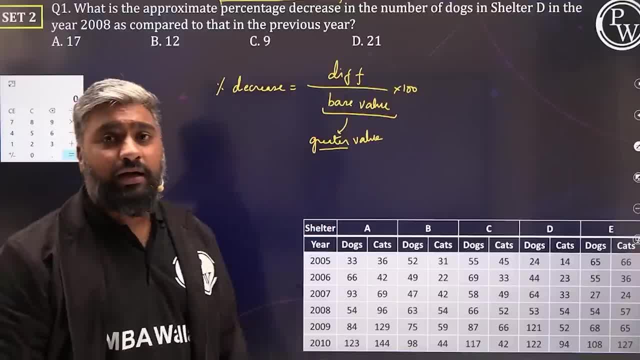 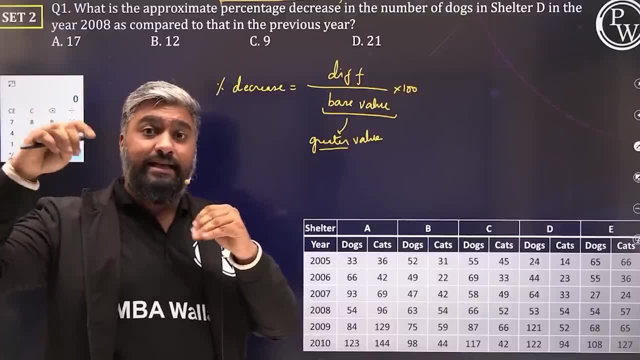 The bigger value will be in the denominator, Because you can compare the bigger to the smaller. You can compare the bigger to the smaller, The bigger to the smaller is not decrease From small to big, From smaller value to bigger value, is increase: The bigger to the smaller value. 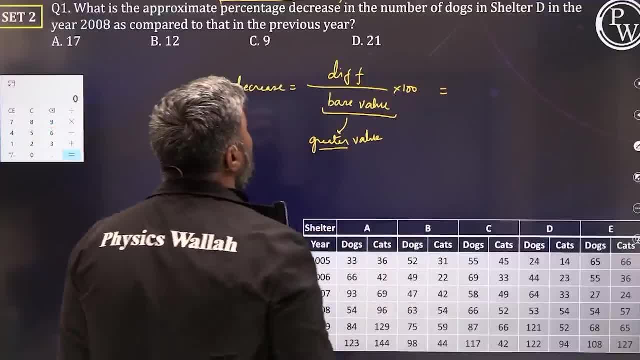 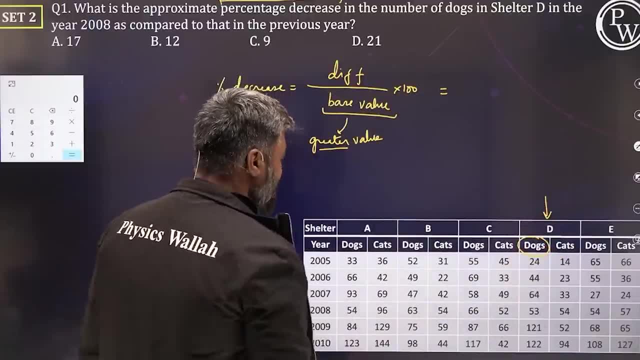 is decrease. Understood, Yes. So let's look at what the difference is. What data do they want? Number of dogs in shelter D. Shelter D: is this Number of dogs, is this column, In the year 2008, 2008? is this, Which is what? 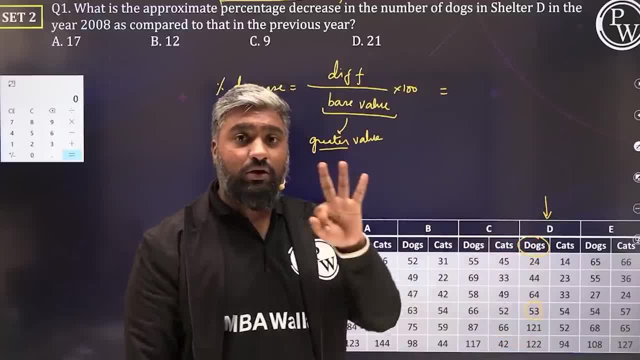 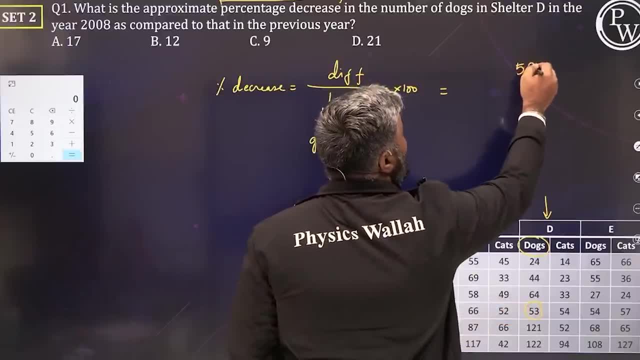 53. 2008 D dogs. Okay, So now you'll have to look at three things: Yes, In the column, sub column and then the row. So 53 needs to be compared. They're saying 53 is decreasing From where? 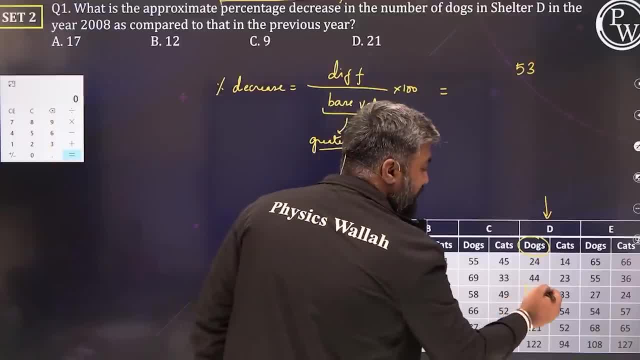 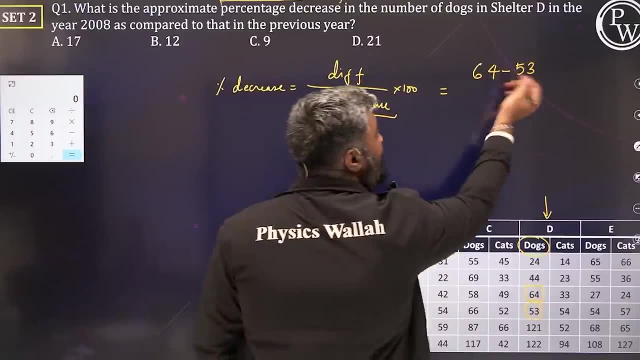 Compared to what? To the previous year? So what was the value in the previous year of 53? 64. So the decrease of 64 to 53 is asked, but in percentage. Okay, So this difference upon denominator, what will it be? 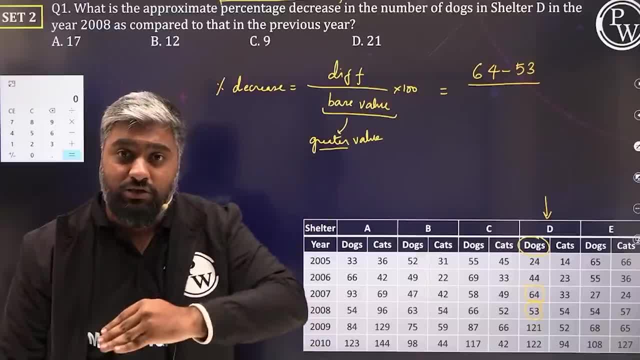 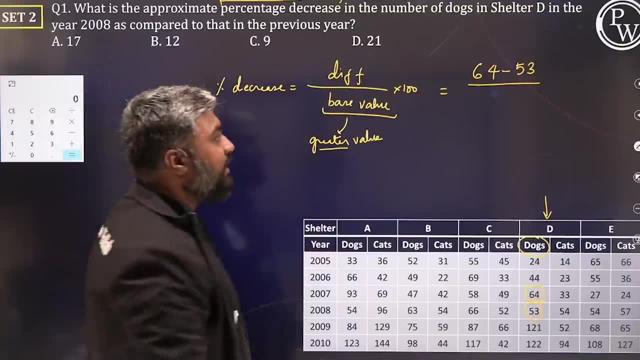 64 or 53?? 64.. Because decrease is from where? From the bigger value to the smaller value, From the greater value to the Sorry guys, From the greater value to the smaller value. decrease is there, Which is how much? 64.. 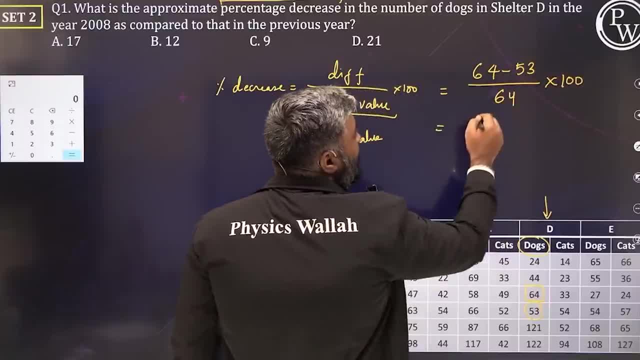 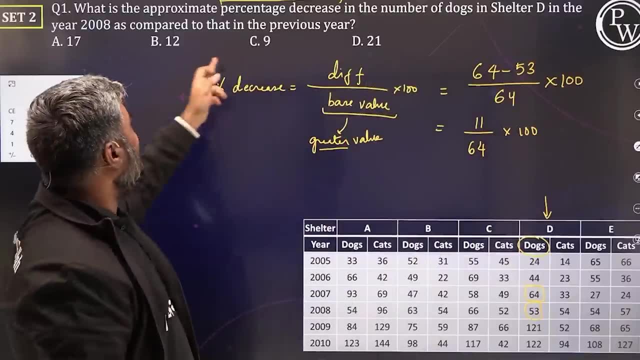 Because it's percentage, so into 100 as well. Yes, 64 minus 53, 11.. 11 by 64 into 100.. Normally again I say that approximately, I'll say that. look at the answer: choices 17,, 12,, 9,, 21.. 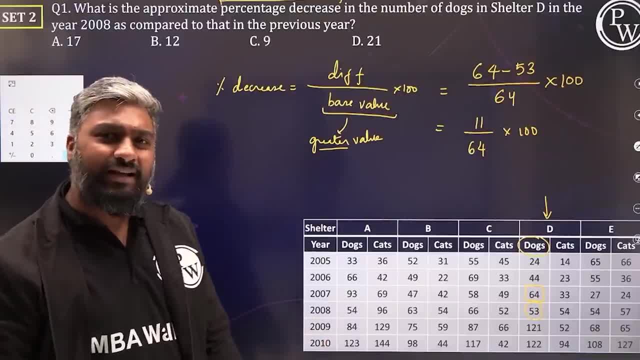 I think we can easily do this right. But because it's a calculator, what's the fun in it, guys? Yeah, So let's quickly go ahead with the calculator. By the way, approximately it'll be close to 1 by 6th. 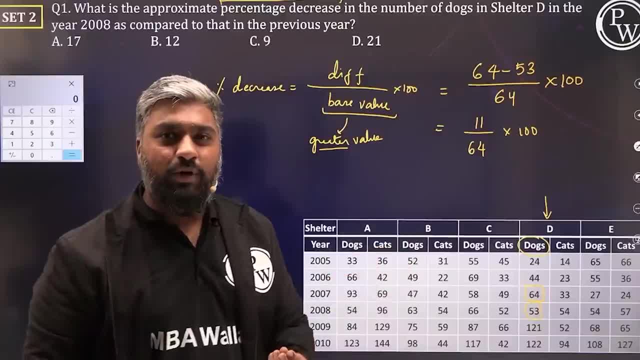 1 by 6th is 11 by 66 approximately. What's 1 by 6th 16.6 percentage? This is 64.. Denominator is small. That means the value will increase, So 16.6 is a bigger value. 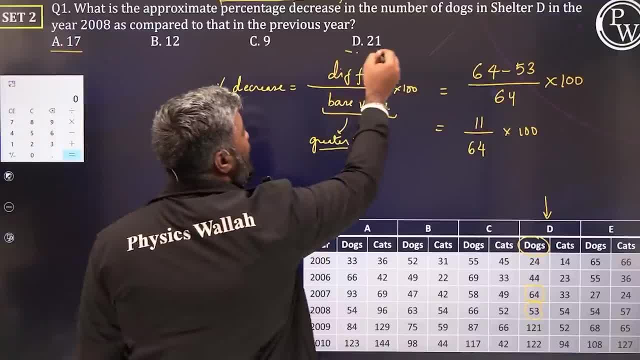 16.6 is a little bigger value. 17. A very big value is 21.. Now we know it's not that big, So we have the answer as 17.. But if you don't want to risk it, 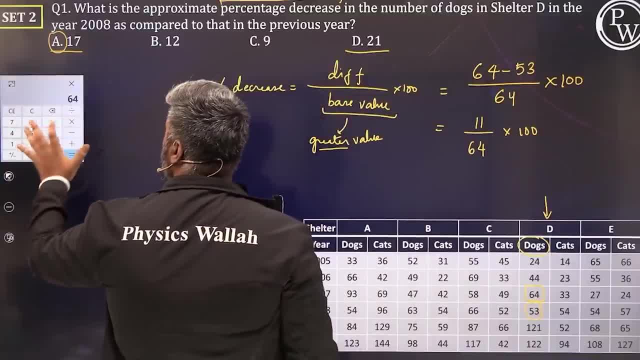 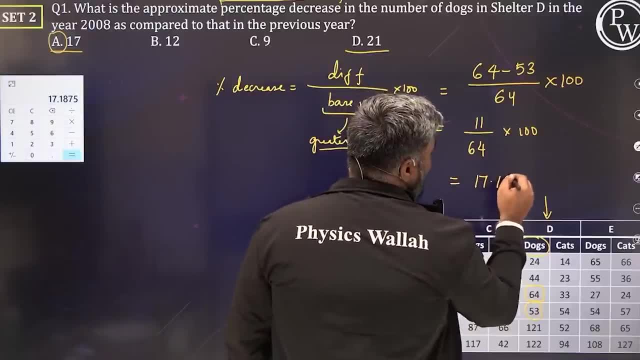 use the calculator. Yes, Let's confirm. 11 by 64 into 100 is how much? 17.17.. 17.1875, which is 17.19 percentage, What's the closest? 17.. Yes, So approximate. 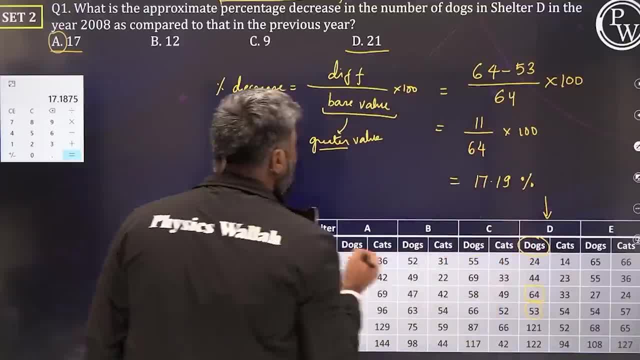 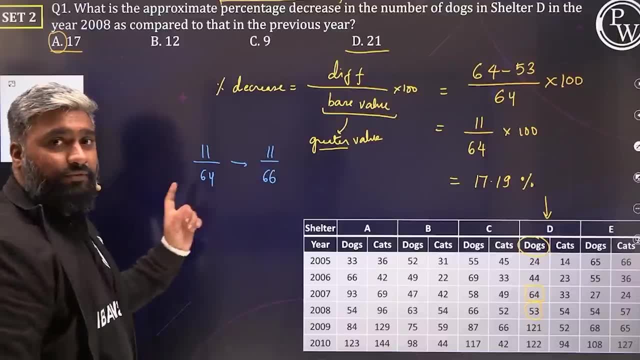 We did approximate. Let's repeat the approximation part. What was 11 by 64?? 11 by 64. I wrote it as 11 by 66. I made 64 as 66. I know this is 1 times, this is 6 times. 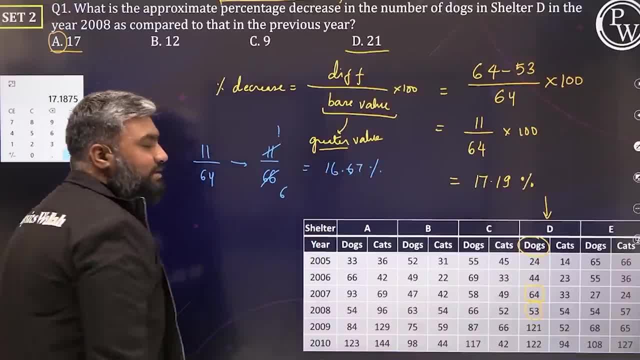 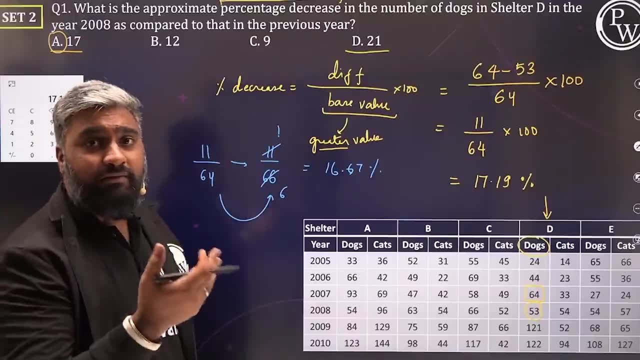 What is 1 by 6th, 16.67 percentage right? Yes, 1 by 6 in terms of percentage is 16.67.. But what did we see? That we increased the denominator. When the denominator increases, the value decreases. 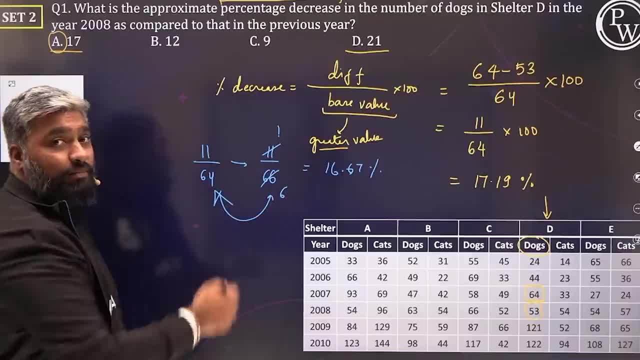 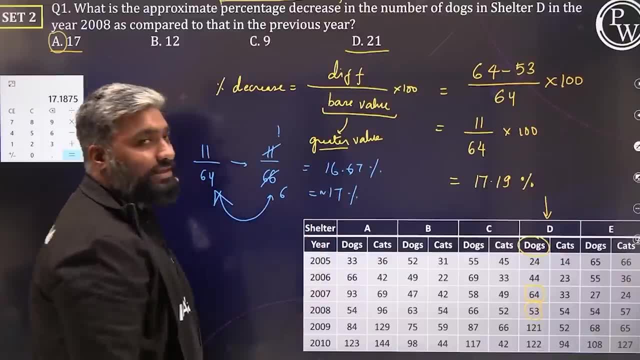 To go back. we have to decrease the denominator, Decrease the denominator. So when the denominator decreases, what happens to the value It increases? right, It should be around 17 percentage. It should be more than 16 percentage. 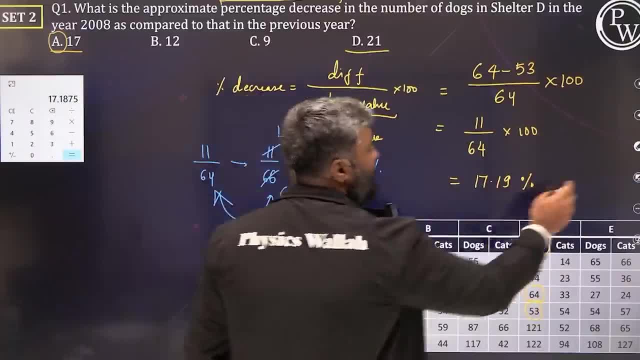 We know this much. Right, Let's say 17.. You will say, sir, you know the answer. That's why you are saying: But we know that my answer should be greater than 16.67.. There are only two answers. 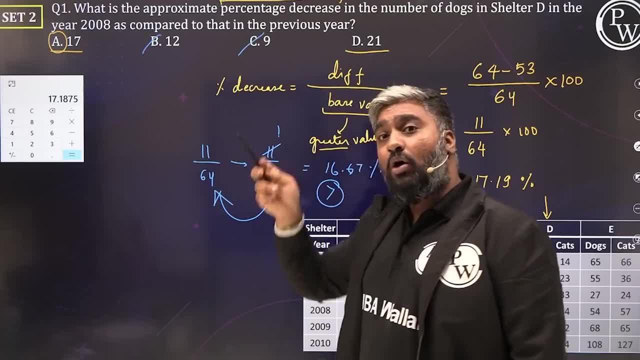 More than 16.. A and D. Between these two, 21 is very big. Yes, 21 is almost 7 more than sorry, 4 more than this. It won't be that big. Closest is 17.. 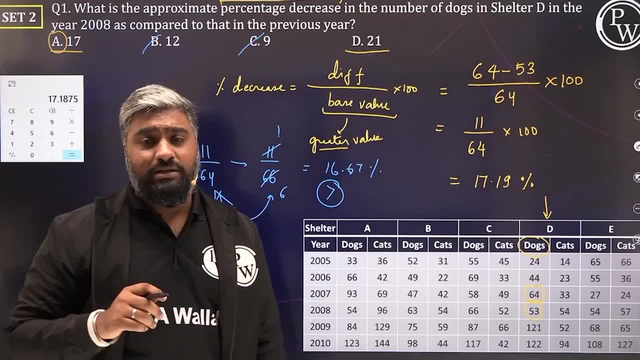 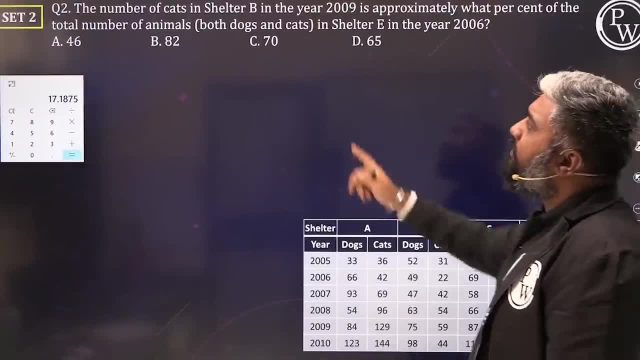 Okay, Do this if you are sure, if you are comfortable with approximation, And if it is not, it is a calculator, don't risk it. Okay, So let's go to the next question now, Question number 2. The number of cats in shelter B in 2009.. 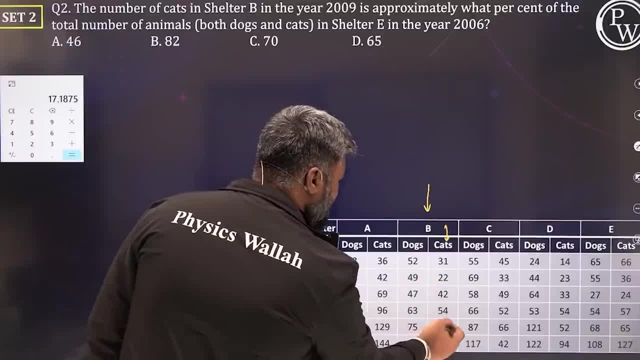 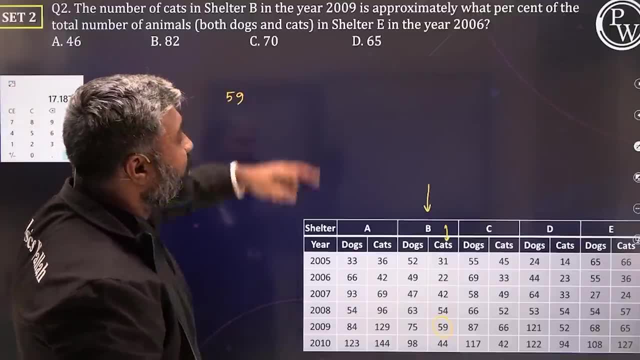 Shelter B: Here it is Cats. Here it is In 2009.. Which is what value? 59. Is approximately what percentage of the total number of animals in shelter E? So shelter E- Cats and dogs for which year? 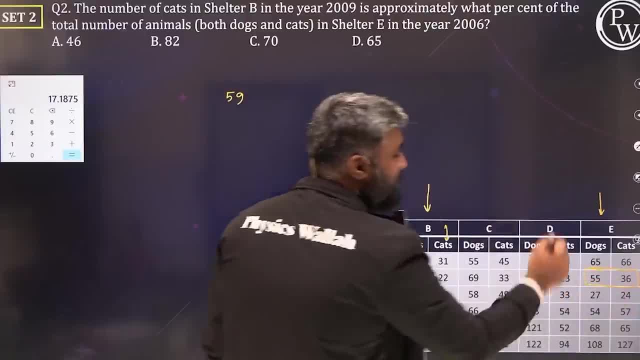 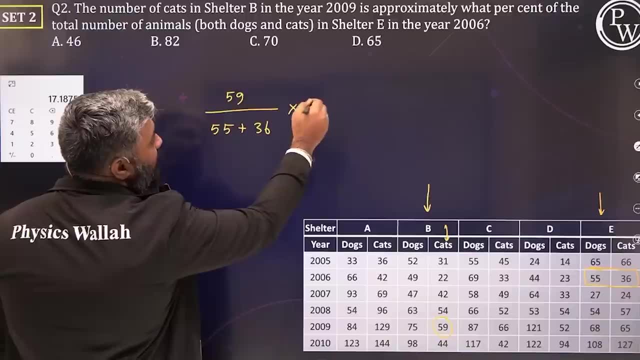 In the year 2006.. So this: What is the percentage of this sum? So 59 is what percentage of which value 55 and 36 together? In terms of percentage, it is said Here increase and decrease is not asked. 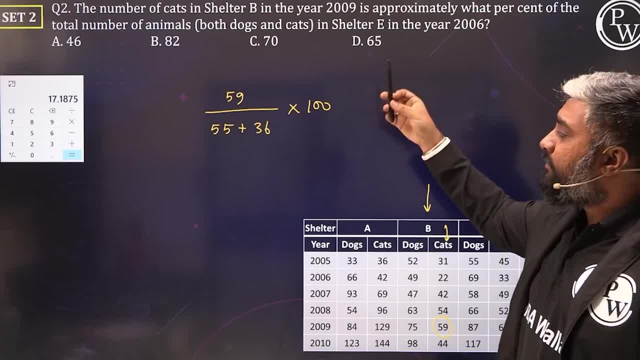 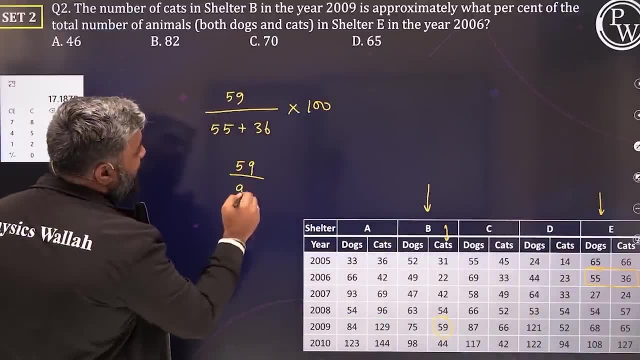 It is just said to compare Cats in B in 2009 is what percentage of this sum This one? Okay, So what happened here? We have to go for what? 59 by this is 80,, 91 into 100.. 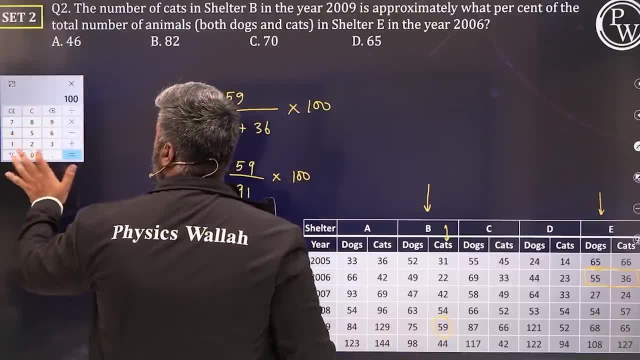 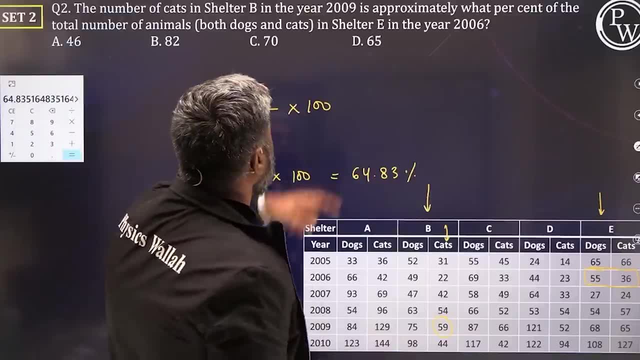 It is a calculator. Use it 59 by 91 into 100.. We get what 64.83, percentage 64.83.. Closest is what 65.. We have an answer, Okay. Yes, I hope you are clear with this. 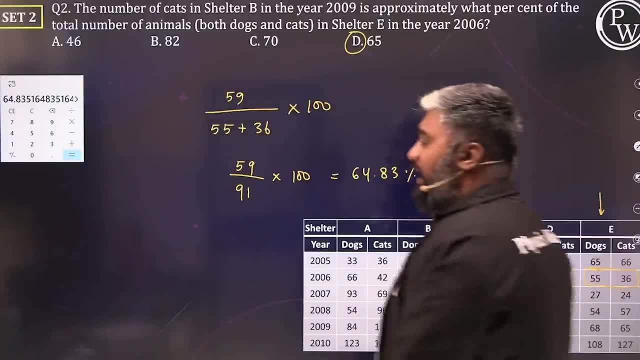 Cats or dogs. keep this in mind, guys. Do not mistake, Make this to be 75.. I will tell you why. If we would have done 75 by 91 by mistake, then we would get answer as 82.41.. 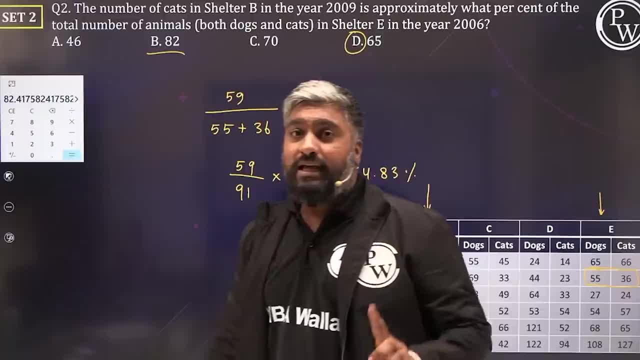 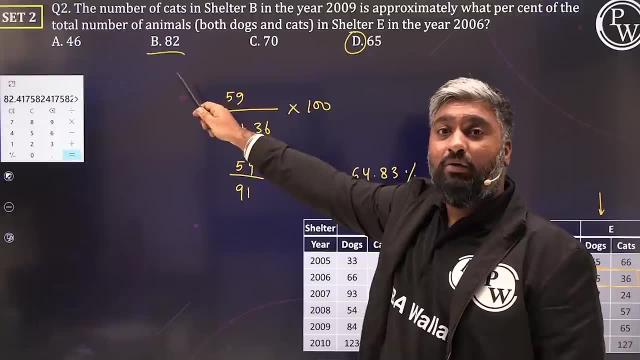 82 is this: They anticipated the kind of mistakes that you could make. If you picked up a dog for 75 instead of cat, then what will happen? 82 will be the answer. You will think that, yes, it was the right answer. 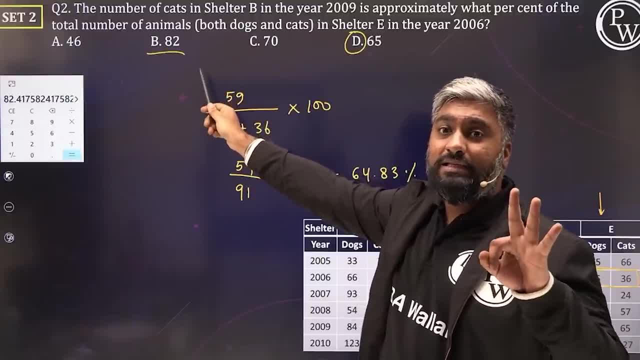 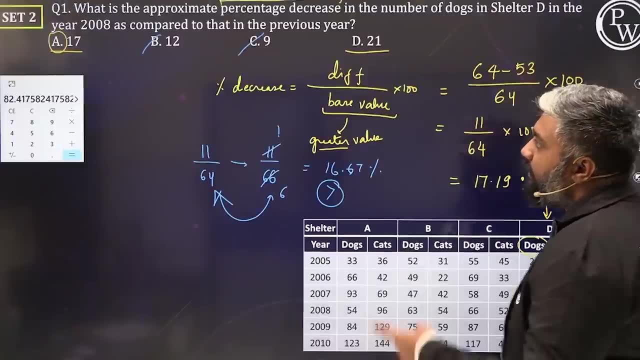 Very easy question, easy set, But you will end up losing out the three easy marks and one negative mark. Okay, Please be careful. Similar trap. Similar trap is also there in this question. See, You have a trap in this too. 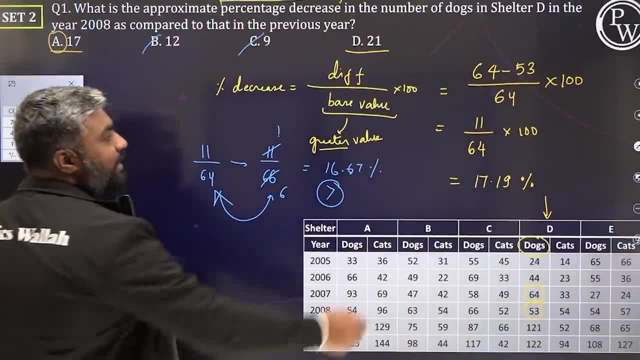 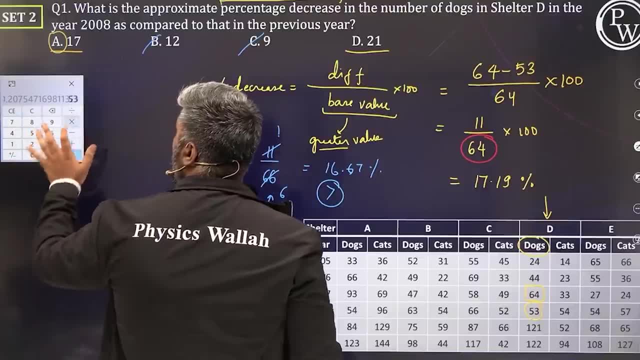 You might not have seen this carefully. Yes, Look at this Here: Instead of taking 64 as the base value, Instead of 64, if I had taken 53.. 11 by 53 into 100.. 20.75.. 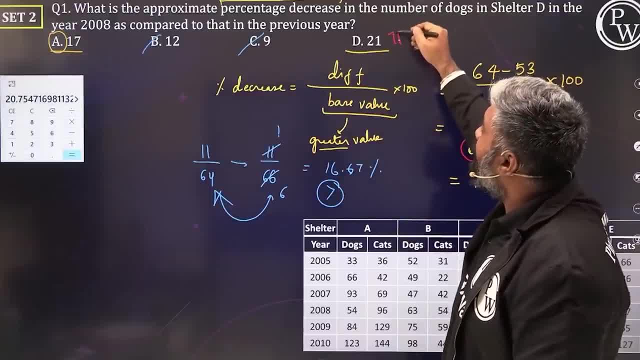 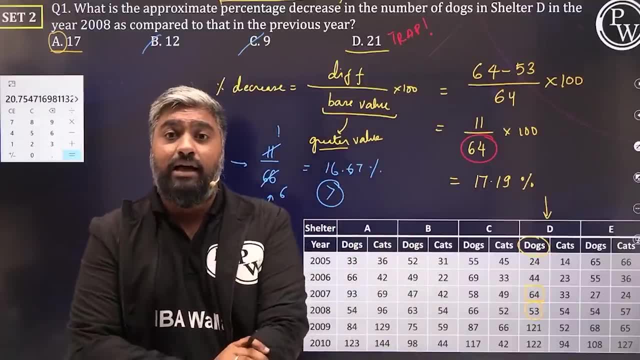 20.75 is approximately 21.. It is a trap. Yes, You have to be super careful about these traps. That is why we anticipate and set that these are common mistakes. Right, When he sets the question paper, he knows what kind of mistakes the candidates can make. 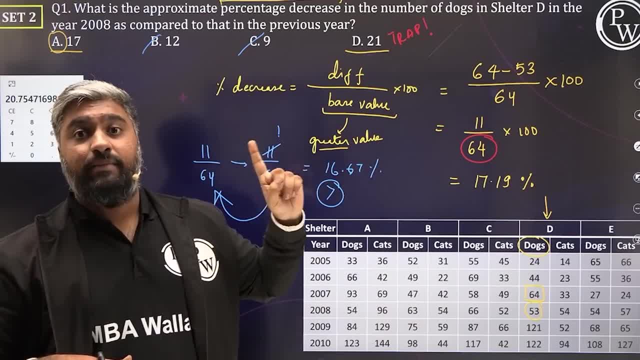 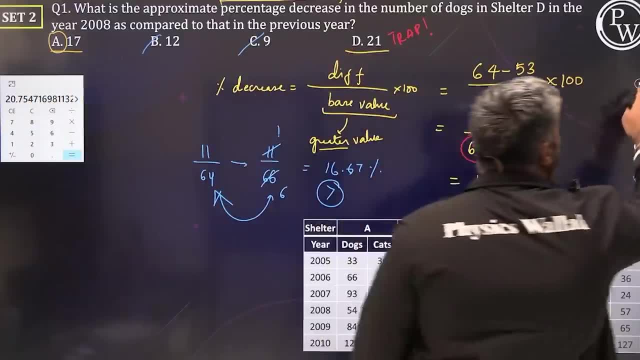 Under pressure. They will take advantage of that by setting these kind of traps. So please keep yourselves away and safe by retaking whatever you've done. Okay, Two questions done and dusted. Yes, Let's move on to the third one. 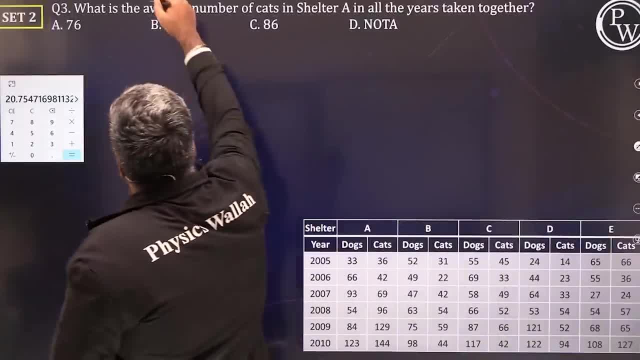 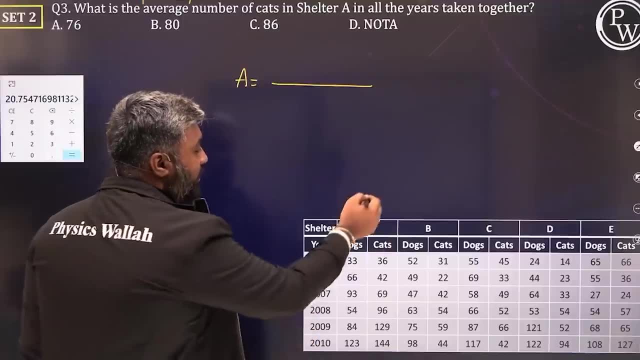 What is the average? So average is asked. I know what we have to do for average. We have to add all of them up and divide The number of cats in shelter A in all the years taken together. Number of cats for all the years. 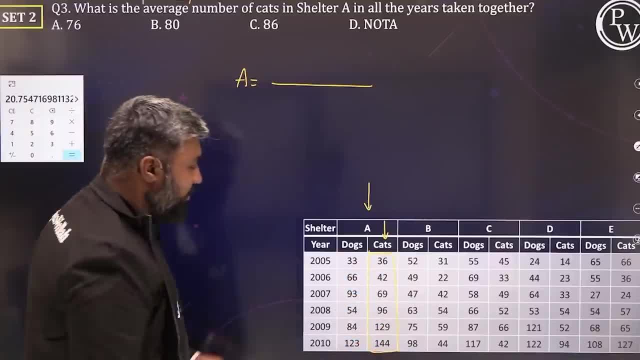 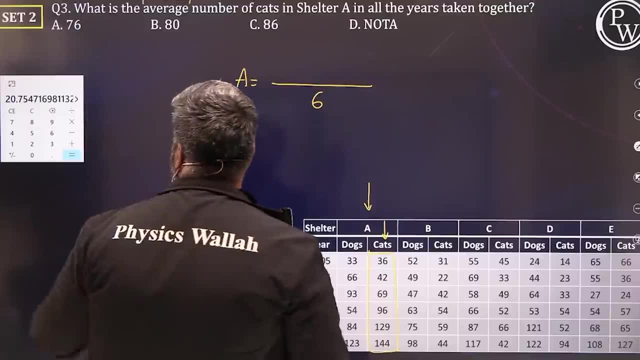 That means I have to add up all of these And divide by what value 2005 to 2010 is six denominator of the six radar. You need to add them all up. Yes, Let's do that quickly. So what is it? 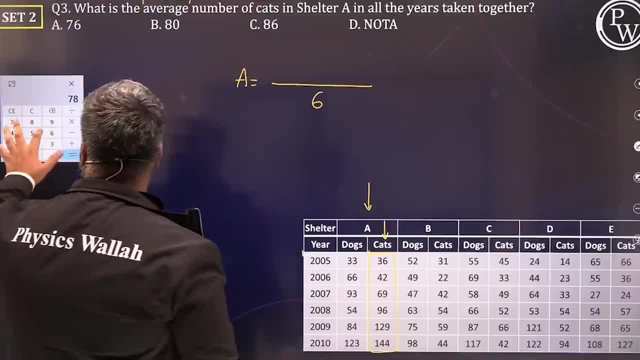 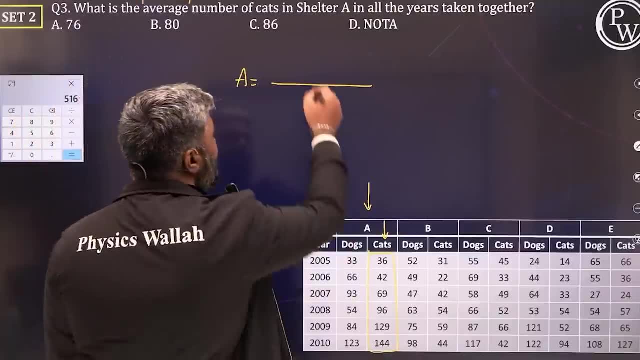 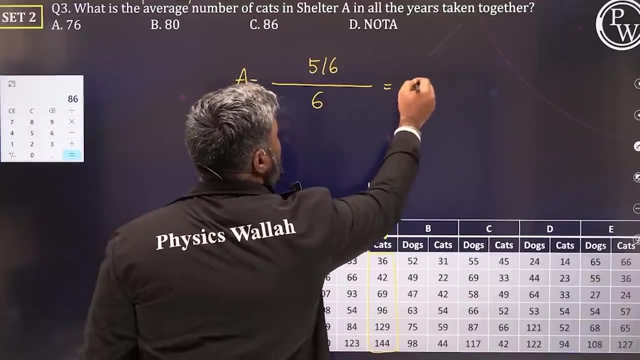 36 plus 42 plus 69 plus 96 plus 129 plus 144, which is 516.. Yes, 516 divided by 6 gives us how much 86.. 86.. What is the answer in the answer choices? Here it is. 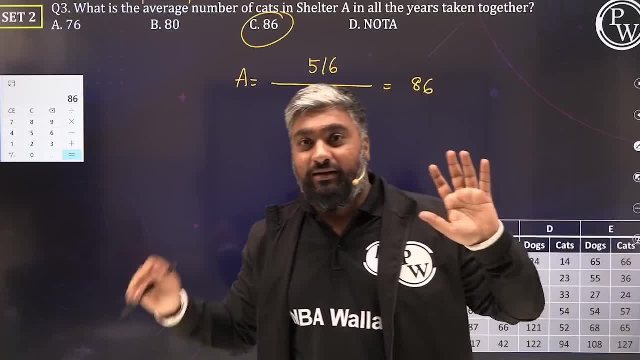 You will think that, wow, such an easy question. If it comes in the cat, then it is very easy, Right. But you made a very huge, you made a big, humongous mistake. The answer is supposed to be none of the above. 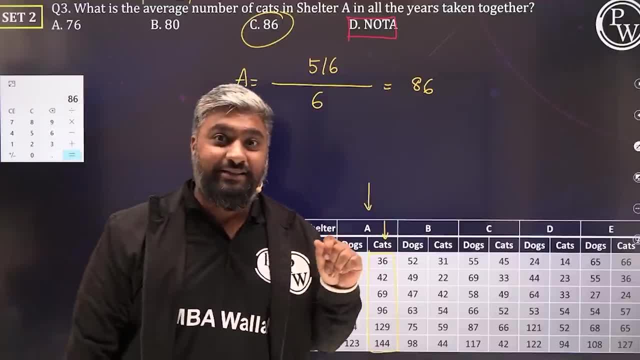 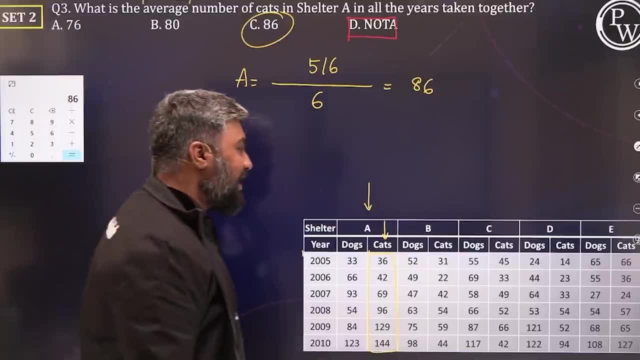 Do you know why? If you know this, quickly drop it in the comments Right. Drop it quickly, I will give you time. I will give you two seconds. Quickly drop why the answer is not 86. Quick, Very good. 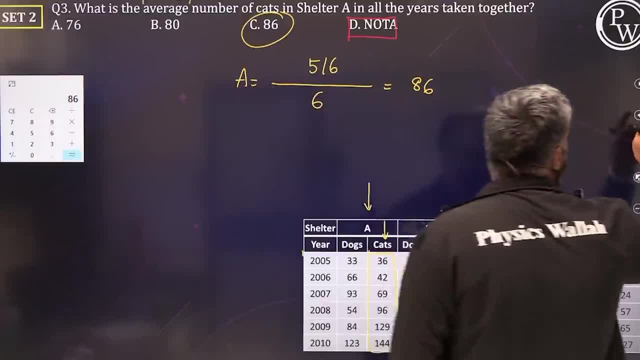 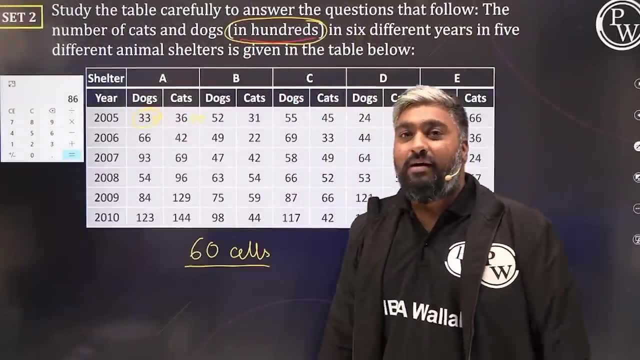 People who guessed it. Very nice, Beautiful, These values. See, we read in the question: These values are not to be taken directly. Instead, what is this In hundreds? Yes, Now you will think that, sir, you did not even talk about these two questions. 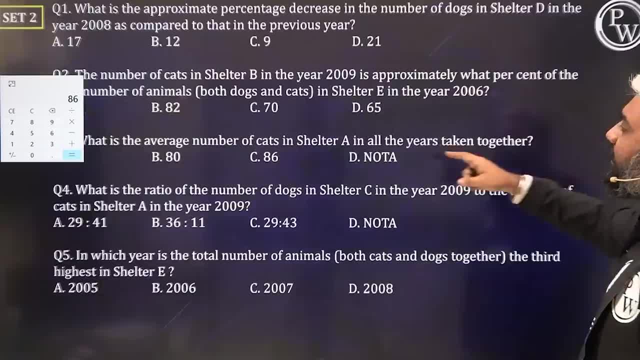 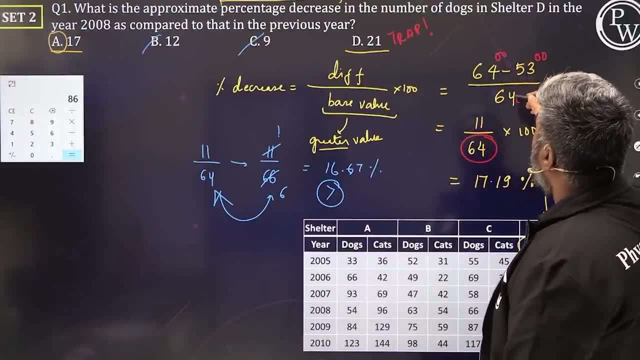 About the scale. Suddenly you are scaling. Why? It does not matter here. The scale does not matter here. Why This? 6400.. 5300.. Divided by 6400.. Yes, 11. 20. 20. 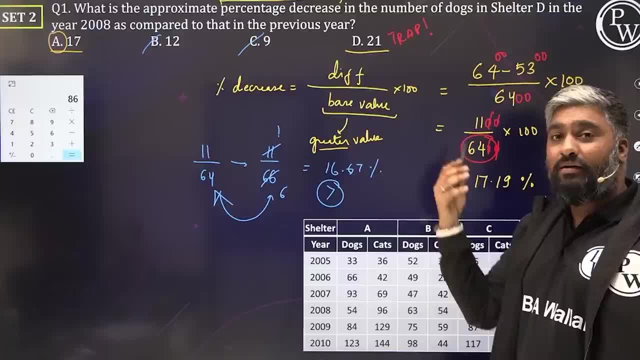 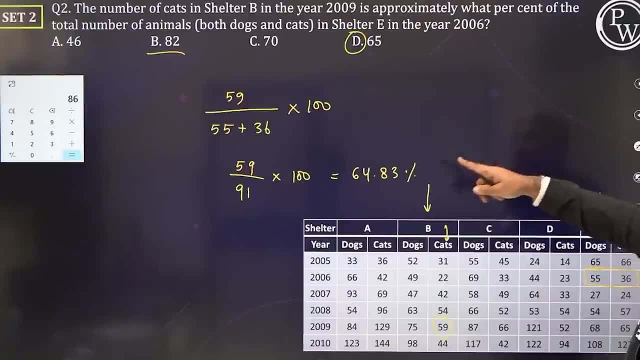 This 20 was getting cancelled anyway. Yes, So in percentage comparison the base has no importance, Right The base. The scale has no importance because it was getting cancelled out. Yes, See here also Same thing: 5900.. 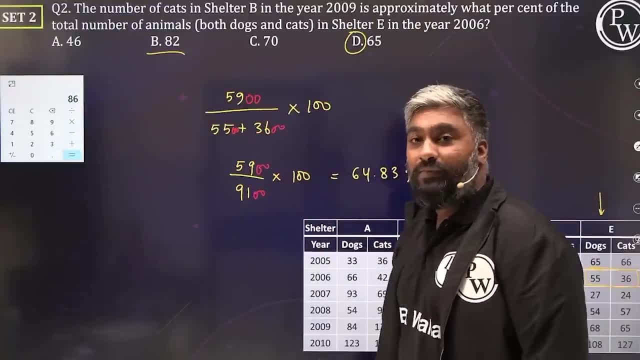 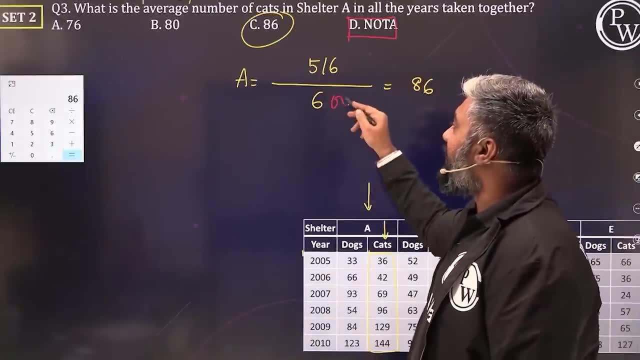 This: 5500.. 3600.. This was in hundreds, So this was getting cancelled out as well. But this cannot happen here. Why? Because there is no 600 in the base. You are adding 600 values. No, You are adding only 6 values. 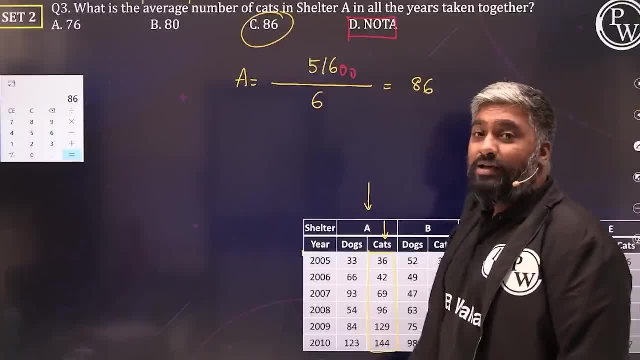 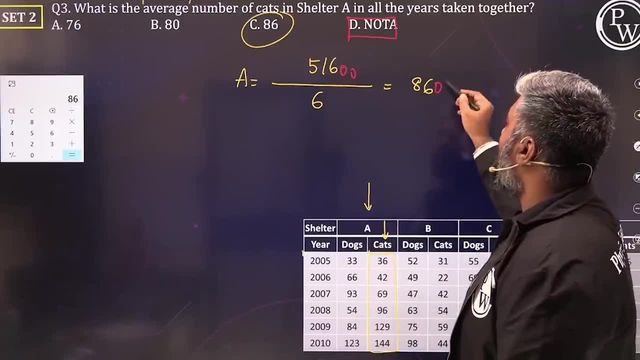 But there are hundreds in your numerator. It is not 516.. The sum is supposed to be what? 51600.. Okay, Please be very careful about it. What will be your average? 8600.. Not 8600, but 8600. 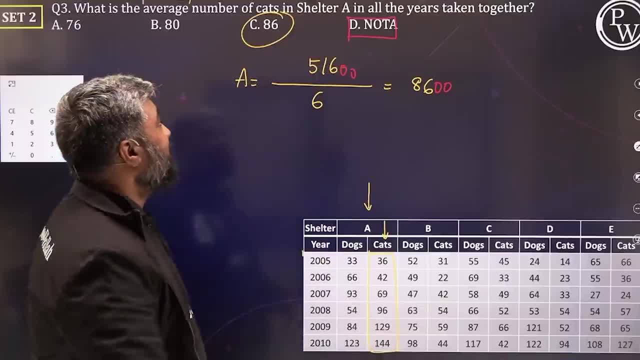 It was a mistake. I anticipated it. I set a trap. Yes, This is a trap. Do you want to fall into the trap? Are you enjoying it, Sir? leave the question. Trap after trap is coming. What is the matter? 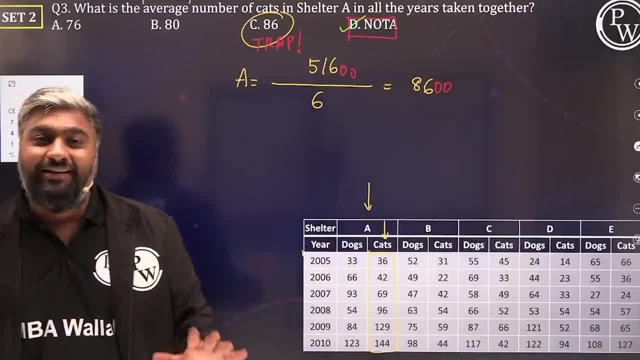 Yes, That is all Cat is all about. Okay, The level of the question will not be so complex, It will not be so unsolvable, But they will play with the psychology like this, Okay, So please be very, very careful. 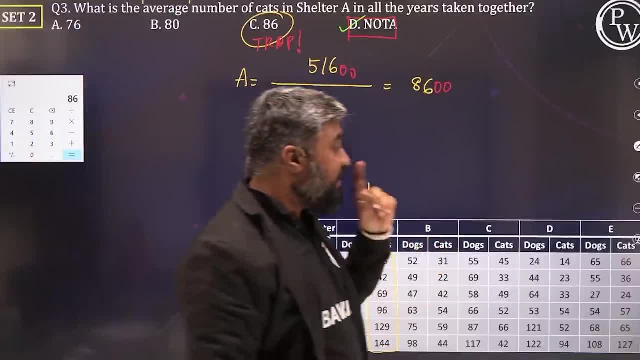 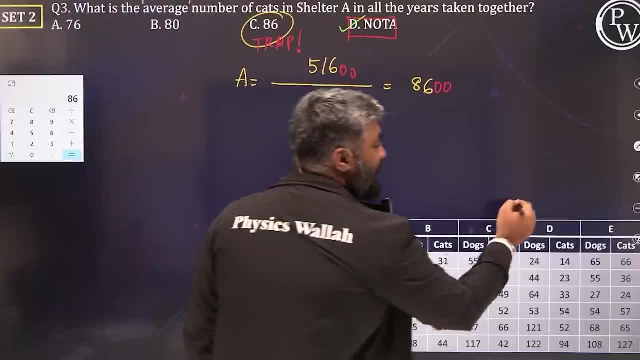 One thing you can do is on the rough sheet. If you will try out your sheet On that, just write into 100.. What does it mean? There is a scale in 100s. This will keep reminding you to use it wherever possible. 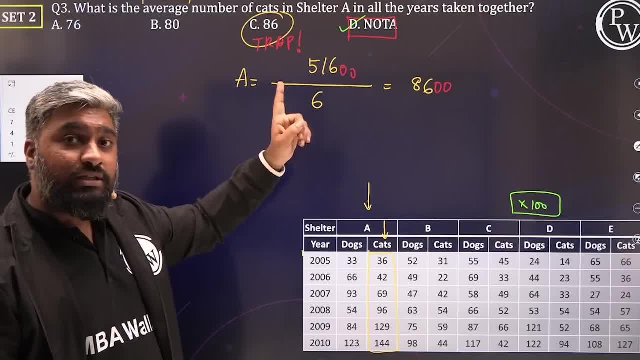 Okay, Let's go Moving on to the next question now, Question number 4.. The ratio is asked: Number of dogs in C in 2009.. C dogs: 2009.. Which is this value: 87. To the number of cats in A. 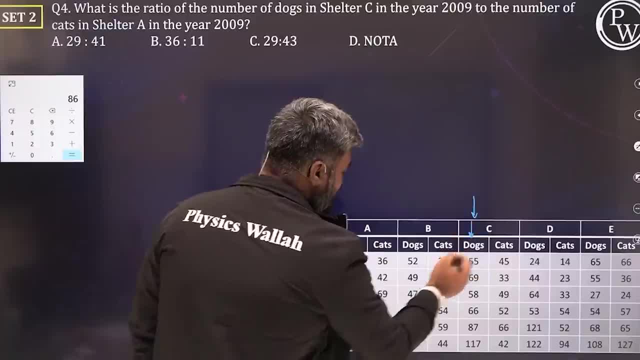 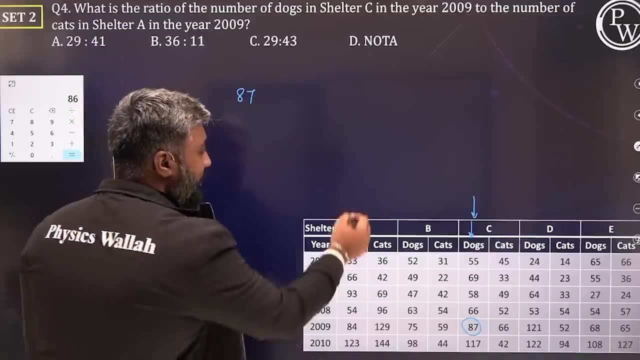 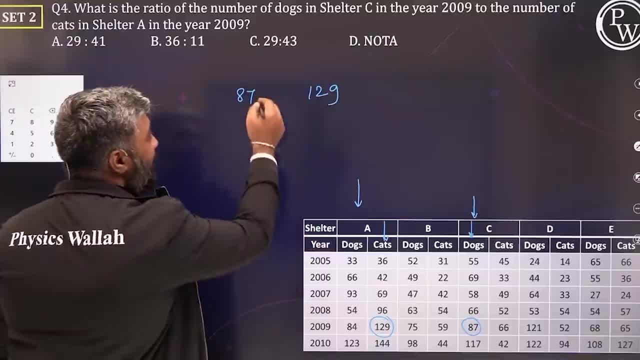 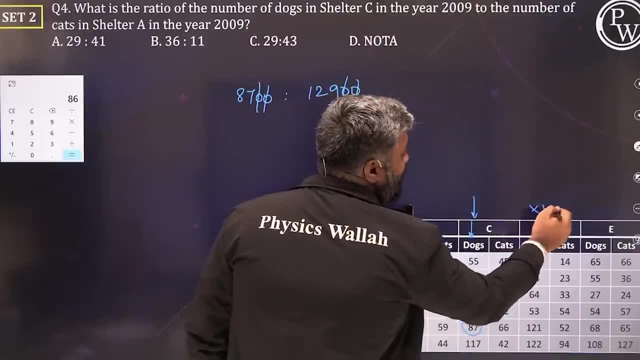 Which here A cats, Which here A cats, Which here: 2009.. 2009.. 2009 number of cats: 1029.. What is here Scale is- But that is cancelled out- 8700.. 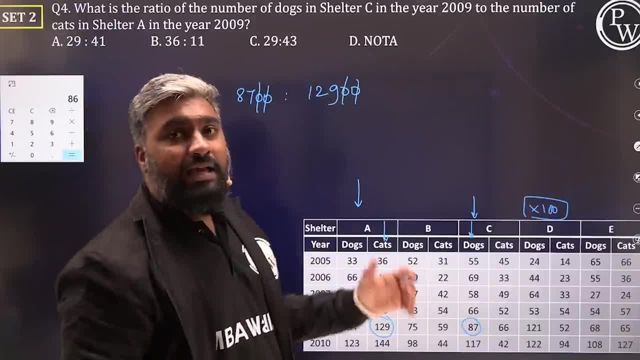 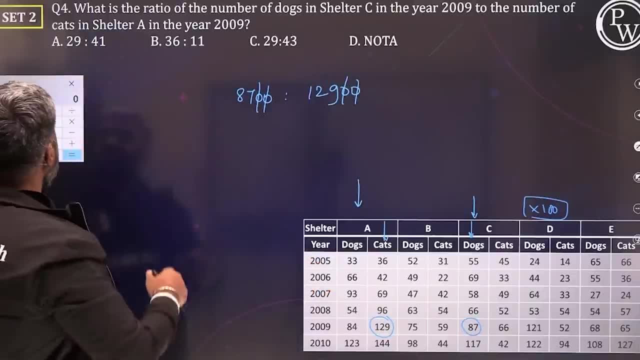 12900.. 2: 0s are cancelled out. scale is X 100.. It's there also, But because the ratio is asked, Both this 200. X 100.. It has been cancelled, Okay. 87.. 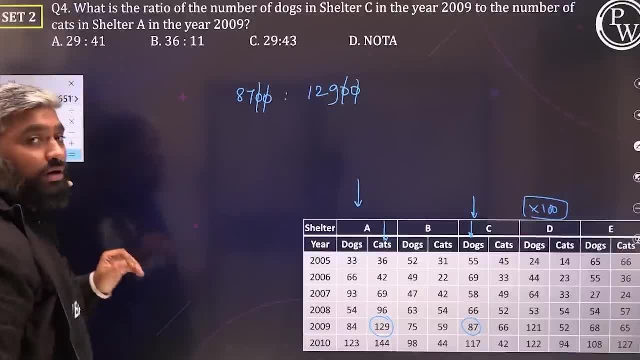 129.. If you want to do that in the calculator, you can do it. You can use the calculator for this. But what will you have to do to ensure that you get the correct answer? See, this value is 0.6744. then you will have to compare with all the answer choices. that where is? 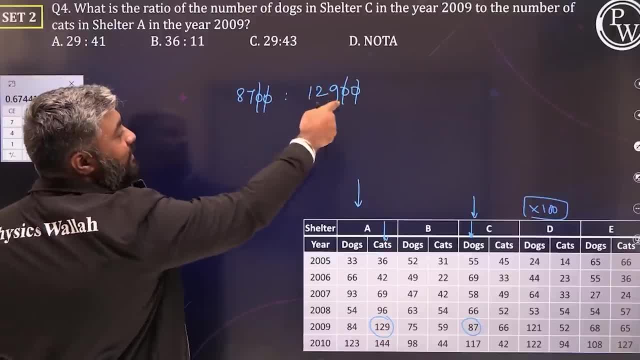 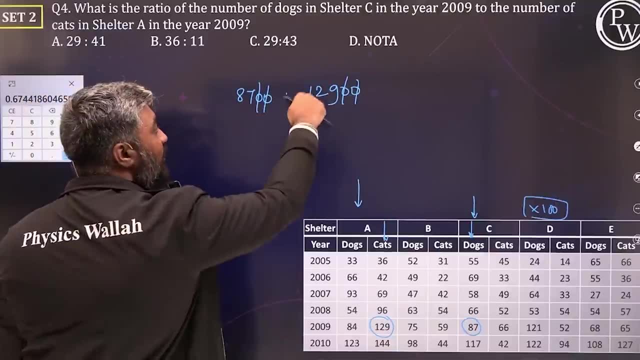 it coming. instead, look at what's common: 1, 2 and 9 thumbs up to so it's not even 7, and 9 is not even the next number. you try it out with this: 3, 8 plus 7, 15 divisible by 3, 1 plus. 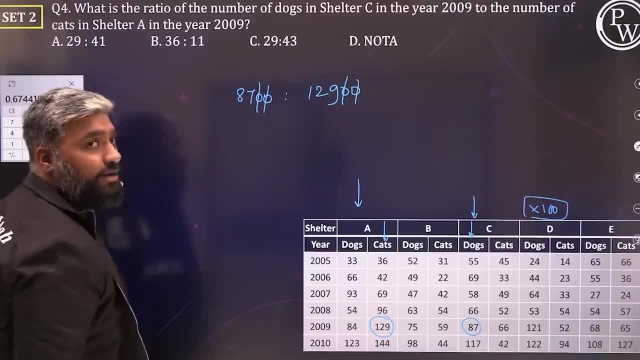 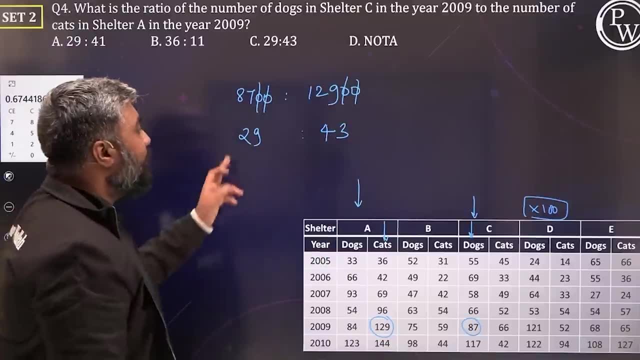 2 plus 9, 12, divisible by 3. so it will be divisible by 3, divide by 3. yes, this is going to be what: 20 and 27, 9, 29, this is 43. above this, 29, we know, is prime number. so to divide this further, 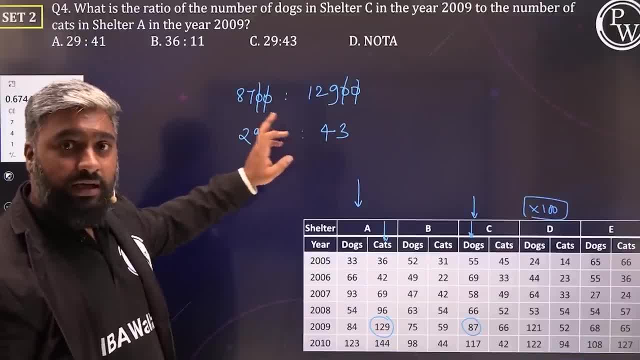 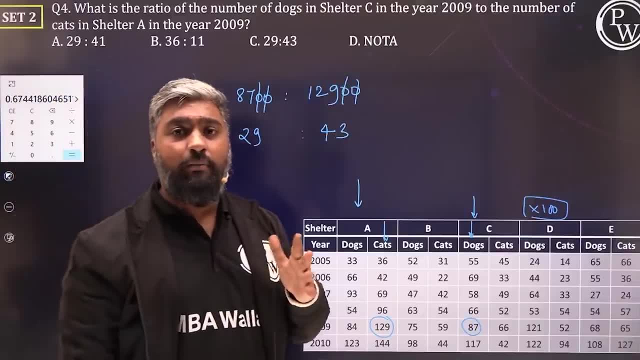 either this should be someone's factor or this should be someone's factor, you know. next multiple of 29 will be 58. this is not. it means 43 and 29 are co-primes. there is no common factor in both of them. 1 is the only common factor here. so 29 is to 43 is your final. 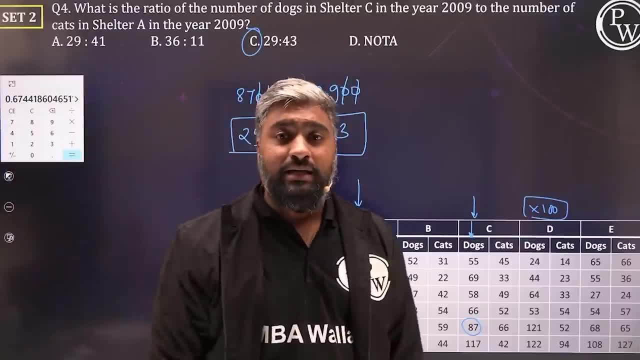 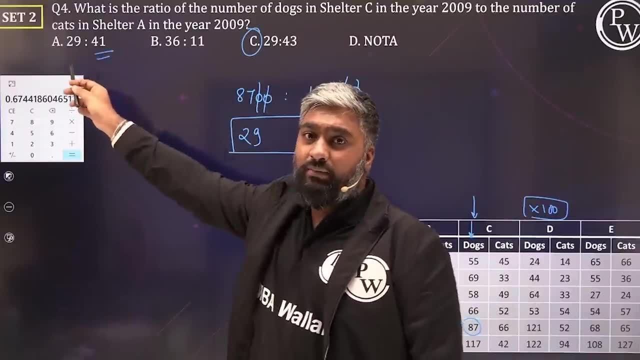 answer, which is what option C, 29 is to 43 is your answer here. only you have to divide this. allora you glossed on 29. 29 is to 41, rushed. if you choose 29,. quickly select it, don't be in a rush. ok, so 4 questions done. moving on to the last question of the set, 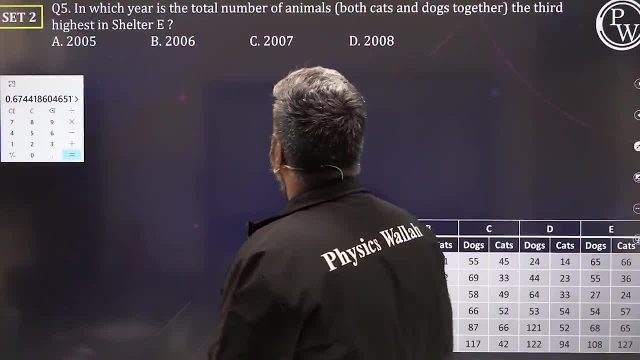 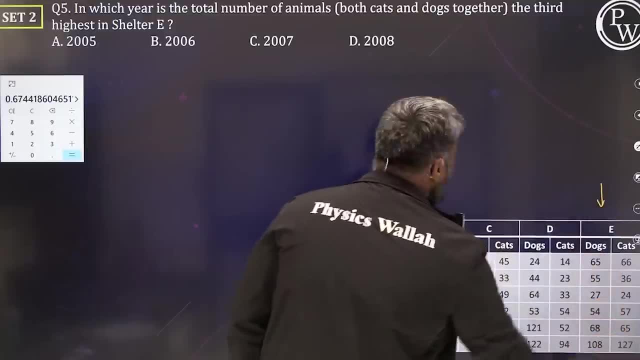 let's do this. in which year is the total number of animals, which is cats and dogs? we have to add, for which shelter investors will say: in the situation of this, shall we add two of them? we will add, and then we need to say which is the third highest of highest. 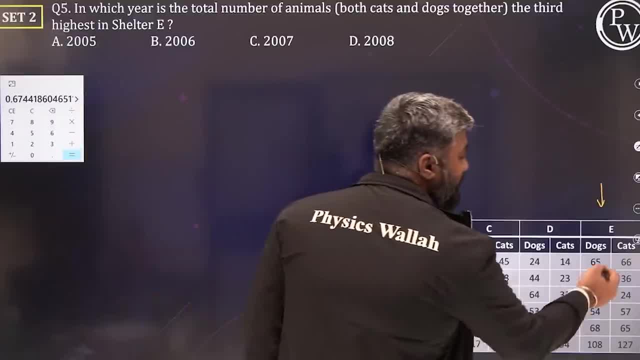 second highest or third highest. we have to deal with third rank. just let's quickly get on with this first threeär. we need to see which is eye to eye and we need to discuss which one will vậy we move forward, or which one will become unlimited. so let's quickly find out which one is. 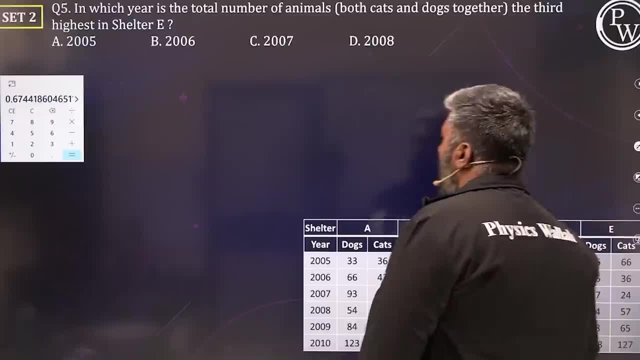 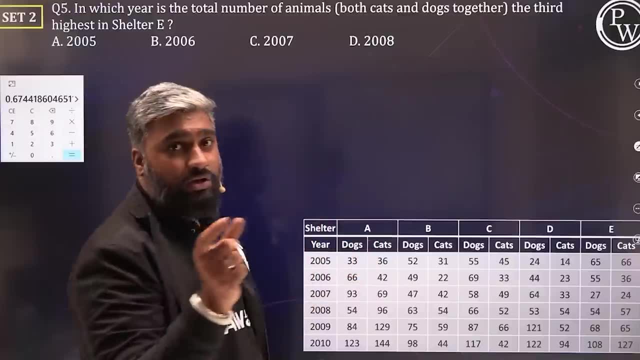 add karna. add karna ke liye bhi. sorry. we're done with four questions. let's quickly move on to the last question of the set. in which year is the total number of animals, both cats and dogs, to add karna hai okay, the third highest in shelter e to shelter e ke values chahiye and we need to do. 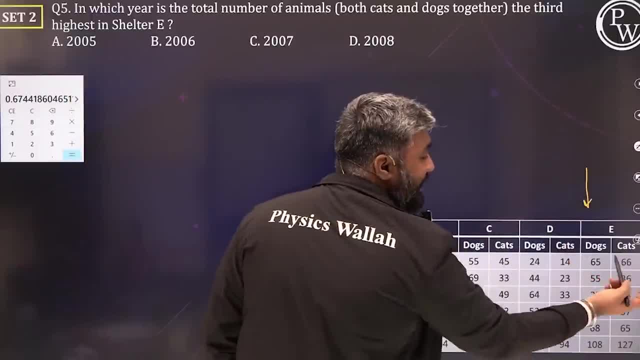 what add them sum. dekhe karna hai, right 65, 66 ko add karna hai, 55, 36 in sab ko add karna hai and then compare right. so ye addition ko liye. agar aap calculator use karna to aapke marzi ye manually. 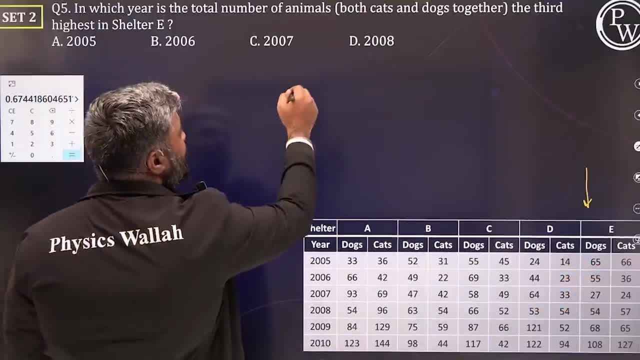 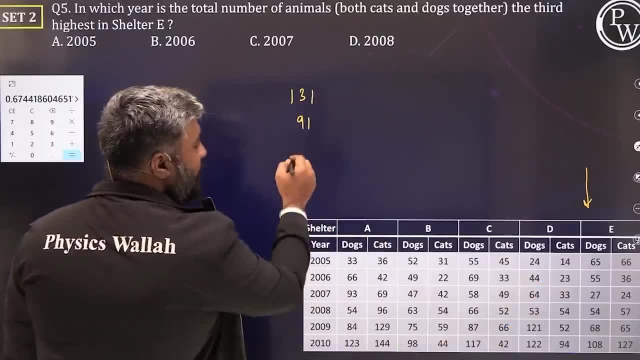 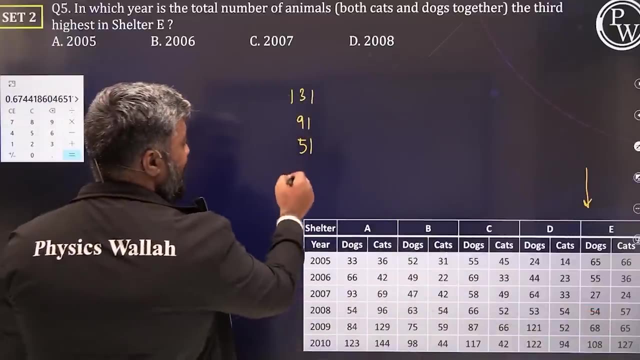 phat, phat se ho jayega. okay, so this is what: 131, yes, next you have 55 and 36, 91, next you have 27 and 24, 51, sab 1, 1 pe. aar. yeah, next uh, 54 and 57. this is 111, ye, bhi 1 pe hai chalo change ho gaya. 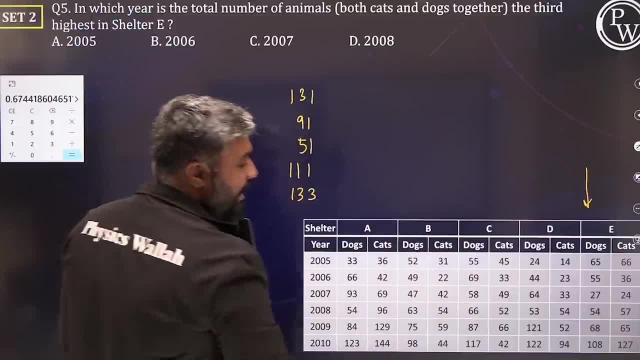 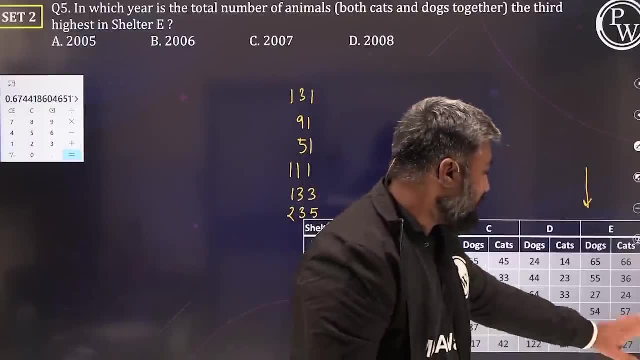 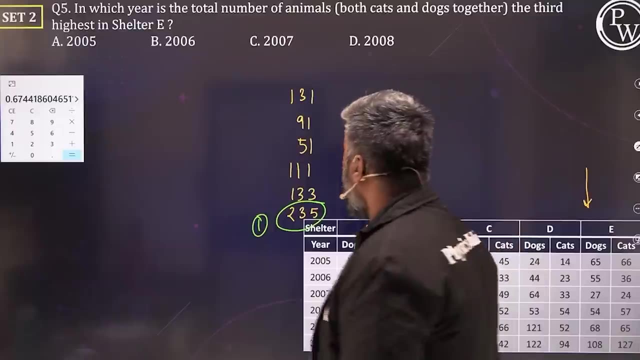 68 and 65, 133 and 108 and 127 is 235. yes you, 235 chalo ye mil gaya hume sum ab hume kya karna hai? we need to find the third highest sabte bada to ye hai. first highest done iske baad. the second highest is 133 done. third highest is. 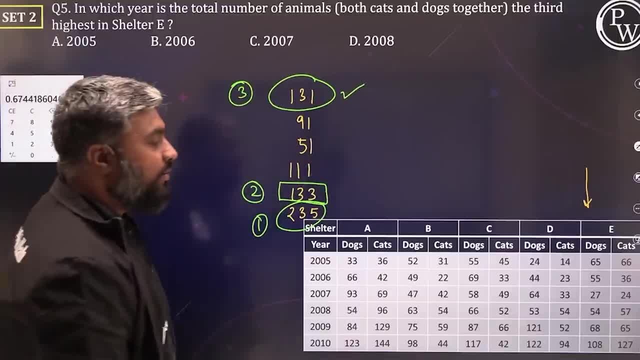 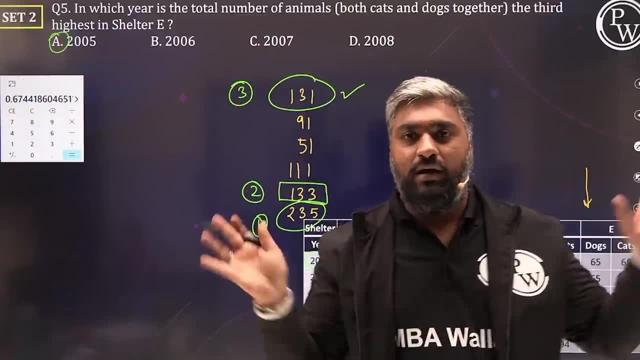 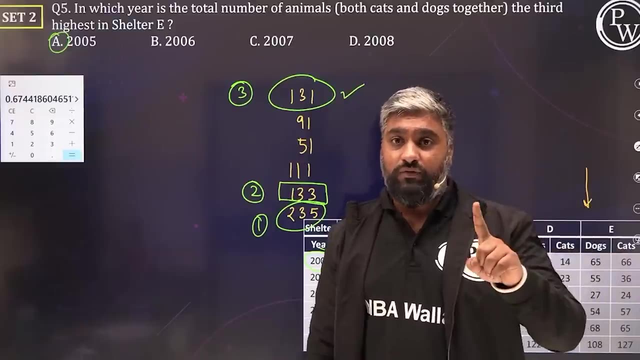 131. this is going to be our answer. 131 was in which year was in the first year, 2005, 2005. hai answer choice. list me: yes, option a done. that's it right. so this set was doable. kaafi saare traps le kiye gaye the right. you have to be very careful to watch out for. 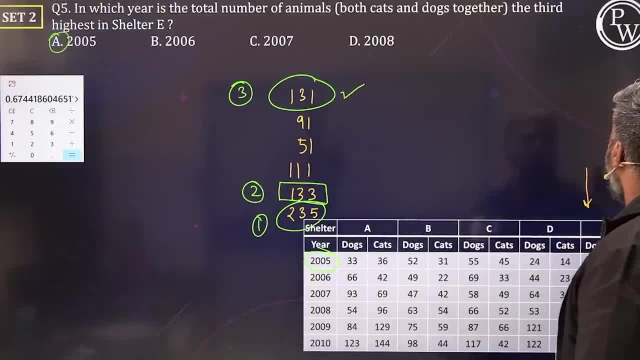 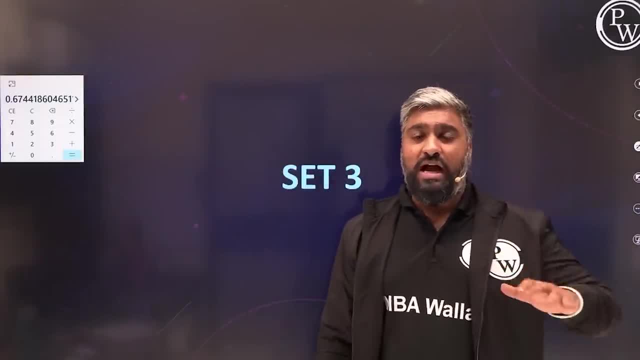 these. take a, don't miss out on these. yes, there are two sets done. let's move on to the third set, the final set. i think we are. we are doing great. our progress is uh at par uh with most cat people, people who are preparing for cat, cat aspirants, jo prepare kar rahe to apna level. 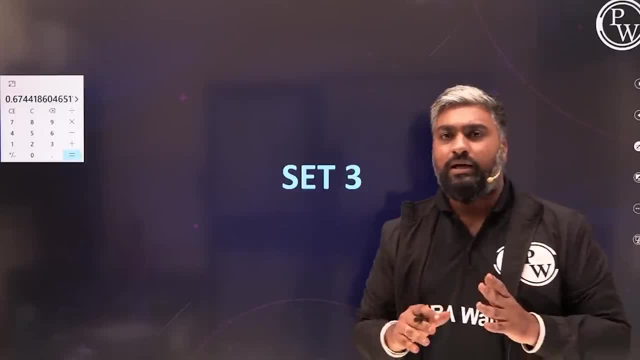 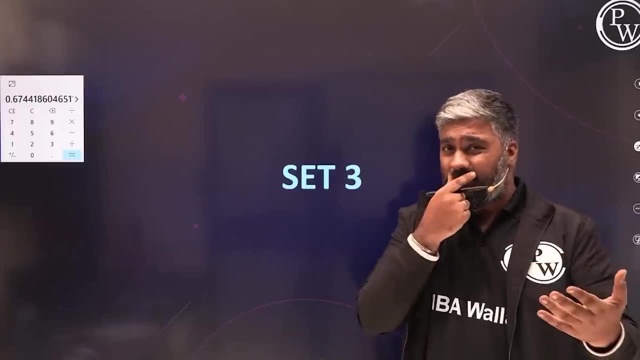 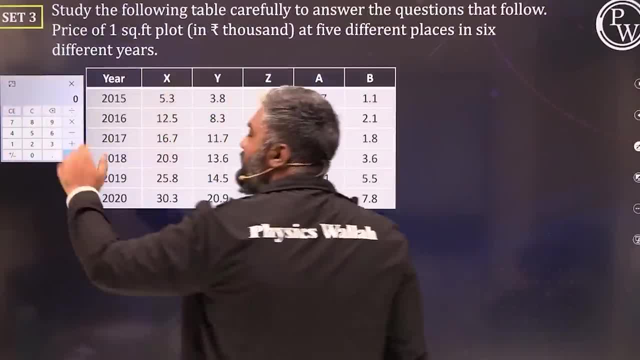 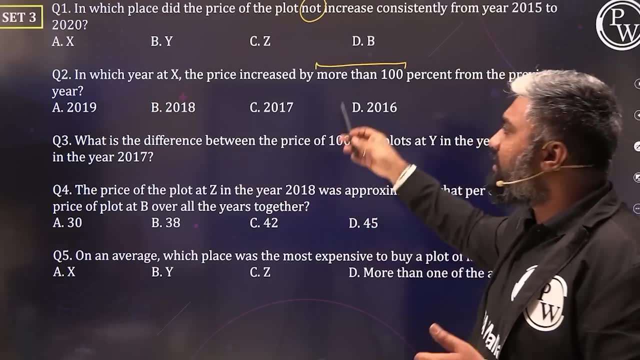 out. uh fatah patse calculator ko clear karna. mat bhoolna, kabhi kabhi iss main mistake kar dete hain. dekhhh. okay doh, let's get started. uh question. kya study the table carefully, answer the questions. we'll talk about that. what is the difference? so yeh second wala. 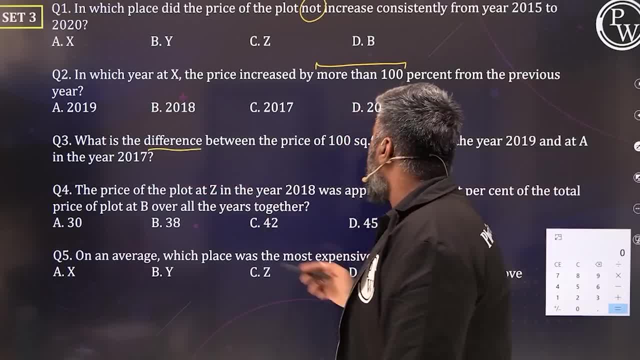 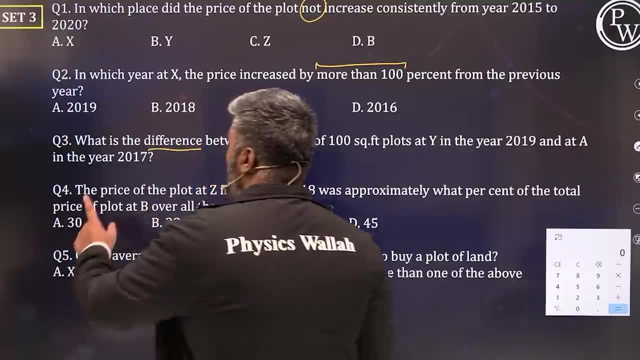 bhi hoye sakta hai. third: wala difference between the price difference poochya hai do values ka difference poochya hai. we can get that from the table easily done. fourth: price of the plot at z in the year い 18, was what percentage of the total price of plot b over? 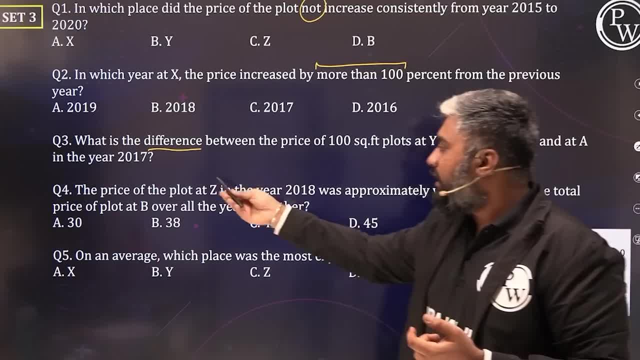 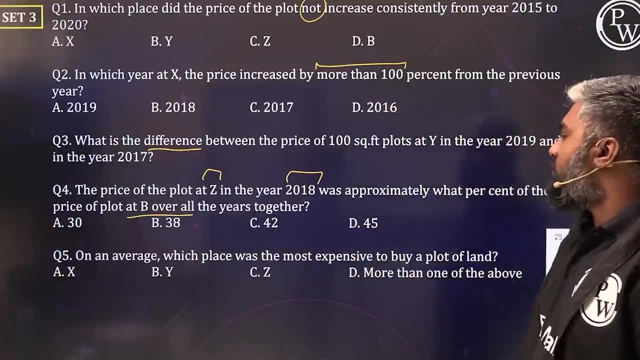 the years. percentage comparison hai. yes, one value needs to be compared: outro whaoe. toh the total Addition bhi karna, division bhi karna. Fifth on an average, which place was the most expensive to buy a plot? Second, one is also analyze, Yes, data chart. dikhne mein khatarnak. 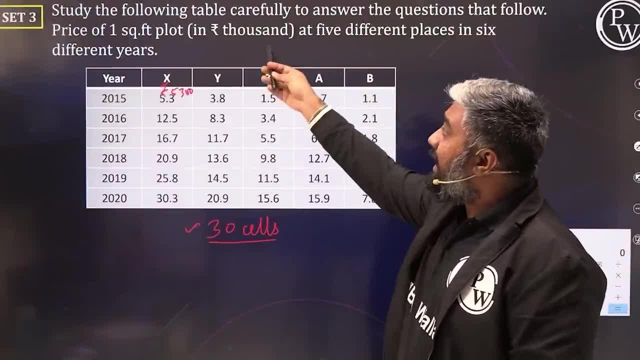 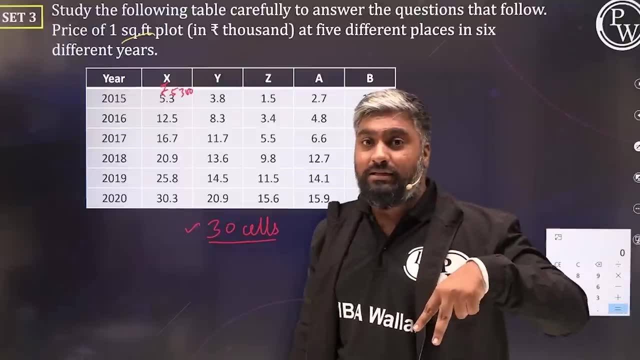 dikh sakta hai, Sir, decimal hai fractions hai scale hai units hai kuch one square feet bhi de raka hai. All this is given, But what can you do? There are two answers jo aap dekhe answer. 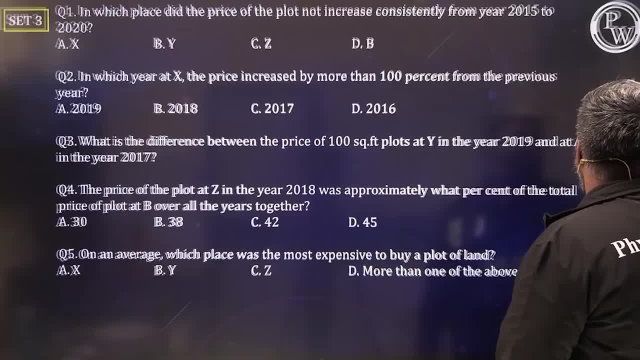 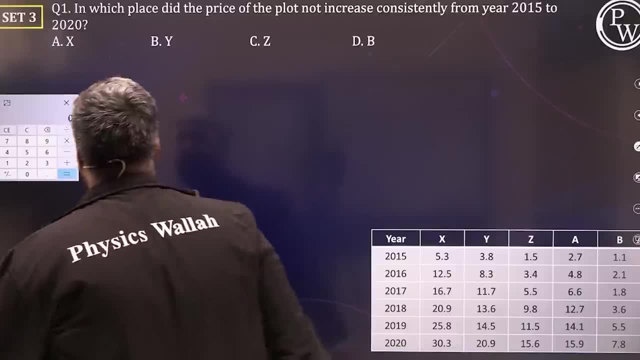 kar sakto. Those are the ones that you should start with. Chalo hum normal flow mein jayenge. Let's get this started with. Here's the first question: Calculator. bhai saab ko uthayenge Yeh kubche mein layenge. Let's do this. In which place did the price of the plot? 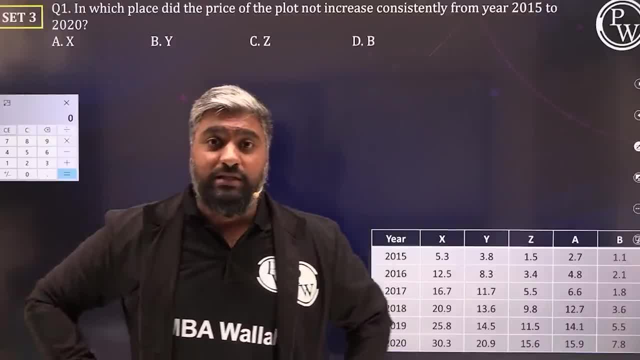 Acha, yeh, I understand positivity, that people have optimism. Sir, hum aise positive dikhta hai, negative nahi dekhna hai. Yeh galti aapne question mein nahi karne hai, Thikhe Not. 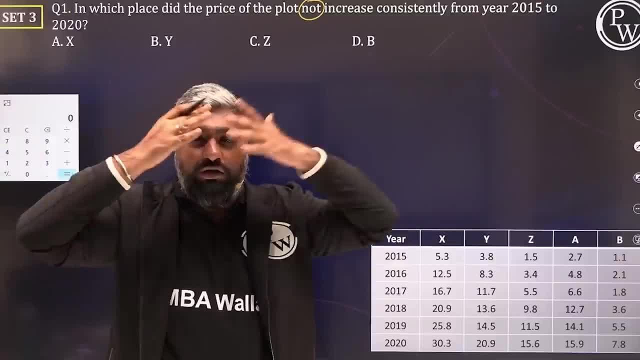 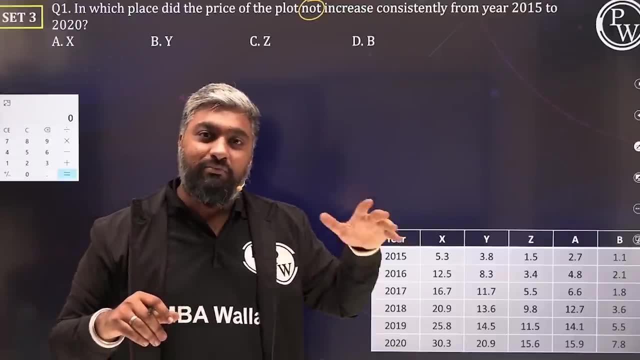 dikha, Not dikha aur usse chhor diya. Sir, negative cheeje chahiye, Toxicity se door bhaag rahe hai. Please keep in mind to read the question carefully. Question mein: yeh judgment mat karo. Do it in people, do it in places, not in questions. Thikhe So in. 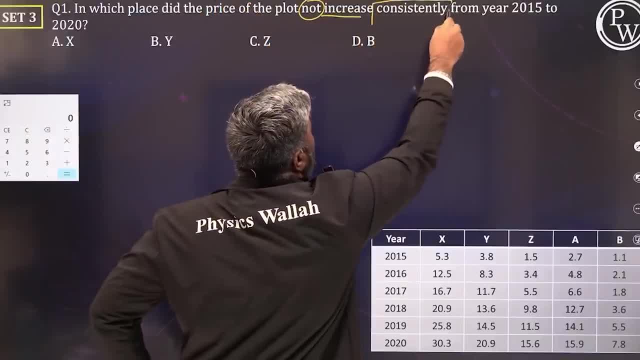 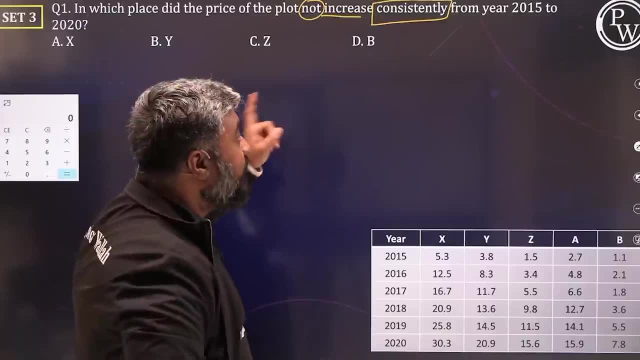 which place did the price of the plot not increase consistently, Matlab kya From 2015.. Every year increase hona chahiye? Yes. Agar nahi hua, increase consistently, woh poocha hai 15 to 2020 ke beech mein? Yes, Char options hai: X, Y, Z aur B. A ko dekhna hi. 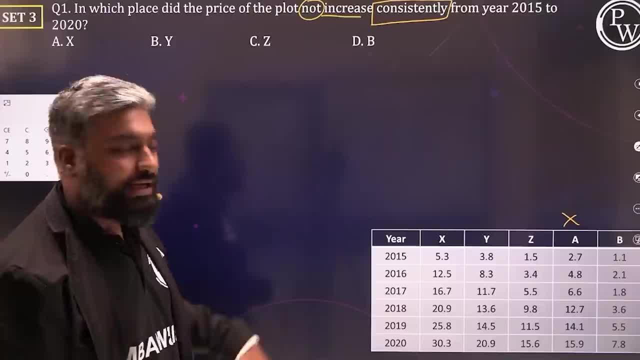 nahi hai Time waste mat karna. Don't look at A, Don't waste your time. Kyunki A options hai nahi hai. Thikhe Chalo X ka dekhenge. 15 to 16: increase, Yes, Increase, Yehaha. 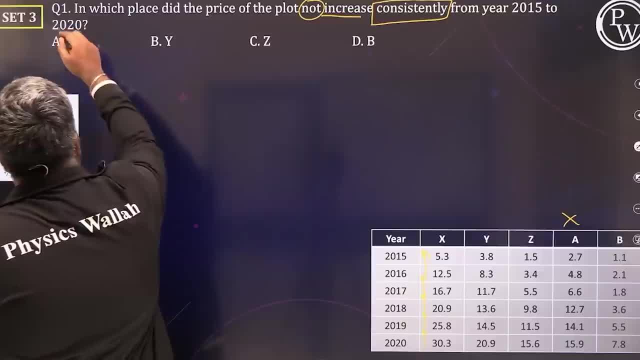 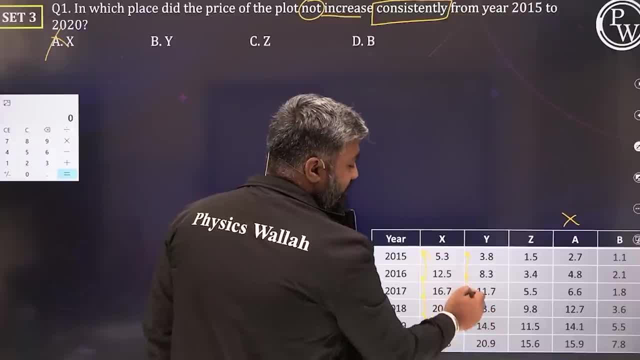 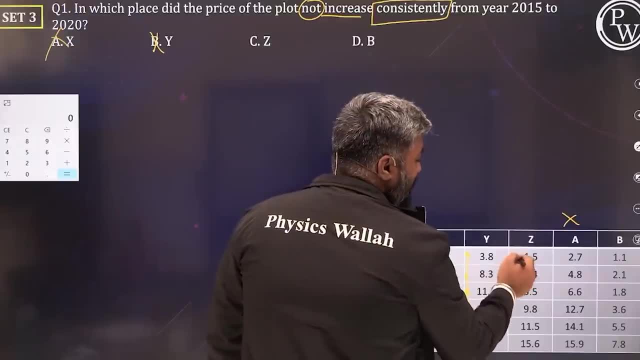 3.8 to 8.3, increase. Yehaha pe bhi. 8.3 to 11.7, increase. Badh raha hai, Badh nahi hai, Badhte hi jaara hai. Yes, Y is also out. Eliminate Z, dekhenge 1.5 to 3.4.. Increase. 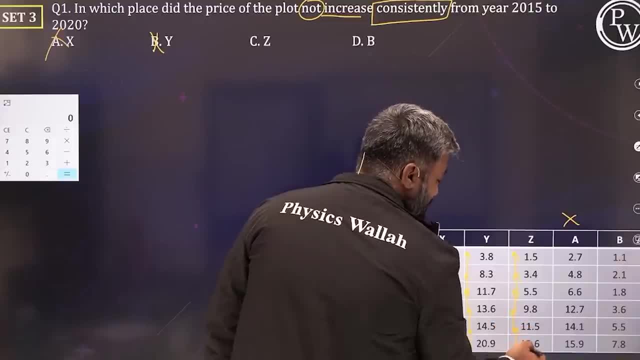 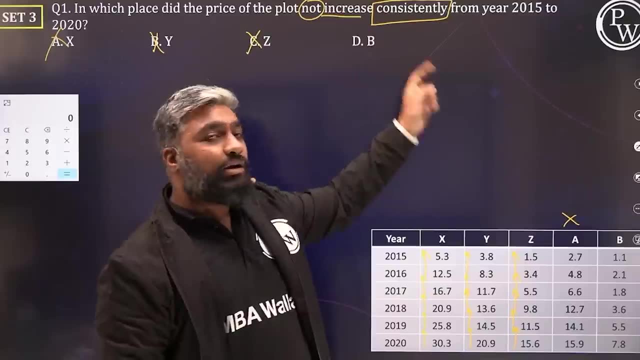 increase, increase, increase, increase, increase Z. main bhi badhe hi jaara hai Abhi 2 cheez ho shakta hai. At this stage, 2 things could happen. One: we can blindly select option B, Place B and B입ne in here. it would increase yuh jaata hai Price up to 200,000. 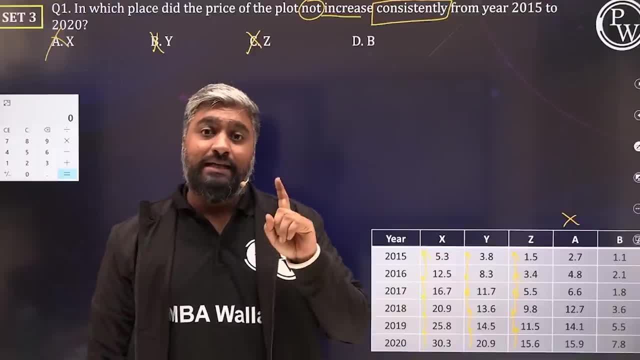 That is that of 5,000.. So if i take Y till Dec i might increase that Aam 72%. Here move out of the question, but but ye bhi ho sakta hai ke aapne question padhne mein kuch. 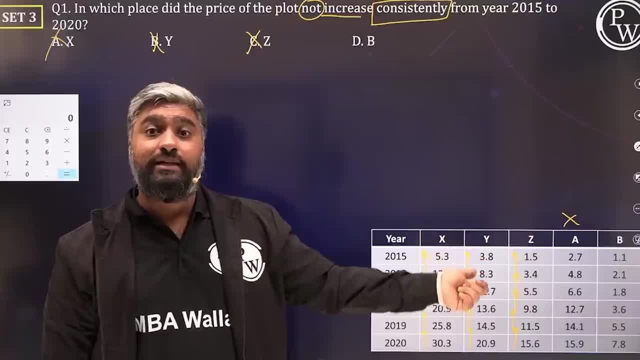 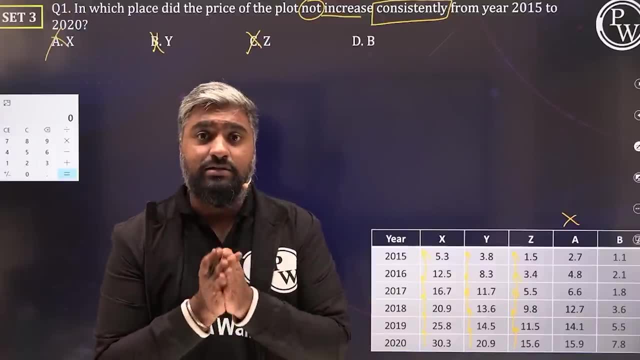 galti kar di, or you are, you've not understood the question carefully or you're not solving it in the right way. right, so, to avoid any such mishap is a mishap, kyaate mishap? right, to avoid any such accidents to occur, what should you do? check kar lo right, kar lo it. 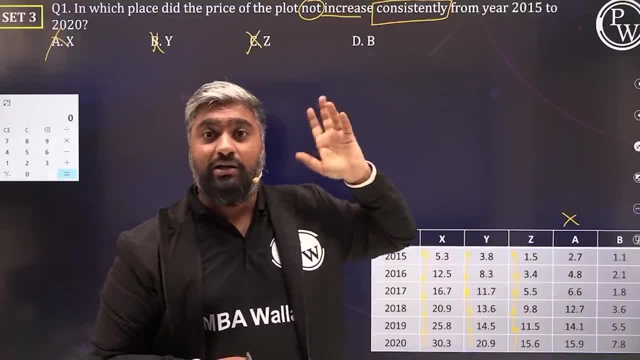 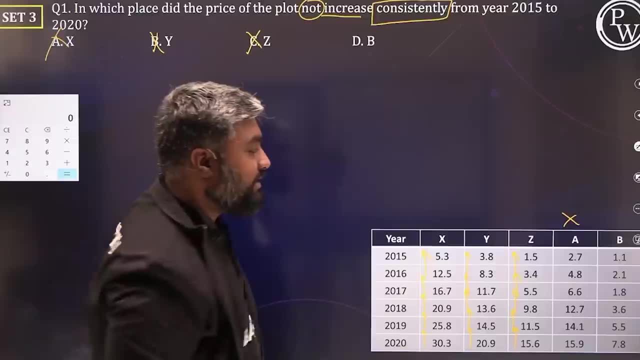 will take what? another 10 extra seconds. we can use the amount of time that we've saved in the calculation. all that here, right? so let's check for b. let's see if b is one of those places where the prices are not increasing consistently. one point one to two point one. 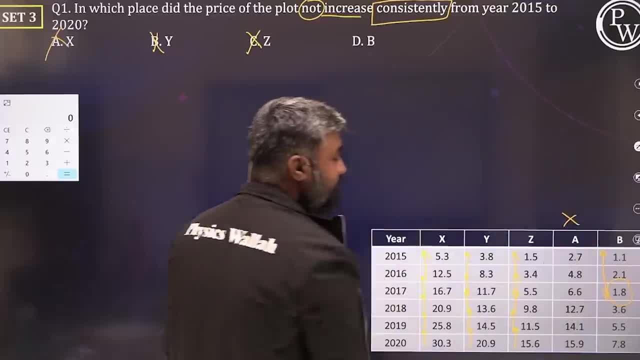 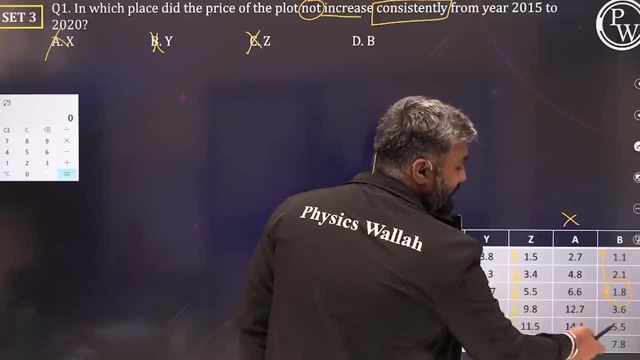 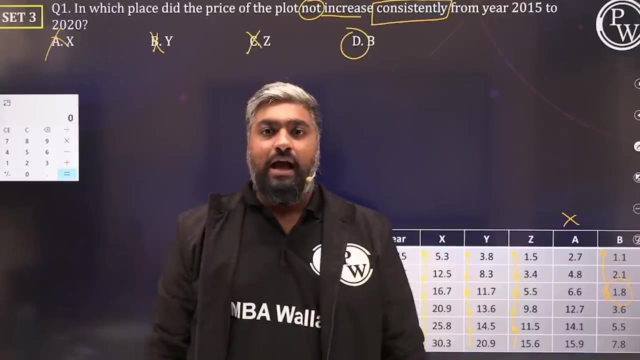 increase two point one to one point eight decrease. so for b in 2017, instead of increasing, the price has dropped. then again, three point six increase. five point five increase. seven point eight increase increase. everywhere else except for that place, b is right. whatever we've been doing is correct. yeah, i hope you understood what we just did. right now, aapne. 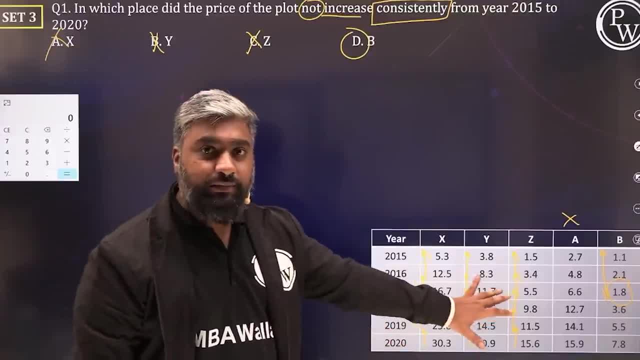 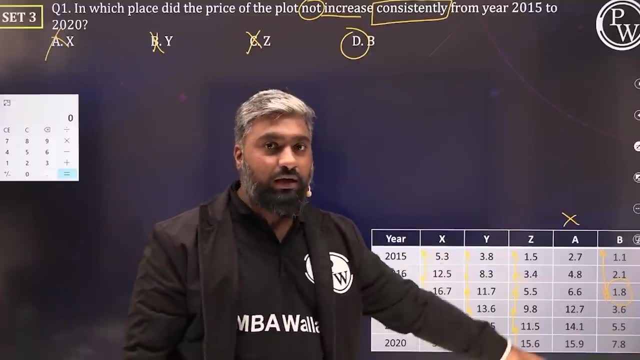 aapko samaj mein aaya. what we just did? what did we do? looked at the data, eliminated the answer choices as we went along, but when we were left with one, we did not blindly select that and move out. yet we checked for it why we are humans. humans end up making mistakes. 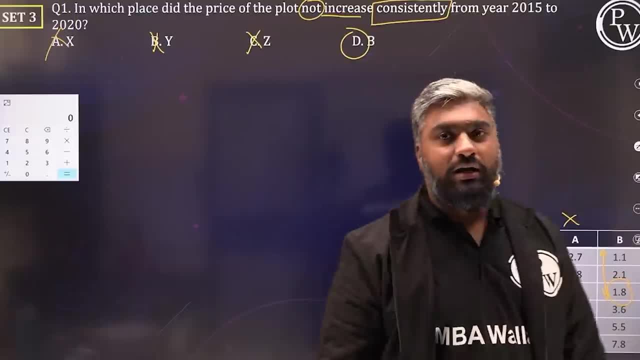 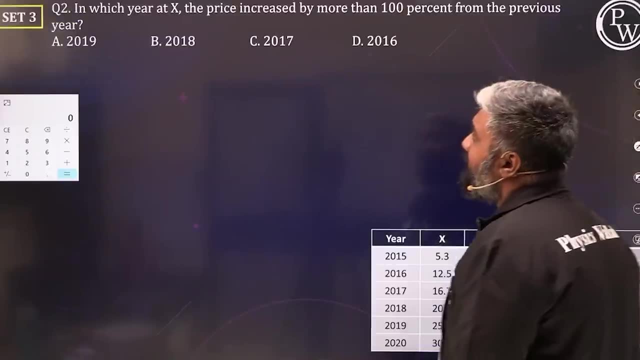 yes, and we don't want to be one of those guys. okay, so in this question we did not have to use a pen and a paper. we did not have to use calculator, bhai saab, either. yes, we're good to go. so question number two: let's get this started. in which year? at x? we don't want any. 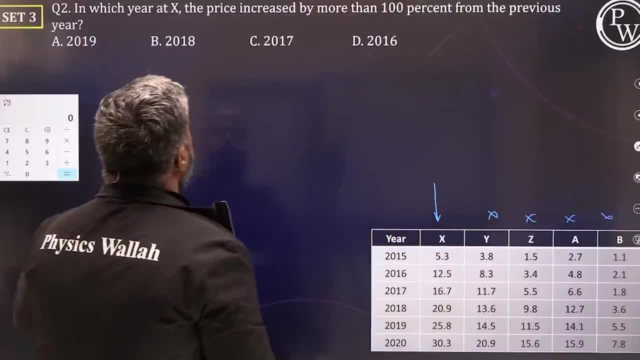 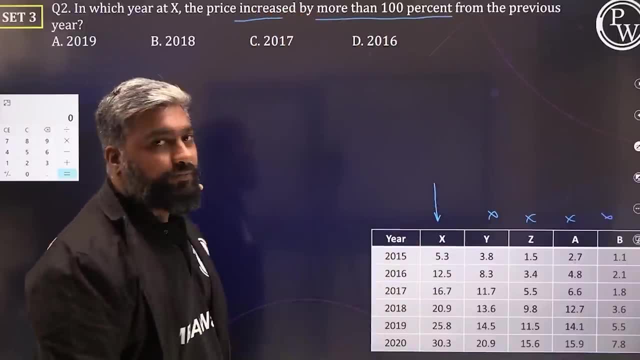 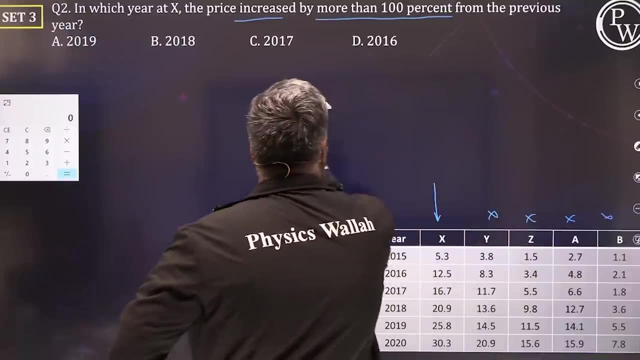 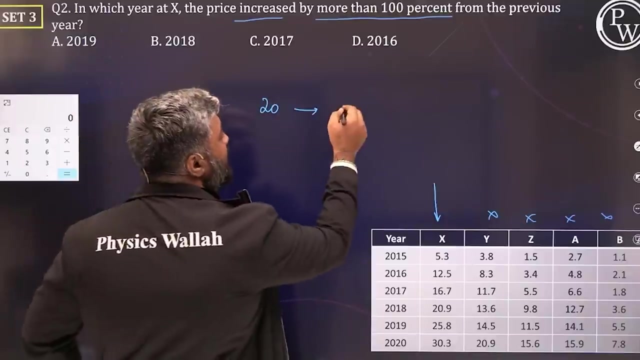 of these values- we only care about x here- the price increased by more than hundred thousand, hundred percent, increased by more than hundred percent from the previous year. yeah, let's take a small example. let's say here: the value is hundred, hundred, hundred, hundred. easy example let's take. let's take twenty. initial value is twenty twenty. say value, say twenty four. 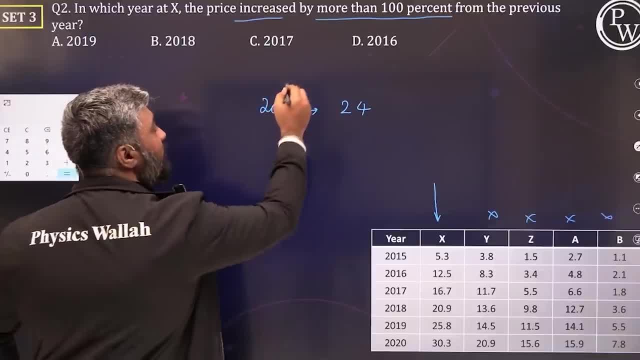 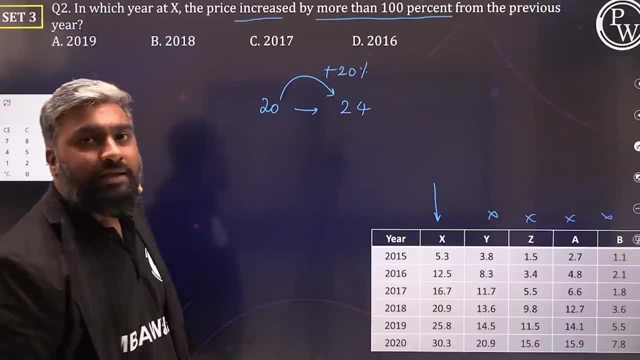 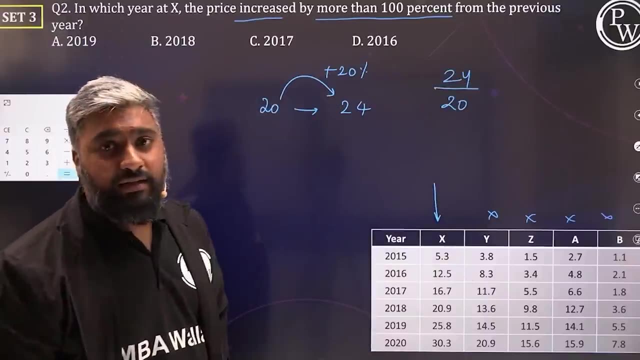 ho gaya. itna increase ho ga in terms of percentage. what is the increase from here to here? itna increase ho ga anybody? twenty percent, beautiful. so there is a twenty percent increase. how do that? how do you see that? simple, just divide the new value by the old value. when you divide the 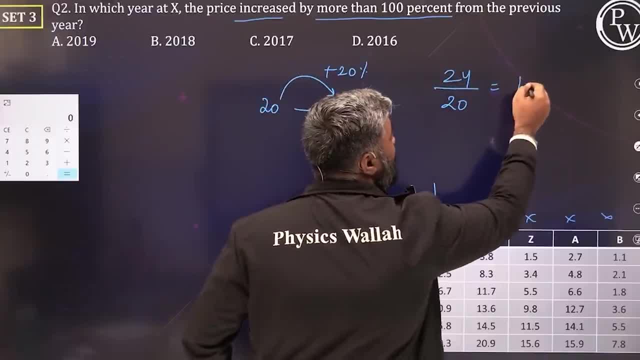 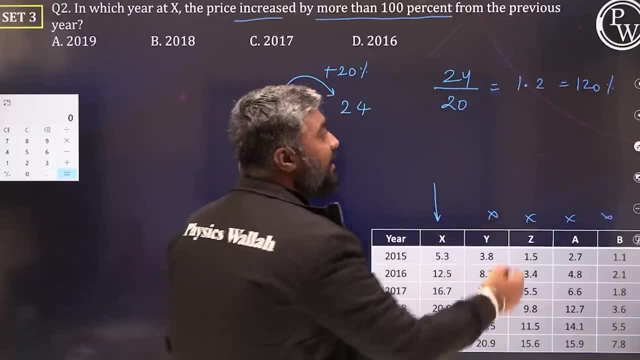 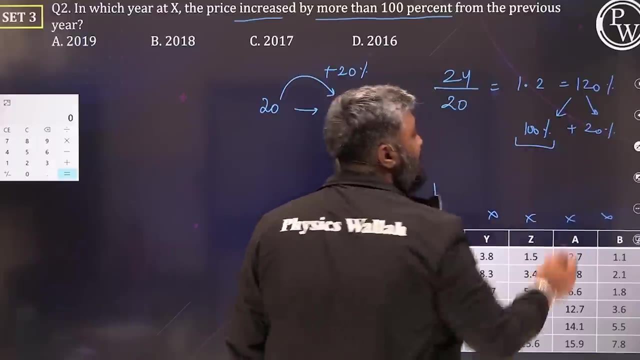 new value by the old value, 24 by 20 is 12 by 10, which is 1.2. yeah, this 1.2 is nothing but 120 percent, am i right? hundred and twenty percent split up here hundred percent, or, yeah, twenty percent, am i right? so hundred percent was the existing value, hundred percent was this this. 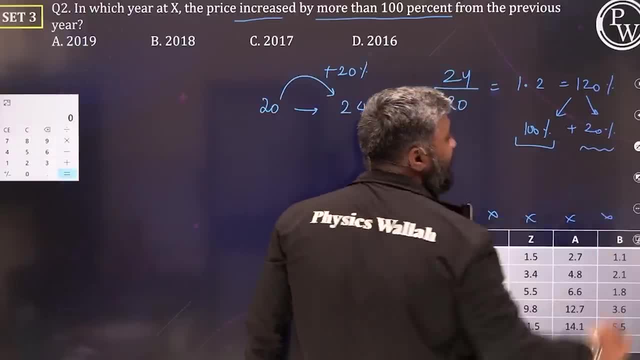 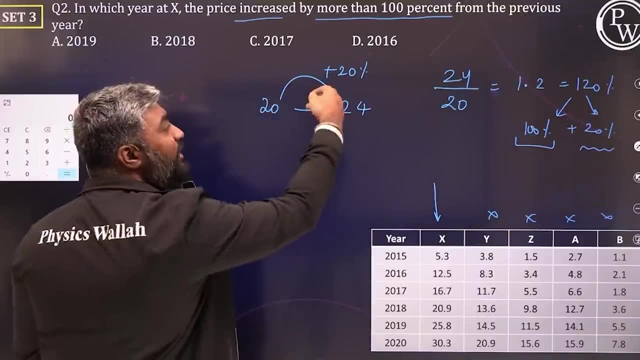 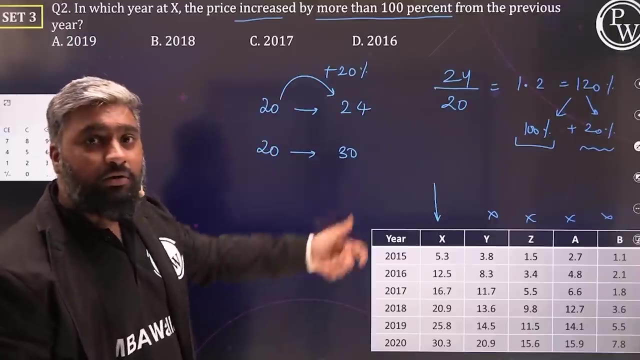 20, this existing value. how much did we increase? we increased it by 20 percentage. that's all correct. we increased it by 20 percent. so here are the increases. how much 20 percentage? yeah, can you quickly guess this? 20 to 30. how much is the increase? 20 to 30? how do you check? 30. 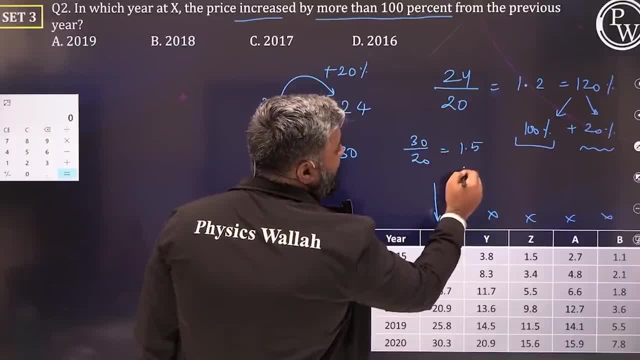 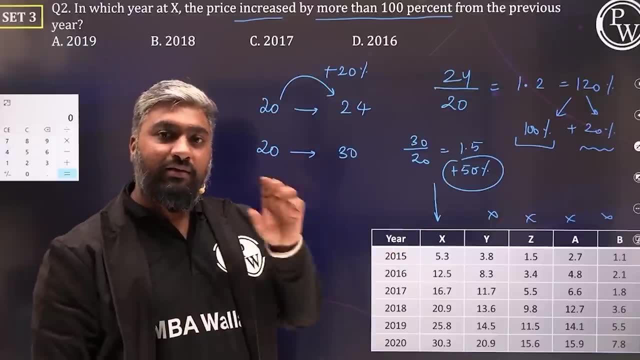 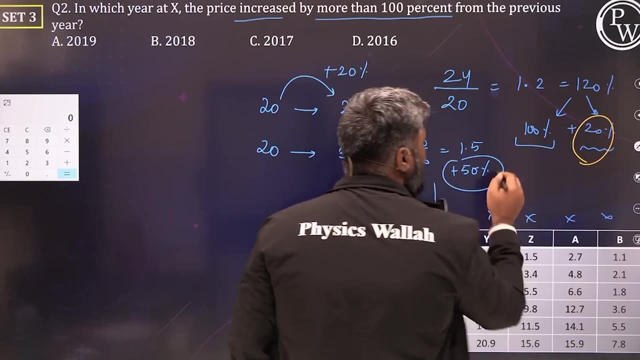 divided by 20. if you do, you will get 1.5, which means there was a 50 increase. am i right? 1.5 is 100 plus 50: 150 percentage is 100 plus 50- 50 increase. yeah, so if the question is asking more than 100 percentage, increase this part, this, this part? 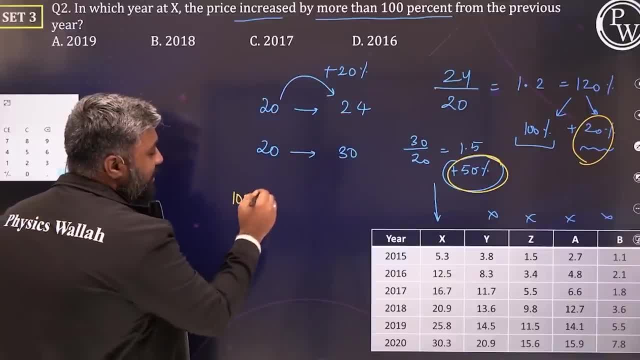 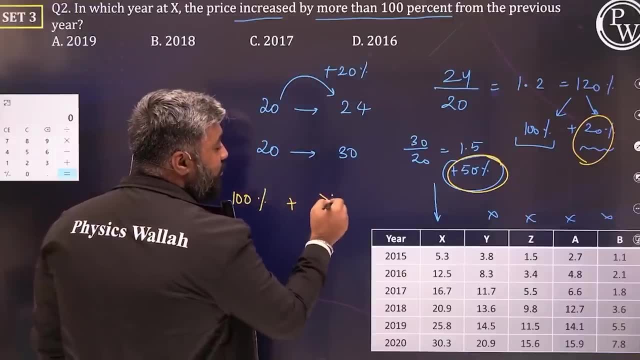 this part should be more than 100. that means already existing. there is 100 percentage palletage value. the old value, 100 percentage, is there. on this, we need the increase part to be more than 100 percent, correct if you were to add 100 percentage with something more than 100 percentage. 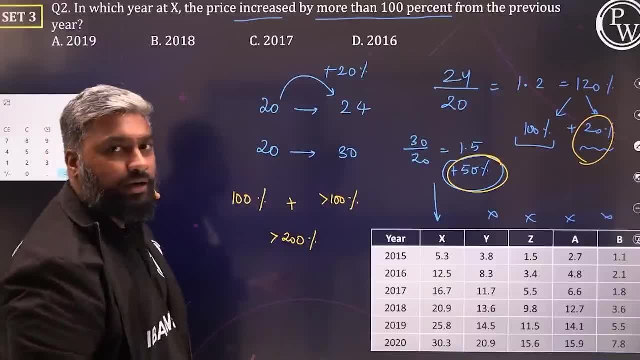 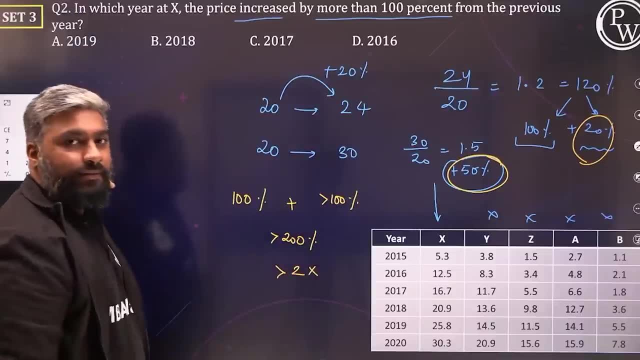 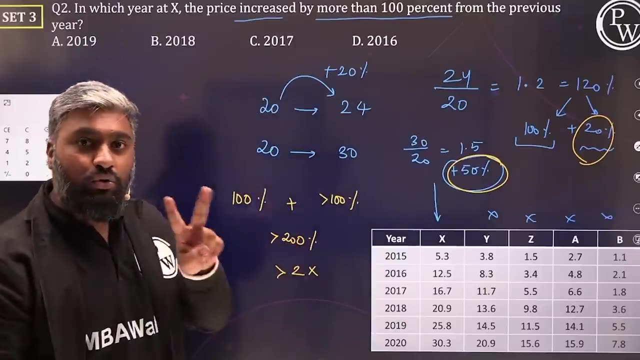 it will become what? more than 200? whatever, 100 plus 100 is 200, but this is more than 100. so more do you mean by more than 200 percentage, more than two times agreed? 100 percentage is once 120 percentage is 1.2. so 200 percentage is going to be what? two? we don't want it to be double, we want. 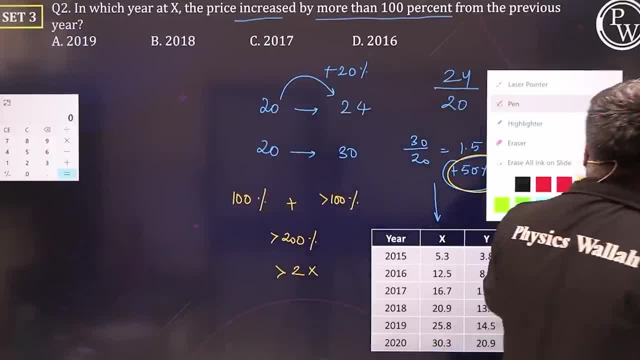 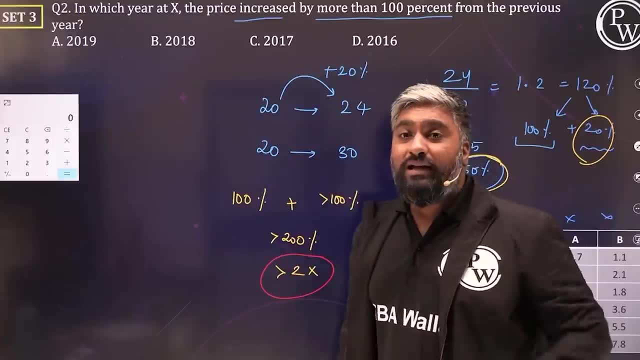 it to be more than double. so all that you have to look out for in this question- this is also kind of analyze and answer question, only why? because all you have to look out for is: when was the value? when did the value doubled itself? yes, let's go by the answer choices: 2019. so if they say 2019, you 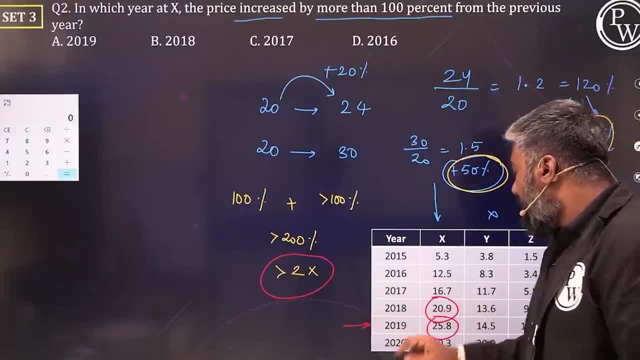 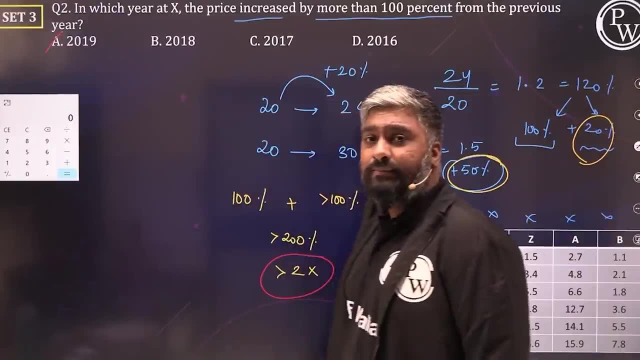 are it with the previous value, 20.9 double? is it 25.8, 20, 40. this is 25. no, 2019 ruled out rs yes, 2018. so for 2018, what are we going to do? we're going to compare these two values previous year. 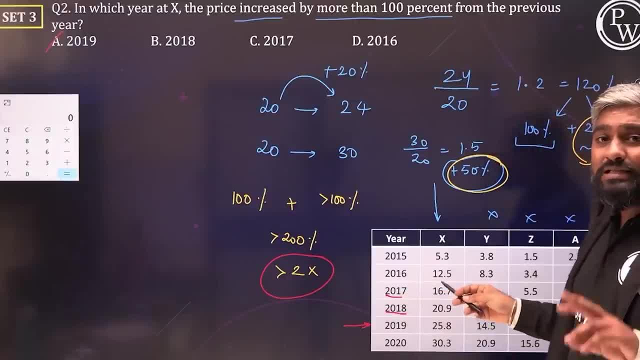 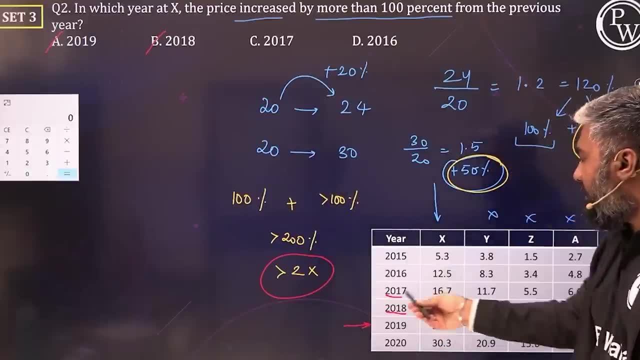 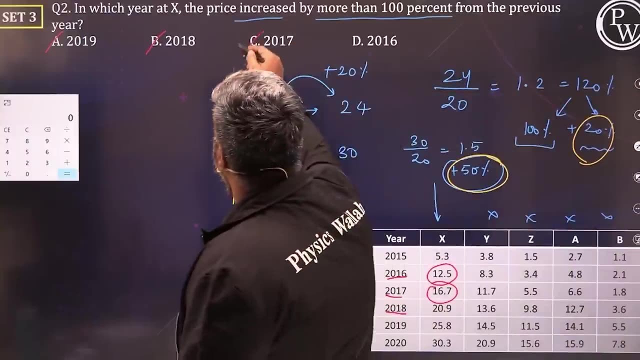 say, compare 17 and 18.. 17 is 16.7 double 32 and above. this is only 20. no, 18 may be increased double 2017.. 16- 12.5 double is 25. this is only 16.7. not working out either. so if whatever we are doing is right, 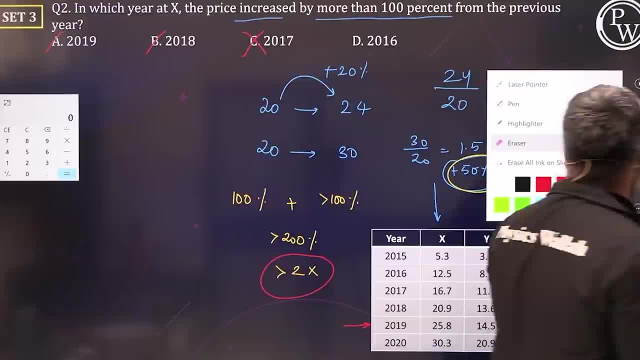 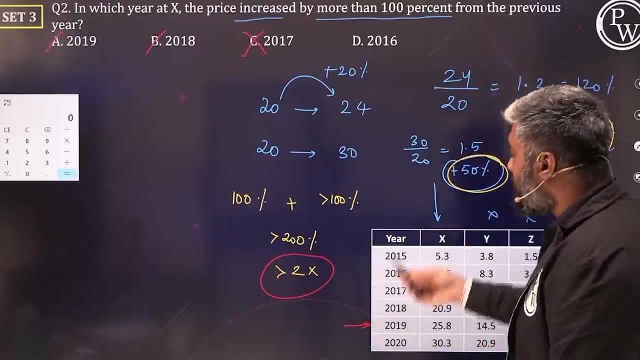 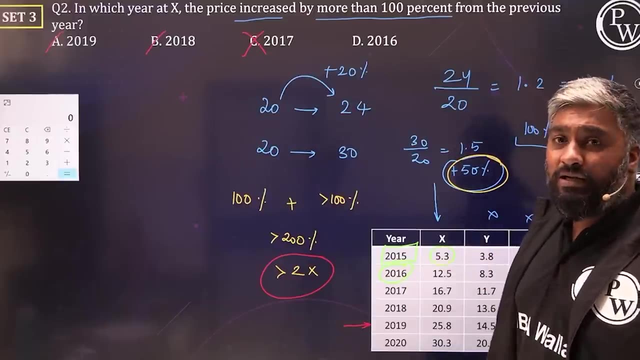 if whatever we are doing is right, our answer should be d, 2016. but how do you confirm on that? are you going to blindly select? now you're going to try and check. so for 2016, for 2016, you'll compare it with 2015: value 5.3. double what is 5.3, cut above 10.6, correct? is this value more than 10.6? 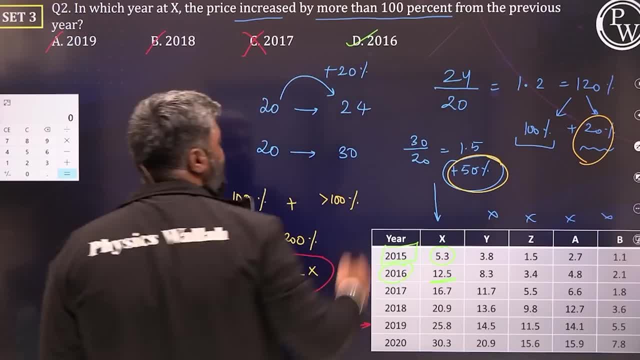 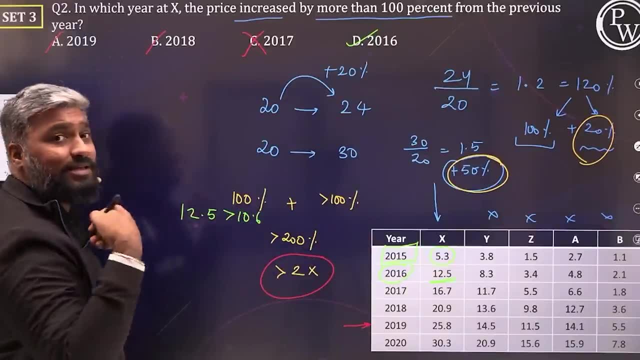 whether it is more than 10 point or it is more than 10.6. correct? this is our answer. are you getting this 12.5? yes, more than double of 5.3, which is 10.6, which means the increase is more than 100 percent. again, if you're still in doubt, 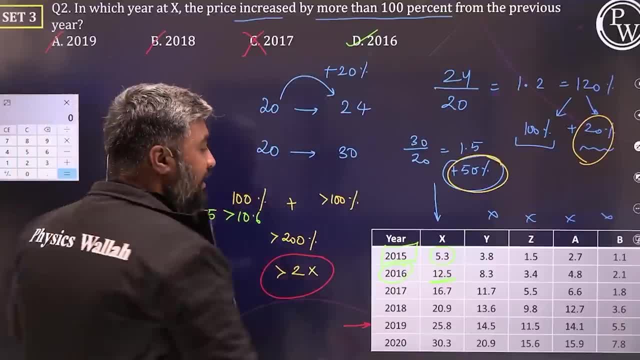 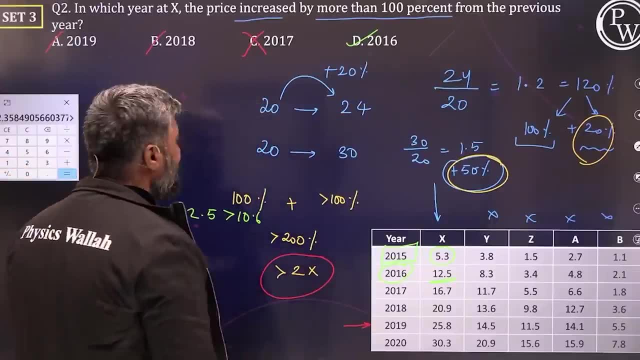 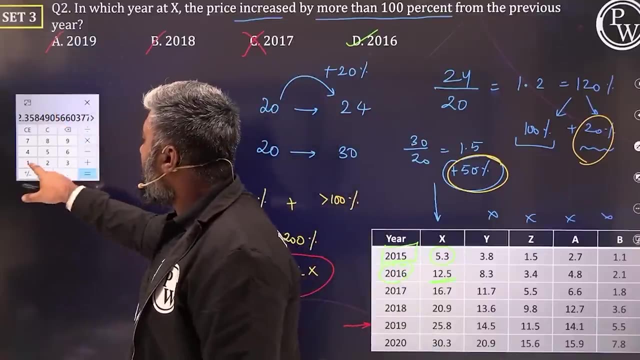 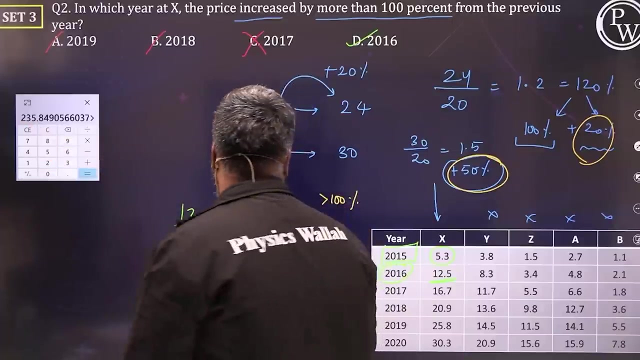 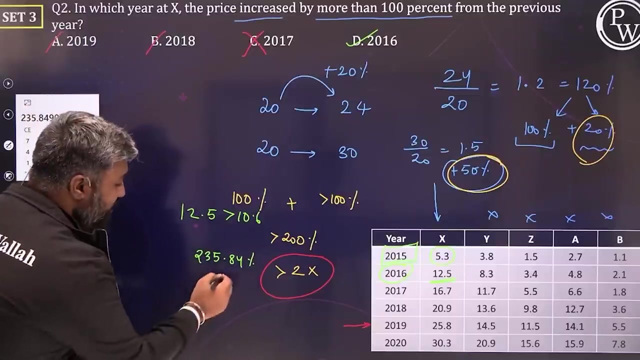 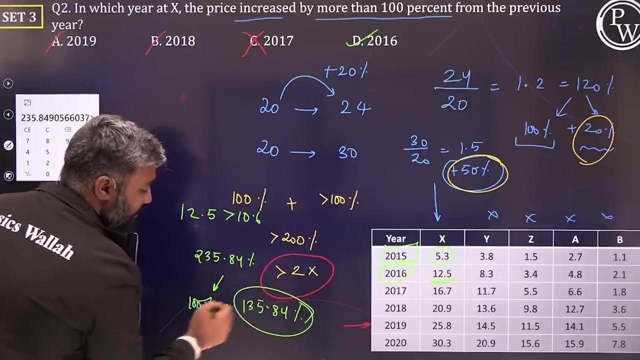 is: give 12.5 is 5.3. اص divide 12.5 with 5 by 3.. How much do I get? Into 100, we get 235.84.. Again, 100% was already there, plus remaining 135.84%. This is the increase. This was already there. This is. 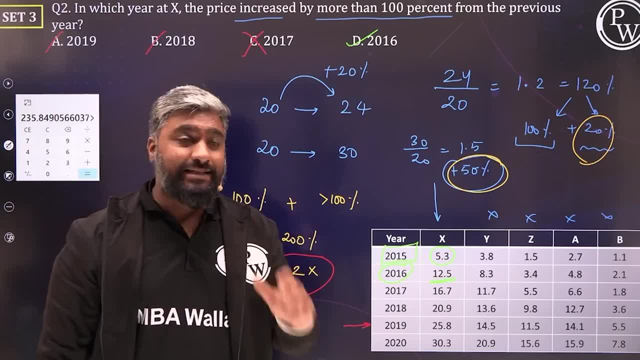 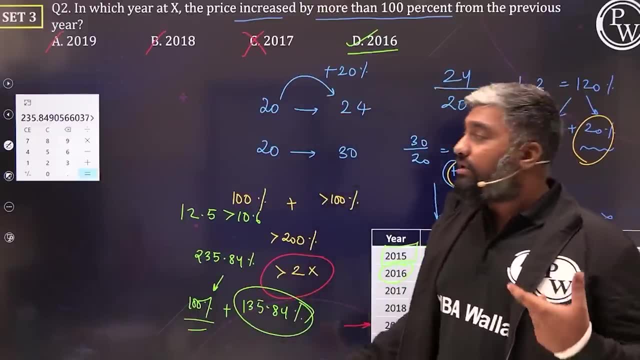 the increase Is 135.84 greater than 100?? Yes, it is. That is our answer. Hear it. Yes, You have to be very careful when it comes to increase decrease. You have to know how to craftily use the calculator. Calculator is given everywhere in most tests, But you 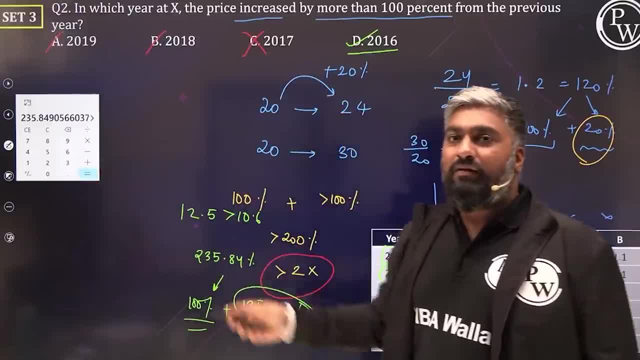 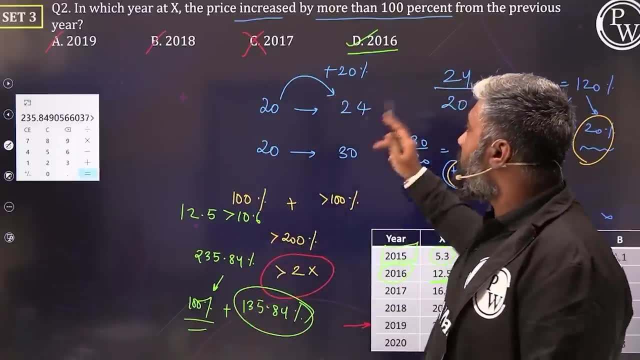 have to be careful enough to know how to use this in a creative way. Otherwise you will do the same thing. You will make a difference. divide it into 100.. It takes a lot of time. Chances of mistakes are also high. So use the right kind of logic Here. what did we? 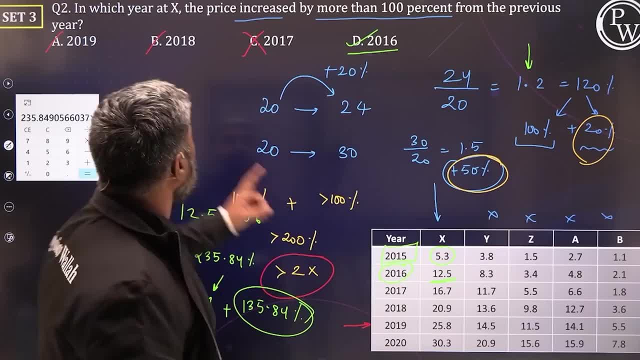 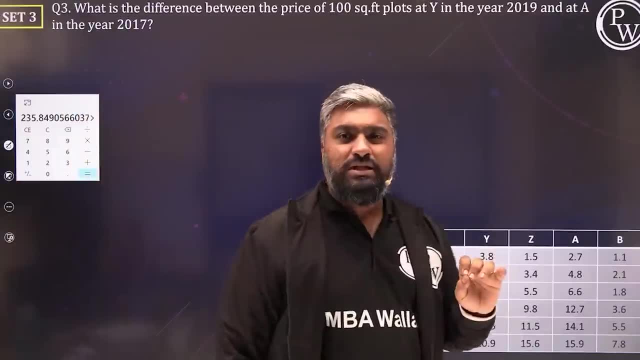 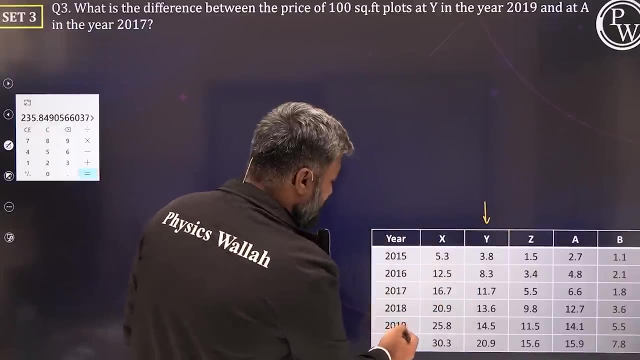 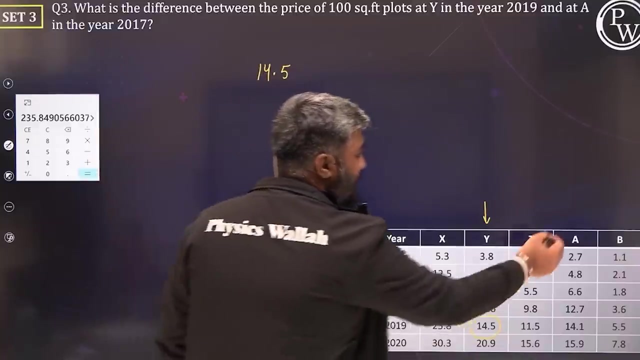 use Multiplicative factor: Cool Chalo. So this is the second question. Let's get ahead. Let's go to the next question now, Question number 3.. Difference pucha hai. Simple subtraction karna hai. What is the difference? 2009.. Y ka 2009.. 2019 is 14.5. And A in 2017.. A in 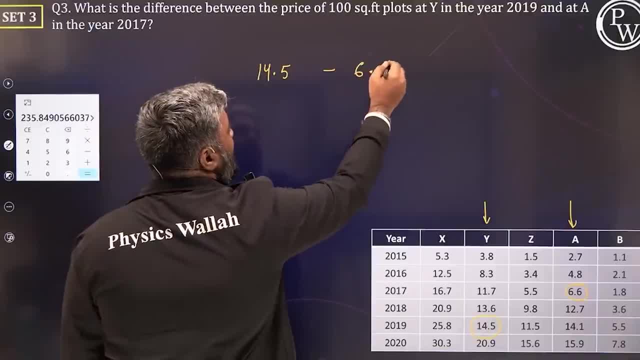 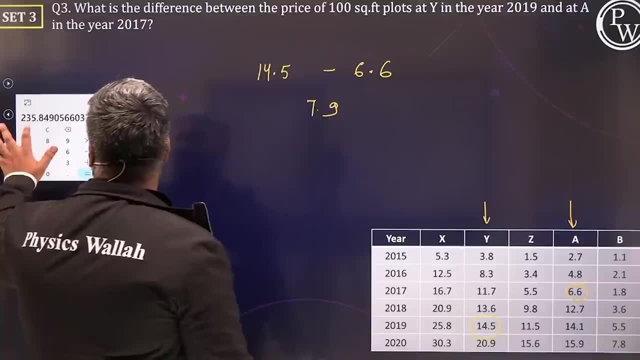 2017 is 6.6.. Subtract karo: What will you get? Calculator use karna hai. 7.9.. Chalo, Chalo. Thik hai. Use karne ka. 1. agar ho raha tha, kar lena Thik hai. Aapke mann mein aise nahi ho jana chahiye, ke sir calculator use kar. 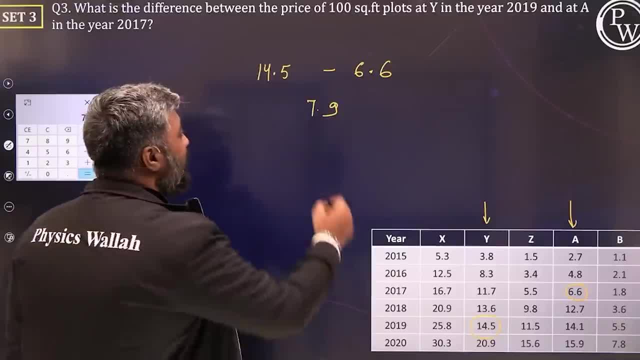 hi leta hai Risk, kyu lena hai? 7.9.. Okay, Now, this is a theta question. Walao is mein negative marking toh nahi hai. Kya is ka walao? yeh hai, ke mai kuch bhi answer likhe ajo. 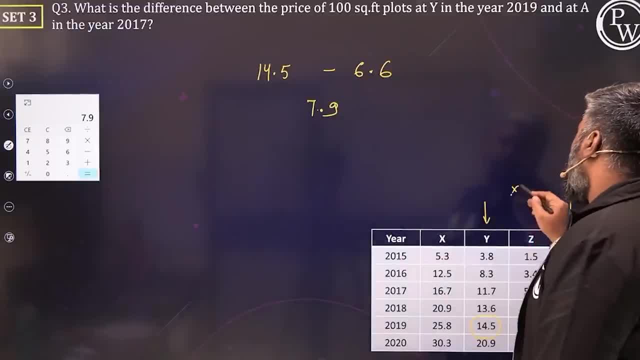 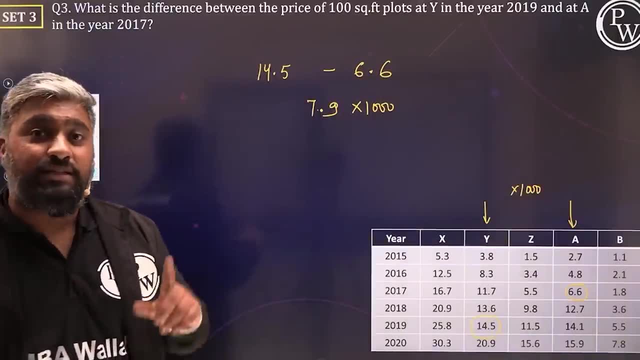 Kuch nahi dekhna. One thing we missed is what Scale In thousands hai yeh. So in 2000 toh hoga hi Right, But do you know what? We also made one more mistake, which is yeh kya. 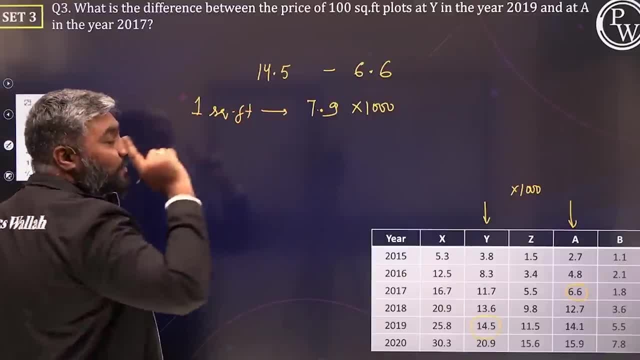 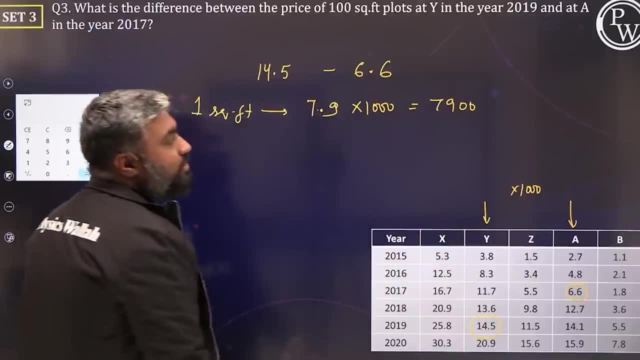 hai One square feet ka price hai. This is the price for one square feet, Not 7.9.. 7.9 in 2000, which is 7900 jo tha 7900 jo tha. that is price of one square feet. Question. 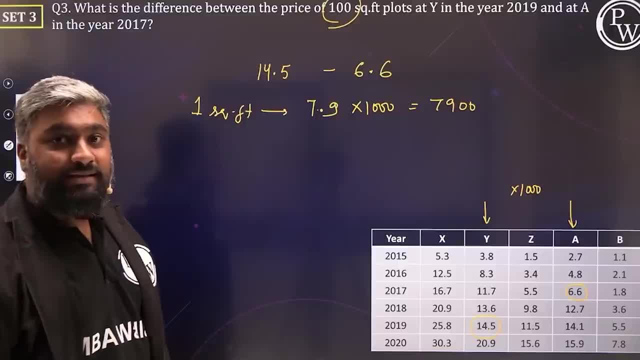 mein kya pucha hai? Hundred square feet pucha hai. Yes, Toda ka calculation karna hi pade nahi, yaha pe. Agar one ka itna hai, toh hundred ka kitna hoga? If this gets multiplied by: 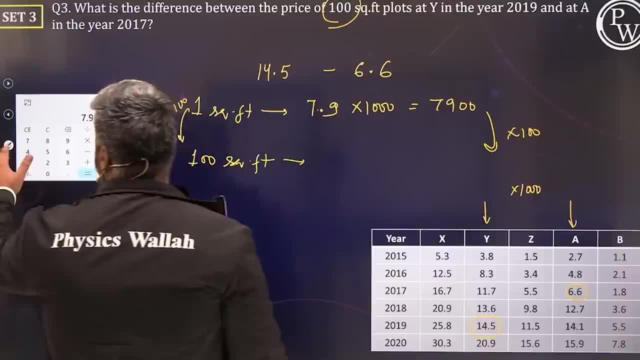 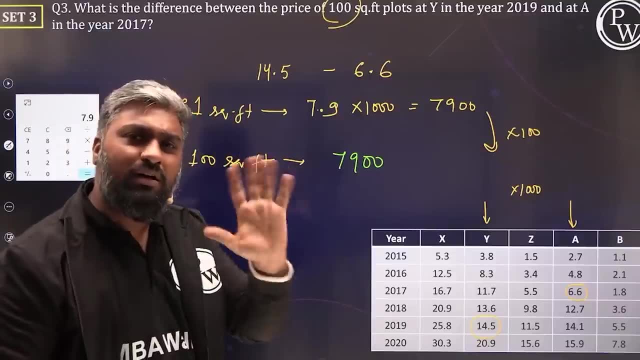 then this also gets multiplied by hundred. Am I right? Simple calculation hai: Hundred se multiply. karlo. Yaha pe na Here, it is okay, even if you are going to the ground level. Bacho jase karo Zero finger pe count, karlo, Koi dikht hai? Nobody is judging you, Aap. 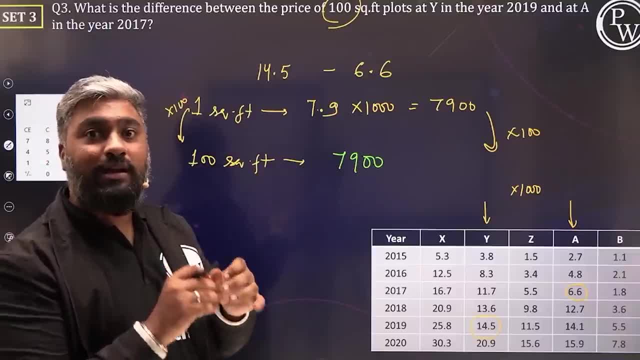 apni taraf se sahi kar raha ho. That's enough. Koi aapko judge nahi kar raha ki. Yeh toh zero finger pe kin raha. Yeh kya kar raha? No. 1, 2, 3, 4.. 1, 2 ho gaya 3, 4.. This. 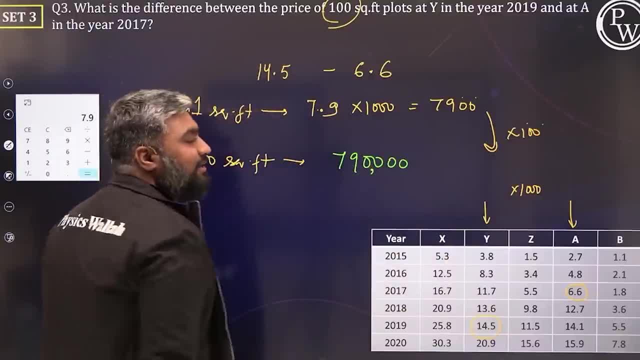 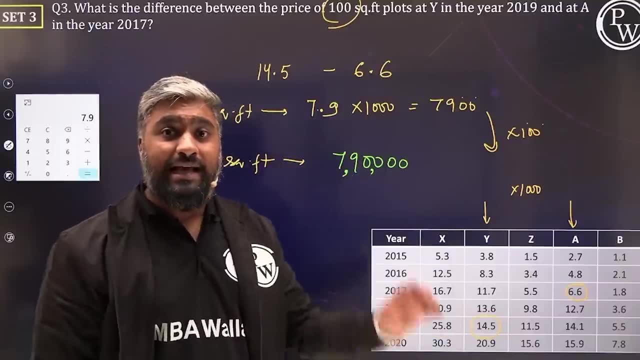 is our answer, Which is how much? 790,000 or 7,90,000.. Jo bhi, Whatever you are using, 790,000 or 790,000.. Either which ways, That is our answer. Samin maa gaya. Yes, So the price of 100 square feet. 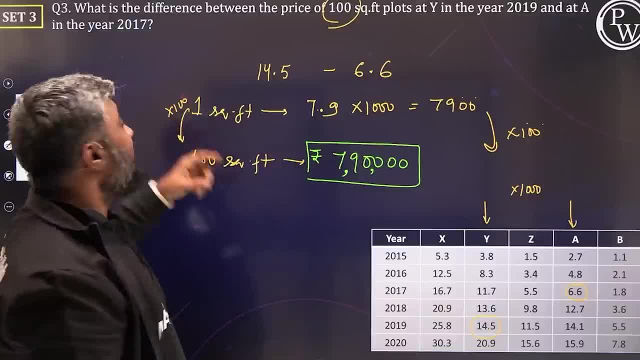 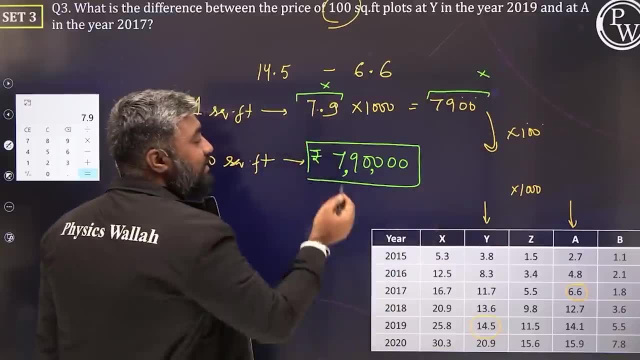 land at Y in 2019 and A in 2017.. Iska difference kitna hai Not 7.9.. 7.9 nahi, 7,900 nahi. Instead, it is what 7,90,000.. Samin maa gaya? Yes, Theta question hai toh negative marks. 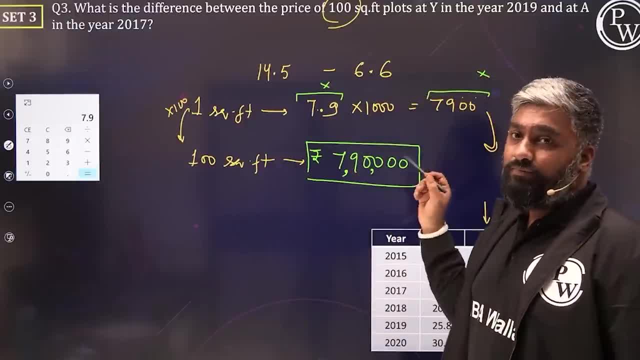 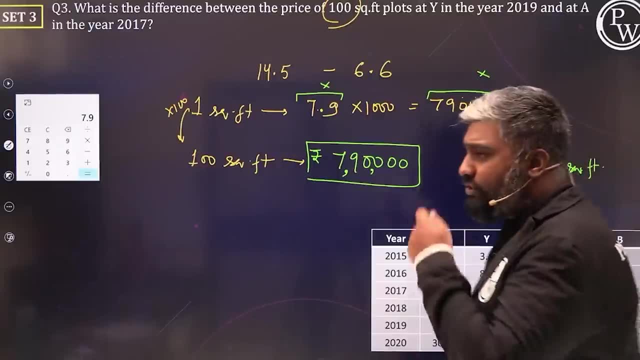 toh nahi aayega. but yeh easy 3 marks chale jaate hai haad se, agar hum, if we were not careful, Yes, Rough sheet hai Rough sheet mein likke rakho: Thousand for what One square feet? Mujh bhi aapko table mein instructions, mein question, mein important information dikhe. 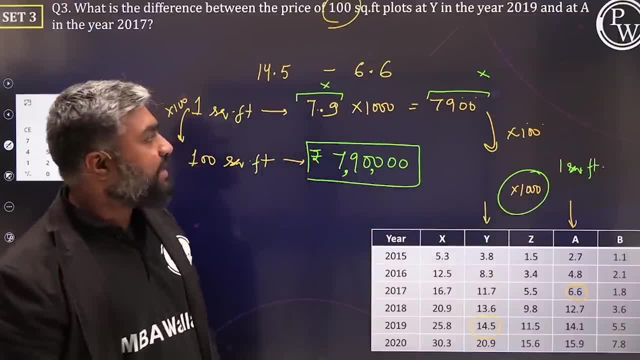 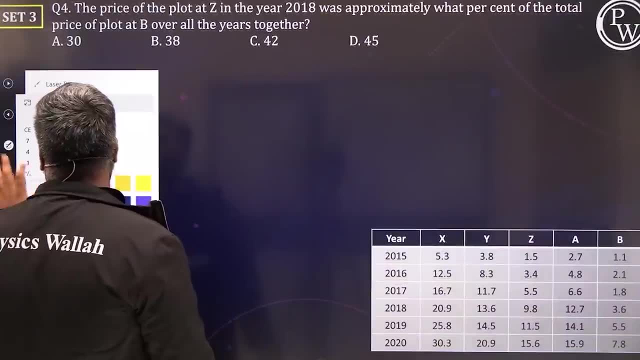 Make a note of it. on the rough sheet that you have Say yeh: Yes, Beautiful guys. Jinone answer 7.9 or 7,900, kar hai. Hope you understood this. Yes, Beautiful, Let's go for the fourth. 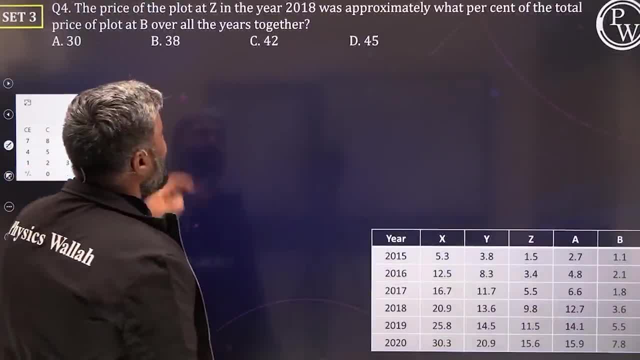 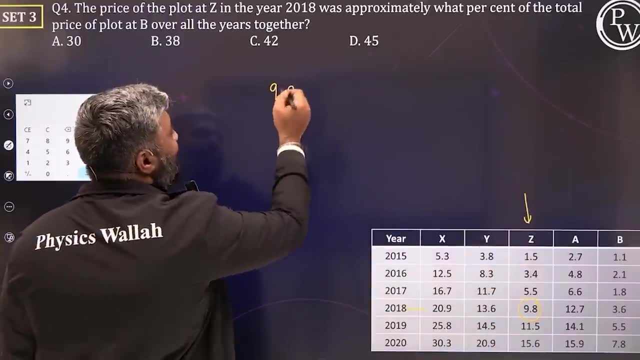 question, Question number 4.. On the screen, The price of the plot at Z in year 2018.. Z yeh raha, 2018 yeh raha, Which is 9.8.. Gyan mein rakho One square feet ka hai in thousands. 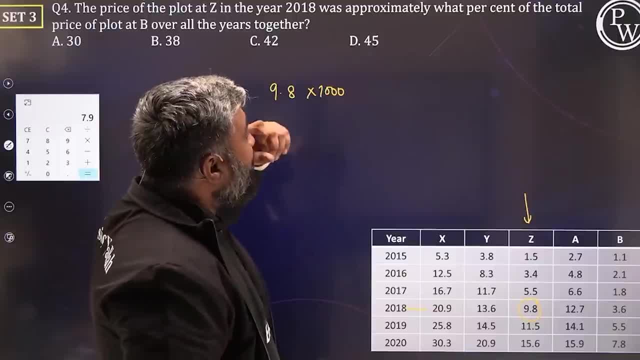 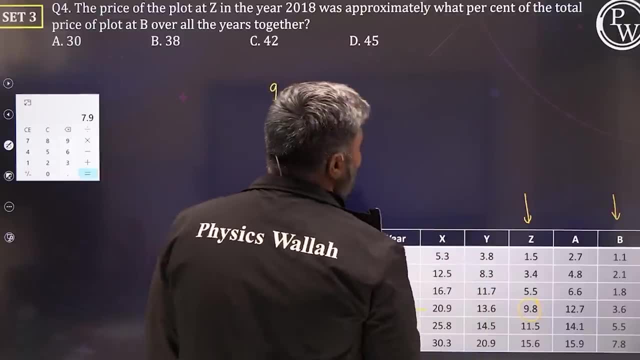 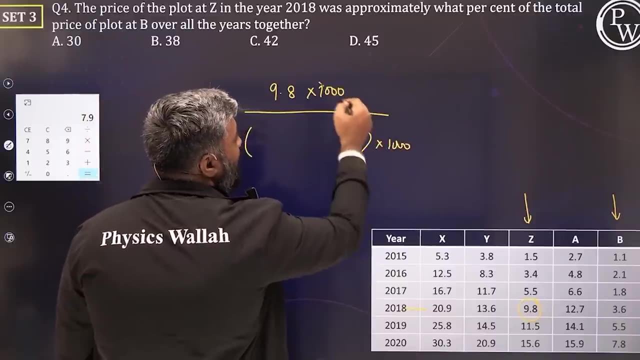 A was approximately what percentage of the total price of the plot at B? B ka total mein kitna tha puch raha hai Toh percentage comparison hai scale ki zarad nahi hai. Jo bhi aap yaha pe add karoge, B ke liye, aap jo bhi total add karoge, Ose waise bhi into thousand karoge. 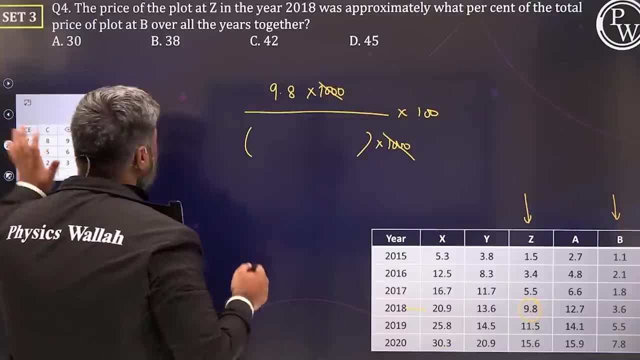 Toh yeh cancel ho gaya. Percentage value dhunni hai. Simple sa question hai: Hina, add ke add kar raha hai. If you want to manually add it, add Risk nahi lena hai. Calculator use karna hai. Calculator use karlo, Yes, Scale nikalna hai, Scale nikal lo, But yeh raha. 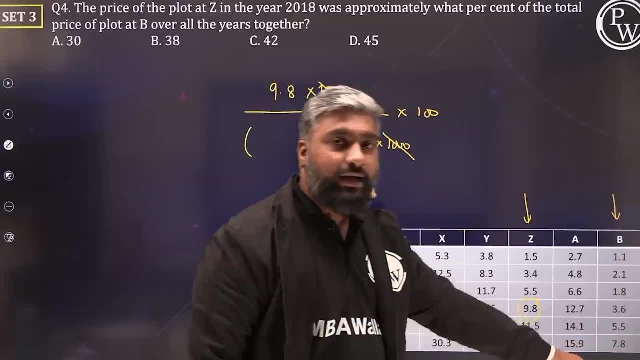 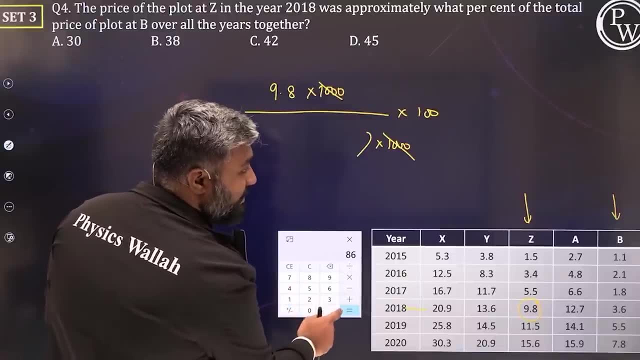 Point, one, point, point. point hai Decimal ko cancel out karna hai. Cancel out, karlo. So you have 11 plus 21 plus 18 plus 36 plus 55 and 78.. Adds up to 219.. Decimal mein kya ho? 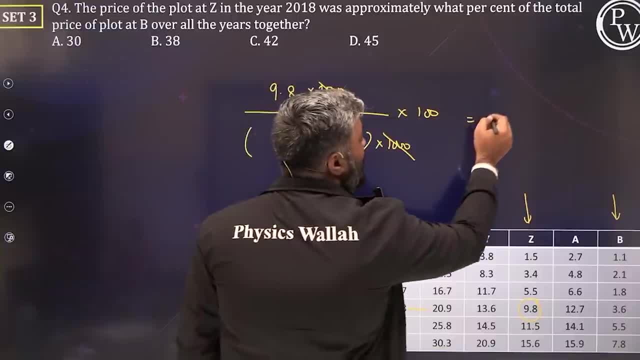 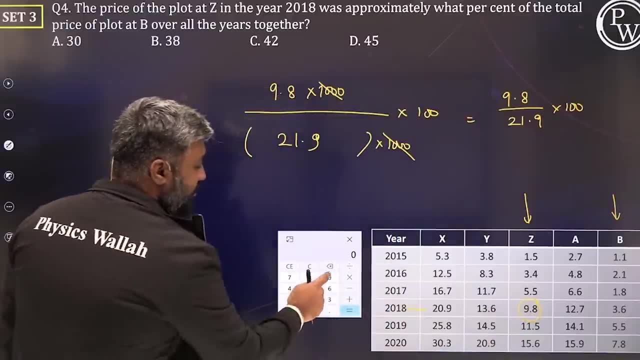 jaga 21.9.. Yes, So our answer is supposed to be what? 9.8 by 21.9 into 100.. Decimal agar upar niche dono se nikalna hai. So it is 98 divided by 219.. Yes, So our answer is. 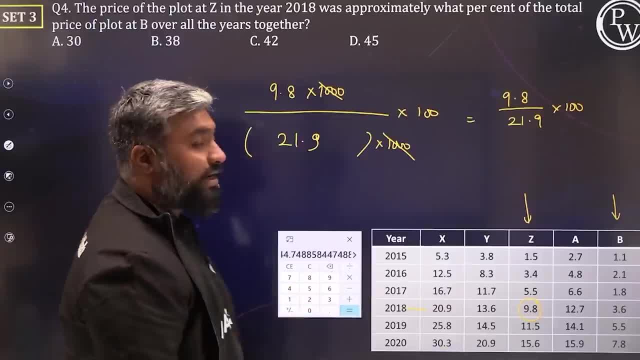 supposed to be what? 9.8 by 21.9 into 100.. Decimal agar upar niche dono se nikalna hai. So it is 98 divided by 219 into 100.. Approximation karne ka agar man ho raha hai. Look at this. 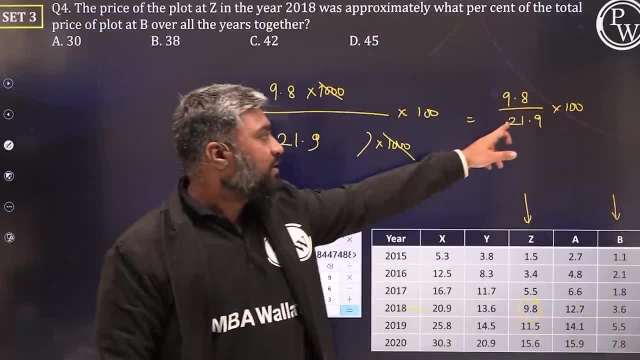 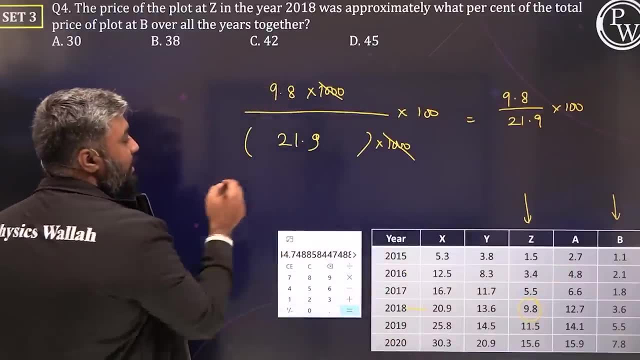 9.8 approximately is 10.. 21.9 approximately is 12. 10 by 12 karna hai approximation. Tike ek baar approximation bata deta hu ma apko: 9.8 approximately 10 hai 21.9 approximately. 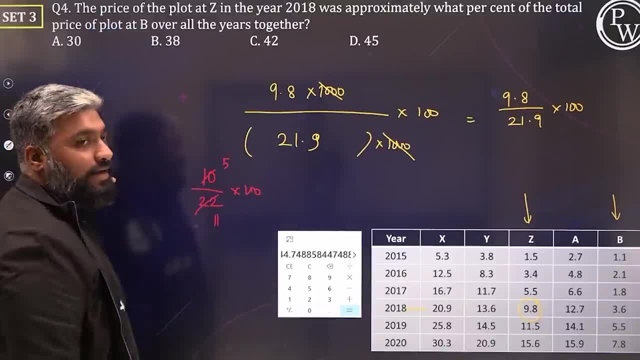 22 hai into 100.. This is how much: 5 by 11.. Yes, 1 by 11 is 9.09 percentage. Yeh bhi amne baat kareeti first lecture, mein Lecture 1.. This is how much: 5 by 11.. Yes, 1 by 11.. 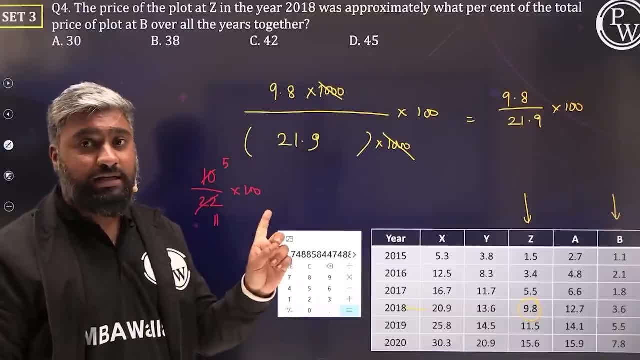 Yes, 9.09 percentage. Yeh bhi amne baat kareeti first lecture mein Lecture 1.. This is how much Of the foundation batch for LRDI. We spoke about this calculation part also, So 5 by 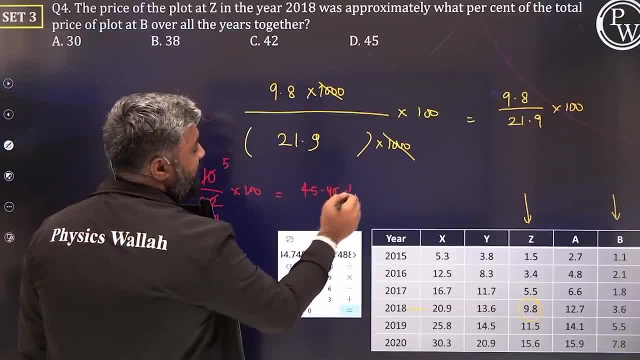 11. kya hoga? 5 into 9 is 45. So 45.45 percentage. Our answer should be more than this, Nahi Less than this. Why? Aur very close to it, Kyunki amne numerator bhi bada hai denominator. 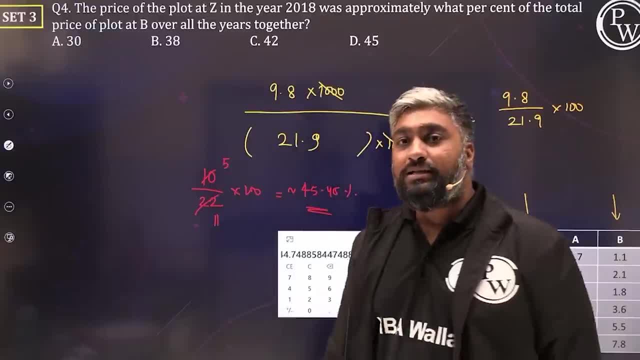 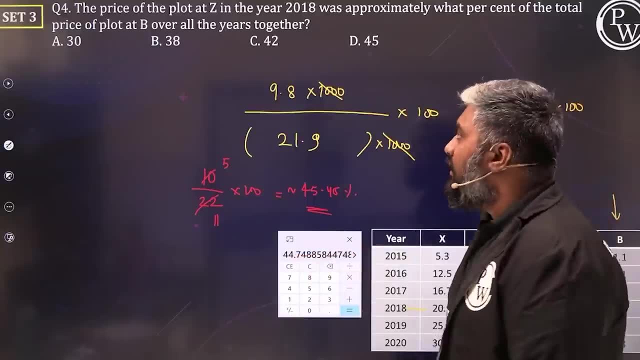 bhi bada hai, So our answer should be very close to 45.45.. But aapko agar risk nahi lena hai, So aap calculator dekh loga hai. We got 44.7488, which is 44.75.. 44.75 is the accurate. 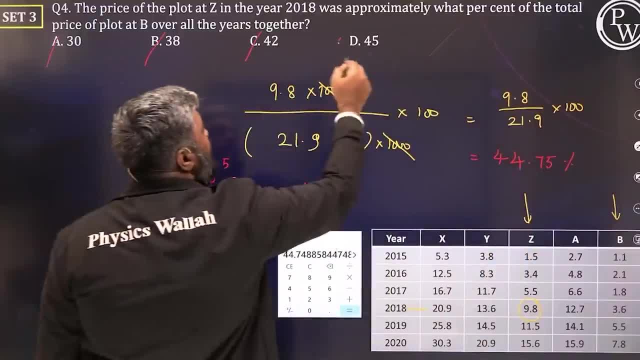 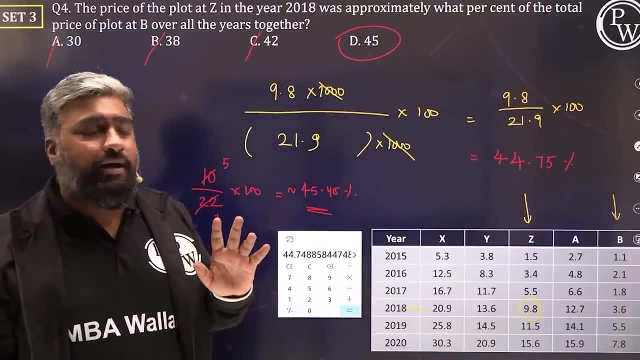 answer 42, 2 less 38, 2 less 32 less. closest answer is 45. So whether you approximate or you use the calculator, Wo choice mein aapke chhota ho. That decision I think you can make, But the selection of answer choice is that Thik hai. So this was our fourth question. 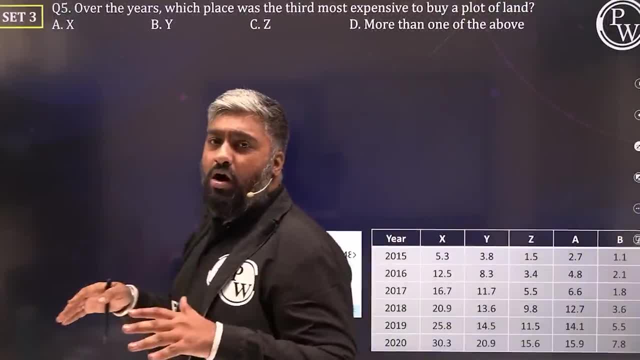 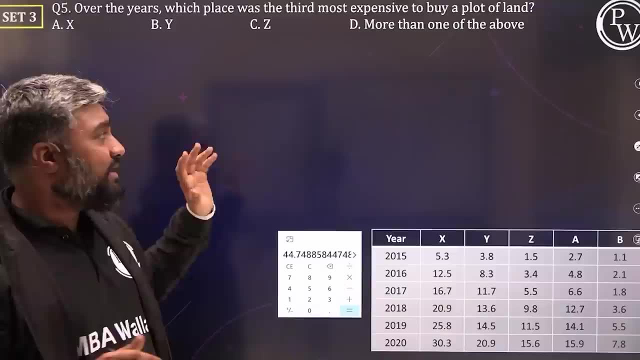 Let's go for the last question of the day. This is going to be the end of the first third lecture. First lecture on tables hai, basically the only lecture on tables. So the third lecture of LRDI foundation batch. Last question: Calculator: refresh maro. Let's read the question Over. 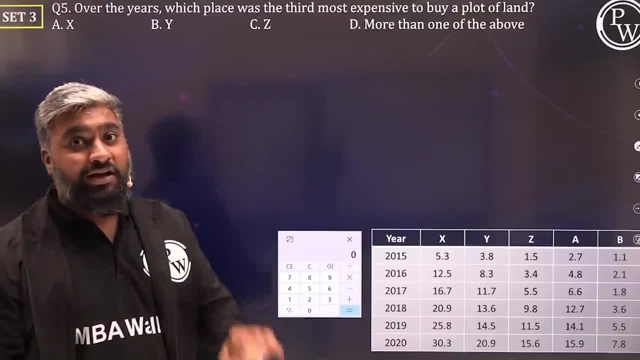 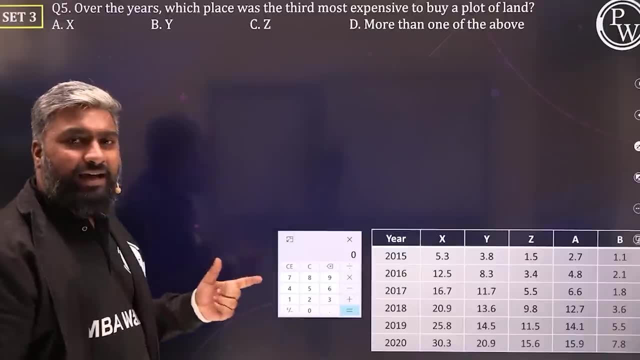 The years. which place was the third most expensive to buy a plot of land? Again, do you remember first, second, third, humne pehle bhi kara tha Third most expensive is what Expensive, Second expensive, third expensive, right Rank karna hai. looking at the prices, calculator ki zarat. 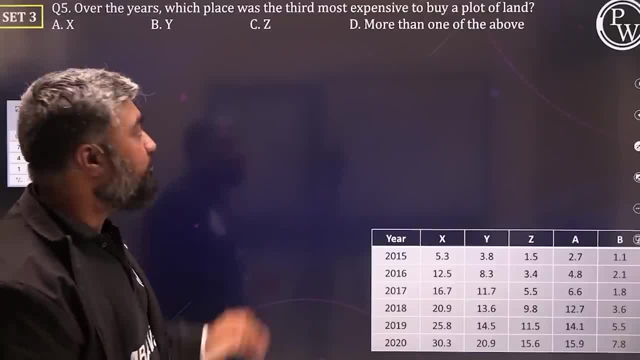 nahi Bhai tu nikal, Yes, ina kar diya Side mein pop chhe mein dal diya Over the years, which means koi particular year ka nahi. bol raha hai Pura Full 30 pieces of information. 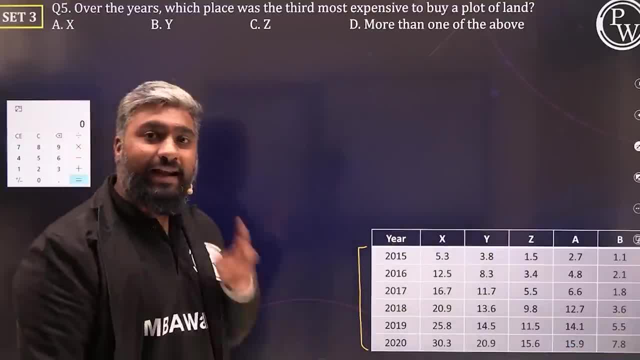 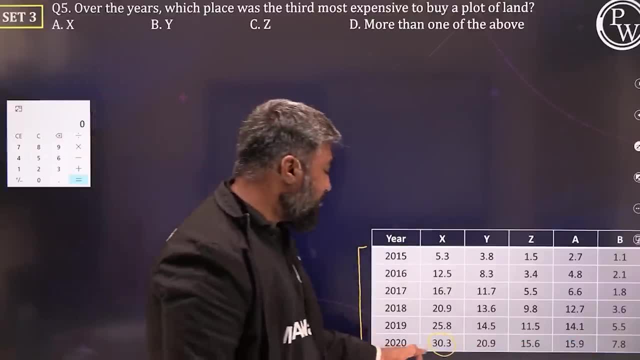 we have to look at- Yes, We have to look at- the third most expensive Analyze and answer Khatam Sabse expensive. aapko kana dikh raha hai Sabse expensive. yaha pe See, you should have noticed ki mein directly 2020 ko hi dekh. 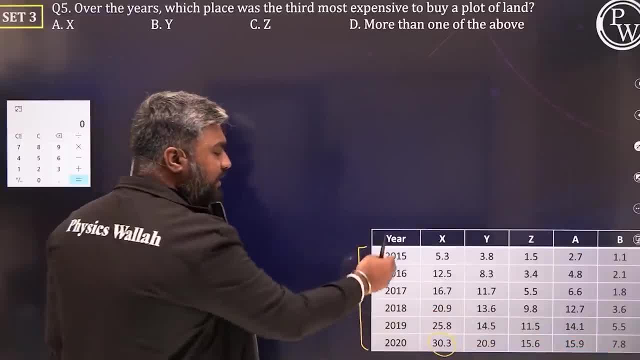 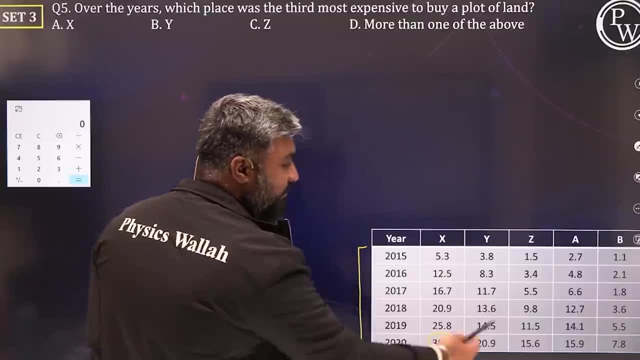 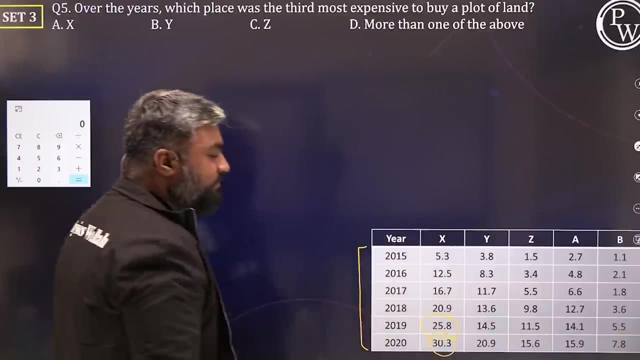 raha hu, Kuki of the entire year, Of the entire period for a particular place Most expensive. last year Kuki sab kuch consistently increase ho raha tha First top expensive, Next Second expensive, yeh raha 25.8.. Kuki 25 se bada aur koi value nahi hai. 20, 15,, 15,, 7 nahi hai. 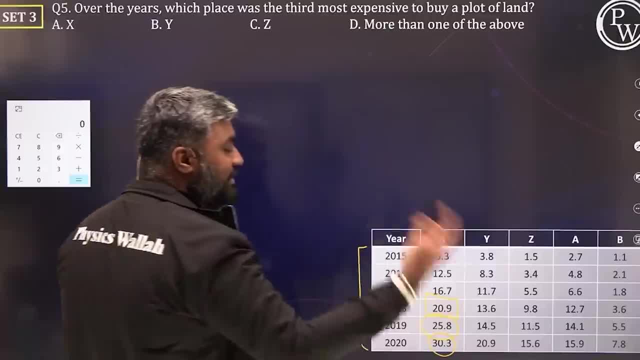 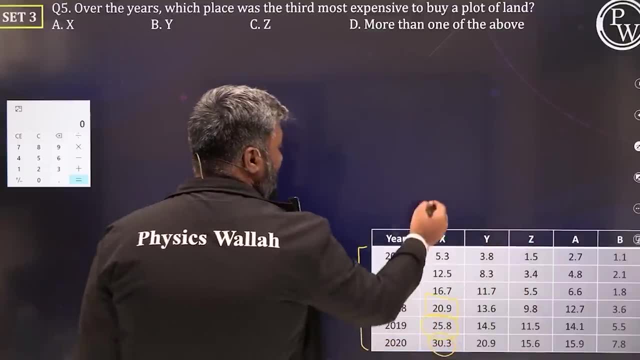 Next, the third expensive, is going to be what 20.9.. 20.9 se bada koi value hai kah, yeh pe 20.9 se bada nahi hai. But Jaldi, jaldi mein, aap kya karo ki yaha pe 20.9.. Kidhar hai. 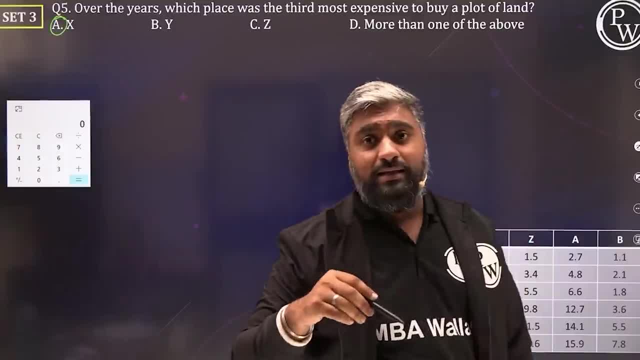 X mein hai Select kiya hai. Aaga hai. No, Don't make this mistake Right. Jaldi ka kaam, shaitaan ka kaam. Let's not do shaitaan ka kaam. Let shaitaan do his own kaam. 20.9 idhar. 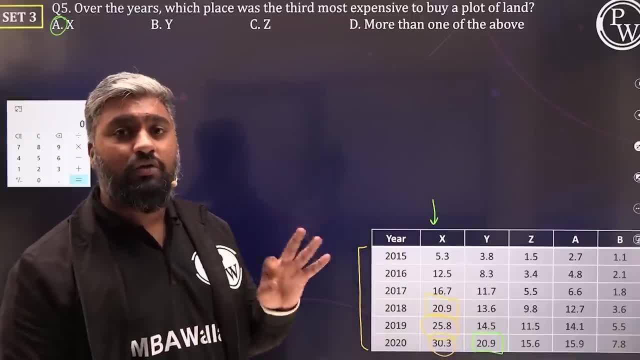 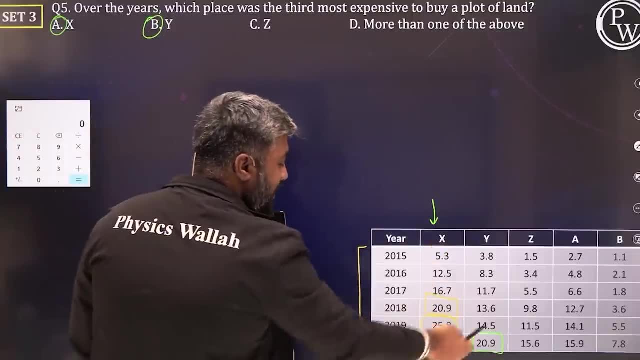 bhi hai, idhar bhi hai, So you have to be very careful. The third highest, The third most expensive is not only X, but also Y, Although they were in two different periods. X was in 2018.. Y was in 2020.. But kuki, over the years, bol hai Pura 30 pieces of information. 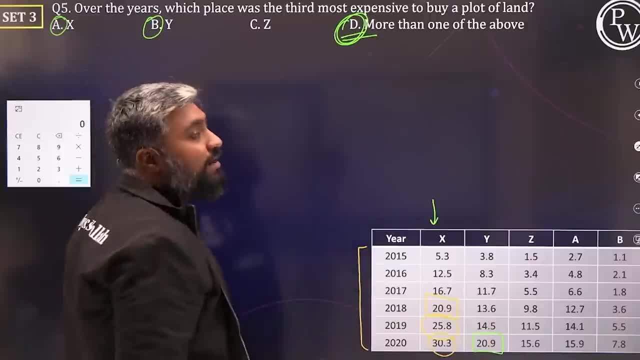 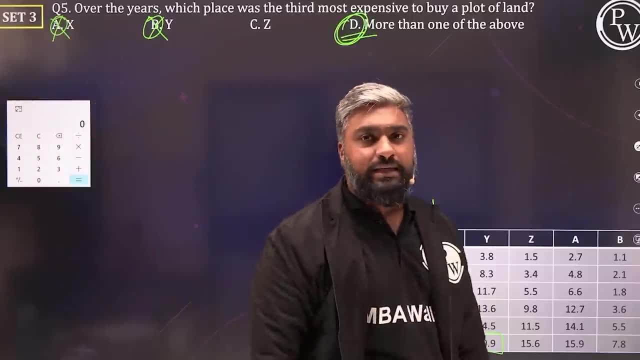 ko compare karne ko bula hai. The correct answer is going to be more than one of the above. Kuki X bhi hai, Y bhi hai. Option B, option A nahi hoga amara answer. Our answer will be option D: Theek hai. Yes, so do not forget, when you look at the chart, also read the questions. 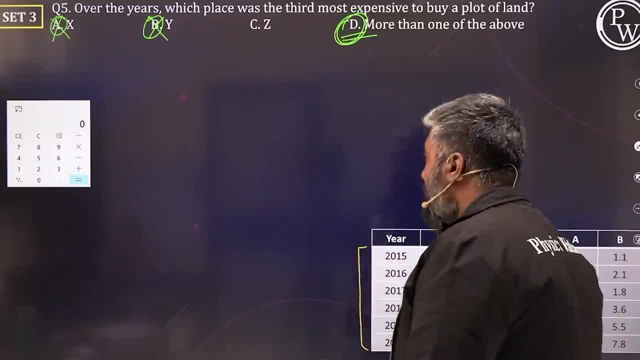 and the answer choices also carefully Jaldi. jaldi hum kya karte Question padte. answer dhunte select karte nikal lete Ghar jaake Phir ek do hafne baad jab amara. response sheet. 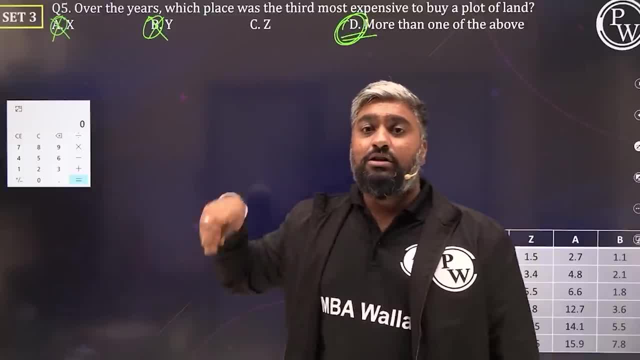 aata hai, tab hume bata chalta hai, ki yeh galti apne karli jaldi jaldi mein. Yes, So this is also an analyzed type answer: Yes, Question data ko. analyzed type answer: Yes, Question data. 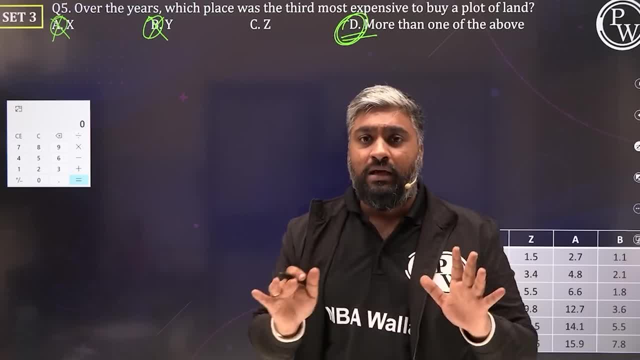 ko analyzed karo, answer karo kaam satham. No need to use a pen and a paper and a calculator, Nothing. So aaj hume kya dekha. Today we saw two types of questions that can be asked in. 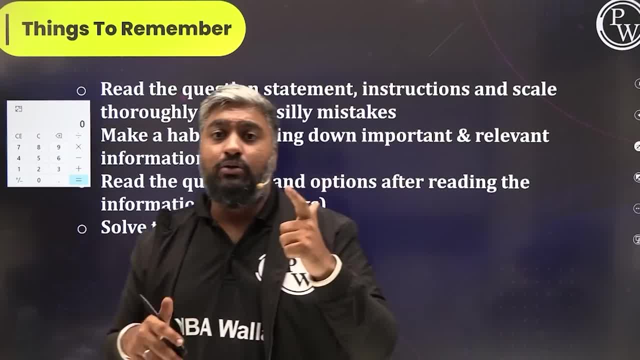 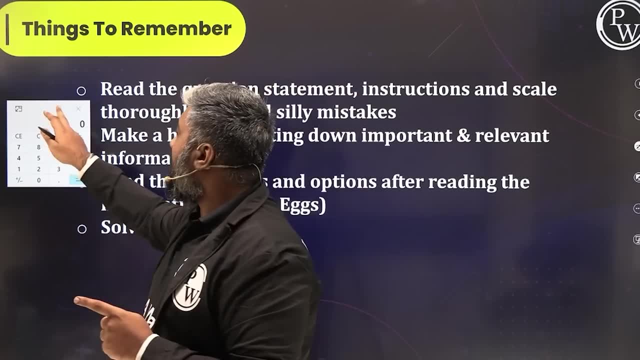 data interpretation. Right One: calculative hai Yes. Number two: analyze and answer. Look out for analyze and answer wale questions Jaha gayi par bhi aapko dikhe. Start using them to ensure ke aapka jo time hai wo kaafi saara bach jaye. Number two: we used calculator. 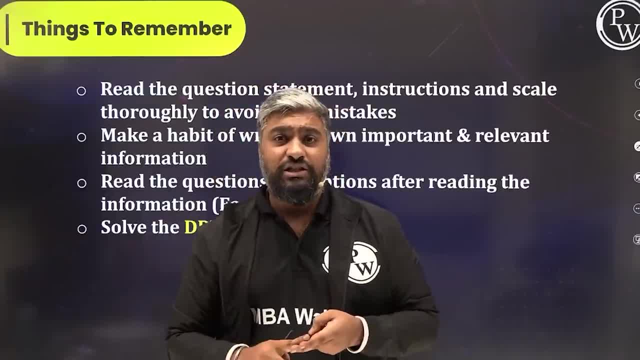 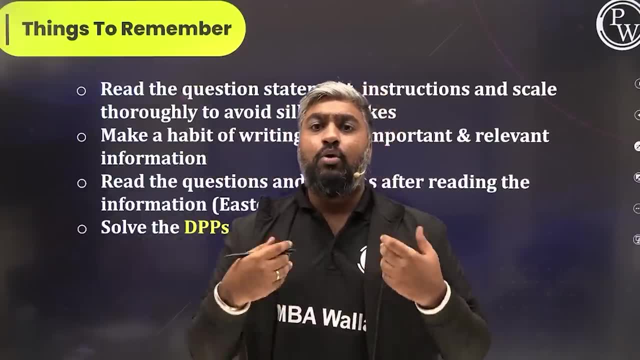 wherever possible. Humne koi masti nahi ki koi speed maths, calculation tricks, square nikalne ki tricks, yeh wo, yeh wo. calculation, multiplication, division, Koi tricks nahi kari, kyun Karna hi nahi hai Right, Who do you want to prove? Whom do you want to? 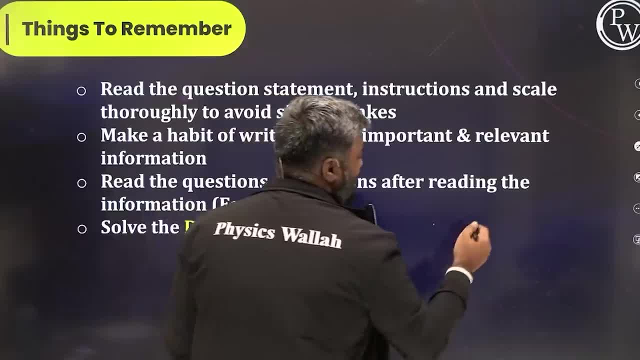 prove, ke aapko aata calculation, vedic maths, aata hai. Sir, main aaya aise calculation kar sakta hu. Do line aise kar di, teen line aise kar di, phir aise isko multiply ka diya. 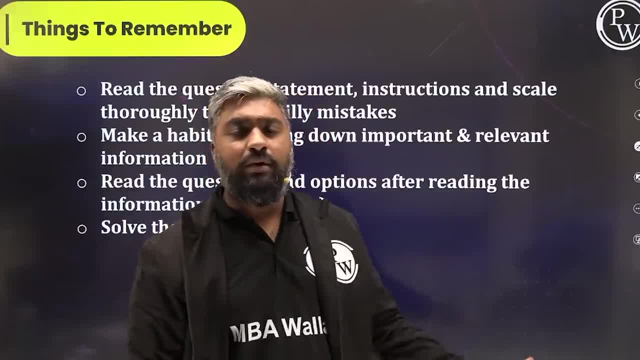 Phir yeh sab kya karoge? Nobody is going to see all of this. Yeh koi nahi dekha? Answer: hai sahi hai nahi hai wahi dekha, hai bas Yes, yeh sab karne se acha Calculator diya. 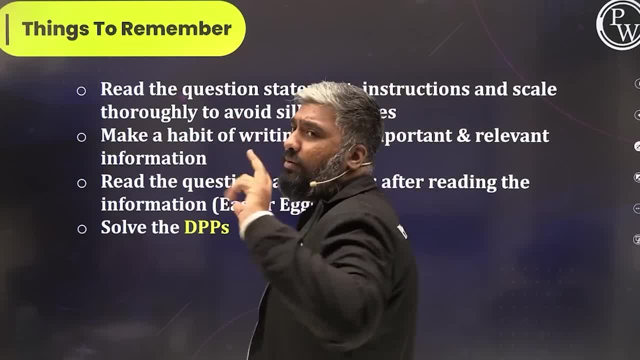 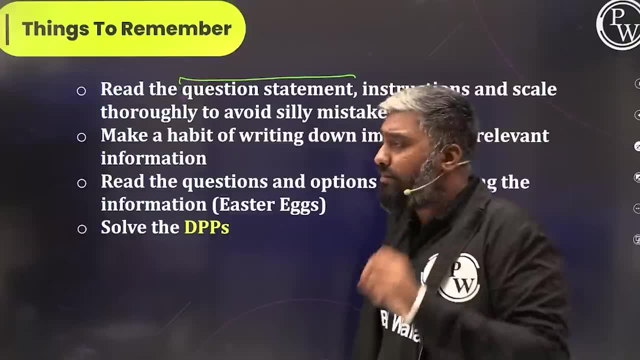 hai bhai, saab ko use karne Thike In things to remember. so we spoke about two important ones. Let's talk about more. Read the question statement very, very carefully, Bohot zyada. each and every word matters. Number two instructions bhi padho. Yes, table ke instructions. 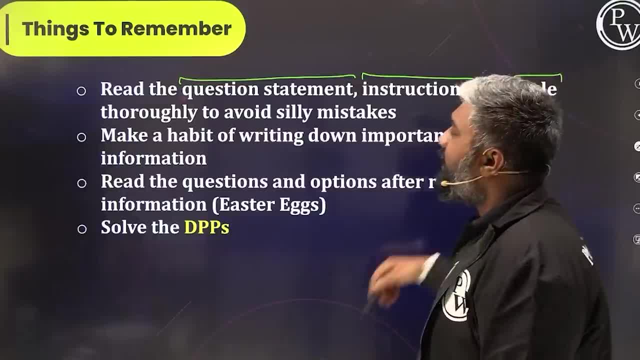 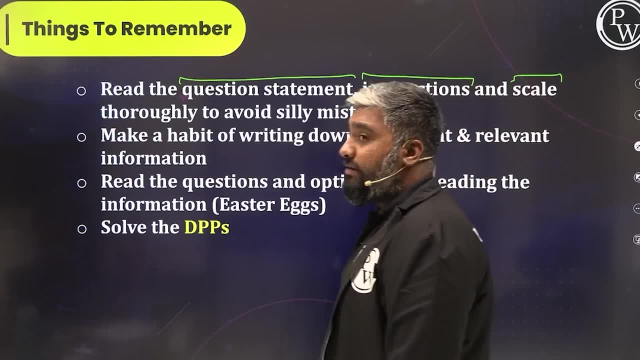 table ka: title rows, columns, everything. Do not forget to look at scale and the units. Scale and units very important, So watch silly mistakes. Next, make a habit of writing down important and relevant information. Yaa de One square feet, hundred square feet information. 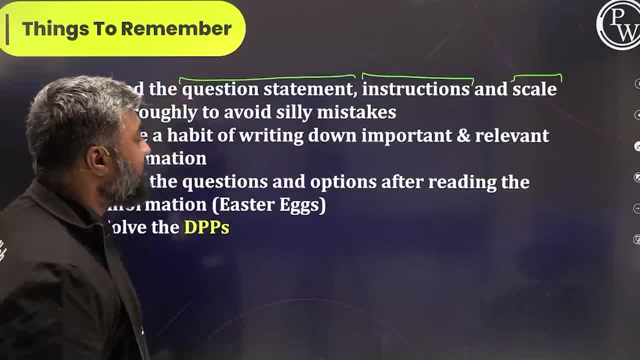 likho Jo zaruri hai, usse likho. Next read the questions and options, Toh aapko sirf chart nahi padna hai. Chart padte hi immediately. have a look at all the questions. Chart question. 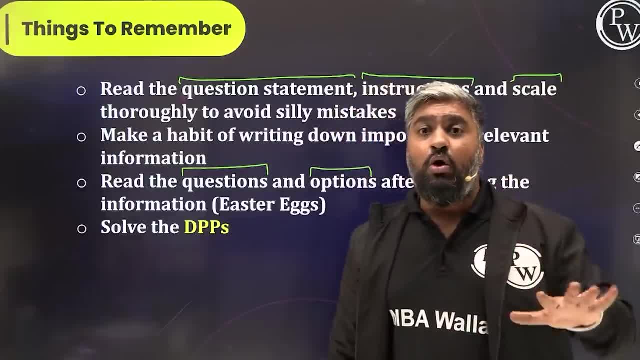 five question six question: jitte bhi diya. Have a look at the questions so that you know what you are supposed to do with the chart. Chart toh de de usse rakhe karna gaya Right That you will get from questions and 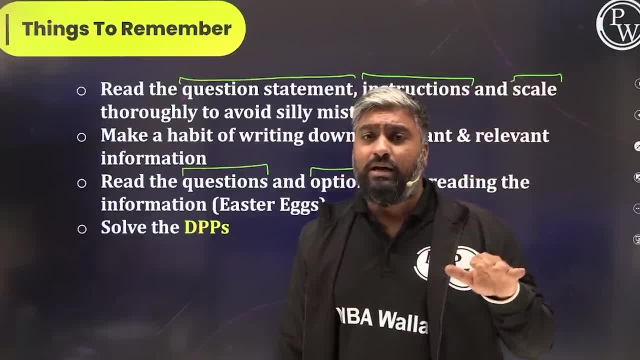 options. Have a look out on tita questions. Jahan kahi par bhi aapko tita questions dikhe, unhe dekho, Pata karo, ke kaunsa aise questions hai, jo aapko easy marks dilaa sakte Thike. 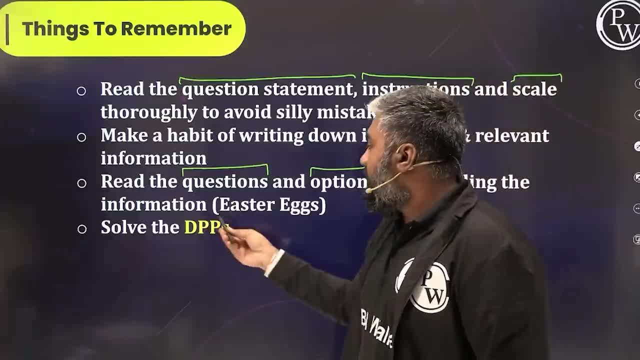 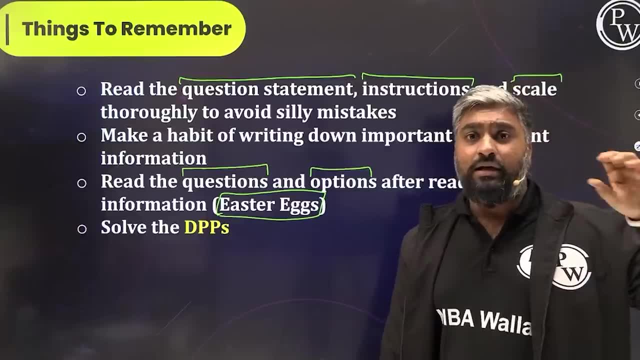 And analyze and answer wale questions ka bhi. look out pe rao Thike, These are called Easter eggs. kyunki kahi baad kya ho jaate hai. some pieces of data could be given in the question, Not in the, not in the set, not in the instructions. but koi information jo question me bhi de sakte. 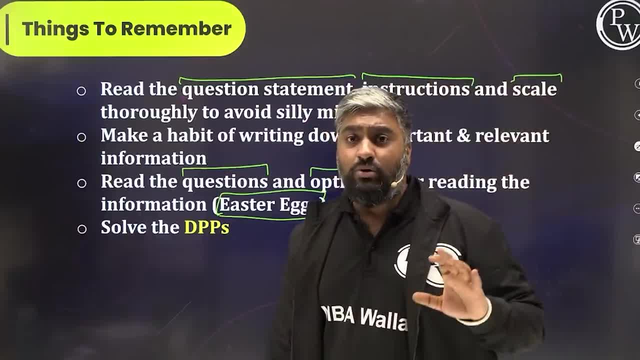 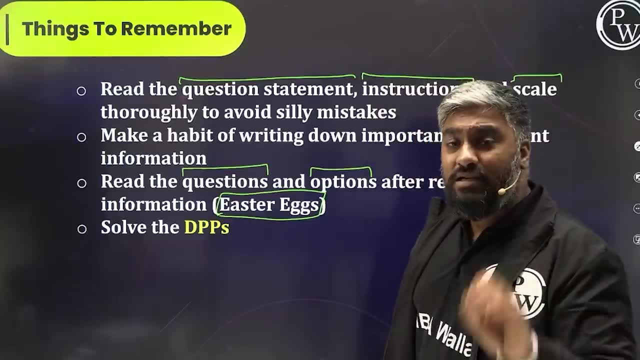 Easter eggs Towards the end, to ensure ke aapne jo bhi aaj kara hai, you are able to use all of those pieces of information, all of those strategies, tricks, tips, suggestions, advice. yeh sab aapke use aa rahe hain. Do it by solving DPPs Thike, Toh iss lecture ka DPP link aapko.